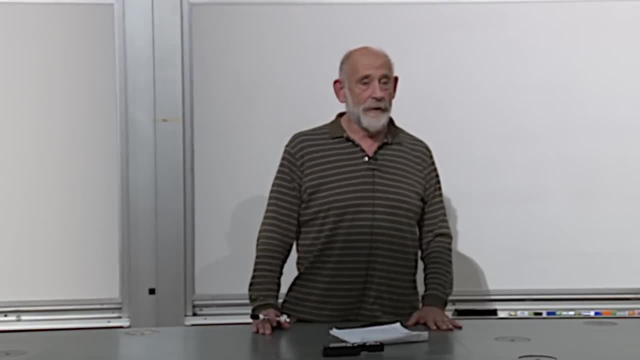 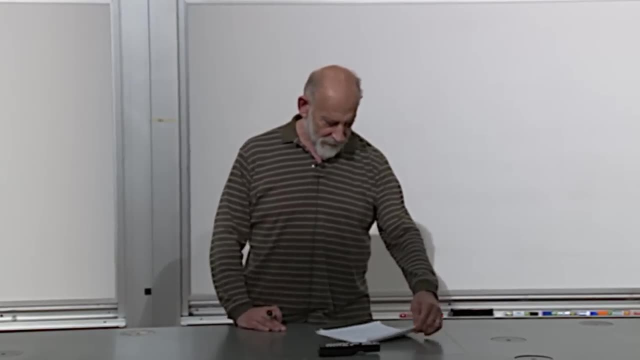 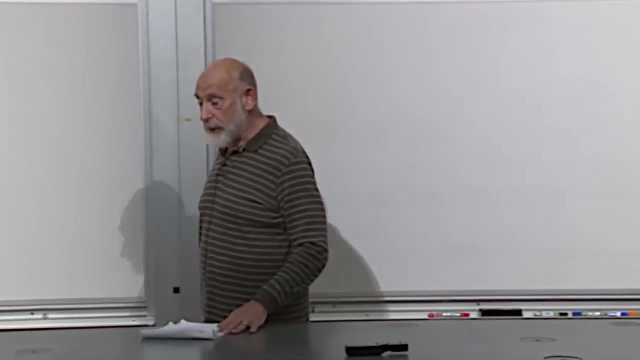 I'm going to do atoms first. And you say, how can I do atoms first before I do electrons? Electrons are part of atoms. It's all right, We'll do a little bit about electrons, just almost nothing, but just enough to be able to write down the basic equations of the hydrogen. 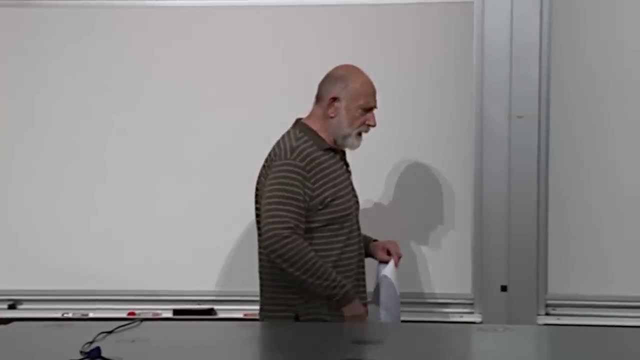 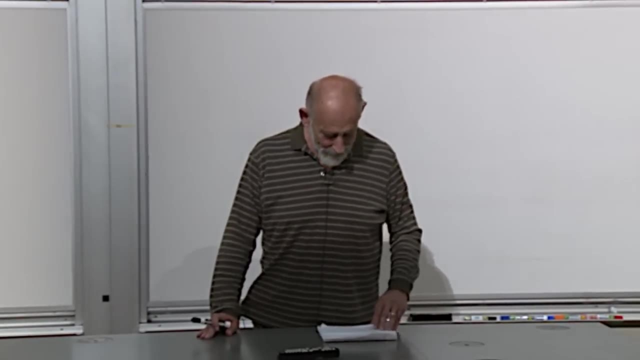 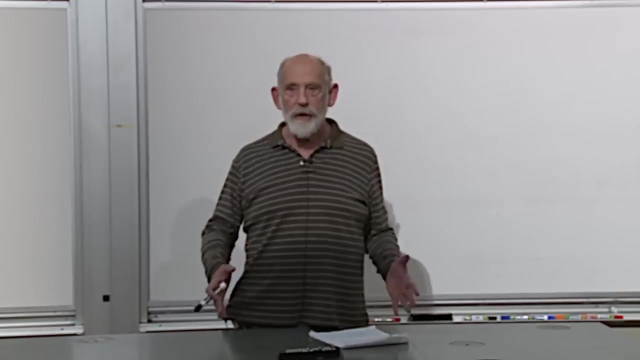 atom, discuss the hydrogen atom a little bit and then move on to further investigations of the electron. And when we say the electron, we're actually studying a class of particles, not just electrons, a wide class of particles which behave like electrons, which include: 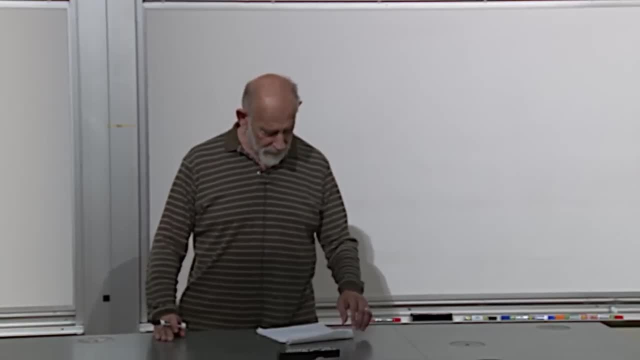 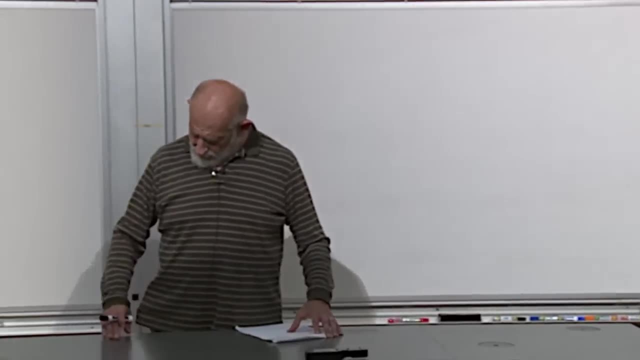 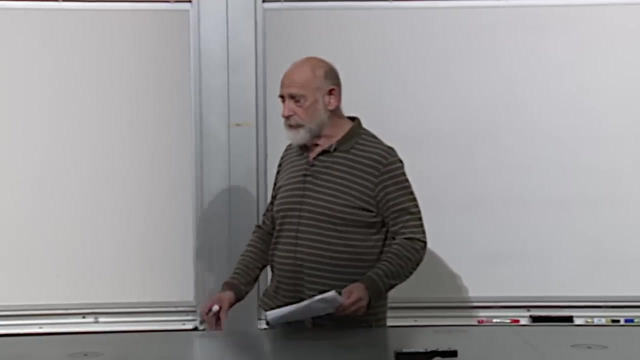 mu, particles, quarks, other things like that, and then the photon. So it's going to be atoms, electrons and photons. But one of the themes that will recur is symmetries- symmetries of nature and how symmetries are realized in quantum mechanics. how symmetries are represented. 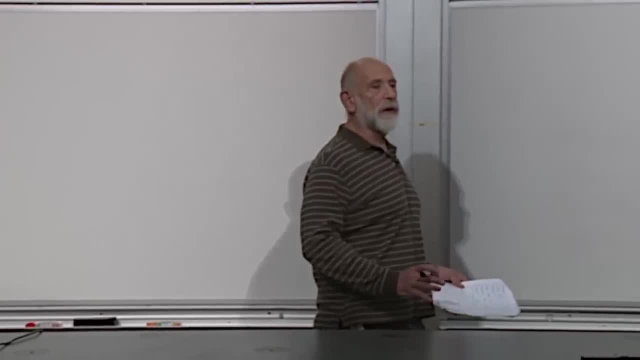 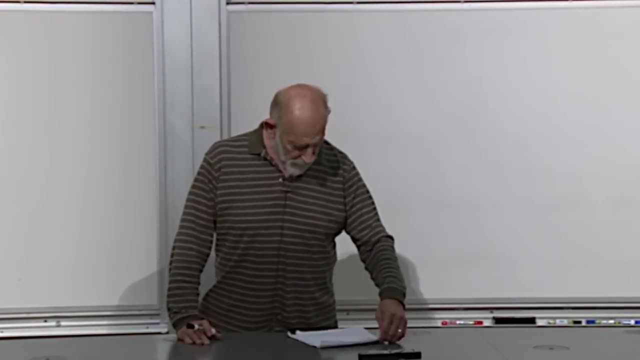 in quantum mechanics and what they tell us about the quantum mechanical system. Symmetries in quantum mechanics are an extremely powerful tool, which I'm going to tell you what a symmetry is. If you don't know what a symmetry is, that's okay. 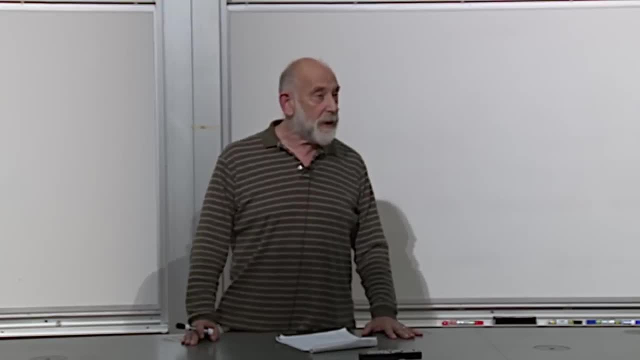 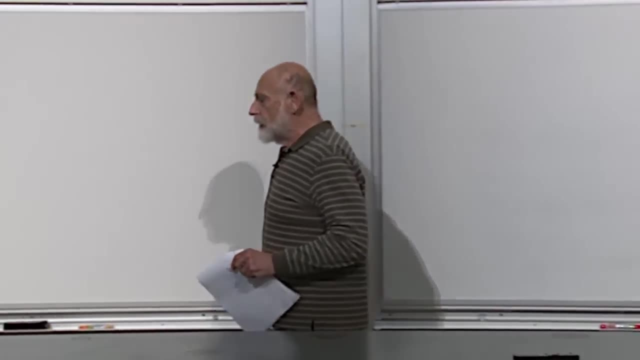 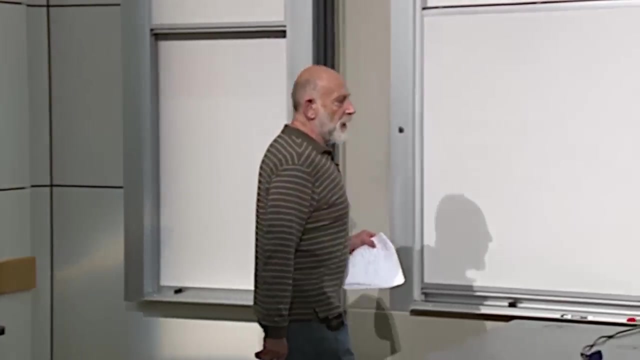 At the moment. But let's begin with a very, very lightening review of the last quarter of quantum mechanics. First of all, the whole story begins by asking: how do you represent the state of a system? We could go back a step and ask what is a system, but I'll assume 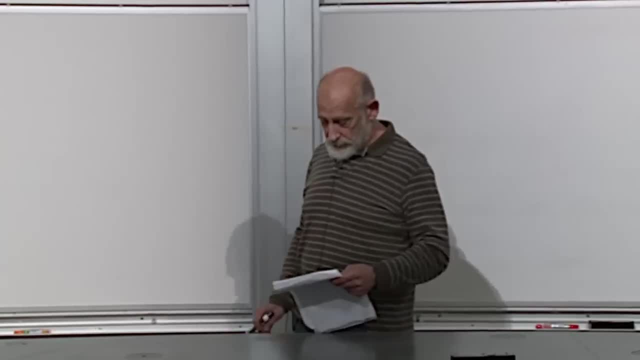 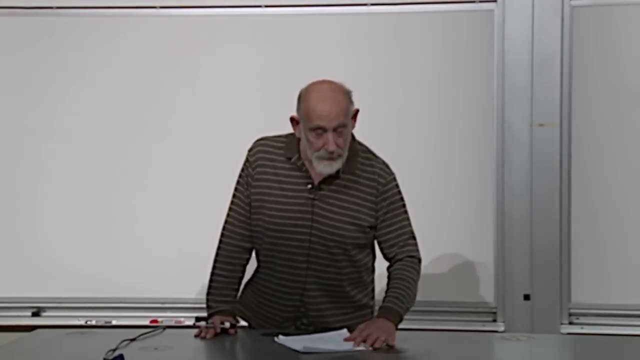 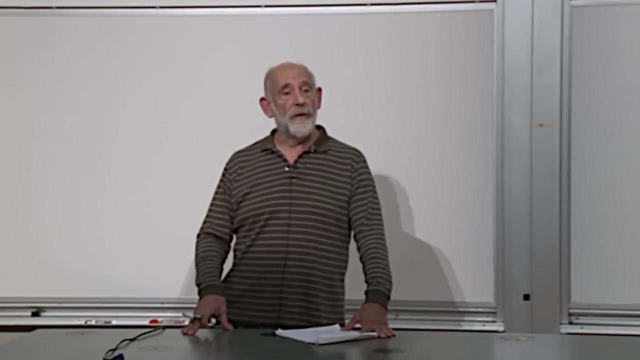 you know what a system is And how do you represent the states of a system. In classical mechanics the states of a system are represented as points In phase space. In quantum mechanics they're represented by state vectors. The idea of a vector is not a vector like a pointer in space pointing in a certain direction in space. 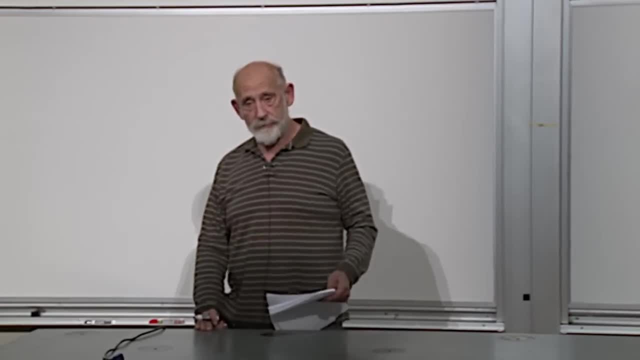 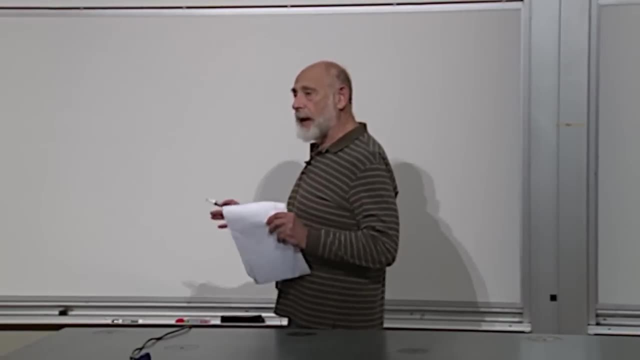 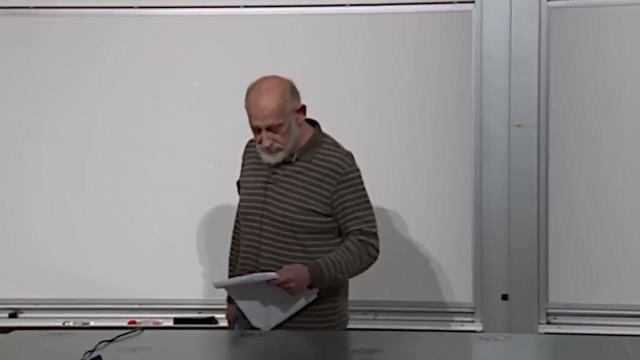 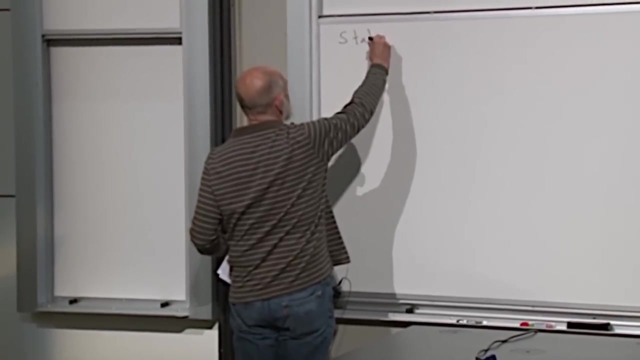 It's an abstract notion. You can add vectors, You can multiply them by constants And the mathematical structure of a state vector is a mathematical vector in a vector space. The vector space is not three-dimensional, except in special cases It could be any-dimensional. So we represent states by state vectors And the symbol for 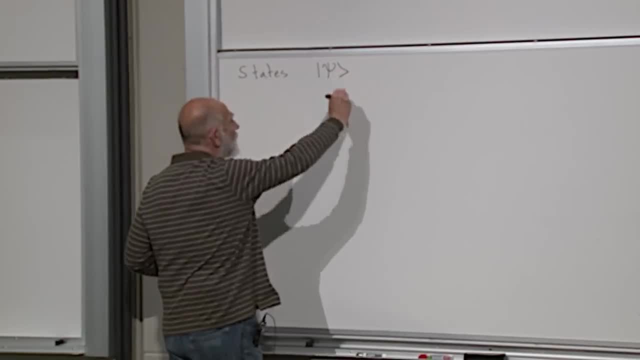 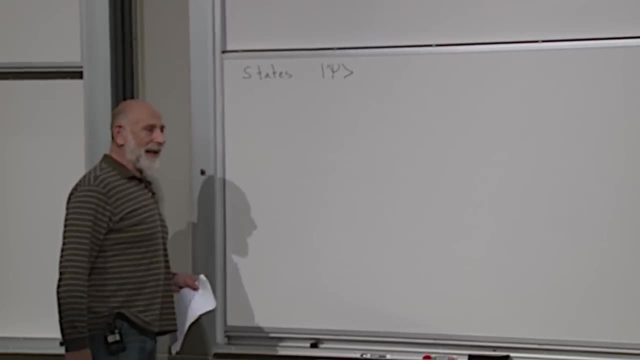 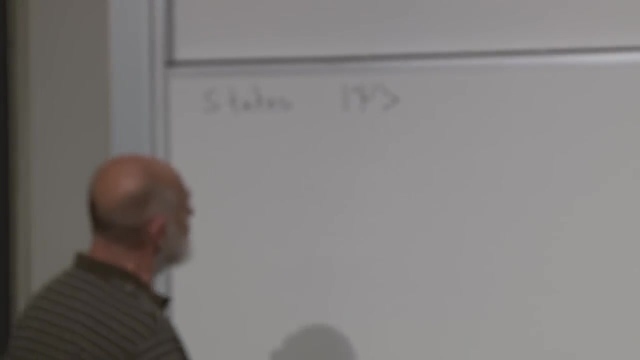 a state vector is Dirac's ket symbol, ket K-E-T, which is the latter half of the term braket like bra-ket or bra-ket. Every state can be either represented by a ket vector or by a state vector. 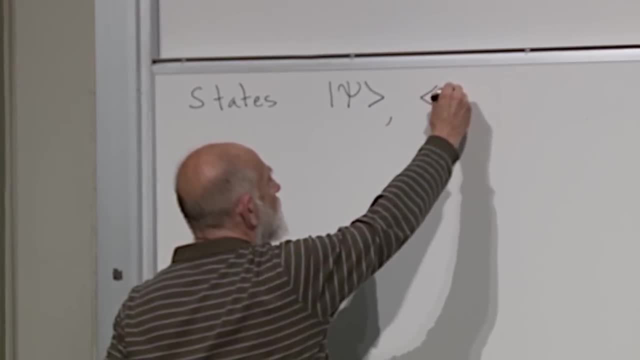 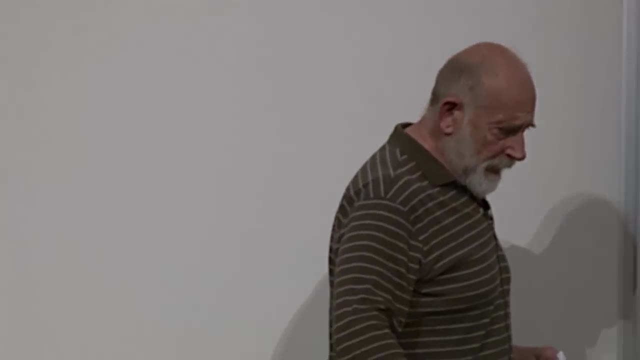 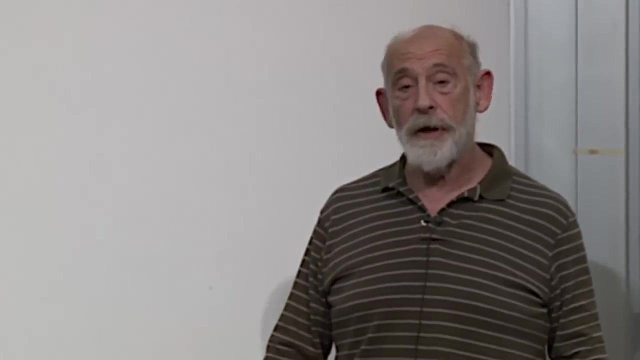 So we represent states by a corresponding bra-vector Together. we often put them together to form a braket or a bracket. The bra-vectors are in one-to-one correspondence with the ket vectors and you should really think of them roughly as being the complex conjugates in the same sense as complex conjugates. 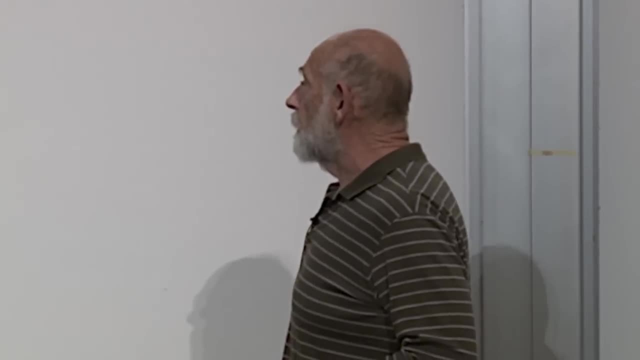 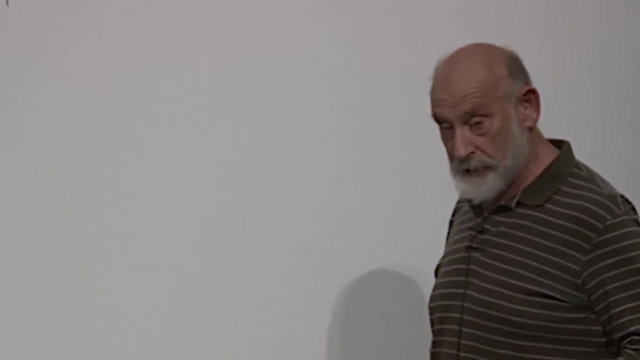 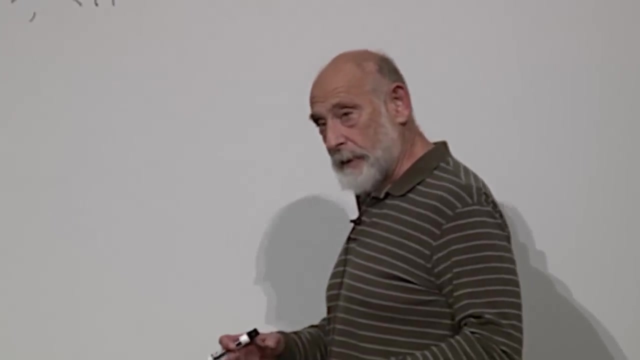 of complex numbers. Complex numbers are ubiquitous in quantum mechanics And so are complex vectors. So state vectors are represented by states. States are represented by state vectors, The state vectors. well, we could say a little bit more, but if I were to say the whole thing, 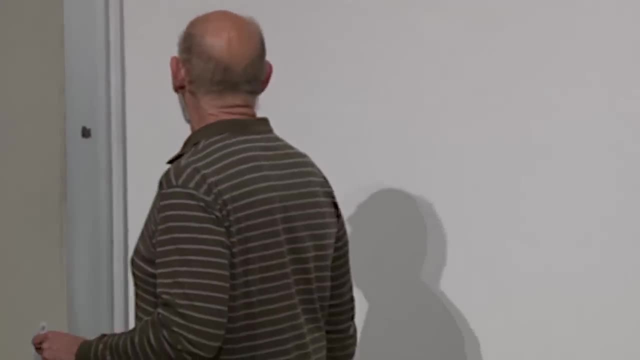 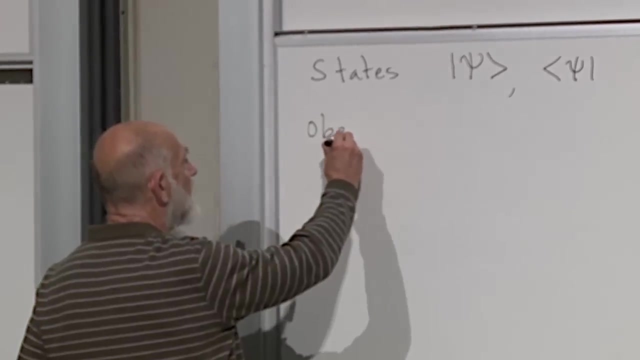 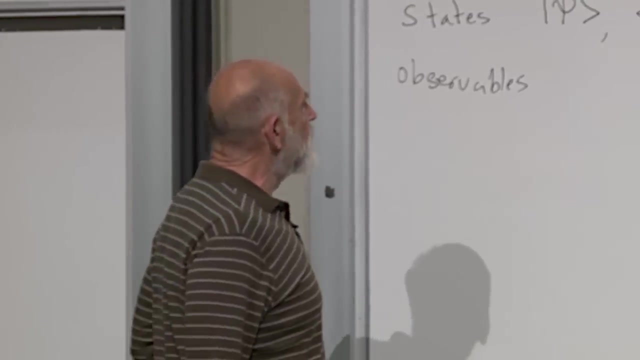 of course, we would then go through the entire quarter, so I won't. In addition, there are observables, things that you measure, Measurables are observables. In classical mechanics there are also observables. These are the things you measure, but we don't spend a lot of time talking about their 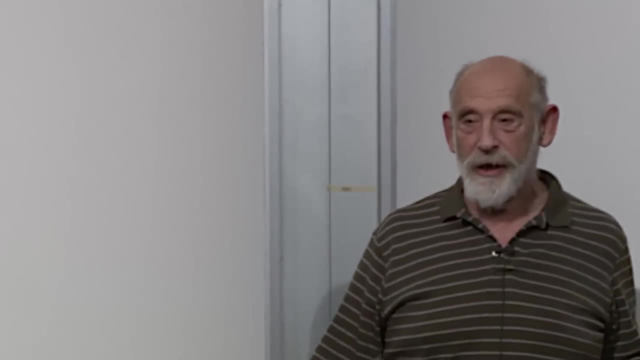 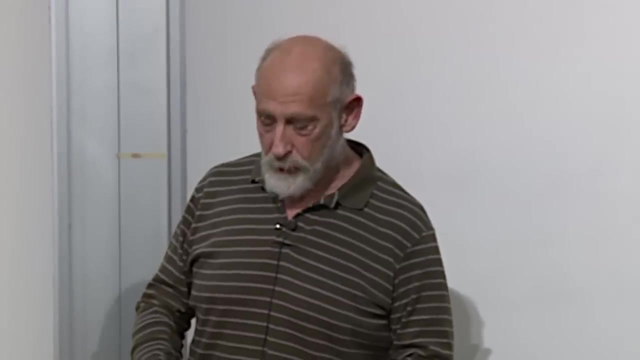 mathematical structure. We just assume you know what I'm talking about when I say position of a particle is measurable, or momentum of a particle, or the energy of a particle or whatever. In quantum mechanics we have to be very precise what we mean by an observable. 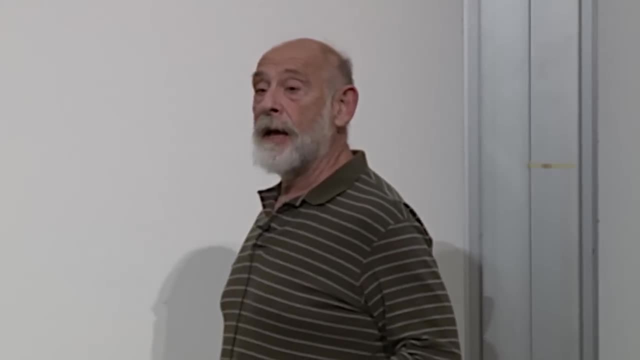 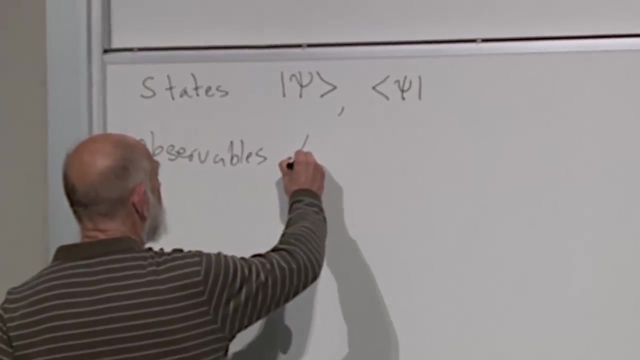 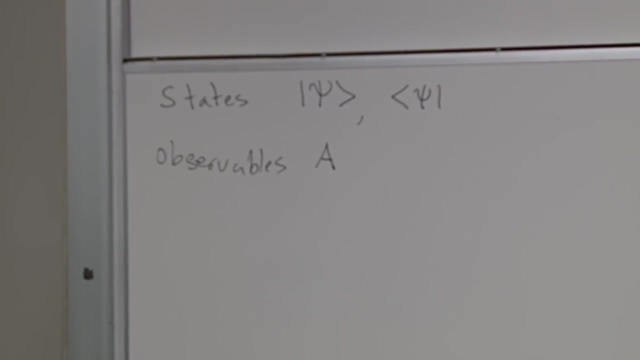 And observables are represented by linear Hermitian operators. I'll label them With. what are these? Let's see, These are Greek letters. What kind of letters are those? English, Roman, Latin? I don't know, All right. 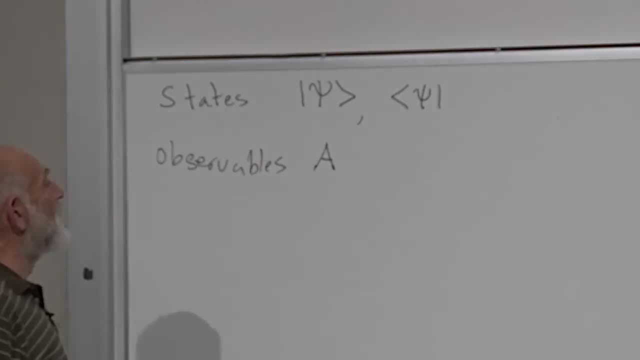 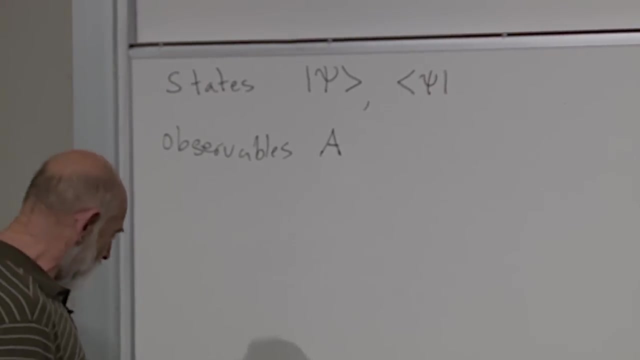 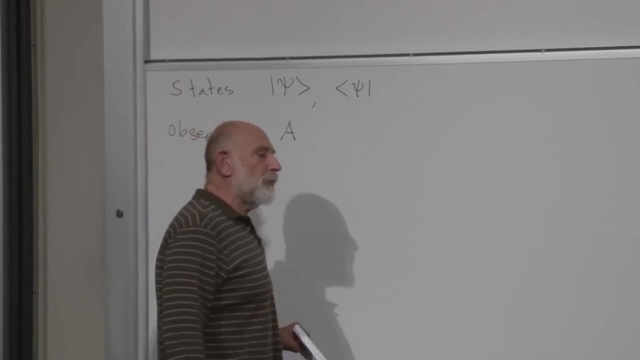 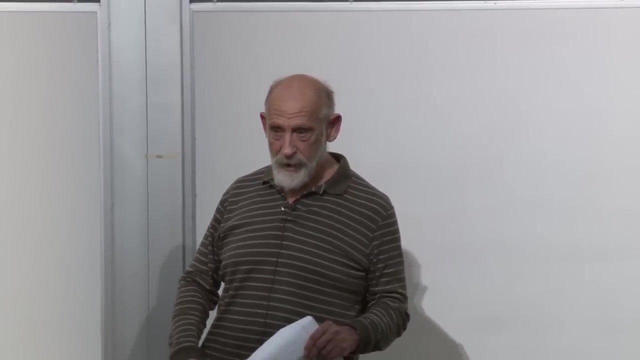 By Latin. Hmm, Yeah, It's true, It's capital alpha, Okay, But Latin letters are representing observables and they are Hermitian operators that act on the vectors. Hermitian for our purposes. It translates: or is the quantum mechanical equivalent of real. 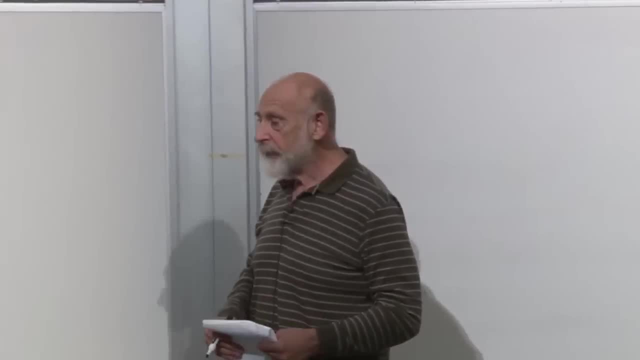 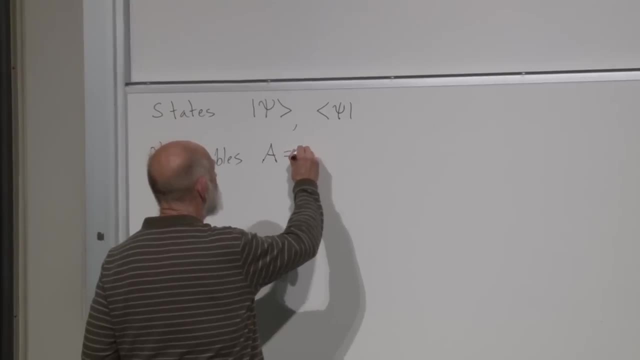 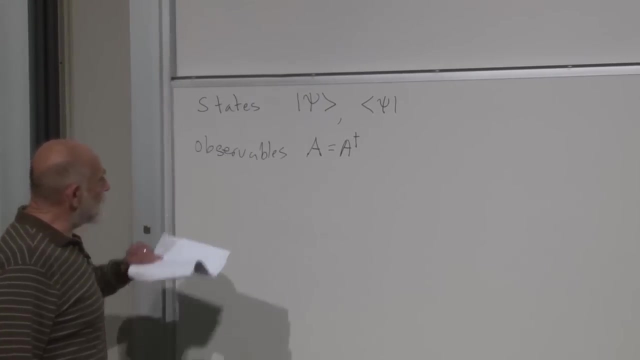 Real as in real or complex or imaginary. They are the real operators which are equal to their own Hermitian conjugate. Every such operator in the space of states is called an observable, and presumably there is really a way to observe it. 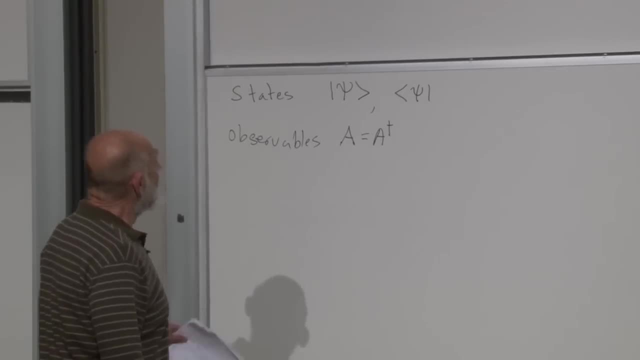 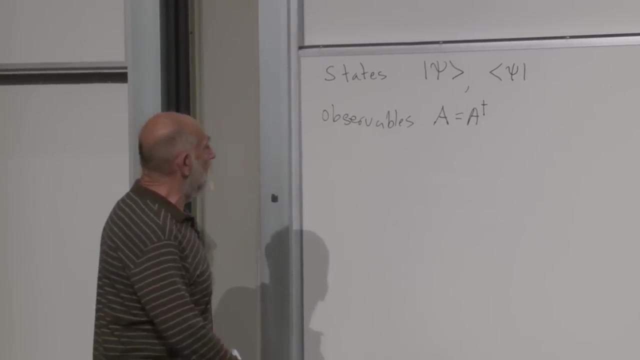 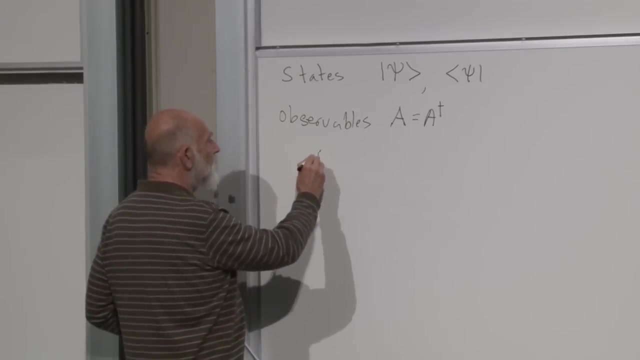 Okay, The eigenvalues and eigenvectors of these Hermitian operators play a special role. So let me just remind you What is an eigenvalue and an eigenvector. If you have a Hermitian operator, you can search for vectors. 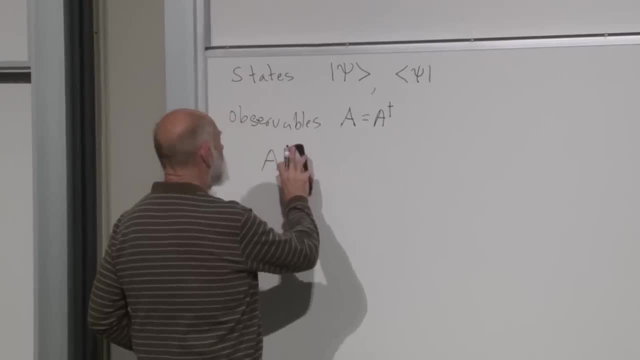 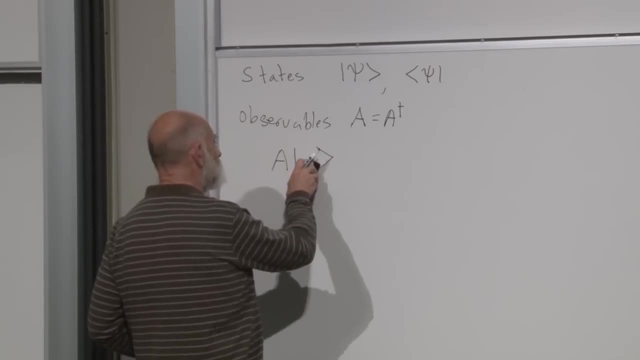 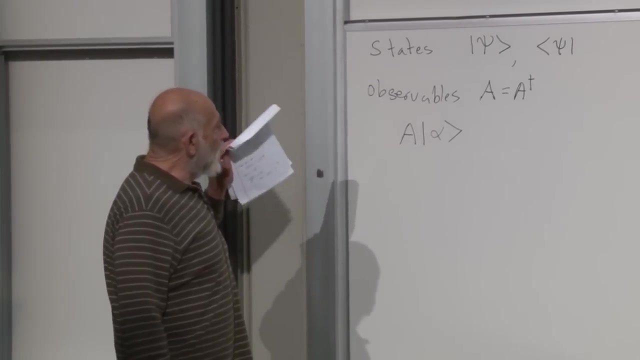 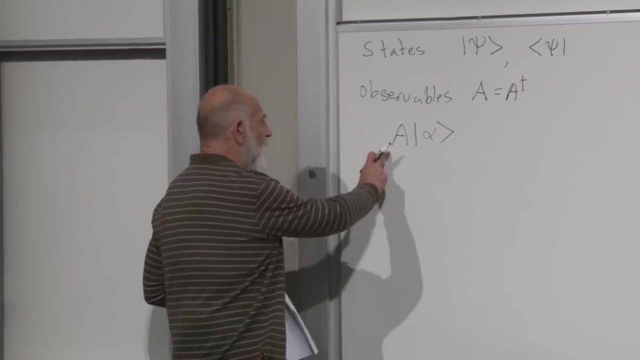 Let's label the vector. Let's label it little, a Okay, Or, better yet, alpha. since we want to label it with a Greek index, Let's label it with an alpha, And a being an operator can act on alpha, and alpha is an eigenvector of a if the action. 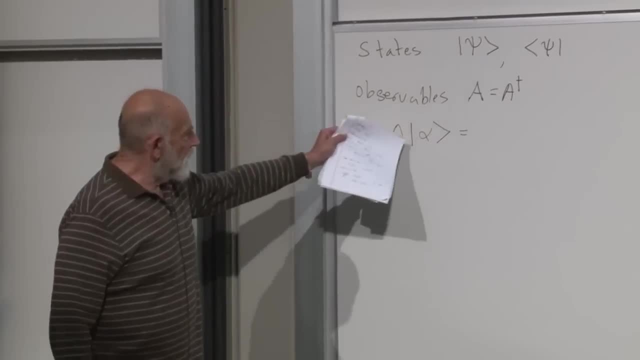 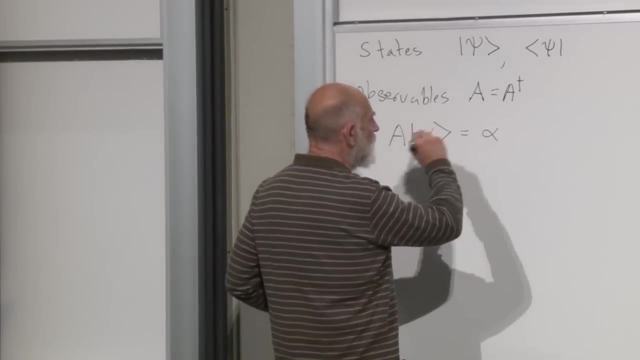 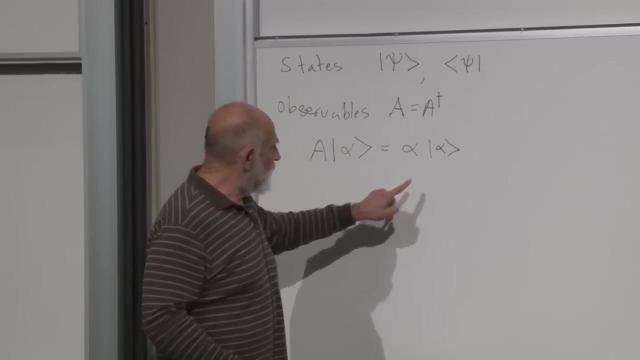 of a is just to multiply the vector alpha by a number. In this case, I'm using a redundant notation. The same notation, The same notation for the eigenvalue and the eigenvector, And this says that the eigenvalue, the eigenvector alpha, is an eigenvector of a with eigenvalue. 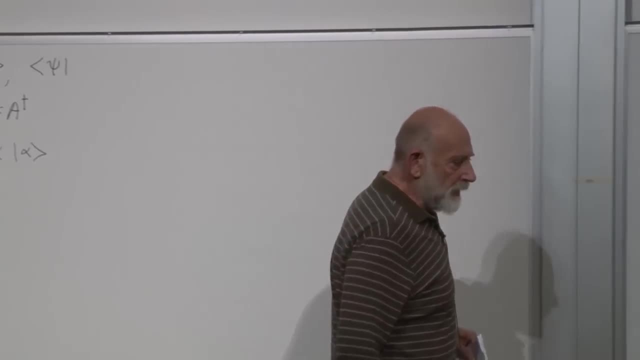 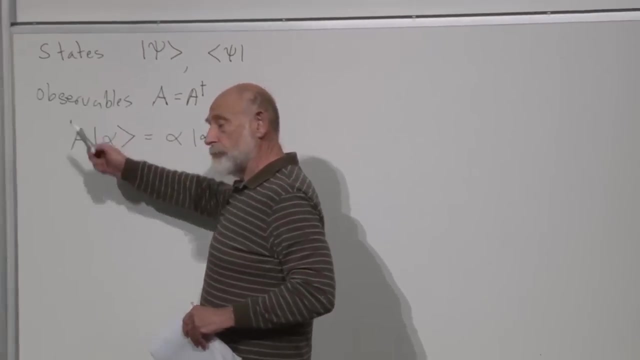 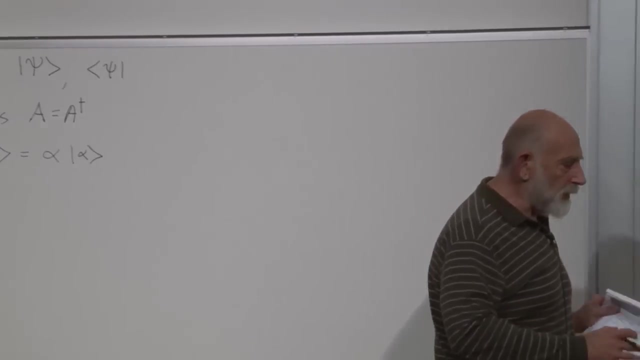 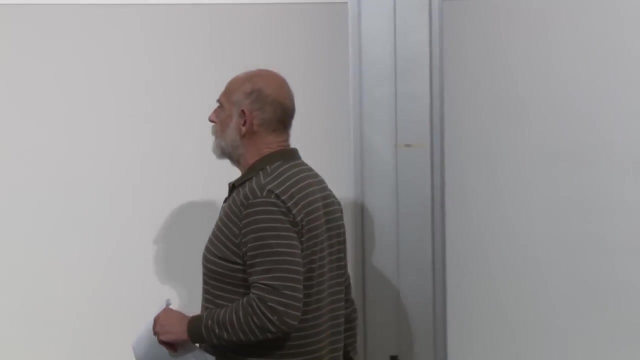 alpha, And the significance of that equation is that, first of all, the set of eigenvalues of an operator or of an observable are the set of possible results of measurement. If you have a quantity, Okay, When you measure it can take on the value one, three and seven, then the eigenvalues. 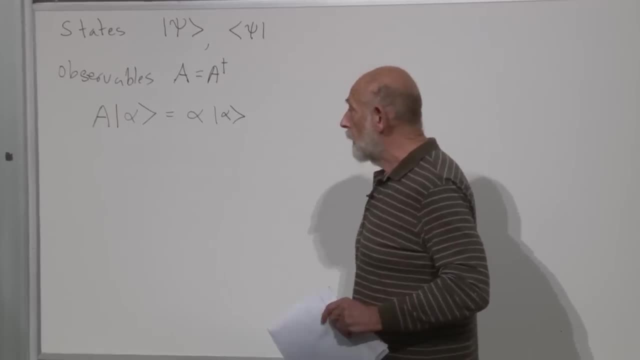 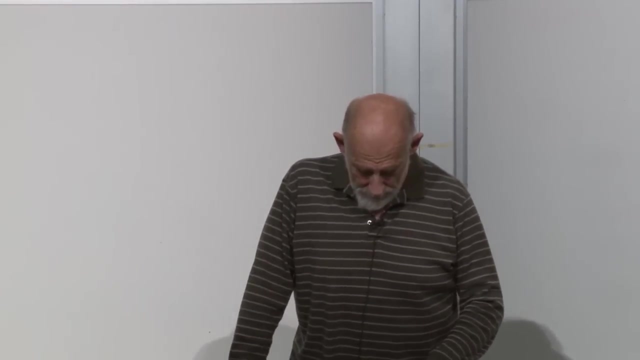 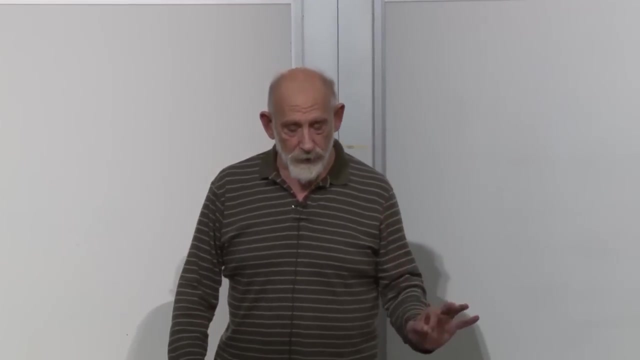 of that operator are one, three and seven and so forth. The eigenvectors are the state vectors of the system for which, if you make a measurement, the answer is definite, not statistical, determined, deterministic, and the answer to the measurement 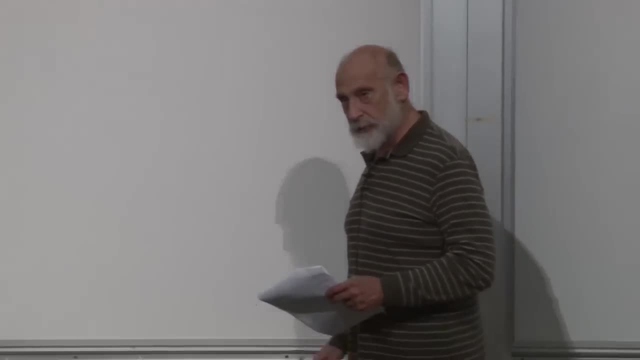 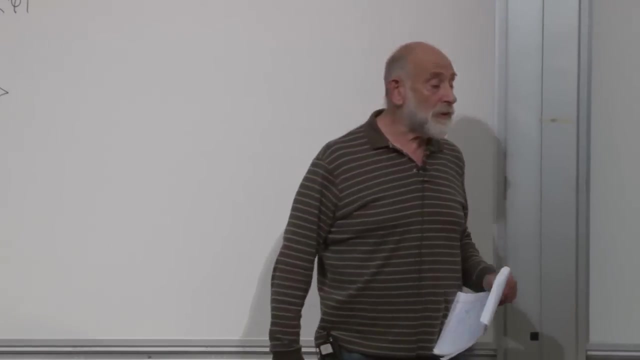 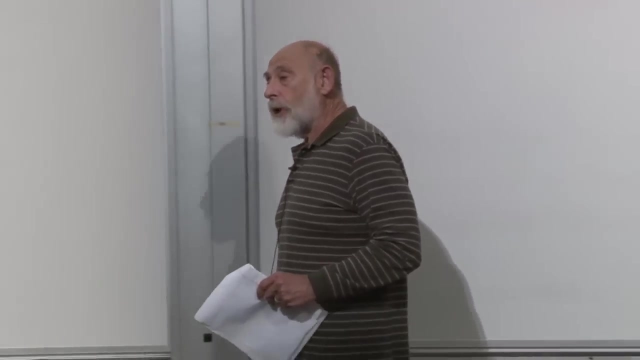 is alpha. Okay, I assume you all remember this. I'm doing this mostly to just refresh your memory. Okay, Now, the particular systems we're going to be discussing mostly in this quarter are systems of particles. Particles are largely characterized by saying they're things which have a location in space. 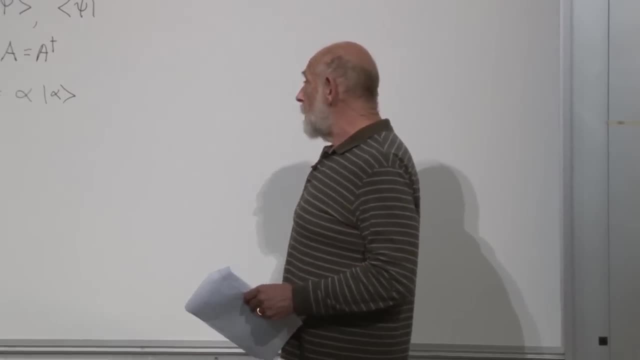 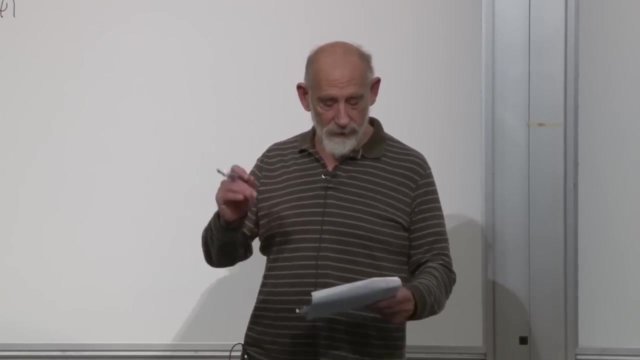 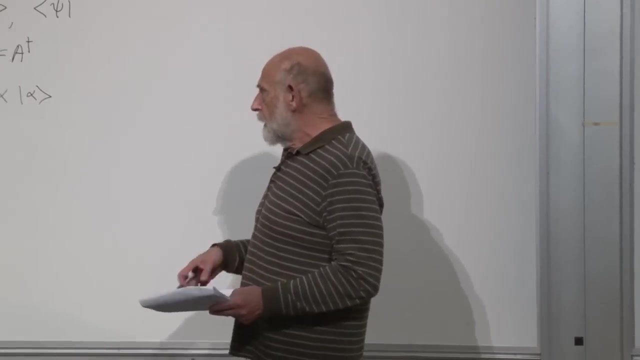 an ordinary location in space. For example, if space is one-dimensional, then a particle is a thing which has a coordinate x, It's located somewhere as an x. If its space is three-dimensional, then particles move around. They have x, y and z and so forth. 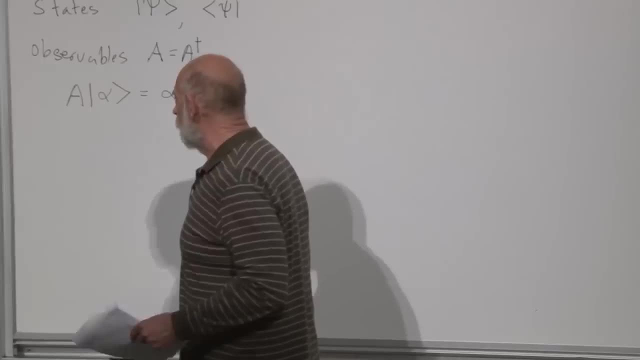 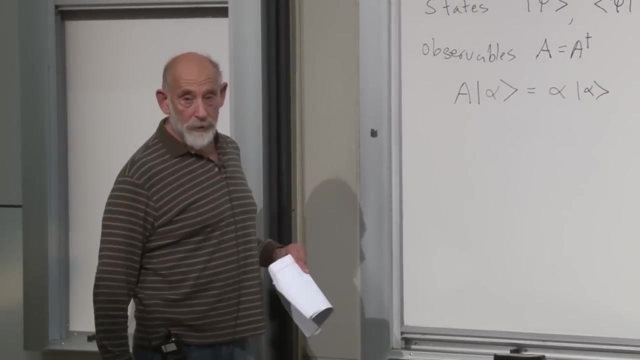 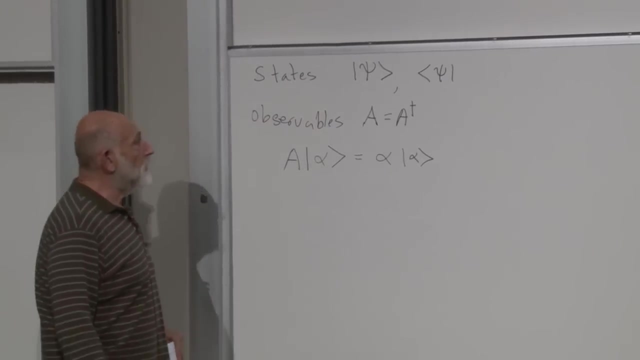 Let's write formulas for the case of one dimension, but I'll tell you what to do for three dimensions in a moment. Okay, Oh, sorry, Let's come back. One point that I need to emphasize for every bra and every ket, let's call the bra, let's. 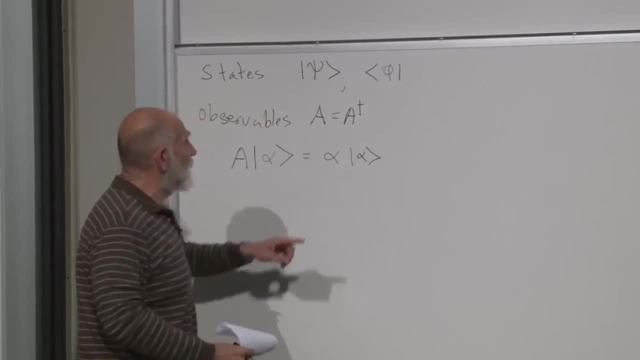 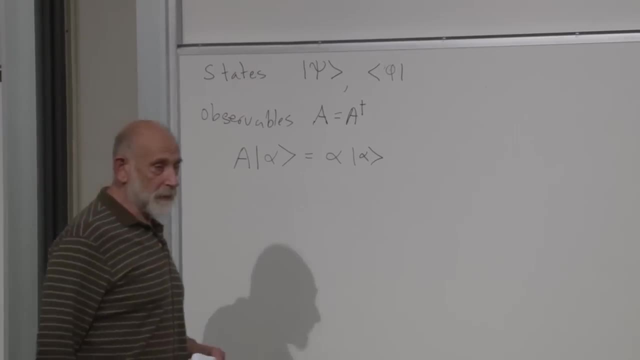 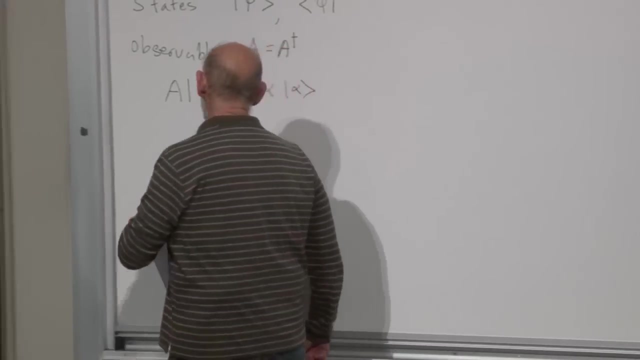 call it phi. it is not necessarily the particular bra that goes together with psi, with the ket psi. For every pair like that, there is an inner product, There is a number. That number is in general a complex number and it is represented as the inner product. 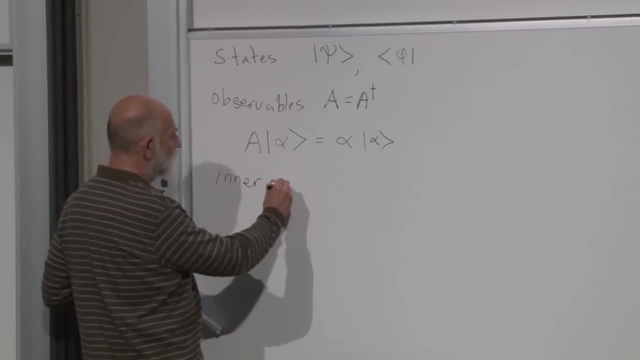 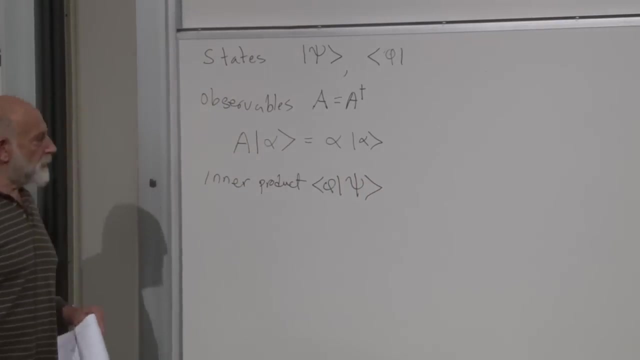 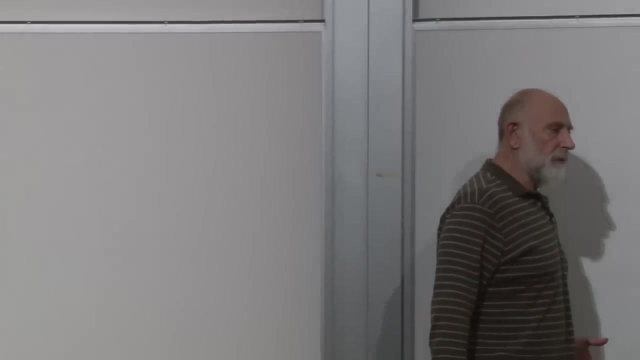 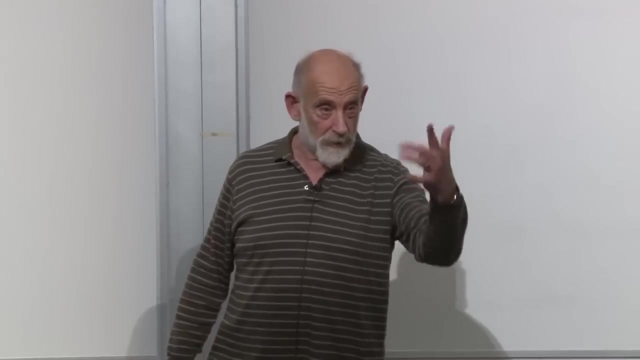 inner product, Okay, Okay, And it's a number. It's a number for every pair of vectors. It represents a kind of product of the two vectors. It's similar in its mathematical structure to the dot product between two vectors in ordinary space, but it's a more abstract object. 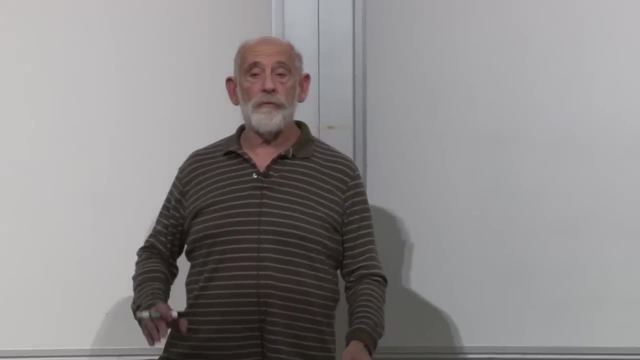 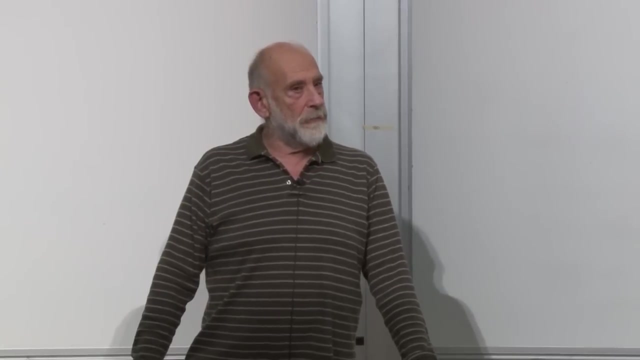 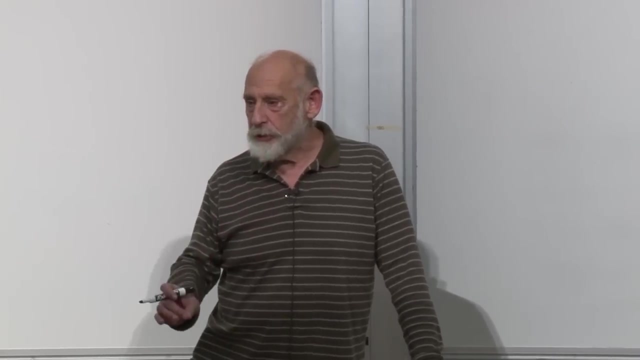 It's the inner product between two vectors and it plays an important role in the logic of quantum mechanics, In particular If two states are distinguishable uniquely by the property that there's some observable that you could measure which would be different than the two of them. let's suppose there's 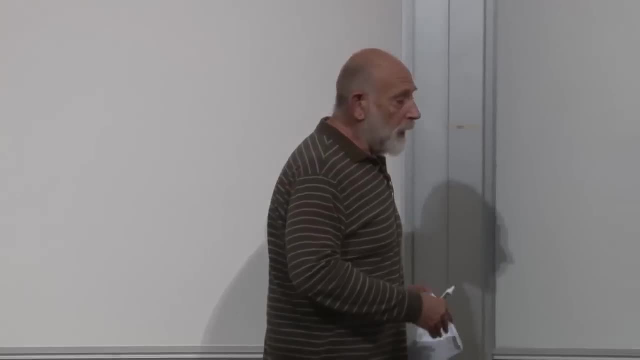 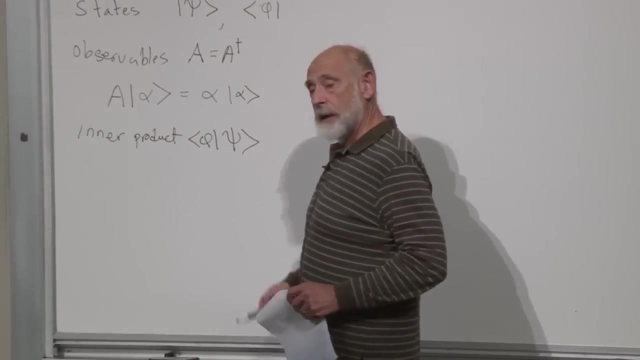 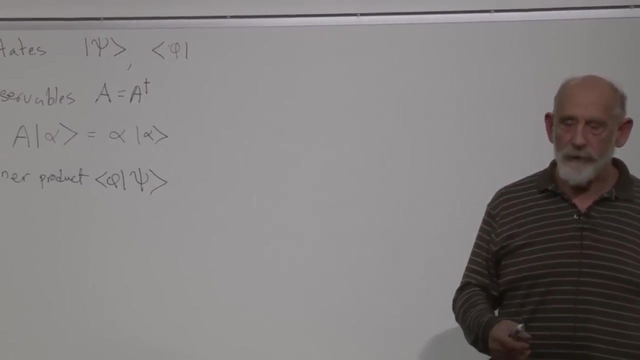 some quantity that you could measure and it is definite that the answer in the state psi is different than the state phi, then we would say those two states are distinctly different. There's no chance of confusing them. There's a measurement you could do to distinguish them. 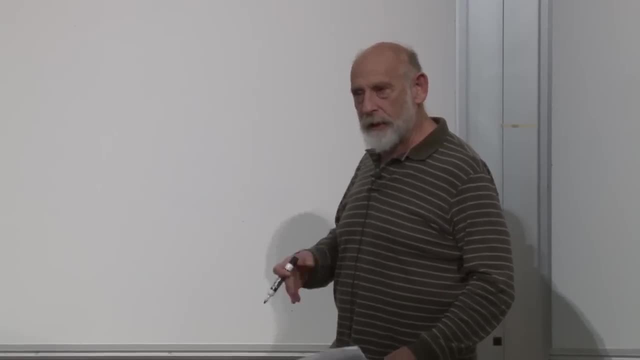 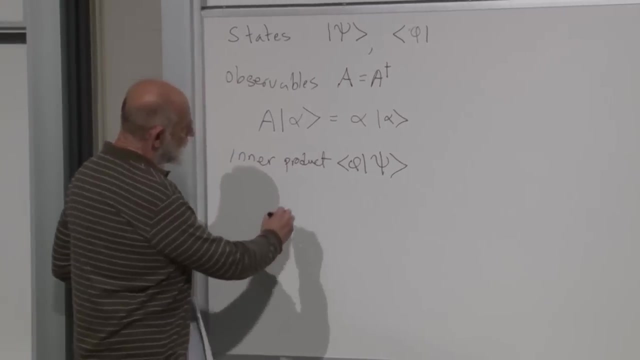 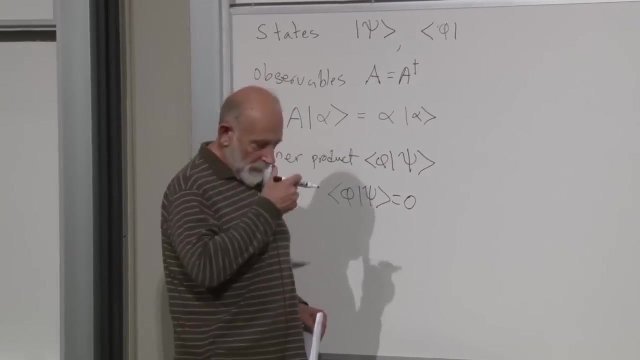 Then those states are said to be orthogonal. Orthogonal means physically identifiably different and mathematically it's the statement that the two vectors have inner product equal to zero. So orthogonality is a fundamental property of relationships. It's a fundamental property of relationships. 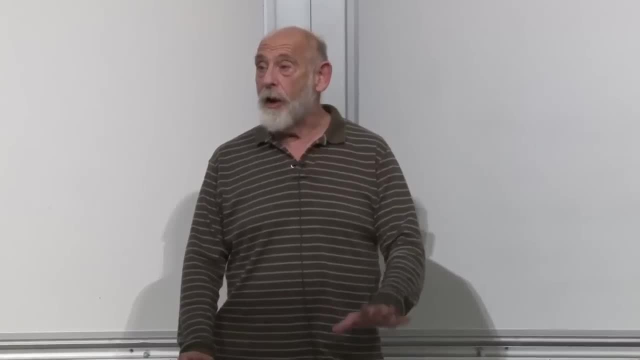 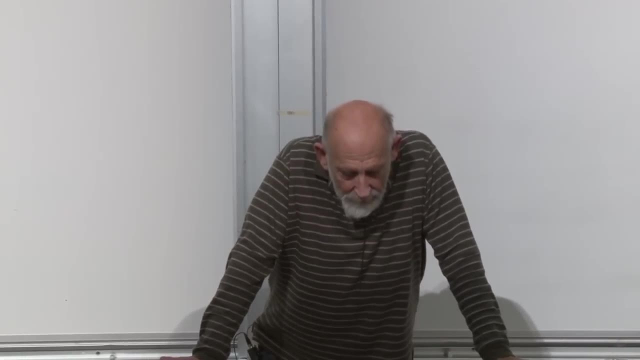 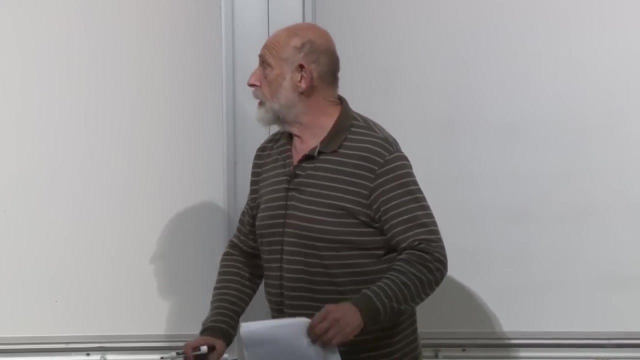 It's a fundamental property of relationships. There are relationships between vectors, which says that they are different. You can't confuse them. Well, you can confuse them, but you shouldn't confuse them. Okay, Now, when it comes to particles, the most important observable is the position of a particle. 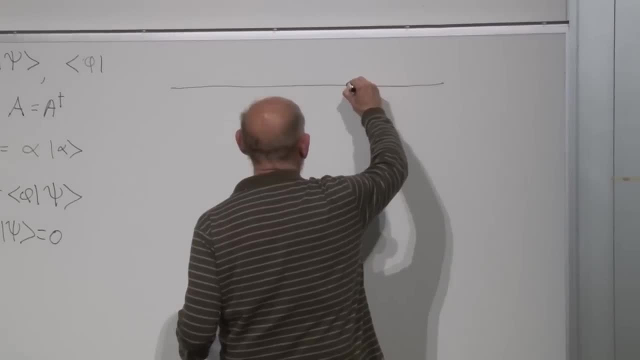 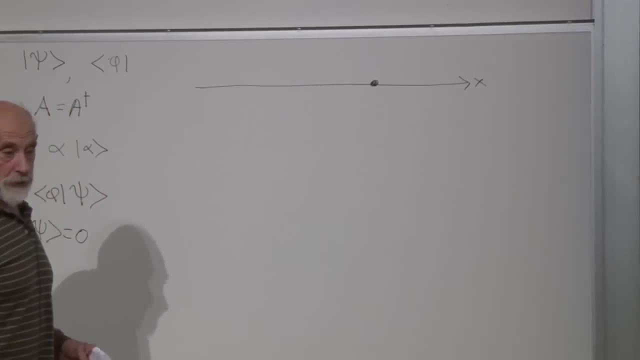 and so let's just discuss particles moving on a line. The line is the x-axis, The location of the particle is just the x-axis, The position of the particle is just the x-axis. The position of the particle is just the value of x, and obviously x should be thought. 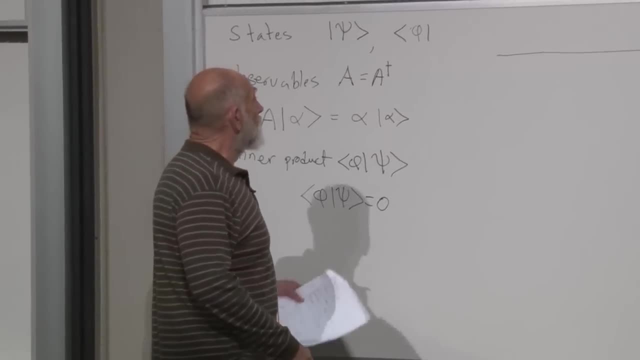 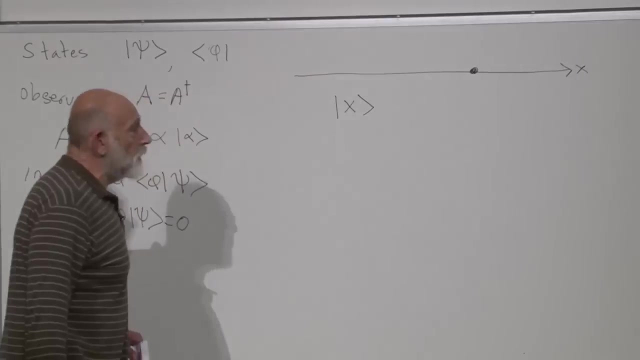 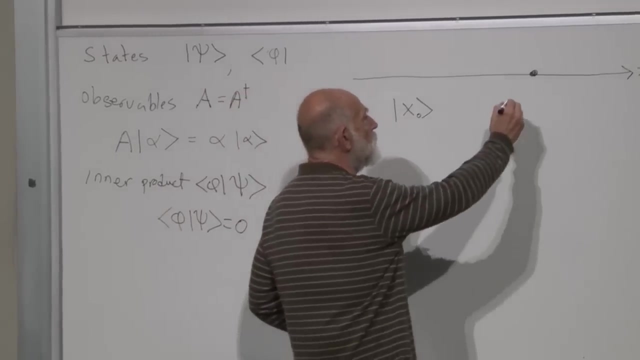 of as an observable. Okay, In particular, there are states which are labeled by a value of position. Let's call it x naught. This is the point x naught over here. I'm just using the naught here to indicate a particular position. 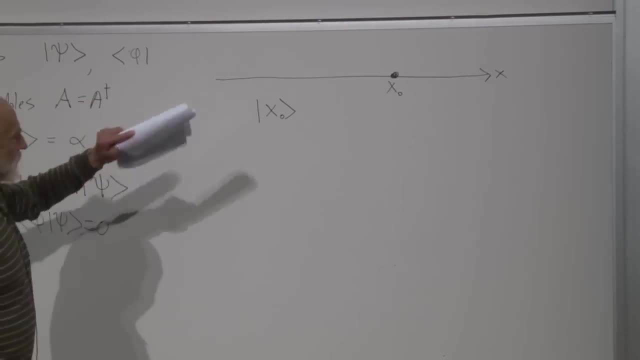 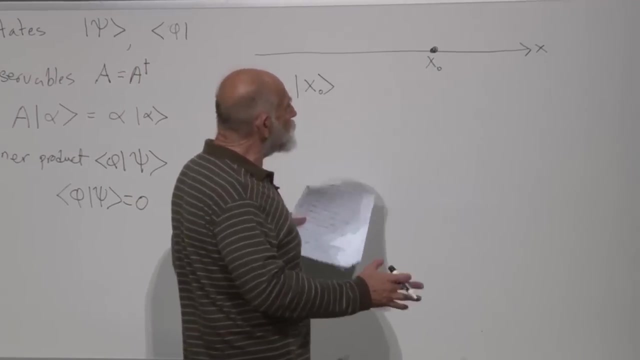 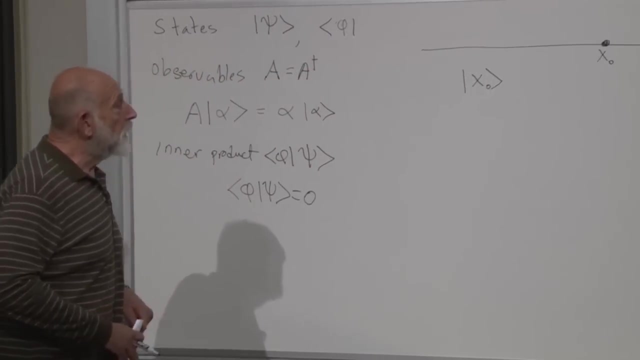 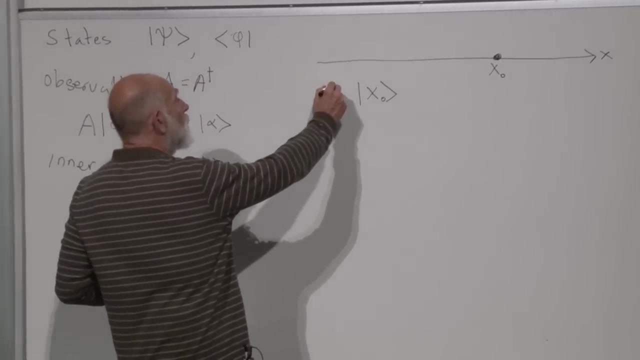 All right, There are states are which are labeled by x naught, which have the property that if you measure the particle, the particle's position, you will definitely find it at x naught. Okay, Good, The next concept. oh, and of course, state vectors for different values. let's call them. 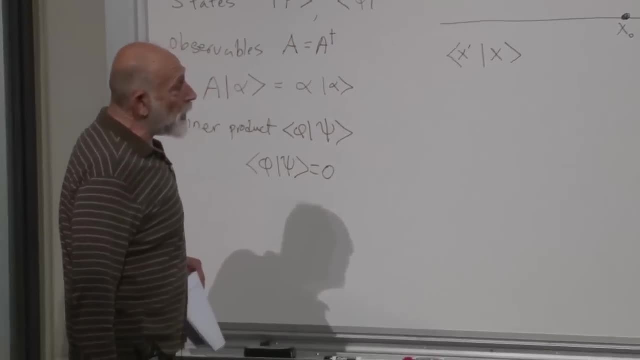 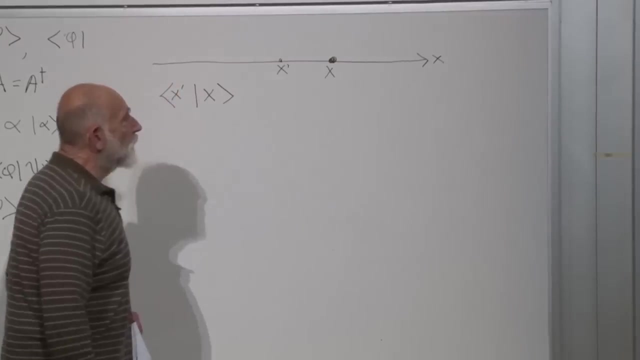 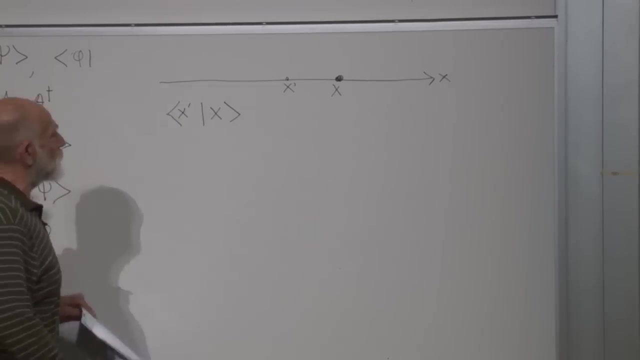 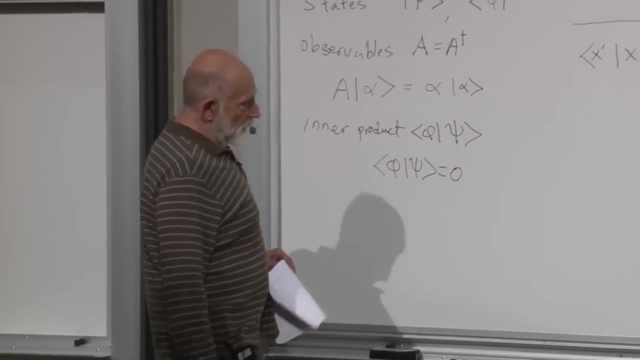 x and x prime. If x and x prime are two different positions, x and x prime, then clearly those two states are distinguishable operationally and by measurement they're distinguishable, so these two states are orthogonal. Now take any state, any state whatever of this particle. 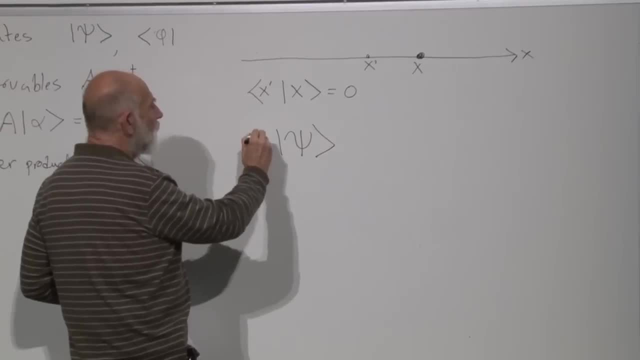 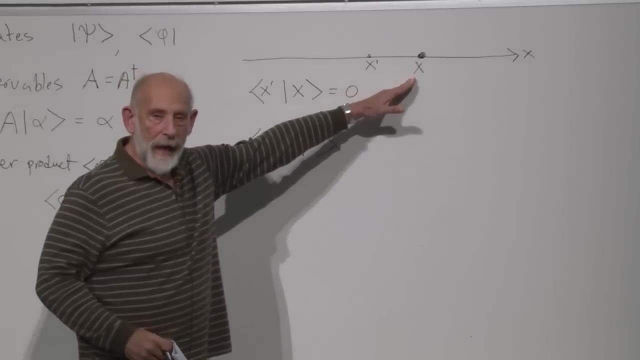 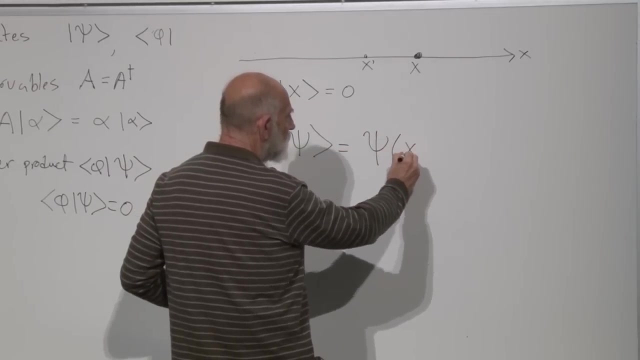 call it psi. Okay, Okay, Okay, Okay Okay. It's in a product with the state representing the particle at x is called the wave function, The wave function of the particle, and it's written as psi of x. It's the psi that goes. 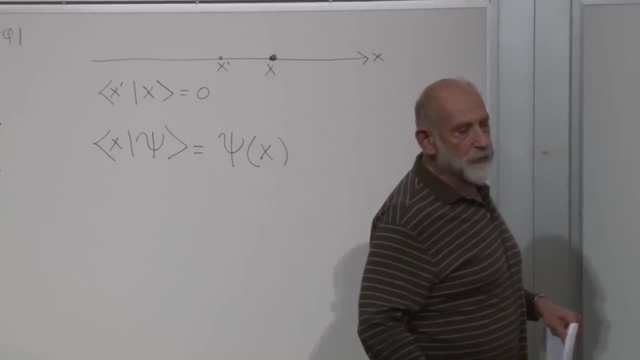 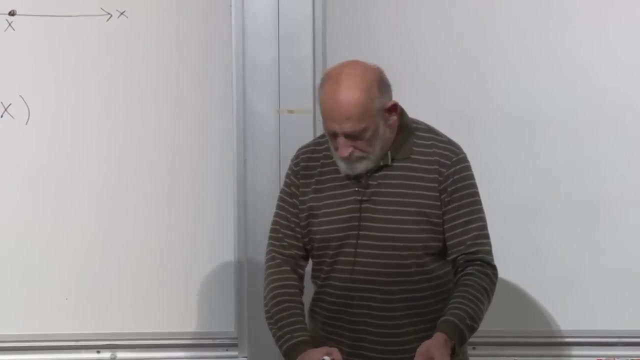 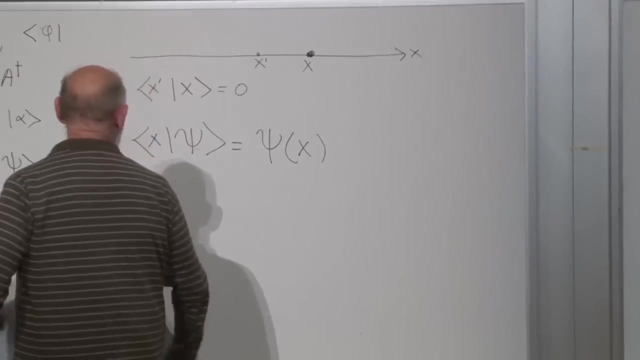 into the Schrodinger equation. It's Schrodinger psi. I believe that Schrodinger was the first one to call it psi. psi And the meaning of the wave function is closely related to, but not the same as, the probability. 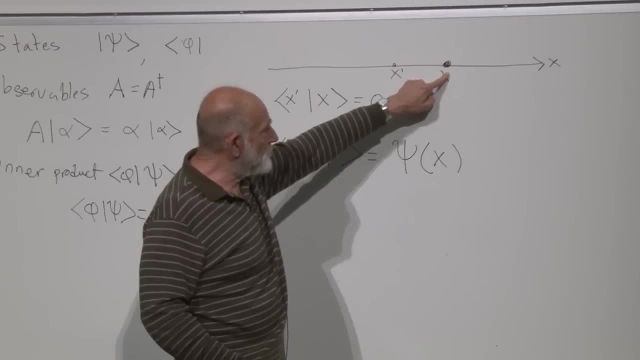 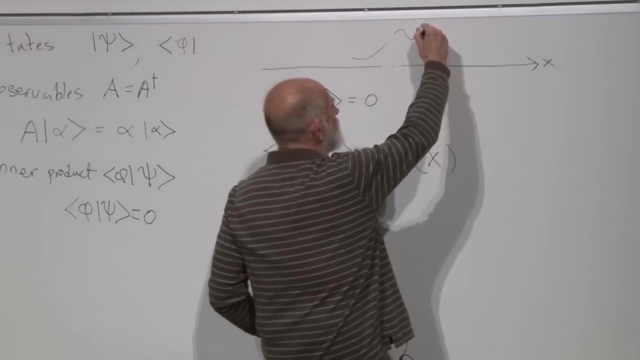 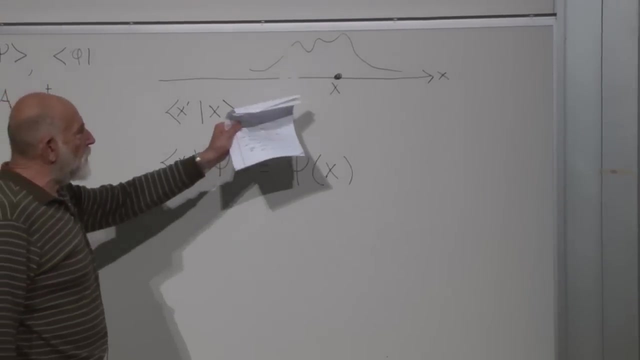 that the particle is at position x. Psi of x is an arbitrary function. Well, it's not completely arbitrary, but let's say it's some function. What does it represent? psi of x. Psi of x is closely related to the probability to find the particle at position x, but it's 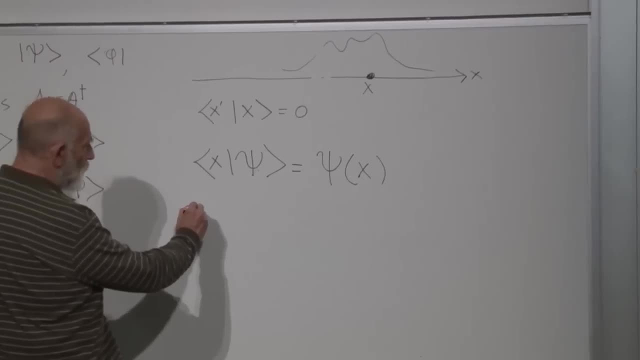 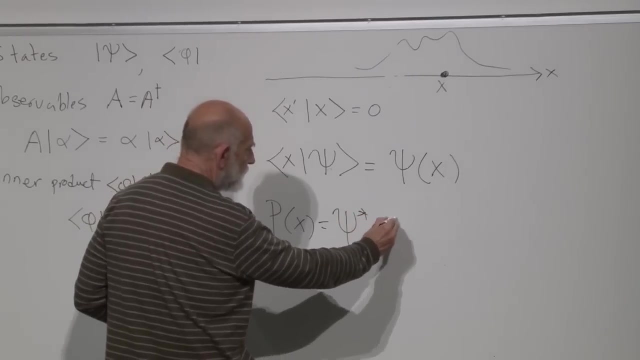 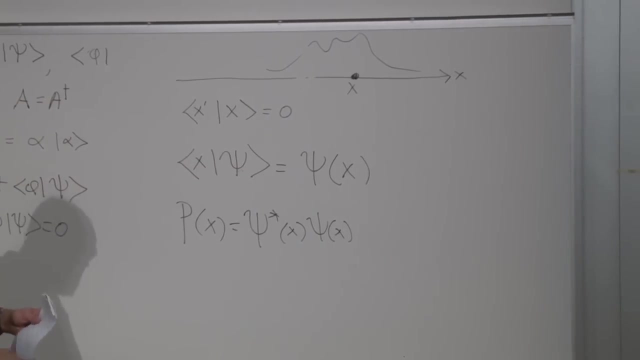 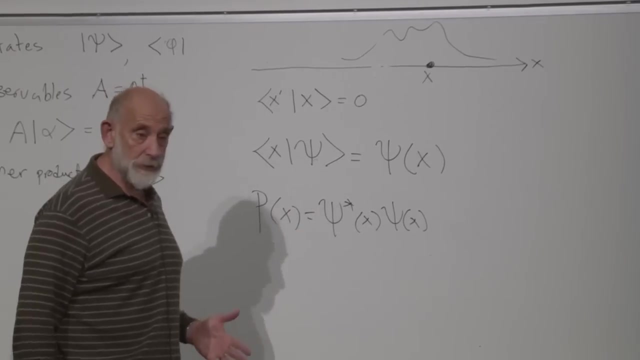 not quite that. The probability itself- let's call it p of x- is the product of the wave function times its complex conjugate. The wave function times its complex conjugate is positive. Any number, any complex number, times its own conjugate is always positive. 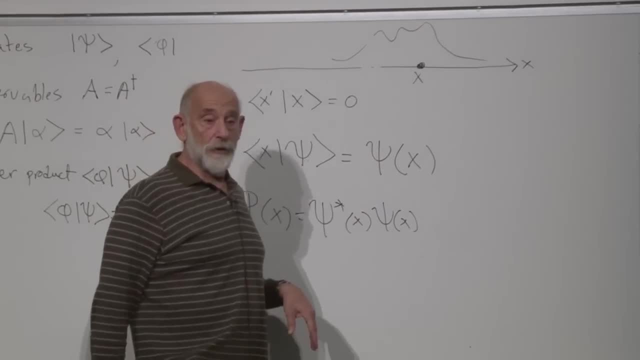 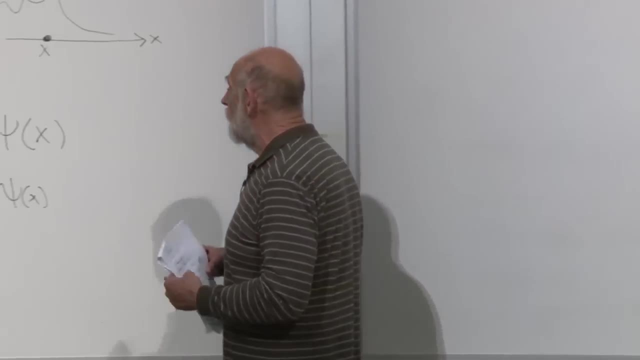 Probabilities are always positive. Psi of x's are generally complex numbers. They can be positive, They can be negative, They can be imaginary, They can be whatever you like. So it would not make sense to say that psi is a probability, but it does make sense to. 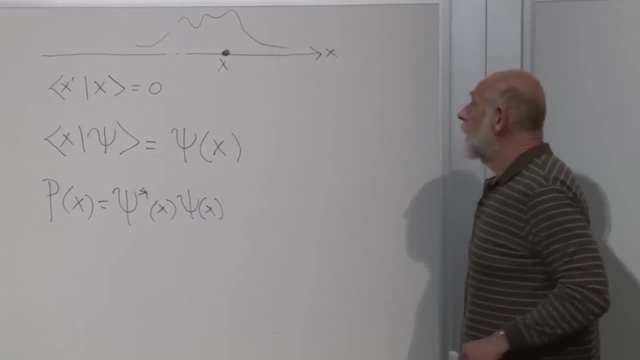 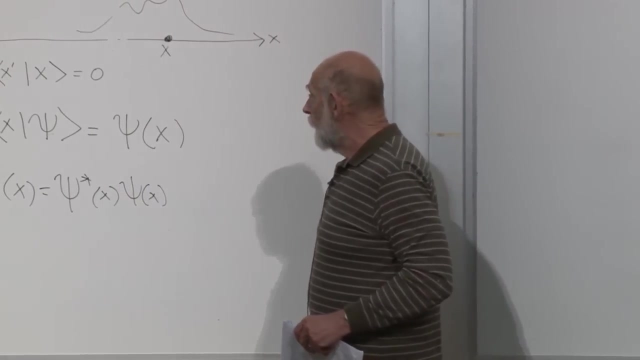 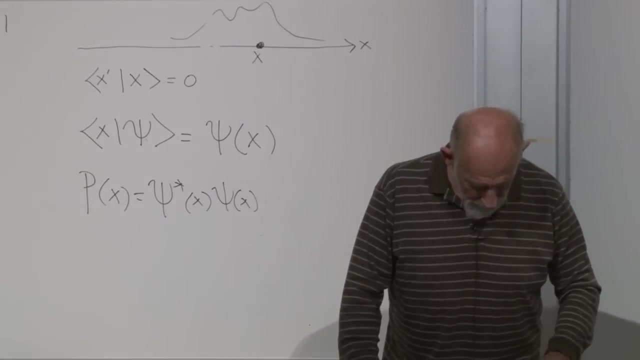 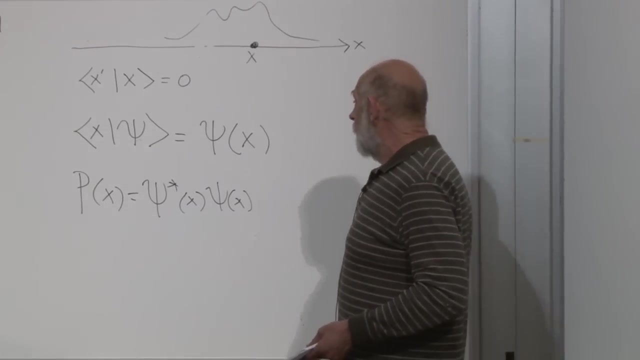 say psi times psi star is a probability. Good, All right, That's the most important, Okay, property of a particle: that it has a position. it has eigenvectors which represent particles of known position and we can construct, of course, a position operator, A position operator. 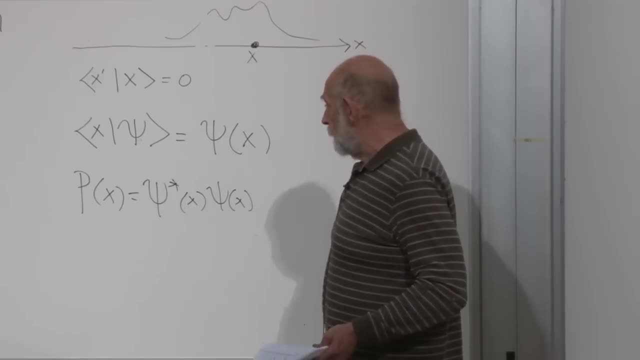 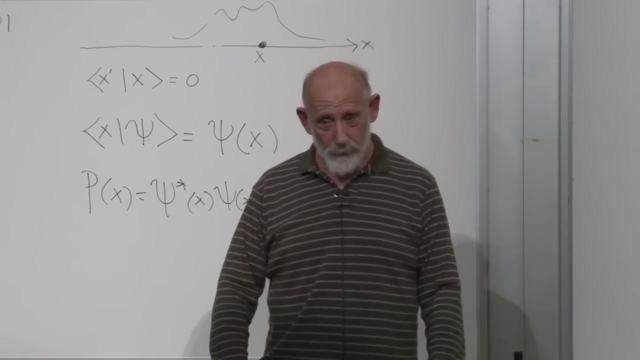 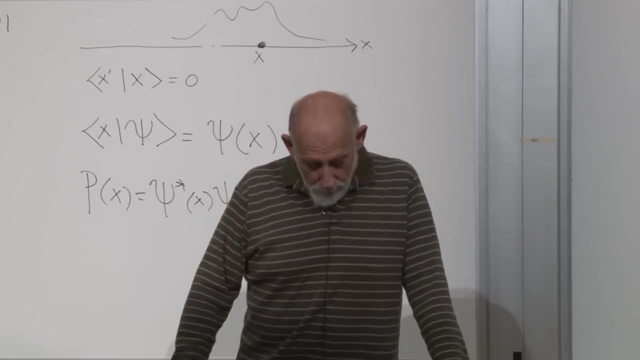 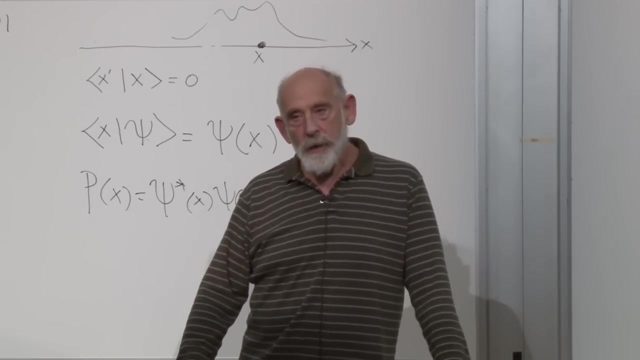 just multiplies psi of x by x, itself by x. So that's the idea of position, The other important observable for a particle. there are many observables for a particle, but the other, particularly important one is called the what, The momentum, The momentum In classical. 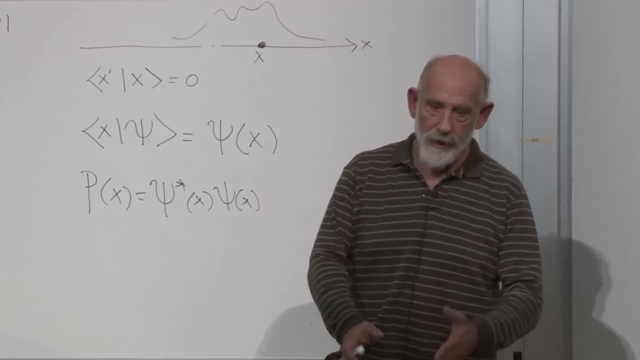 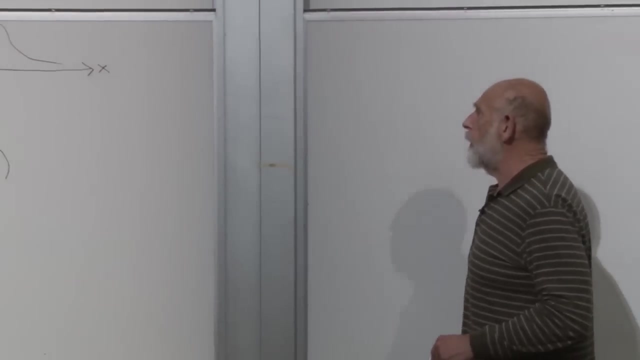 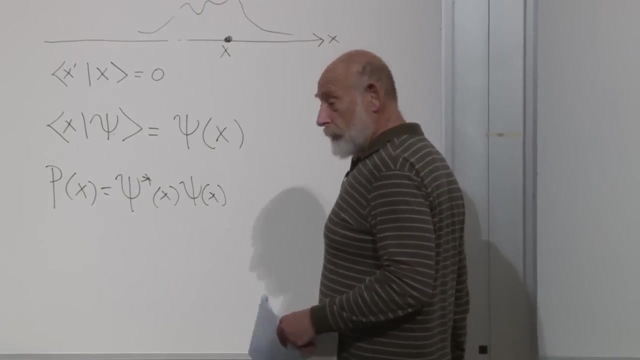 mechanics and in quantum mechanics, positions and momentum come together. Oh, before we do that, I should discuss the issue of a particle moving not just in one dimension but in another. What happens if a particle is moving in three dimensions, In other words like? 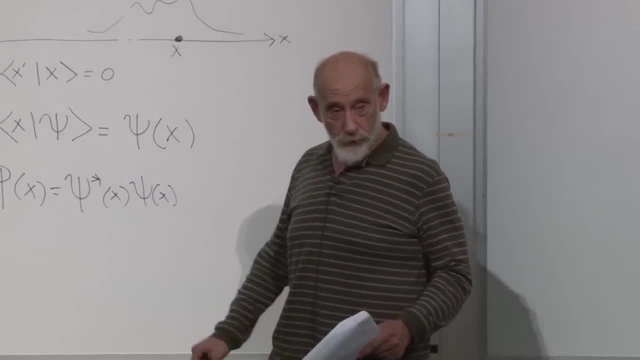 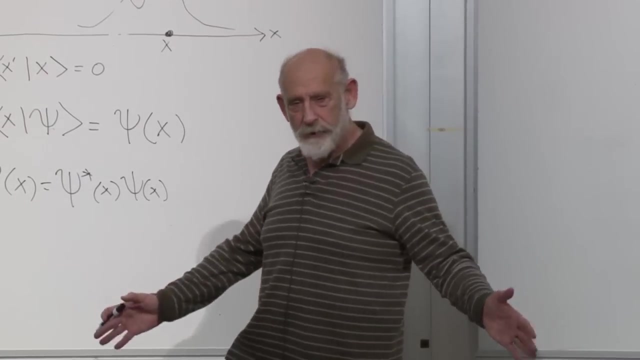 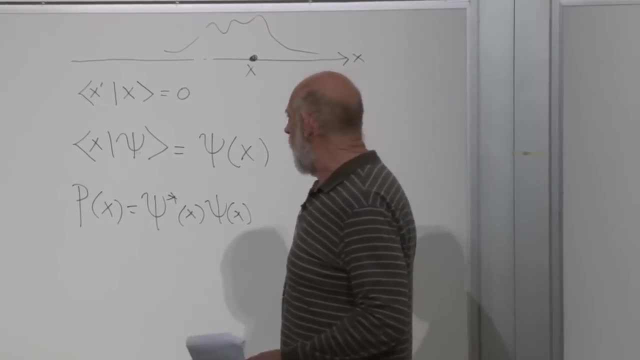 a real particle, Then it has three observable positions, the three components of its position, namely x, y and z, if you like. But since you can rotate axes, you can just think of the position as a point in three-dimensional space. In that case, we would just think of: 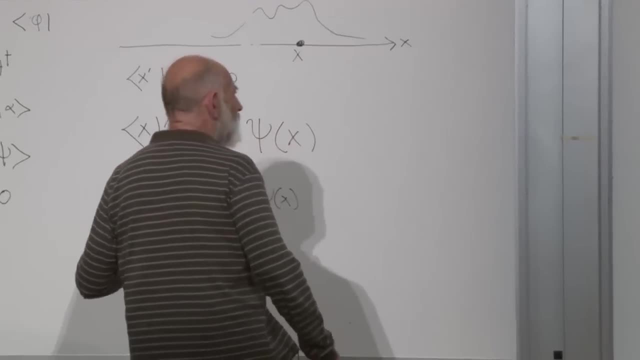 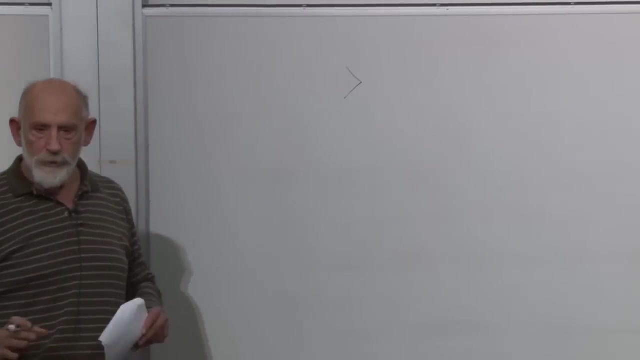 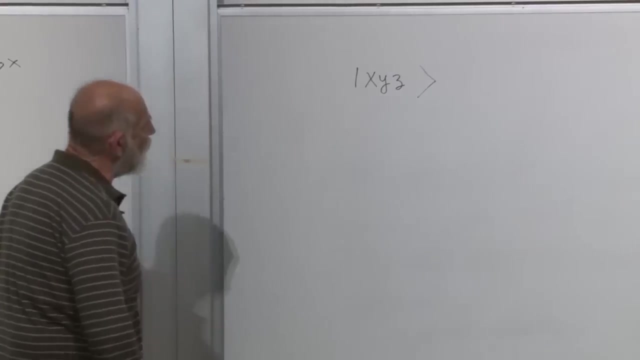 x here as a point in three-dimensional space. We could fill it out. We could fill out the equations by saying: there are states which represent particles at known locations in three dimensions: x, y and z. This represents a particle located at a point in three-dimensional space over. 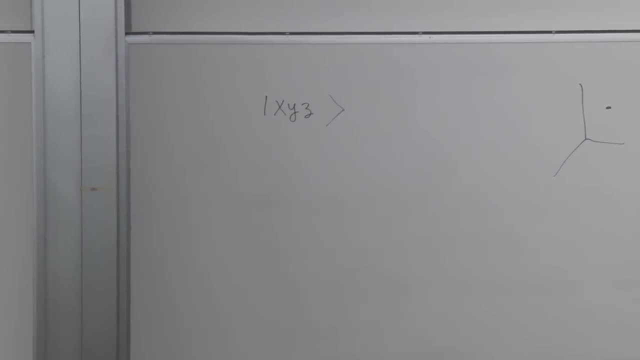 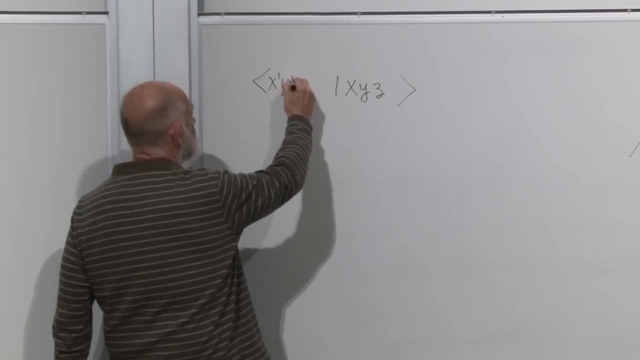 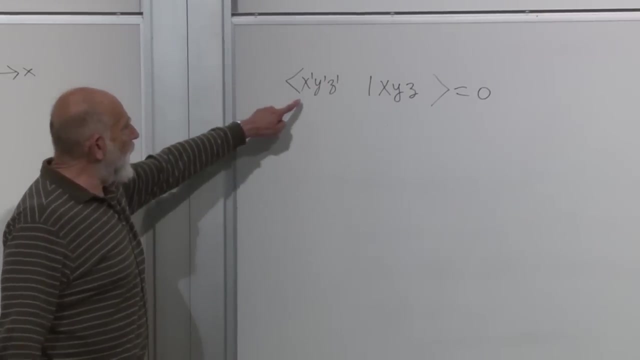 here x, y and z And the rules would be similar, very similar, The inner products of x prime, y prime, z prime. that would be zero if there's any mismatch, not if x is not equal to x prime and y is. 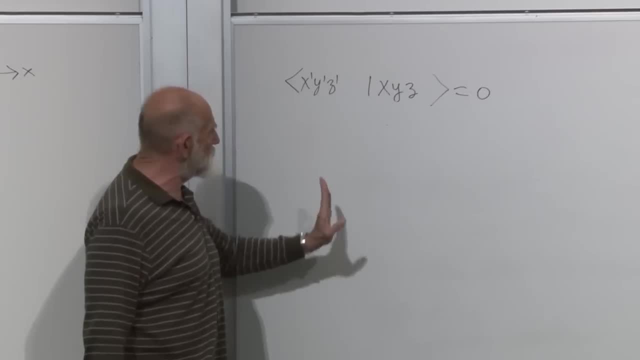 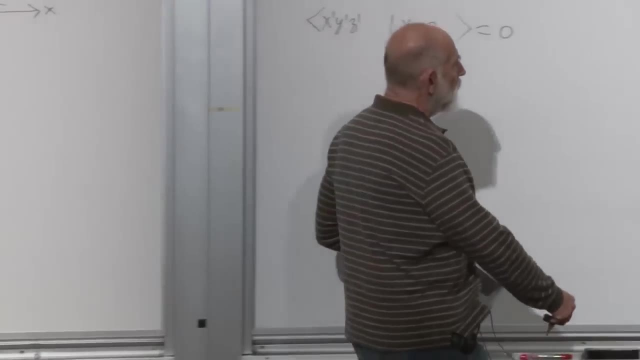 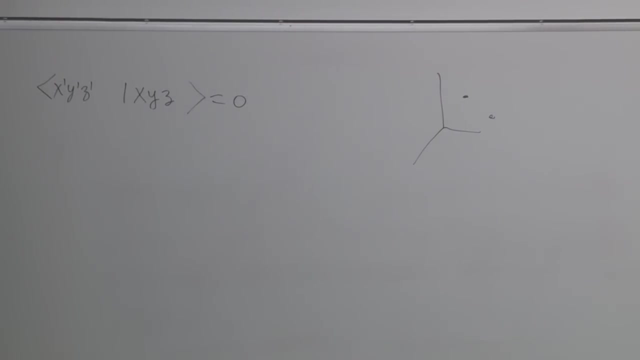 not equal to y. but if the entire point x, y, z is not the same as the point x prime, y prime, z prime, then these are observably different positions for a particle and the states are orthogonal to each other. I'm not I'm going to suppress the y and the z. I'm 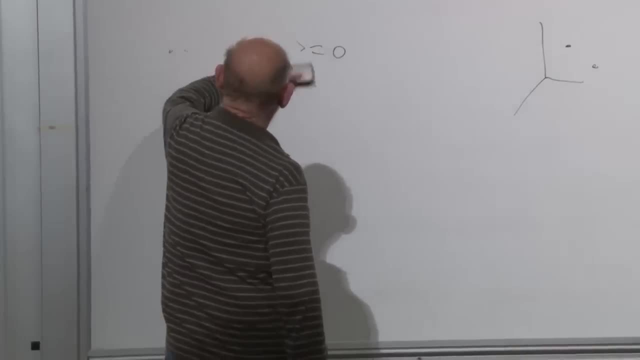 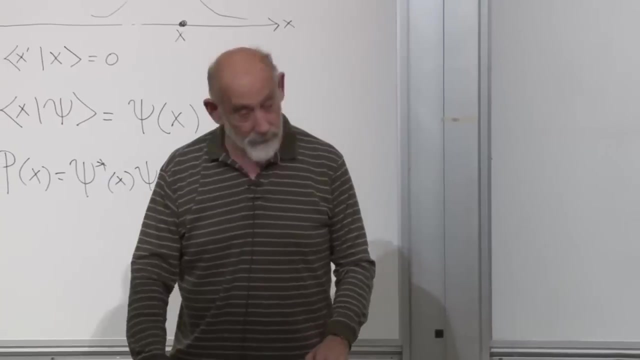 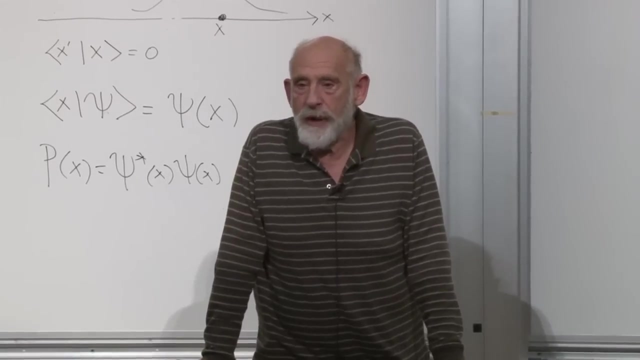 going to get the y and the z, but keep in mind that the position of a particle depends on the dimensionality of the space that we're talking about, And in the real world space is three-dimensional. Okay, for each component of position, there is also a component of momentum In classical. 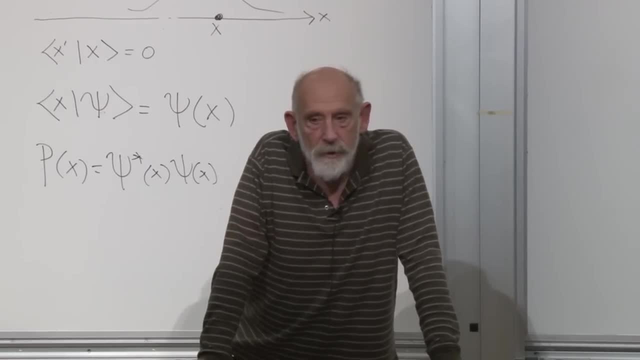 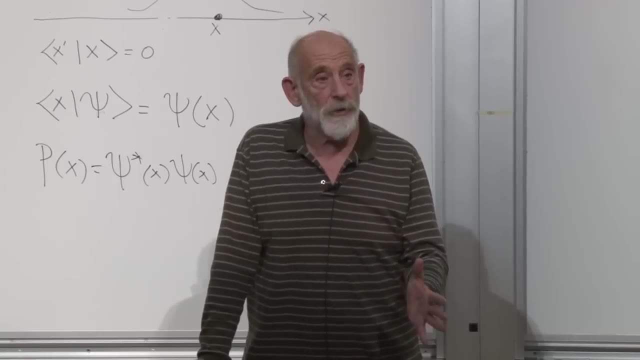 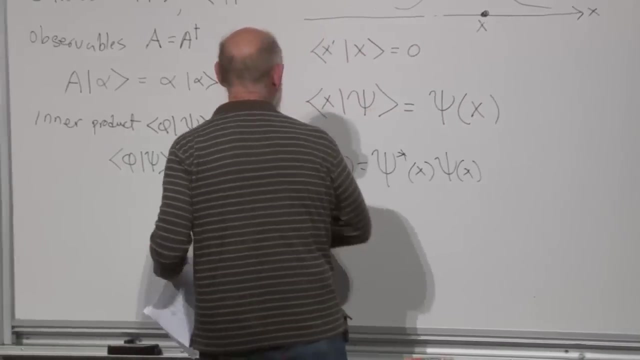 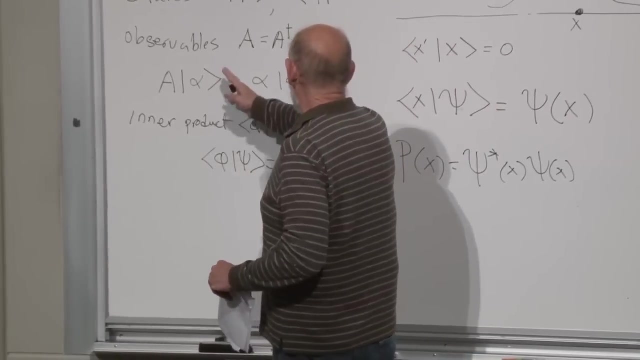 physics, for non-relativistic, classical physics, the momentum is just the mass times, that component of the velocity. Okay, Okay mechanics, the momentum is also observable and is also represented by an operator, by a Hermitian operator. Hermitian operators can be thought of in the abstract as objects which act on mathematical. 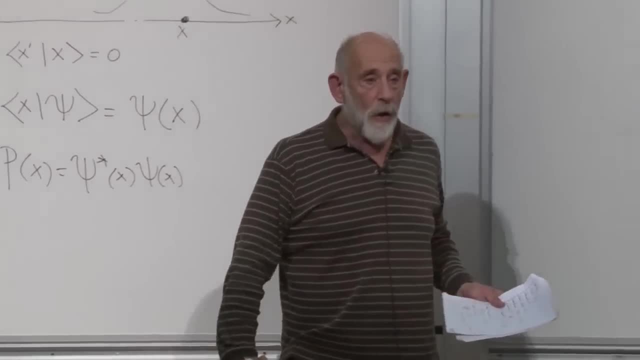 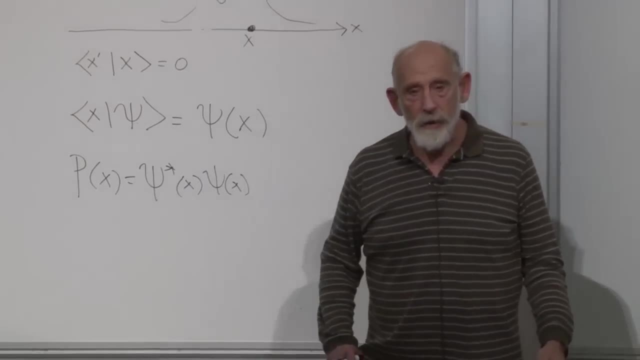 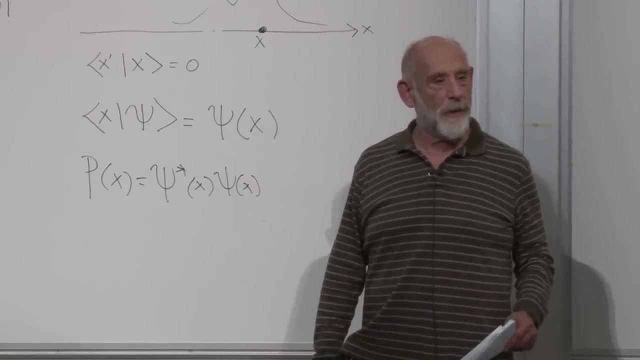 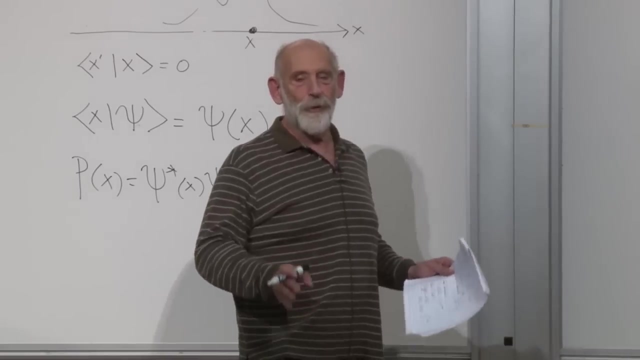 vectors, the space of states, or they can be thought of more concretely as operations on wave functions. Either one, you can think of them concretely as operations that you. what about x itself? What is the operation that represents the operator x? 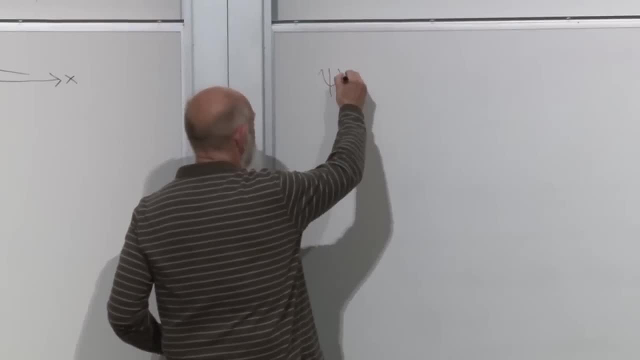 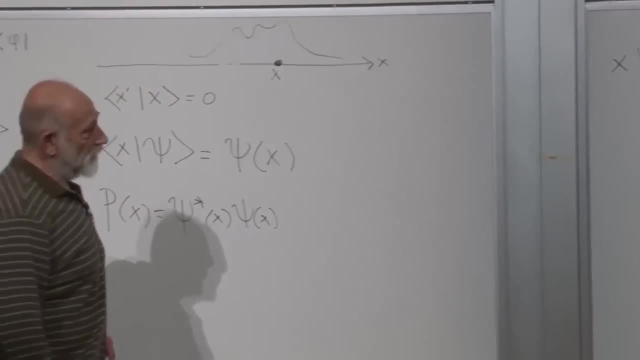 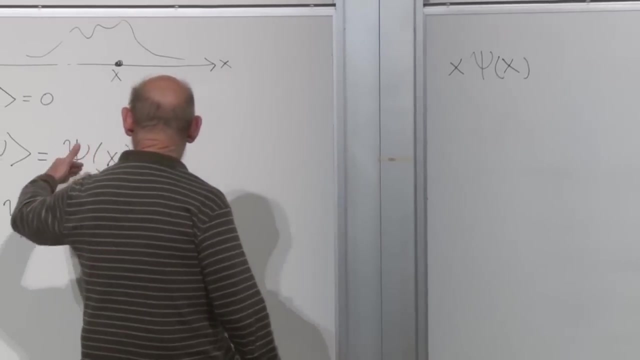 Well, it's just taking the state vector psi of x, or taking the wave function and multiplying it by x. If psi of x is a function Representing the probability amplitude, Psi of x is called the probability amplitude of the wave function of a particle. 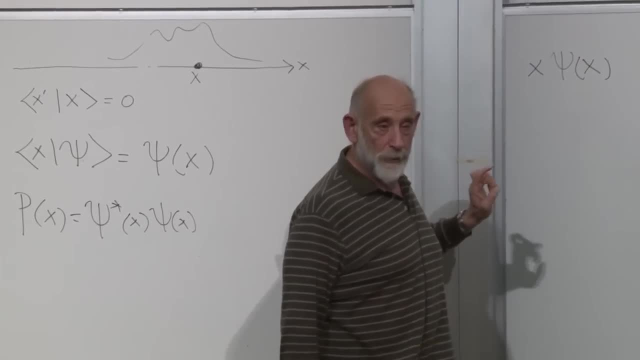 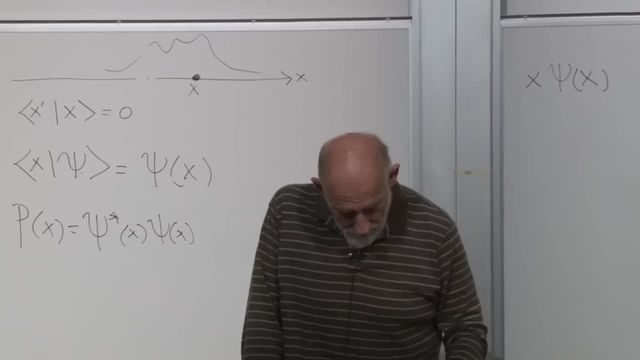 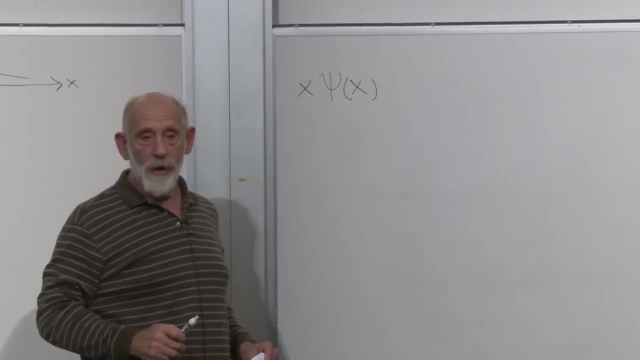 Then if you want to apply the operator representing position to psi of x, you just multiply psi of x by x. That's all. The eigenvectors of x are the wave functions, which are highly peaked, very, very narrow Dirac delta functions. 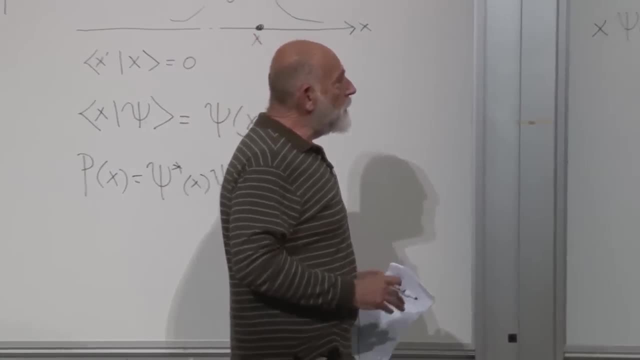 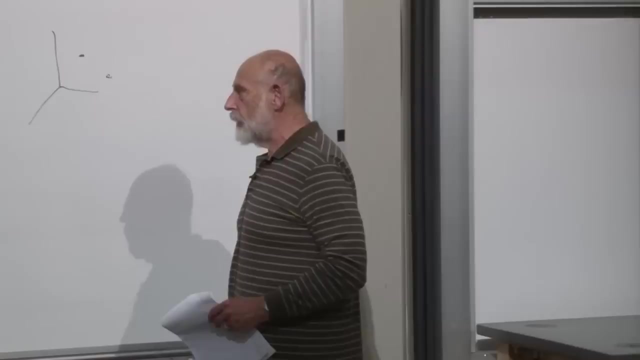 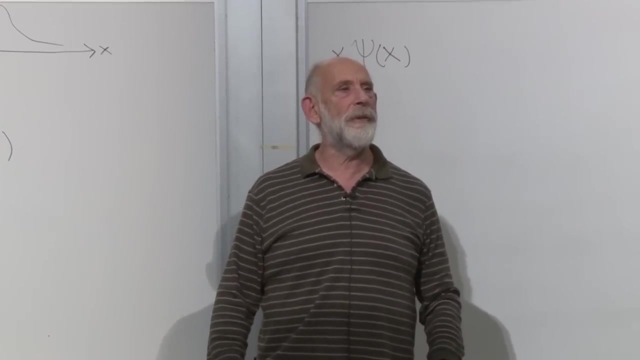 All right. In the same way, The momentum operator. Now, I'm not going to explain this in detail. For this you go back to the lecture notes or to the lectures themselves. What lecture was it that we talked about momentum? Anybody remember? 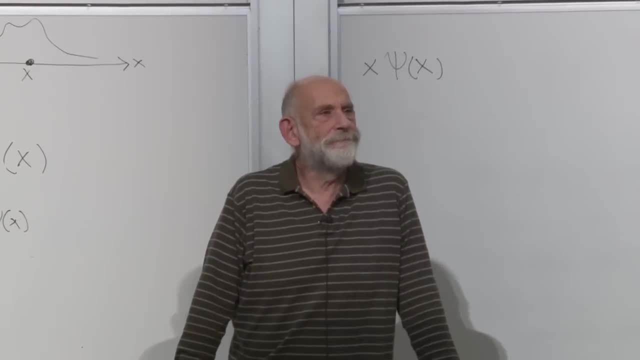 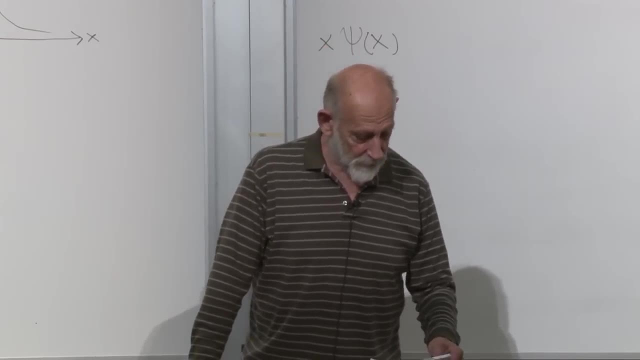 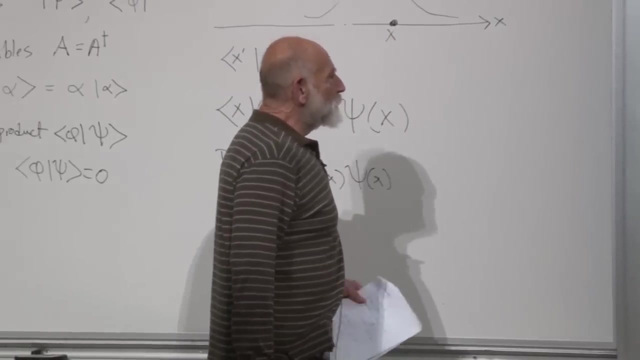 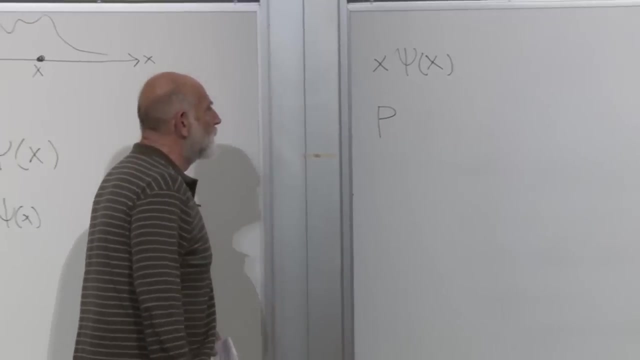 Art, Several of them, but I think around eight Eight. Yeah, yeah, yeah, eight Eight was that's right. I remember, with great grief, Lecture eight, right, Okay. So the momentum of a particle is represented by an operator called p. 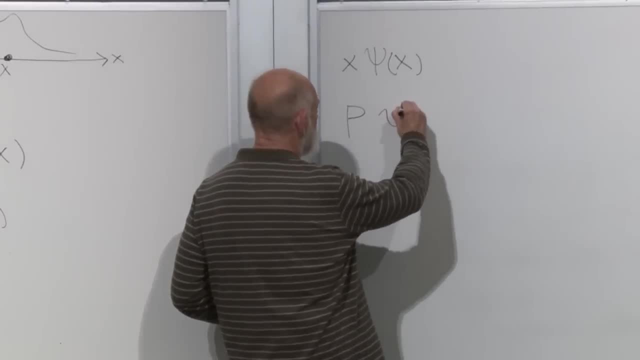 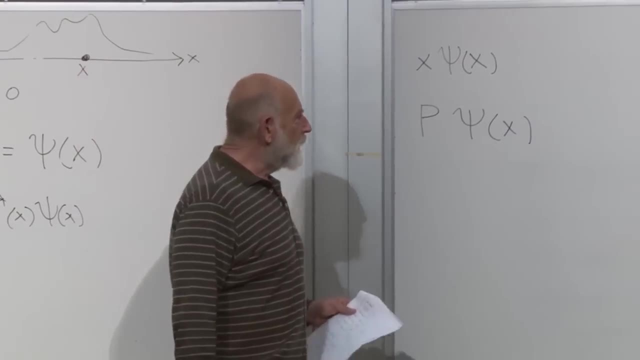 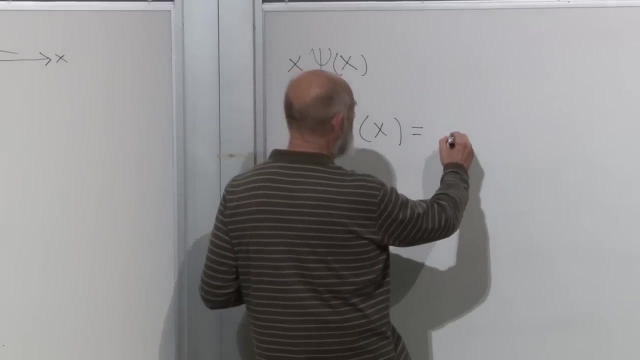 And p also does something to psi of x. What it does to psi of x is it differentiates it. It differentiates it with respect to x, but not quite Really. The original thing is that it multiplies it by minus. i, the complex number, i. 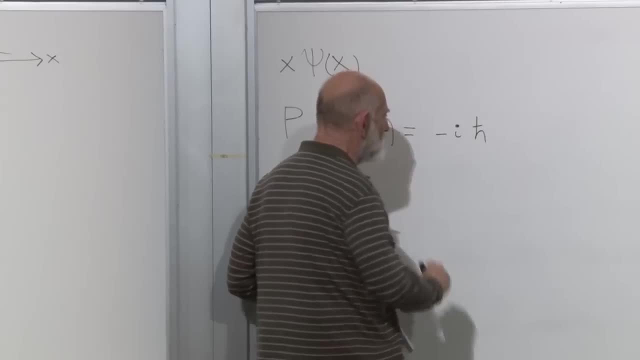 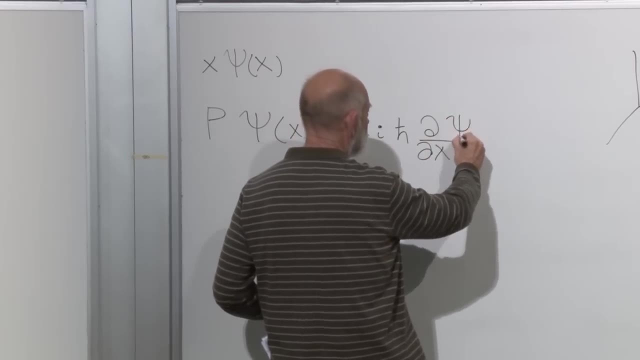 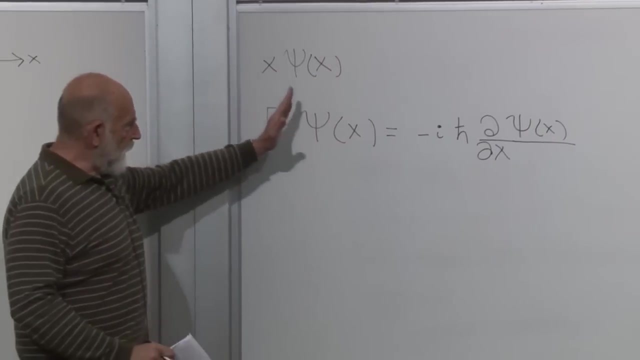 There's a factor of Planck's constant h bar, and then it differentiates psi d by dx, Psi of x. That is the operator that acts on wave functions, That represents the, The, uh, the observable momentum. Everybody remember this. 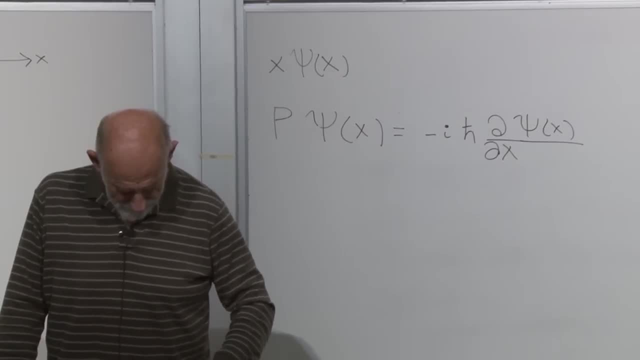 Yeah, We went through it. Okay, Now what about the eigenvectors of momentum? The eigenvectors of position are Dirac delta functions. They are functions which are zero everywheres, except at the, At the, At the. 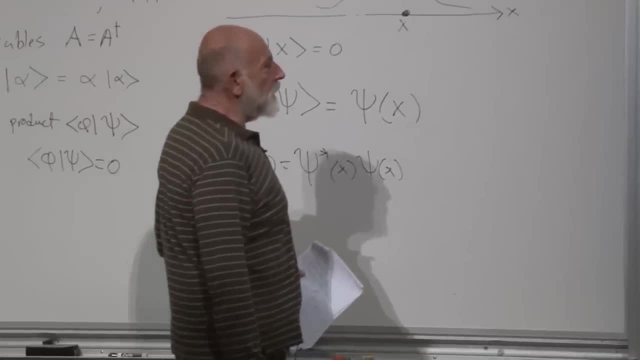 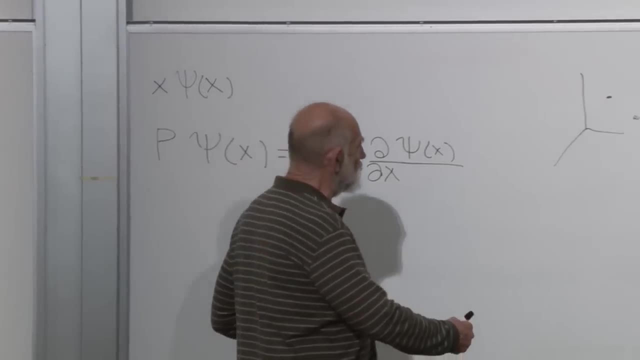 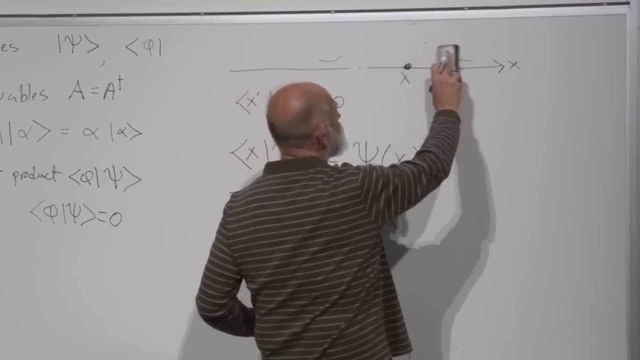 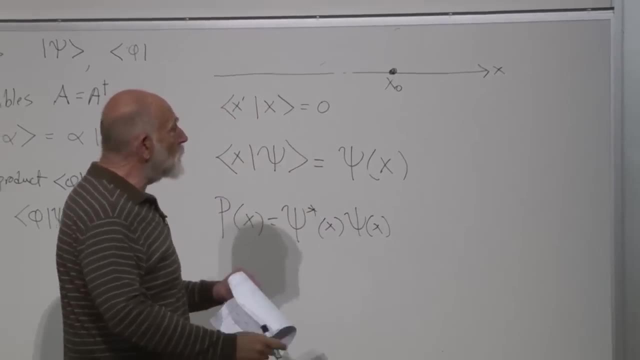 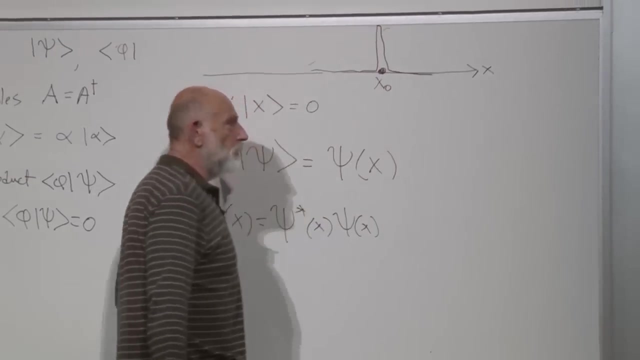 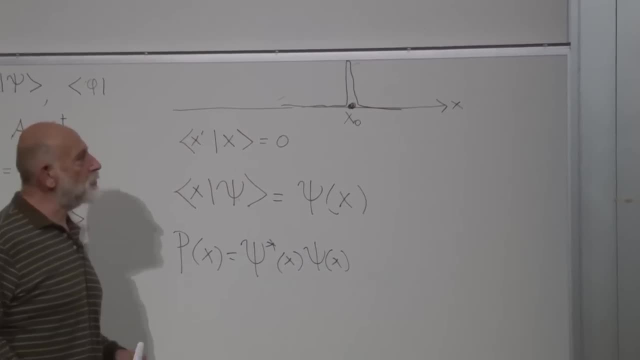 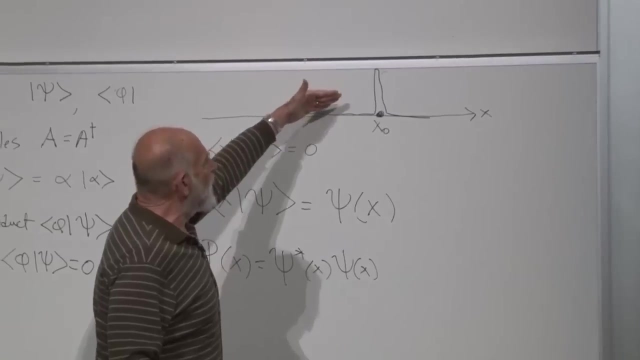 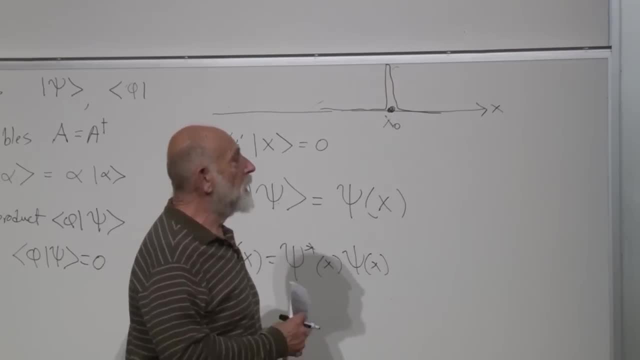 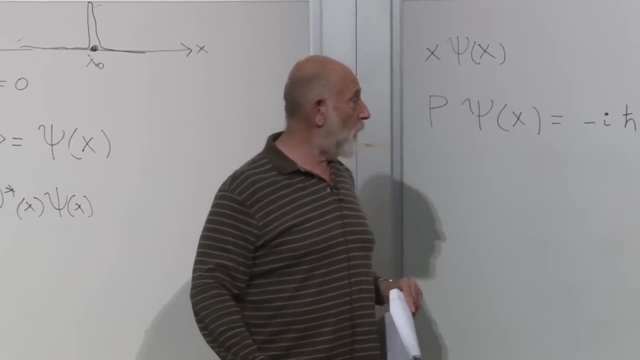 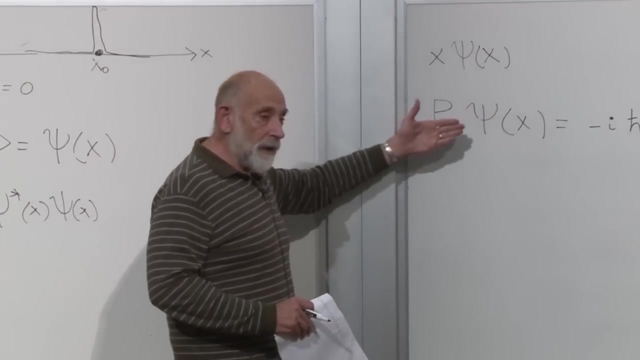 is zero everywhere, except at that point. That, of course, makes sense. Now, what are the states for which the momentum is certain? In other words, what wave functions correspond to particles with definite momentum? And those are gotten by solving the eigenvalue equation. The eigenvalue. 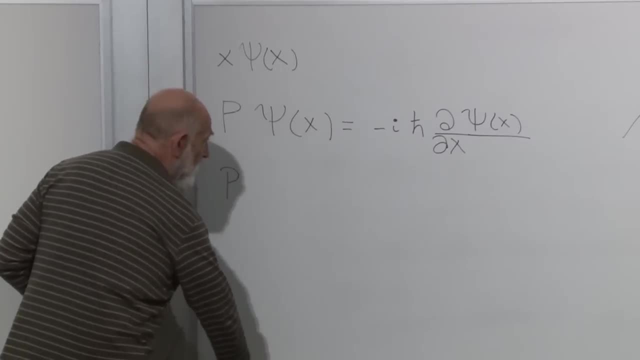 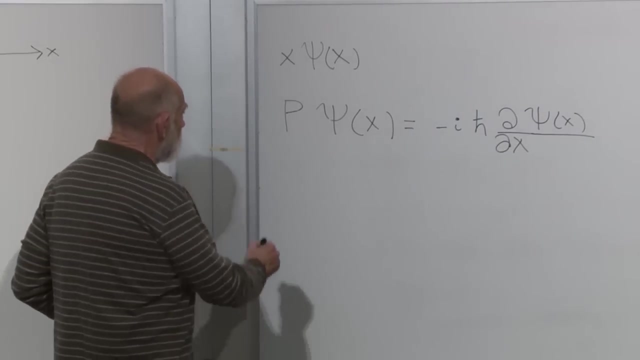 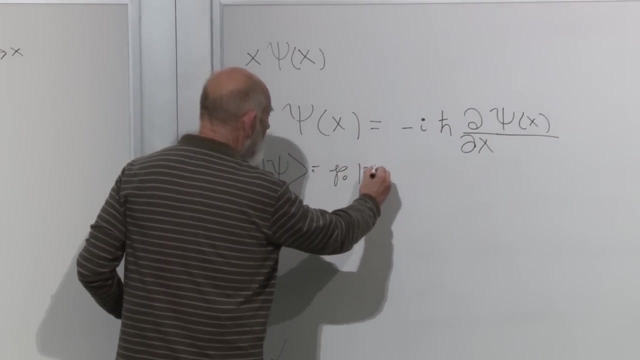 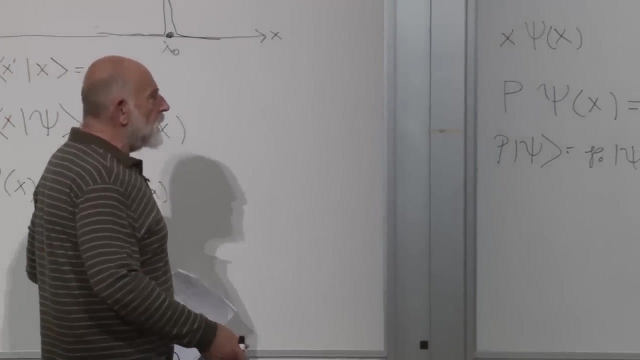 equation is that p, whatever it is, in fact, we know what it is. well, let's write the abstract equation first: that p on psi is equal to little p naught times psi, the eigenvalue being little p naught. Little p naught is the value of momentum that this particle has. 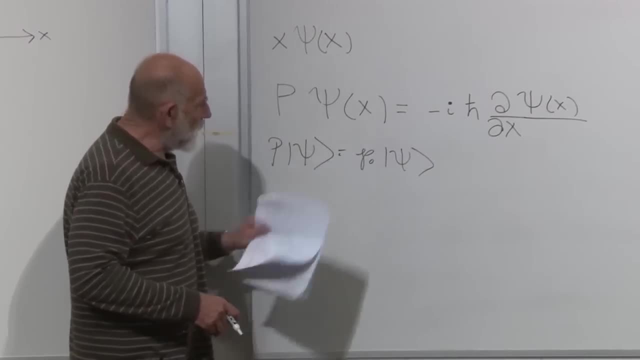 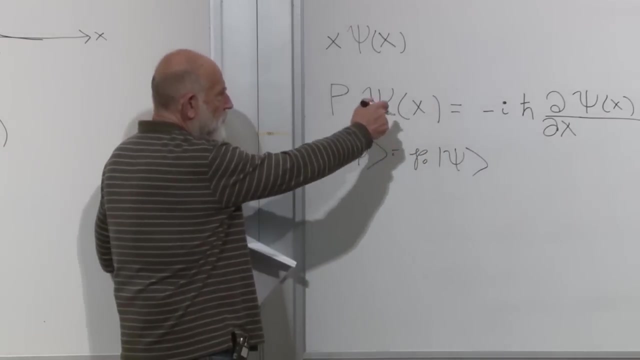 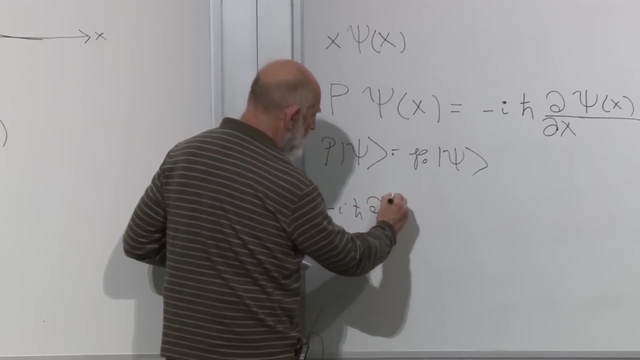 and in this particular state, the. the momentum of the particle is known to be p naught. This equation translates just: replacing p by minus i h bar d by dx. minus i h bar d psi by dx is equal to p naught the number. 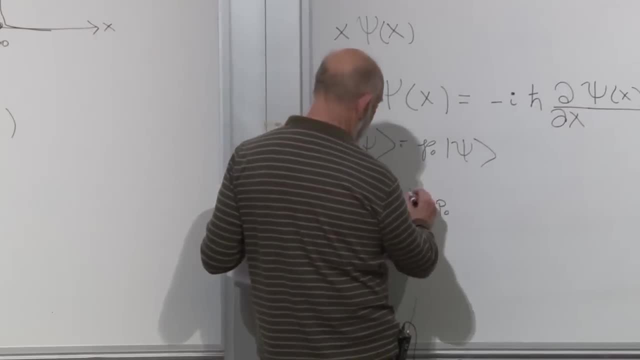 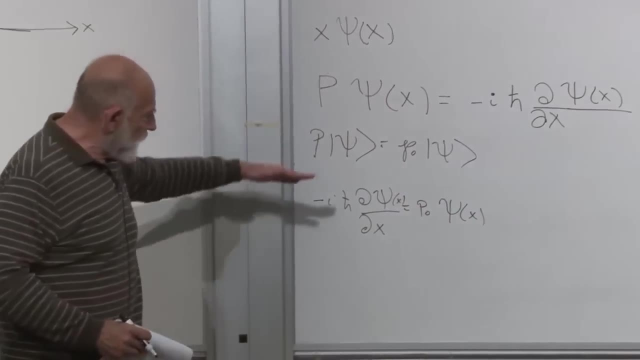 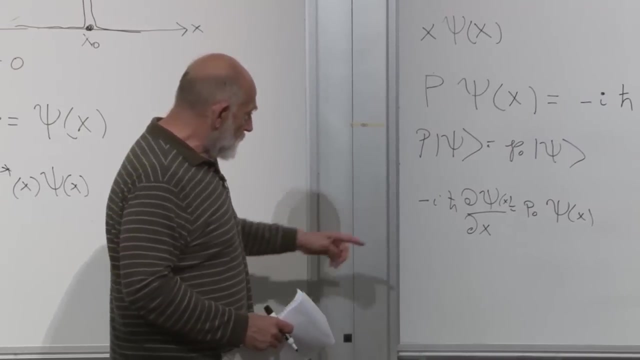 a numerical number times psi of x. Psi is a function of x, psi of x, And this is easy to solve. This is one of these equations which says that the derivative of something is proportional to that same thing, Derivative of psi apart. 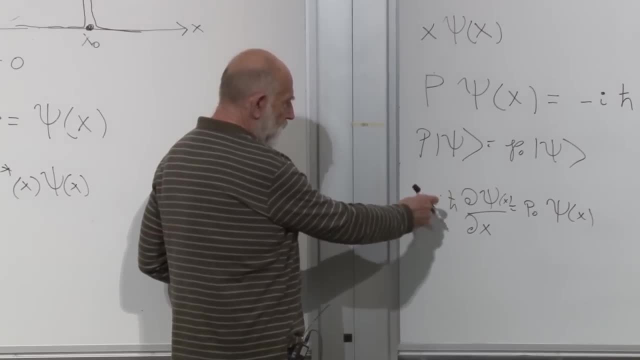 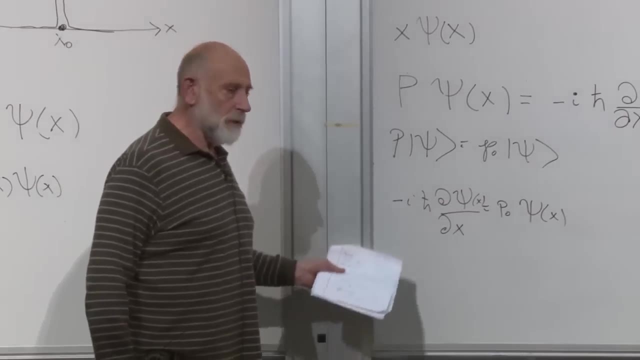 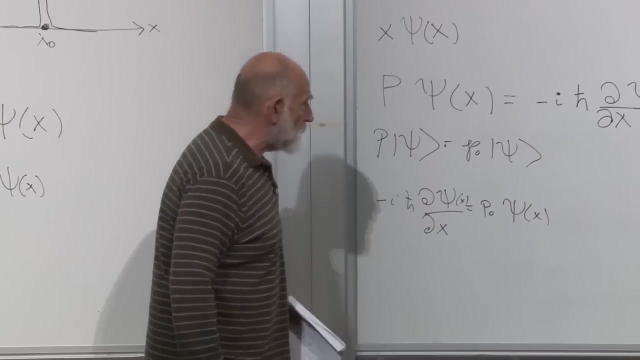 from a numerical number, the numerical number. we could get rid of the i h bar on this side. it would reappear on this side. this is the equation of the type that represents an exponential. The derivative of something is proportional to something itself and the solution of it. 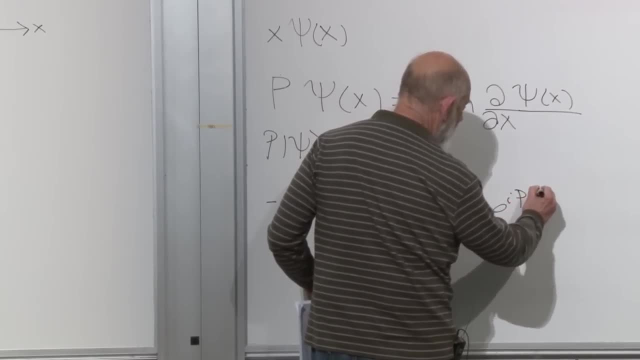 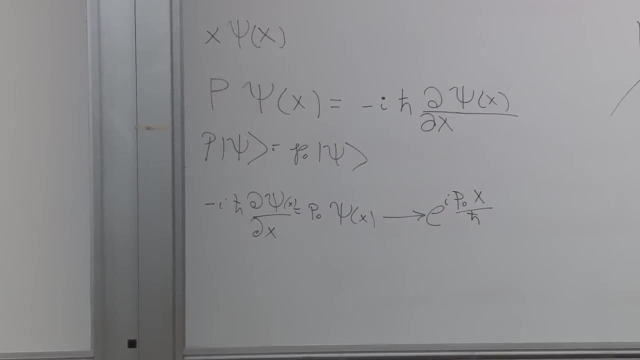 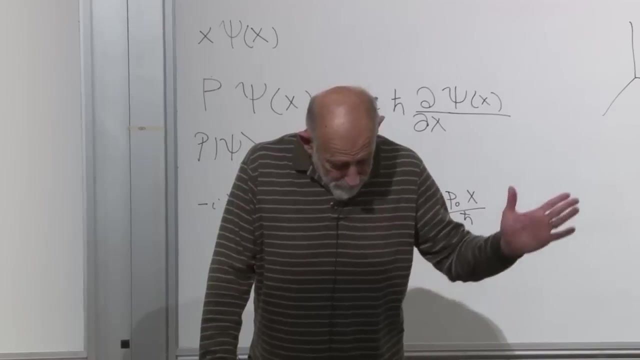 is e to the i h bar. So we have p naught x divided by Planck's constant. Now I often get very tired of writing Planck's constant and I often just set it equal to one. We'll sometimes do that, in fact, from. I'll try to track it for the time being, but 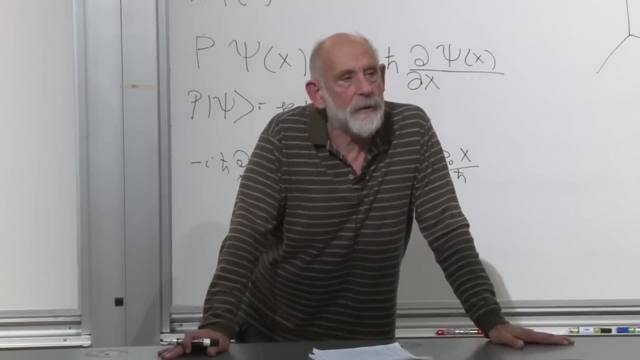 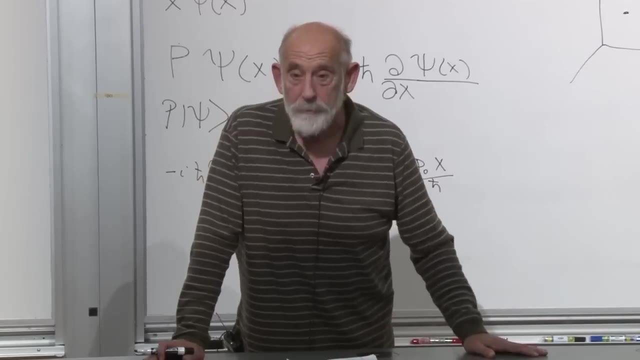 later on I may just drop it, And I think by the time I do drop it I will have done it enough times that you'll know where the right, the right place, where Question. Yeah, In the two equations you just wrote there- the upper one with the with the kets- that 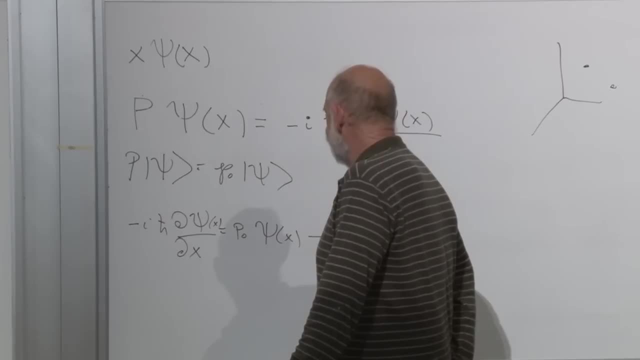 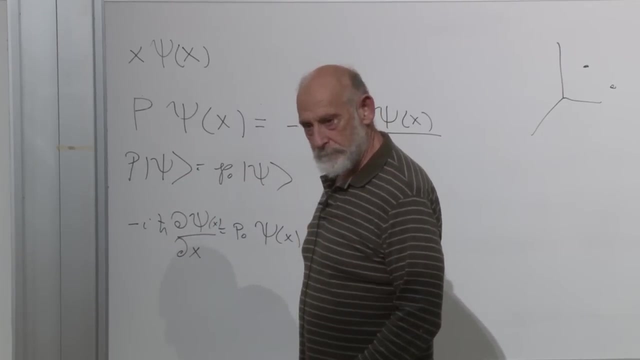 would say that those are or that's a eigenvector of the moment. Yeah, that says that eigenvector. that psi is an eigenvector of p, with eigenvalue p naught, But the one below holds for any wave function right. 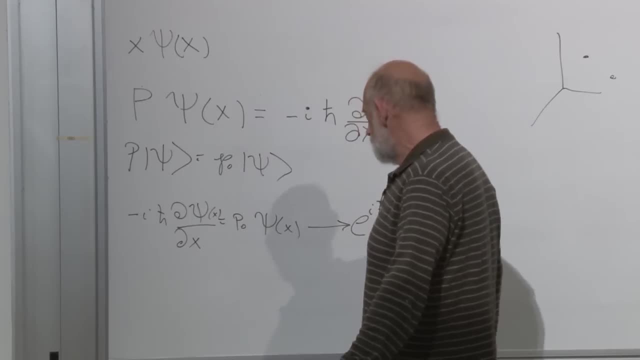 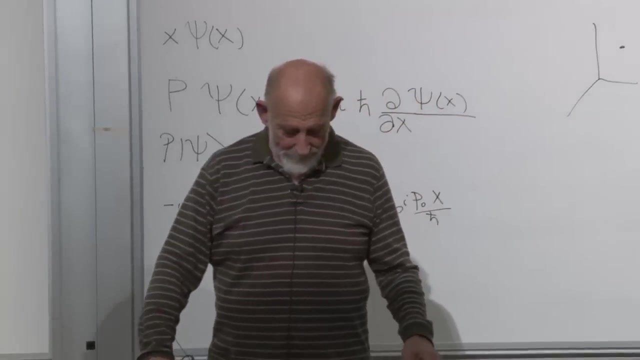 Any. you think any wave function is e to the i, p, a, p, x, No, no, no, but the equation before it, Here, It holds for any wave function. No, The equations don't satisfy this. equation No. 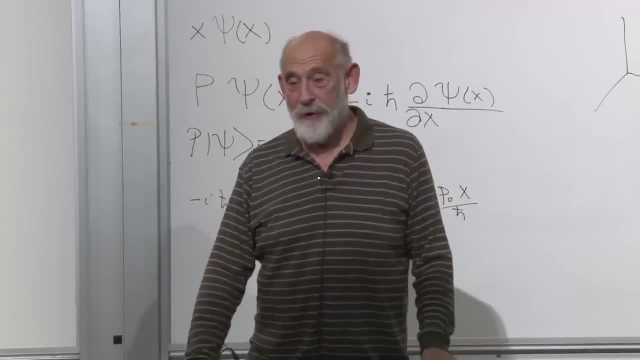 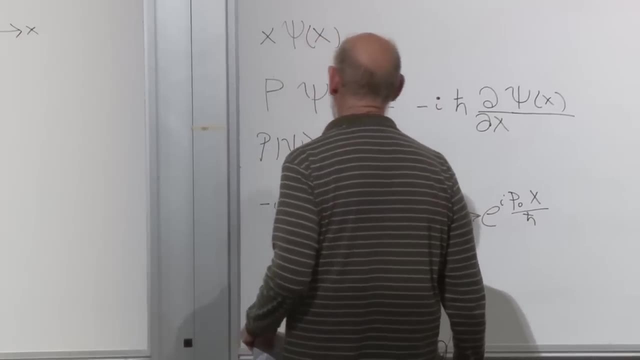 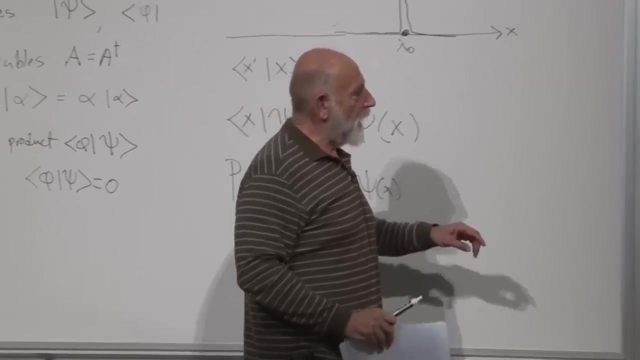 In fact, it's true for basically this wave function. Okay, Now you'll notice, of course, that there's a huge difference between the eigenvectors of position, which are these narrow little spiky functions, and the eigenvectors of momentum. 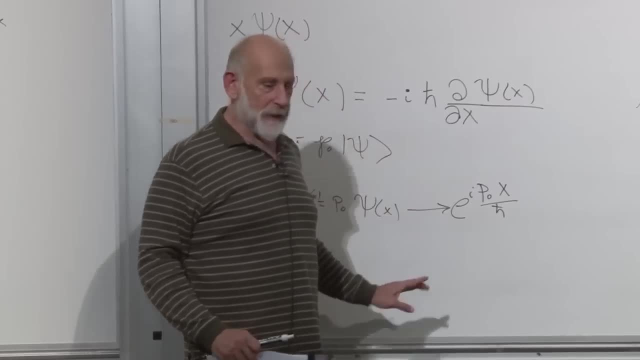 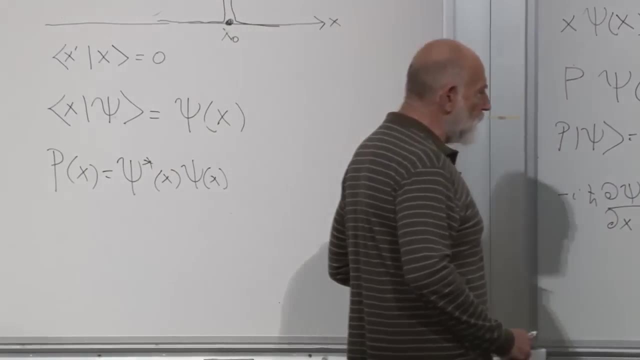 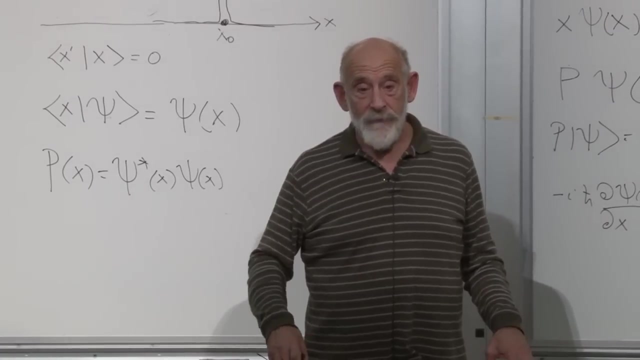 in particular. Let's take the probability that's associated with e to the i p naught x, That's multiply it by its own complex conjugate. What happens if you multiply this by its own complex conjugate? You get one E to the i something times e to the minus i something is just plain one. 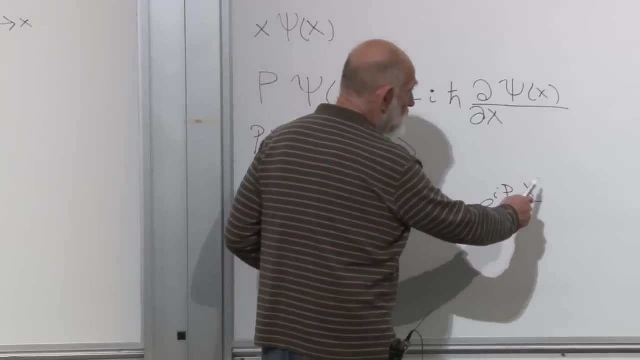 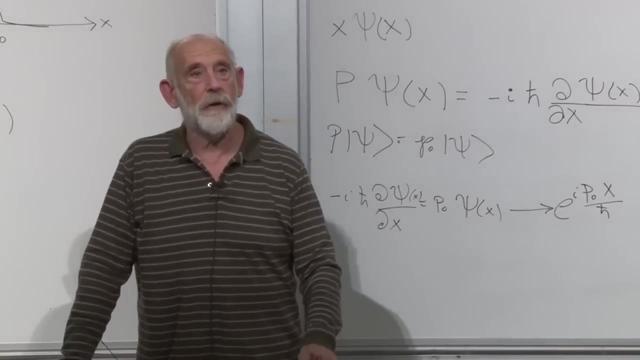 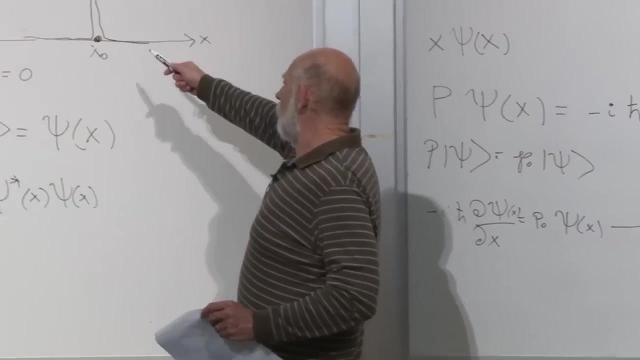 So this wave function, the one which represents a particle at with a definite momentum, its probability distribution is smeared out over the entire line. Okay, By complete contrast, the eigenvector of a particle located at a definite position is highly concentrated, infinitely narrow. 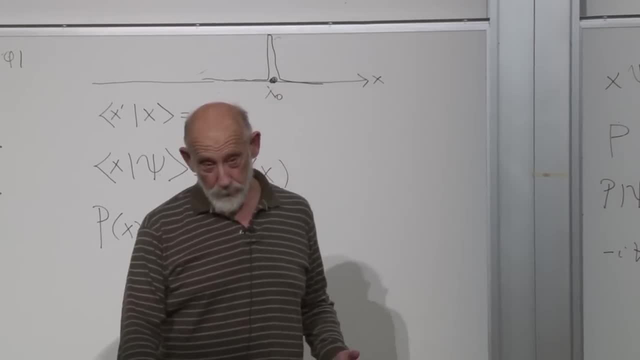 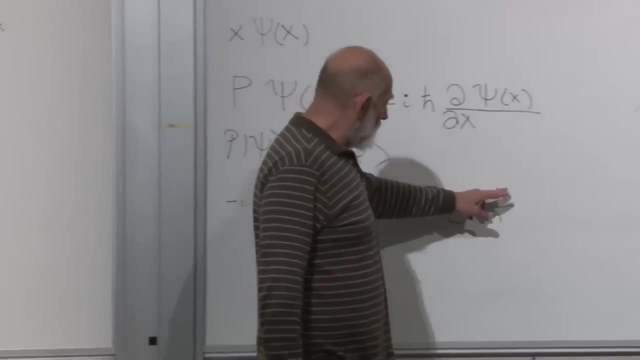 And this, of course, is a manifestation of the of the uncertainty principle. If you know, well, if you know the momentum of a particle, then its position is completely uncertain. And likewise, if you know the position of a particle, its momentum is also uncertain. 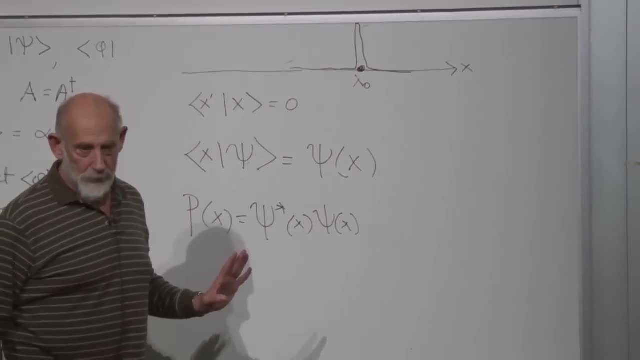 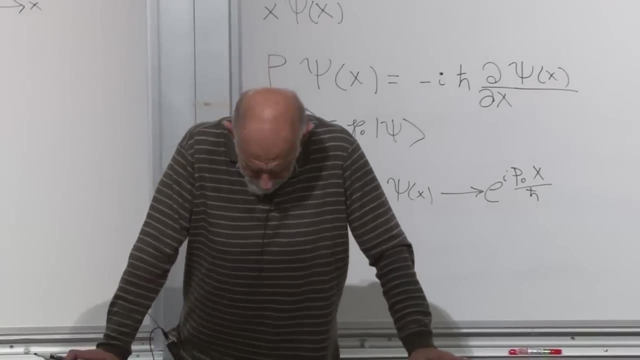 Okay, Well, if you know well, if you know the momentum of a particle, then its position is completely uncertain. If you know well, if you know the momentum of a particle, then its position is also completely uncertain. I'll refer you back to the lecture notes, uh, to for that purpose. 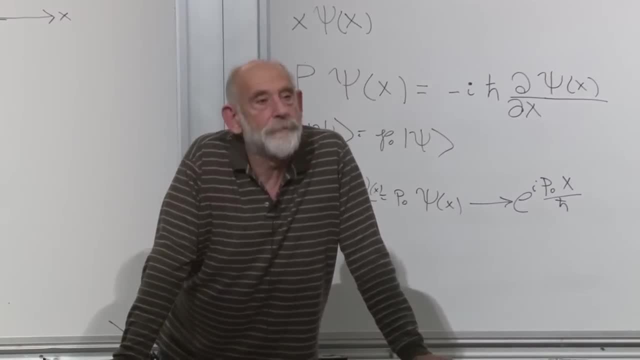 That's basically quantum mechanics in a nutshell. Question, please, I'm a little bit confused. I thought you said this: we know it's p zero. Yeah, So it's known. Yeah, the momentum is known. The momentum is known. 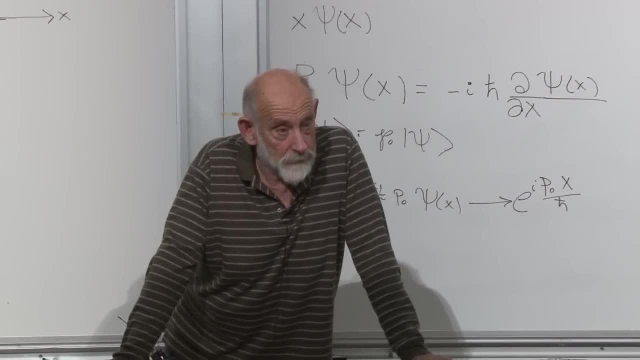 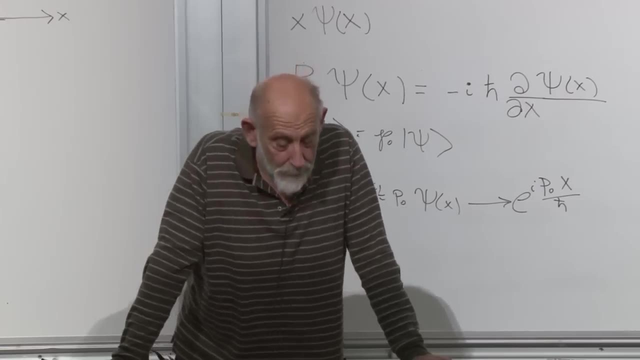 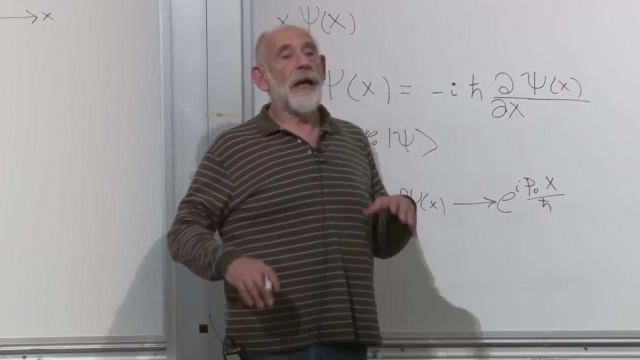 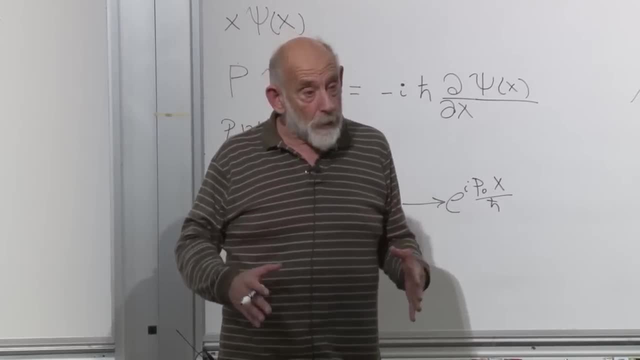 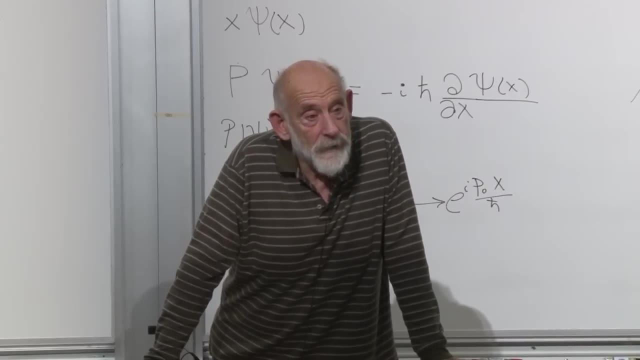 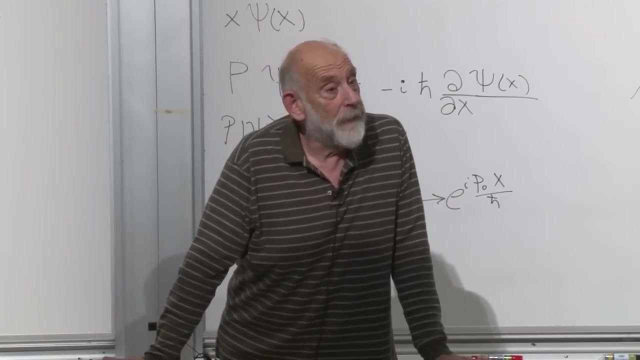 not to check its momentum, but it's going to do an experiment which measures its position. Two different kinds of experiments: Hm, And that was phi of x. Phi of x is- Sorry, The the probability of amplitude for position. That's right. 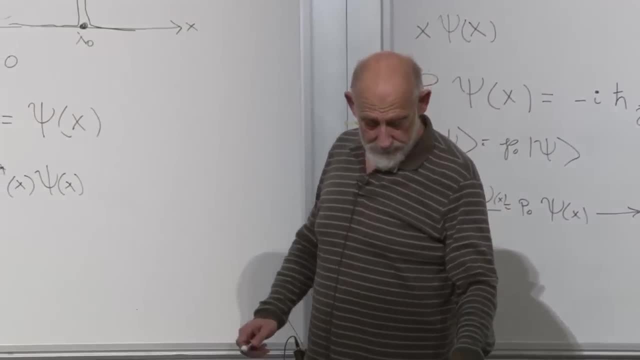 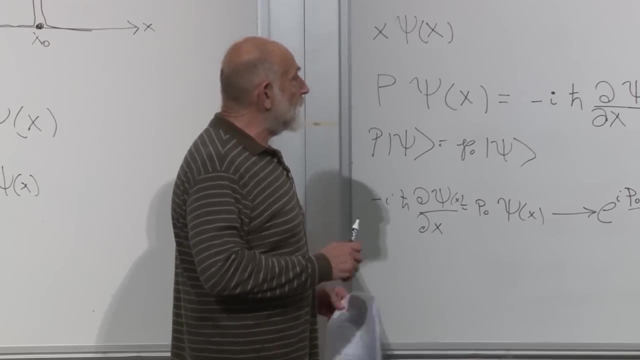 That's right. If the argument That's right, That's correct. There's also a notion of an amplitude for finding different momenta and I'll just remind you that's connected to Fourier transforms of psi, of x. But I'm not going to do that now. 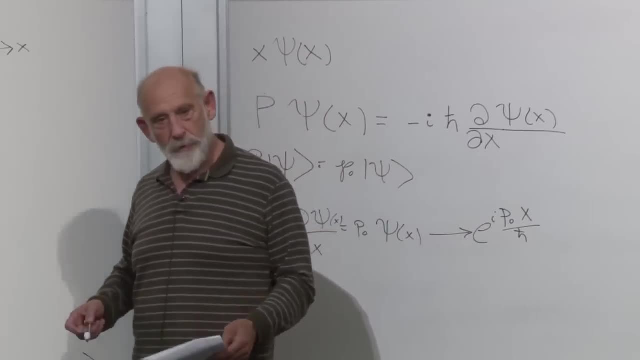 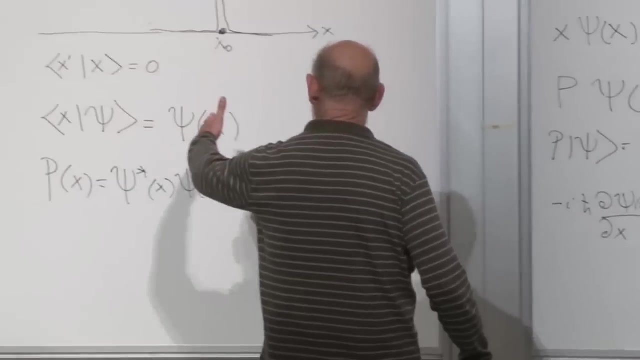 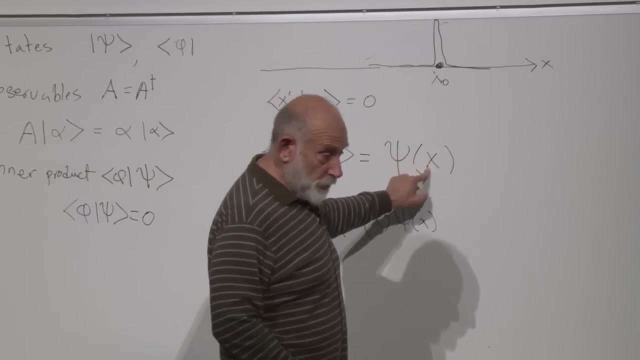 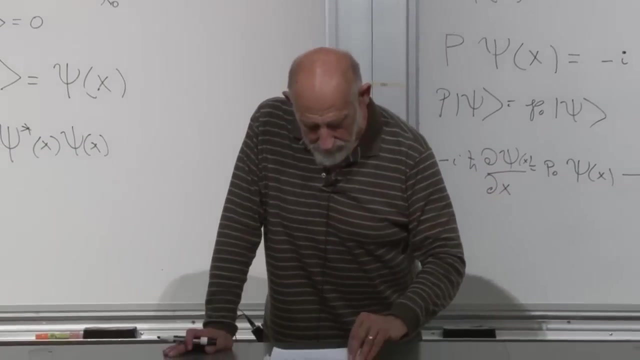 If we need Fourier transforms, we'll come back to it. At the moment, Fourier transforms and the momentum representation. this is called the position representation. The representation of state vectors by psi of x's is called the position representation. There is also a momentum representation, but it will take us too far afield right now. 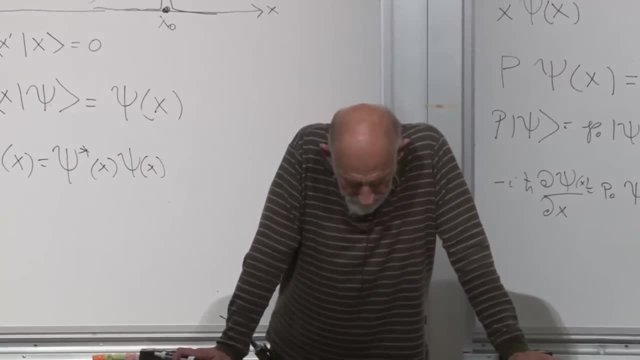 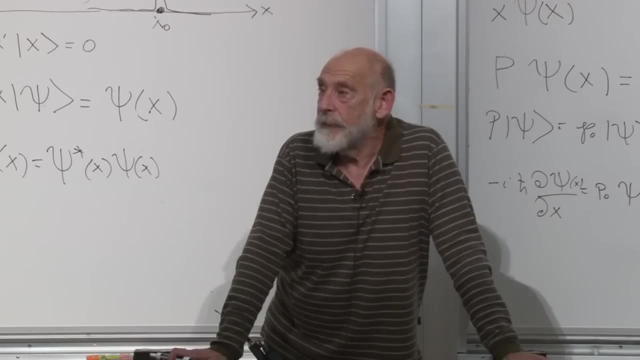 Question Yes, What is the probability of the position? So, in other words, Psi, star, psi of x, If the psi function, the wave function, is the Dirac delta function. what is it when you multiply that You know the wave function. 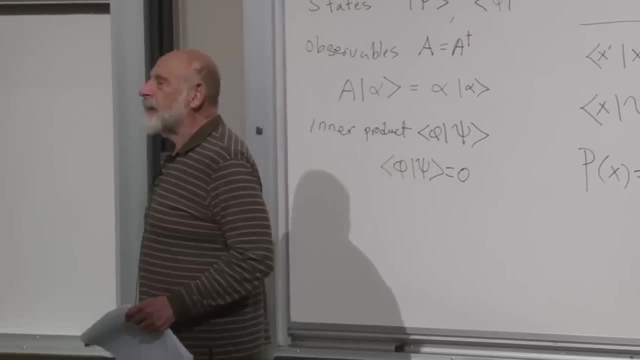 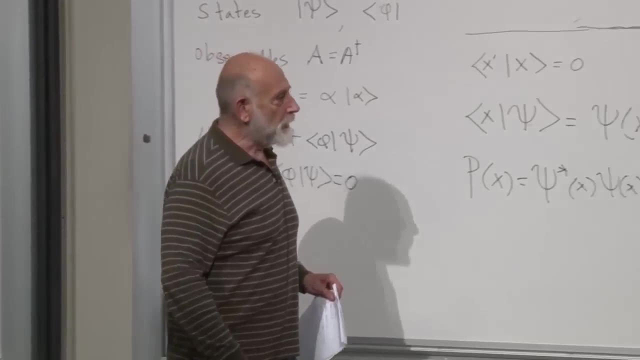 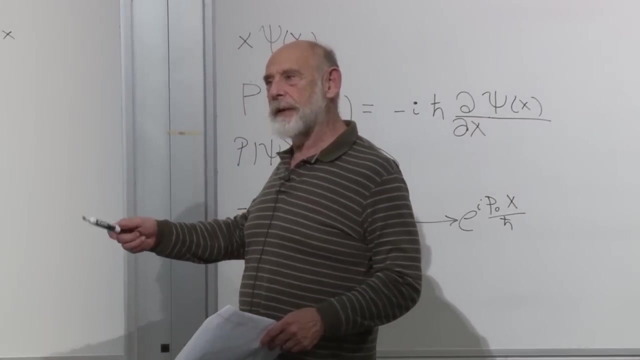 When you get it to probability, what does that look like? It looks like the square of a delta function which is just higher than the delta function, but it's concentrated at the origin. It's concentrated at the origin and we have not talked about normalizing wave functions. 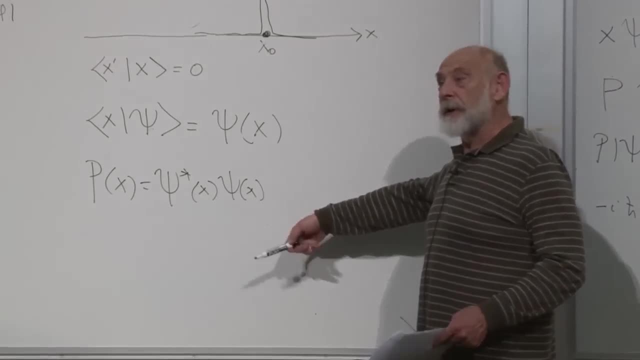 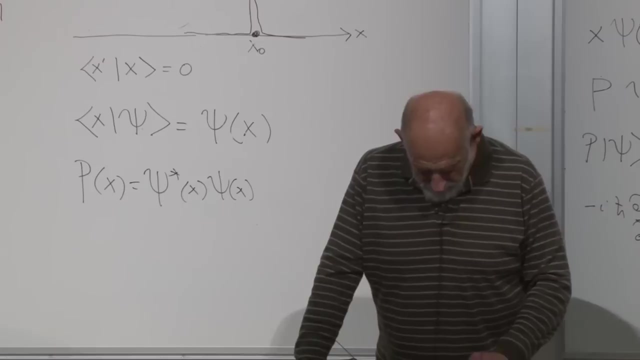 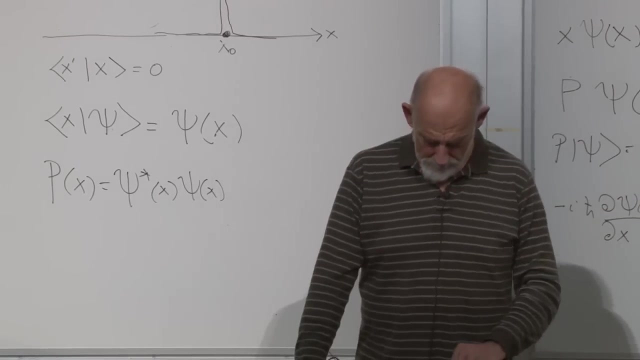 making the area under here equal to one. That's a thing that we want to do, but, as I said, I hesitate. I hesitate to go into any given thing too deeply because we'll wind up doing the whole class again. Yeah. 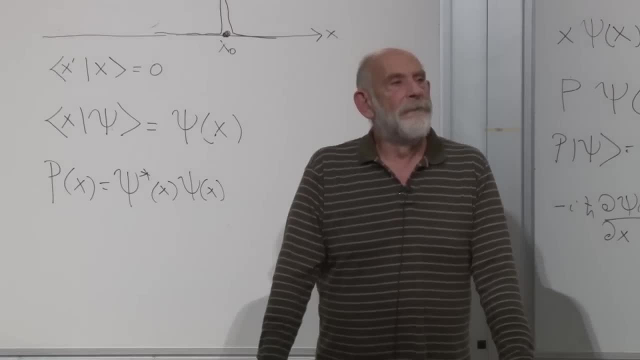 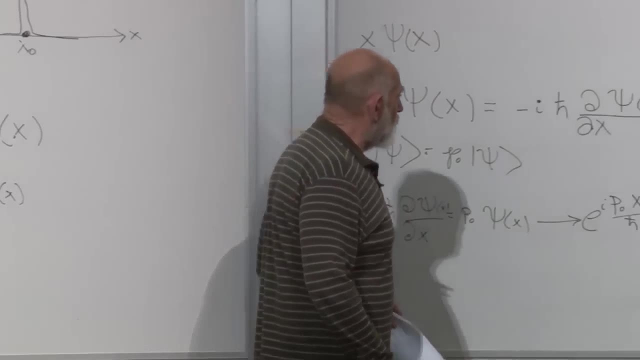 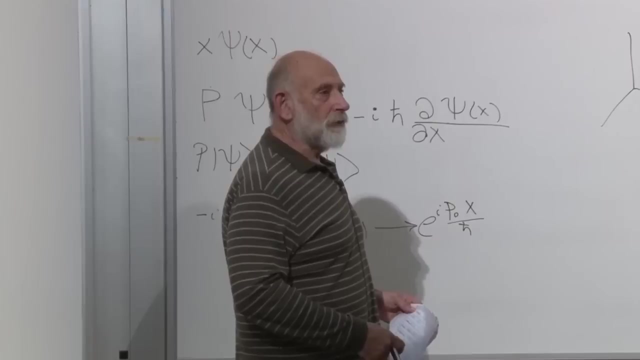 So these state vectors are all represented by column vectors, is that it? You can represent them by column vectors, in other words. but it would be a little awkward to represent psi of x by a column vector. X takes on a continuous infinity of values, whereas the column vector is useful for a. 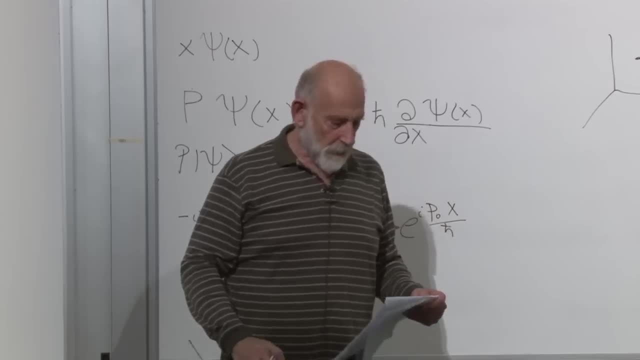 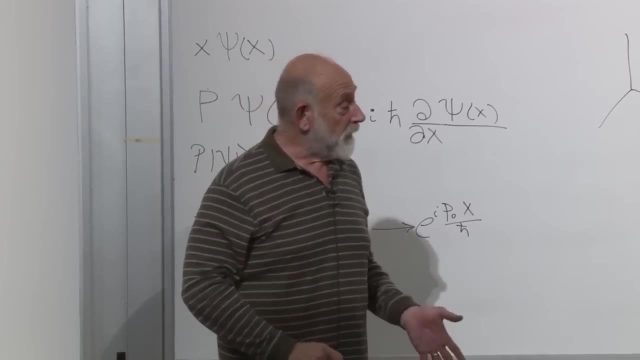 quantity which takes on some discrete set of values. So you'll get the idea. Okay, So you can think of it formally in your head as some kind of continuous column vector. That's for the ket vectors and the bra vectors you can think of as rho vectors, okay, 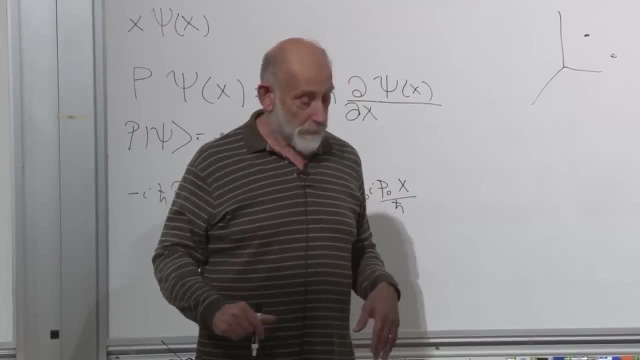 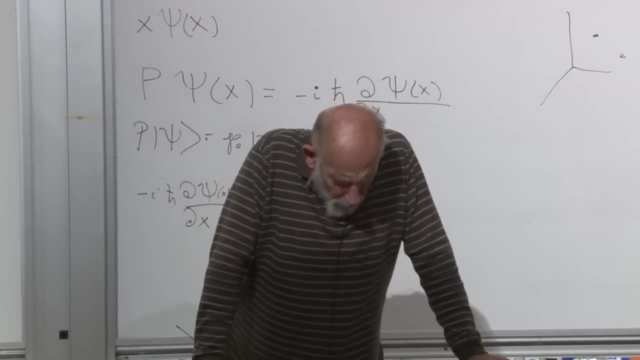 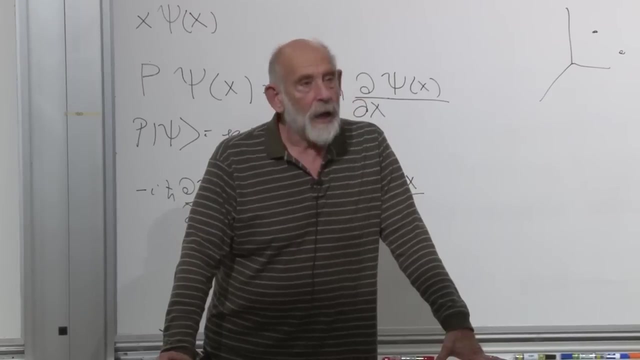 But when we need that, I'll remind you. By then you will have gone back and studied the lecture notes and you won't need it, Okay. Next thing: how do things change with time? Things do change with time, Okay. 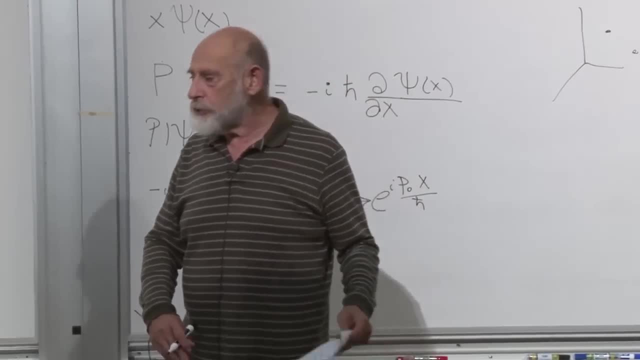 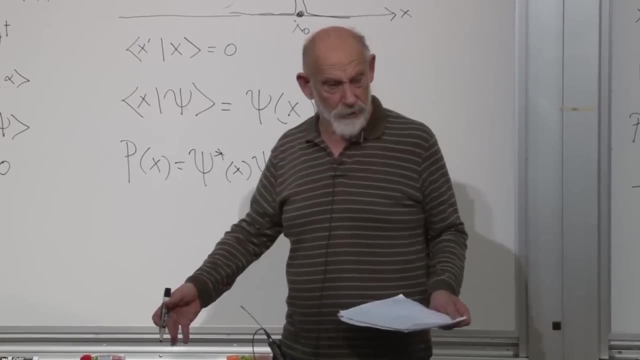 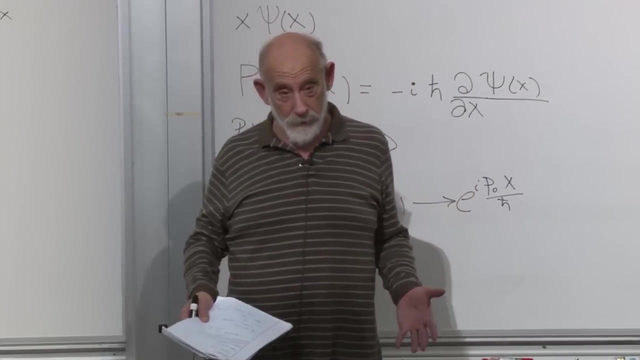 And the evolution of a system with time is a special case of transformations that you can do on the state of a system. That, of course, is also true in classical mechanics. The motion of a system is represented as a transformation in phase, space. a transformation. 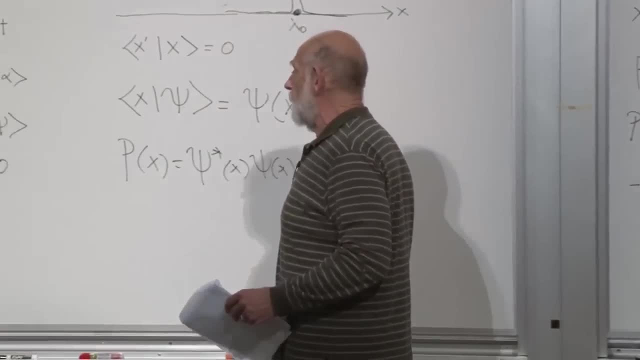 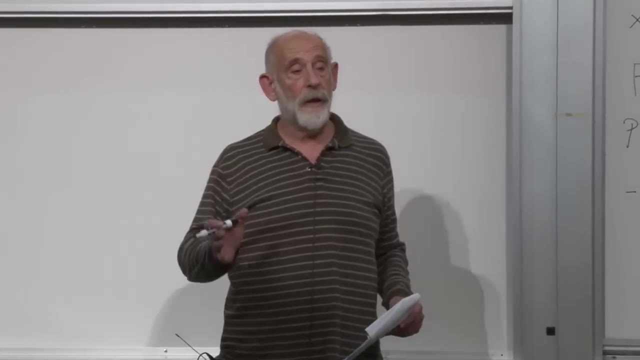 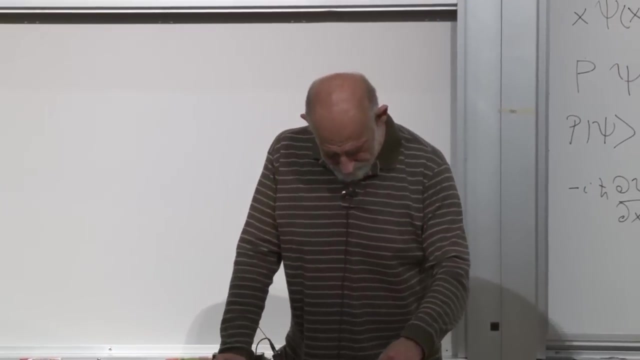 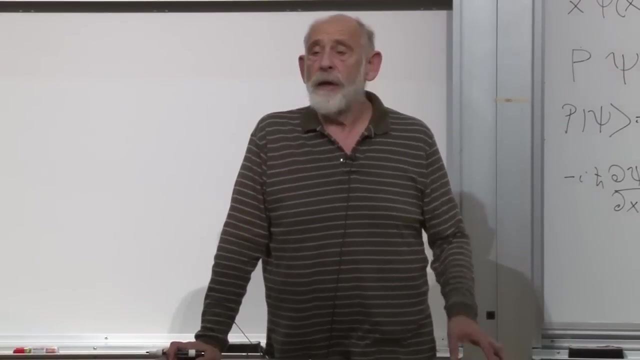 of the phase space position In quantum mechanics. the evolution of a system is a special case of a transformation that you can do on the space of states, taking every state to some other state, And of course the idea is very straightforward: If the state at one instant of time is some psi, at some later instant of time it is. 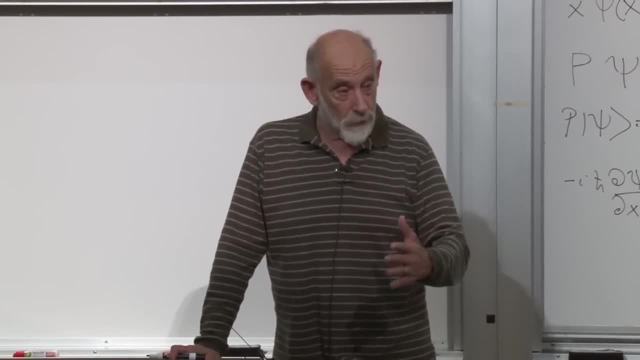 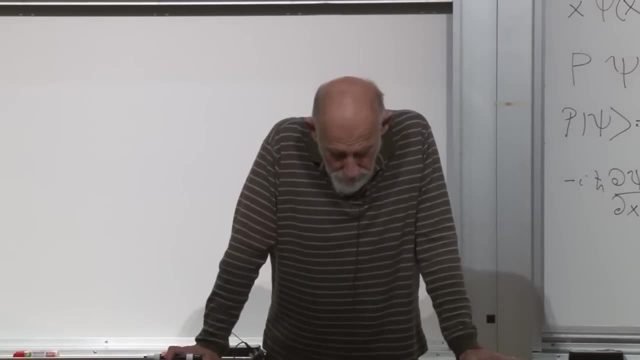 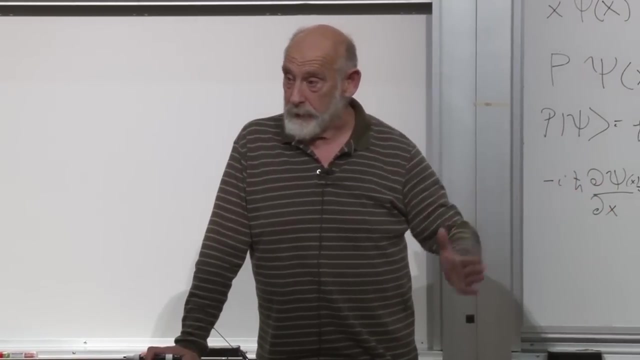 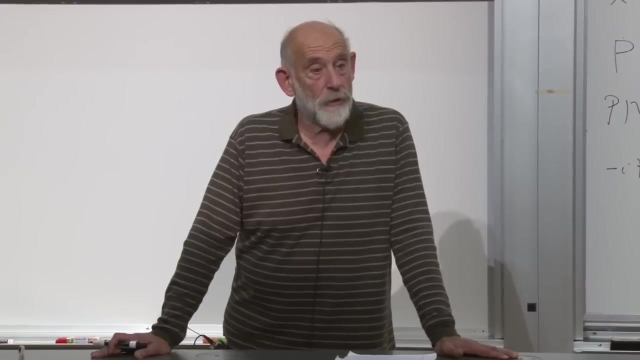 something else, and that something else is a transform or a transformation of the original psi. Okay, Okay, All right, So let's talk about the evolution of that transformation. Oh, that transformation depends on the amount of elapsed time. okay, If the amount of elapsed time is very, very short, then you would expect this transformation. 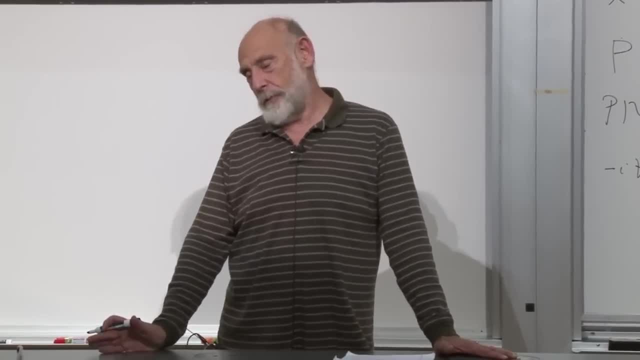 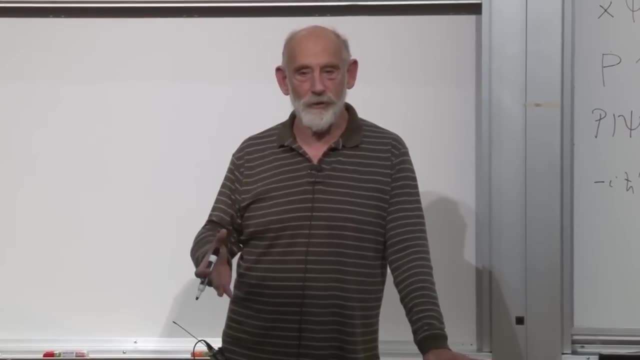 to practically be the identity transform. In fact, let's go back. If the amount of time that's elapsed is zero, then of course the transformation is completely trivial. It just gives back the same state You can say in that case. 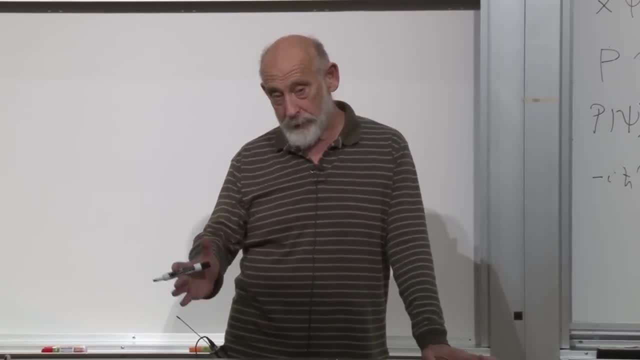 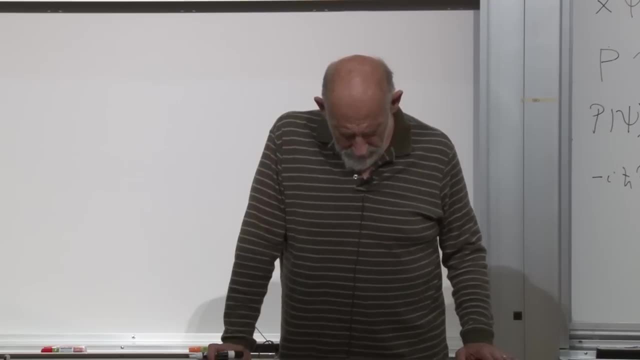 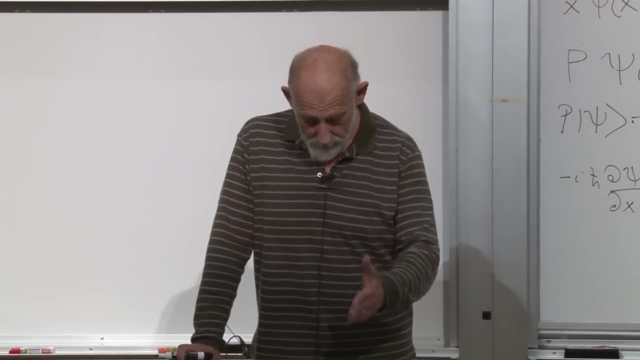 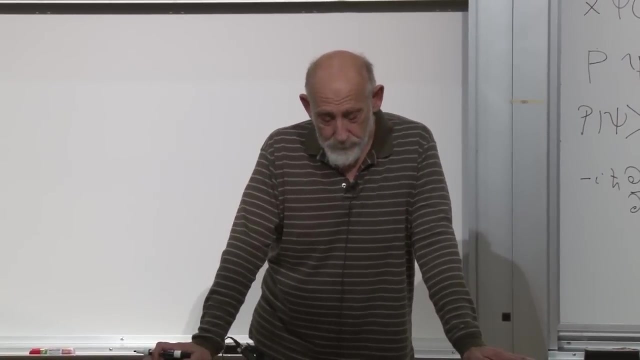 That the transformation was just the identity operation on the state vector, But more generally the time evolution is characterized, or the time evolution operation. let's now call it operator. It is an operator in the sense of operators. It's an operator, but it's an operator which depends on the amount of elapsed time. 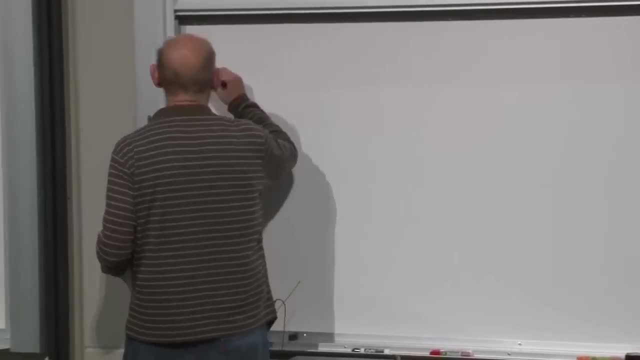 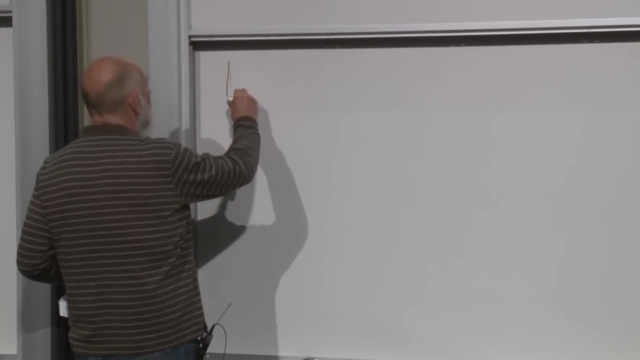 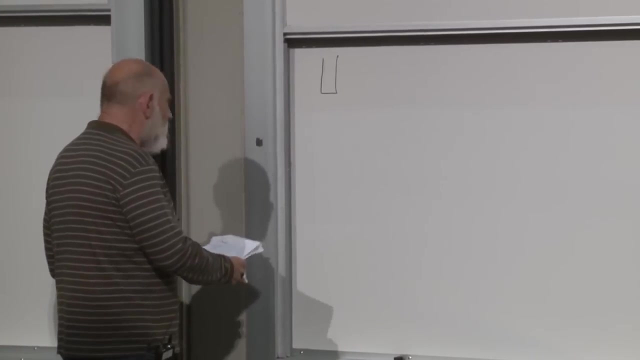 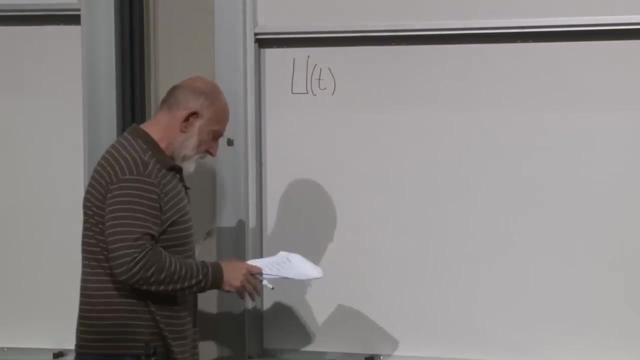 So let's give it a name. It's usually called u. Okay, u stands for unitary, but we'll come back in a moment for what unitary means. And it's parameterized by an amount of elapsed time, And it's such that when it acts on a state at a given instant of time, 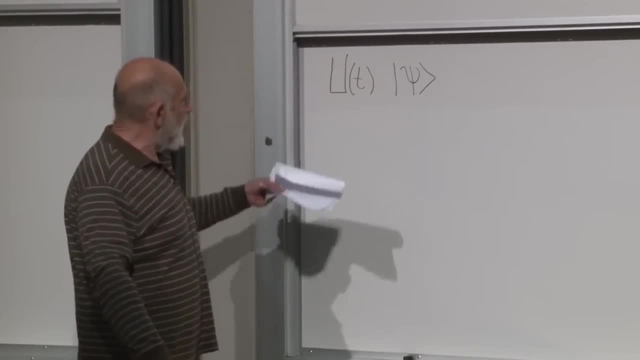 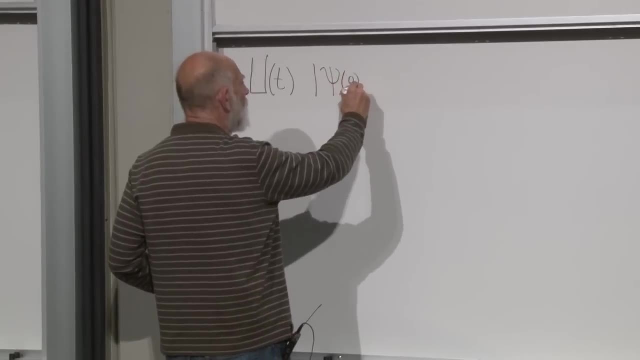 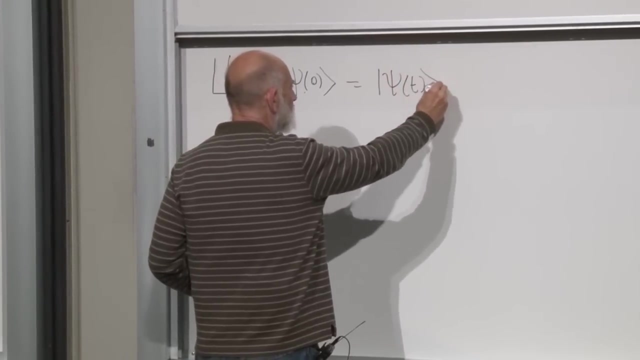 Okay, Okay, It takes you to the state at an amount of time t later. So, for example, if it acts on the state, whatever the state happens to be at time, t equals zero. then it will give you psi at time t. 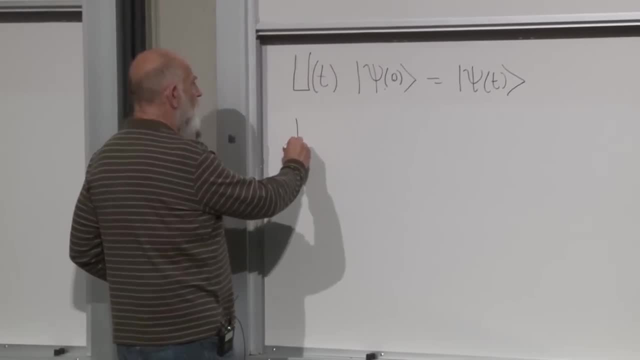 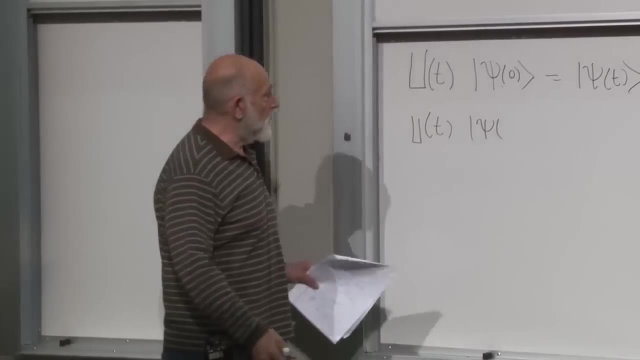 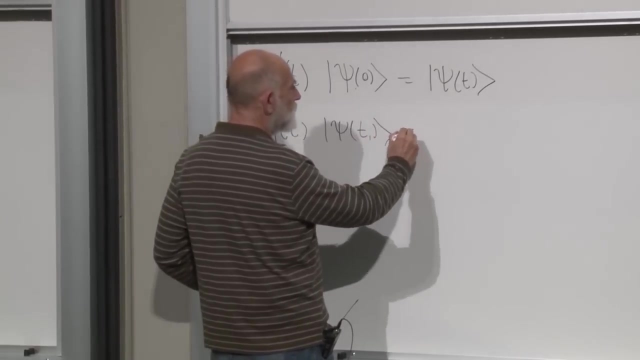 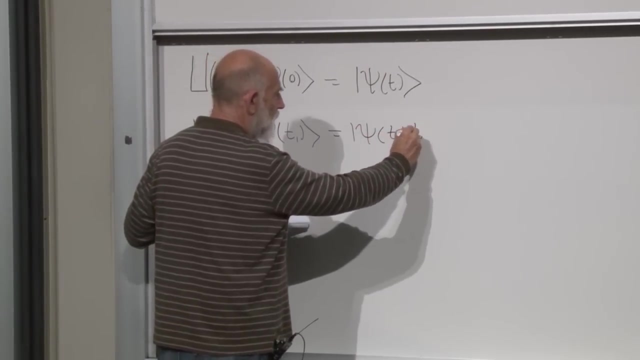 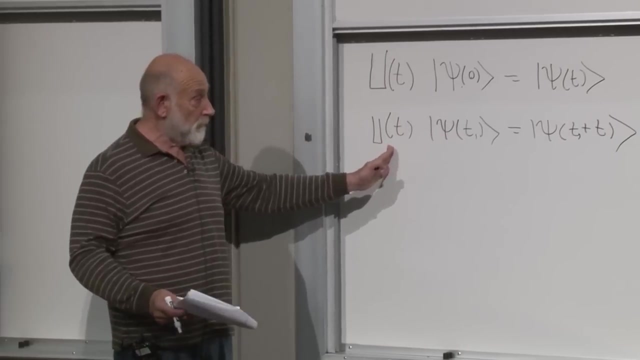 It just updates the state. If it acts on some state which happens to represent things not at time zero but, let's say, at time t1. Okay, Then it takes you to the state at time t1 plus t. In other words, it represents the evolution of the system from t1 to t1 plus t. 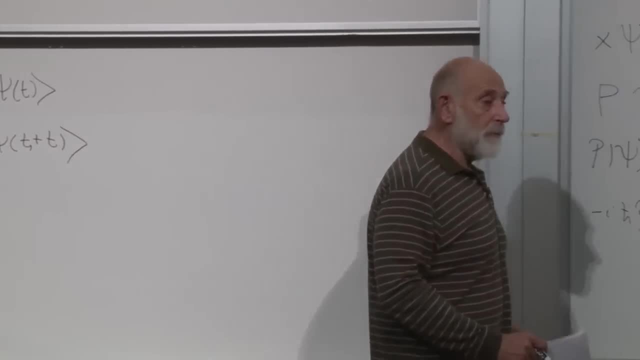 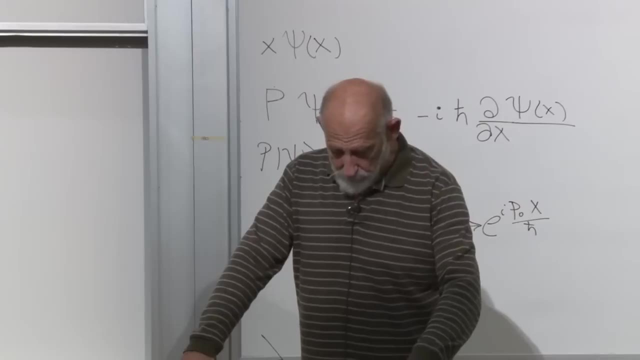 That's the notion of u. That's the notion of a time evolution operator. It's a linear operator, but it is not a Hermitian operator. What kind of operator is it? Well, now we need a postulate, And the postulate is: 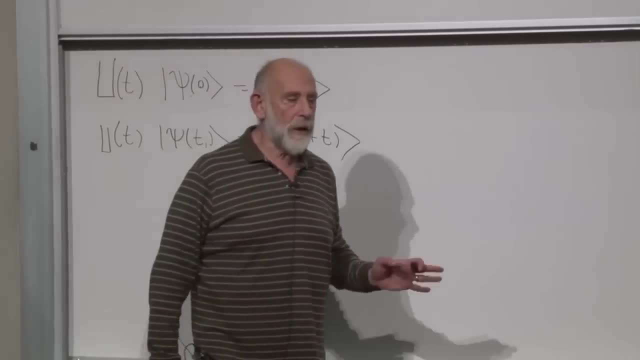 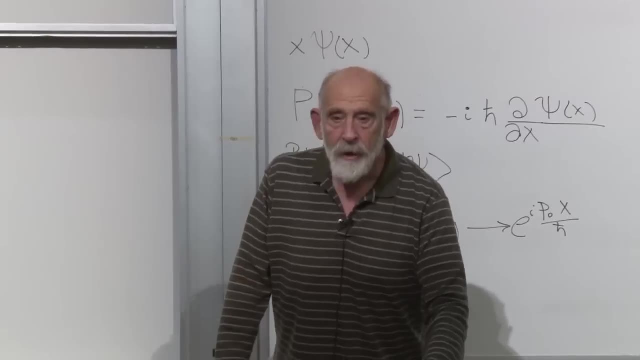 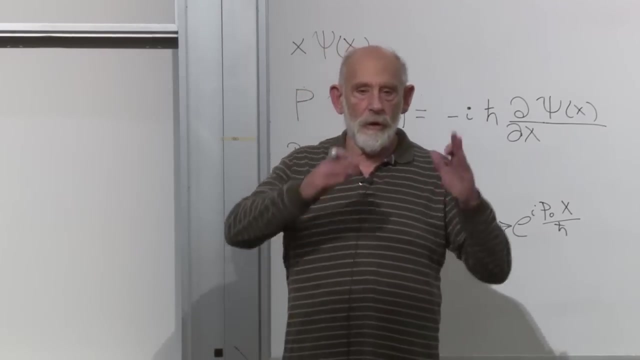 We can say the postulate very easily. It goes back to this minus first law of physics that I harp on all the time, that information is conserved In quantum mechanics. what it means is that if you start with two vectors, two states, 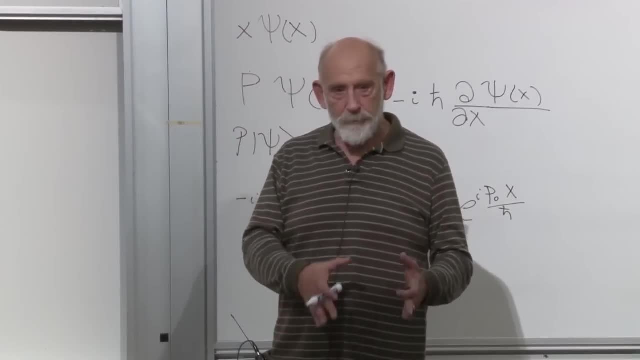 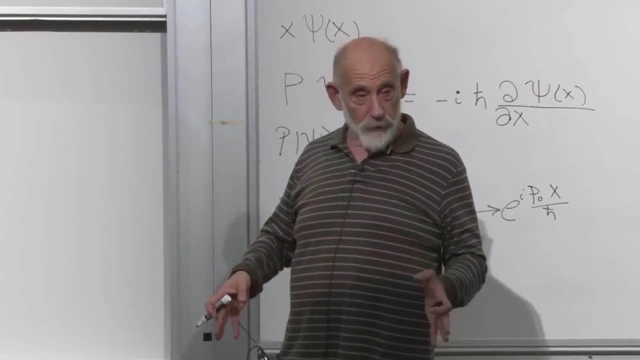 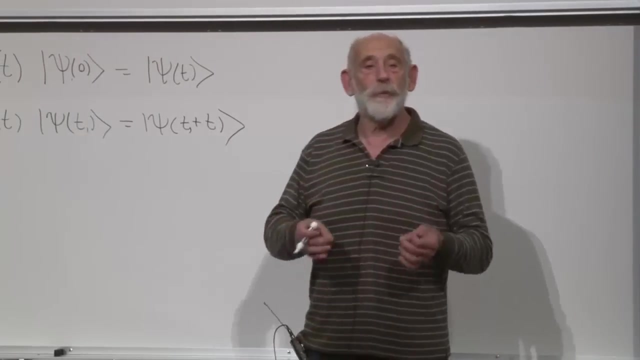 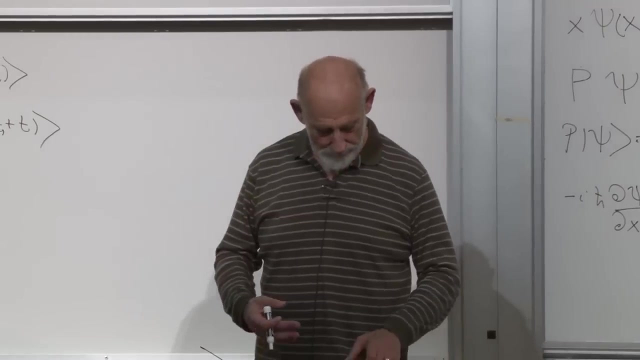 which are observably different, which cannot be confused, in other words, which are orthogonal, and you let both of them evolve, they will stay orthogonal. It will not happen that two states that are observably different will evolve into into states which are not observably different. 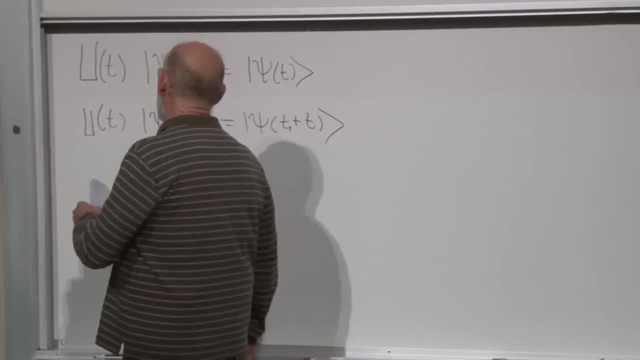 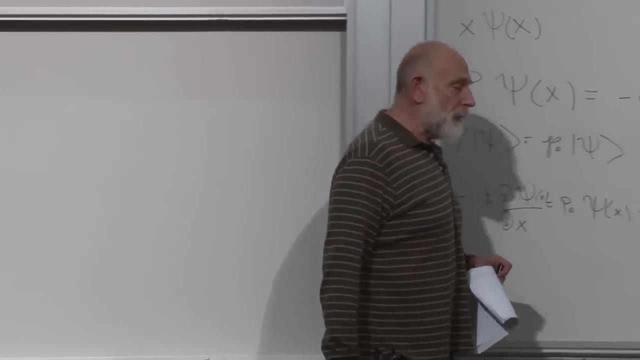 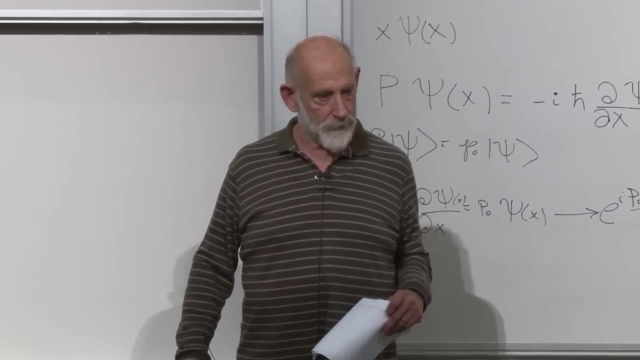 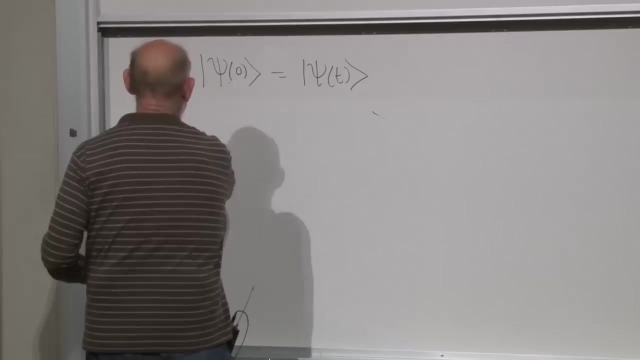 All right. so what that says is that orthogonal vectors remain orthogonal. In fact, you can do a little bit better. You can prove from that statement that the inner product between vectors is unchanged by time. okay, So let me just explore that idea a little bit. 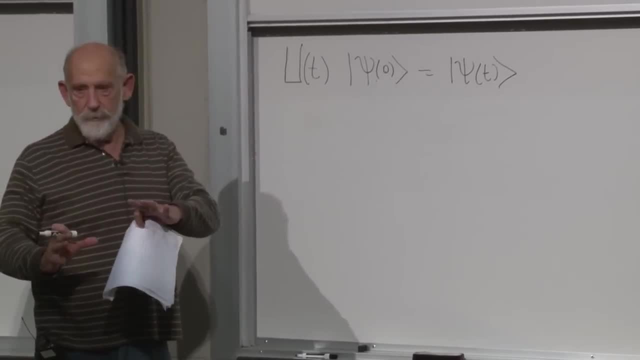 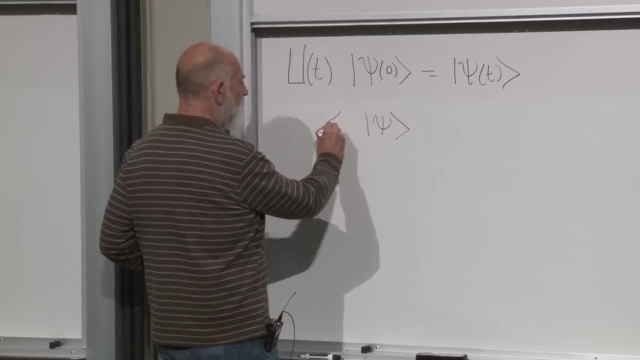 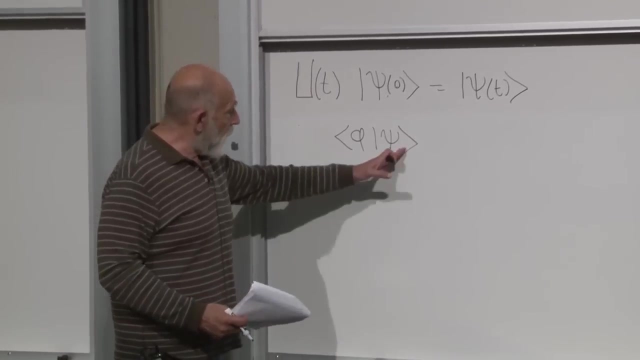 Whatever u is, it preserves the relationships between pairs of vectors. So, for example, if we start with psi and phi, two vectors, they may be orthogonal or they may not be orthogonal. If they're orthogonal, this inner product is zero. 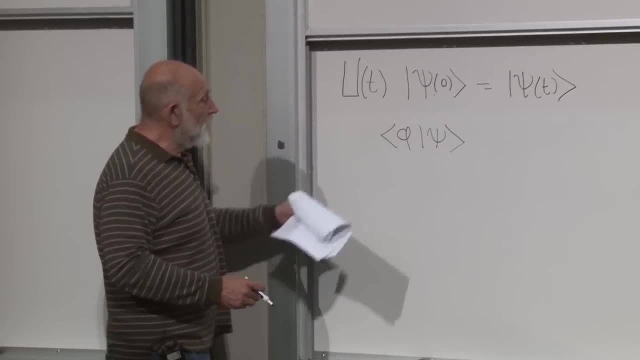 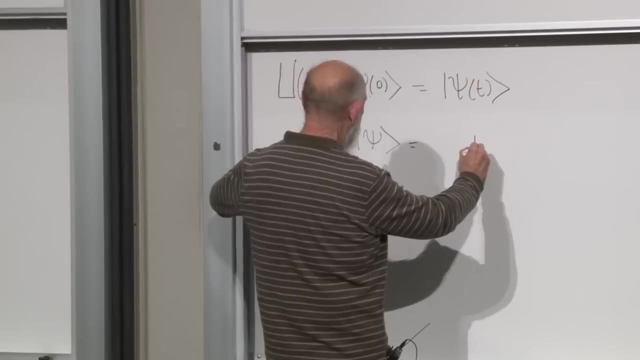 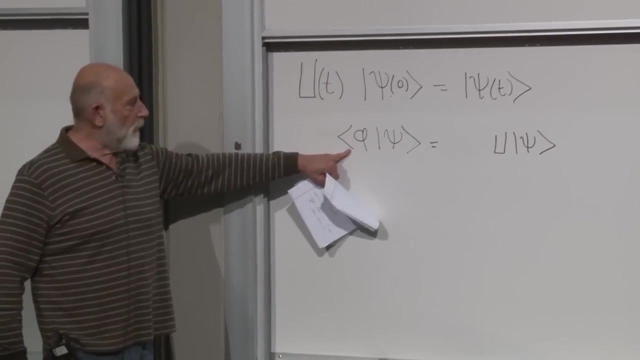 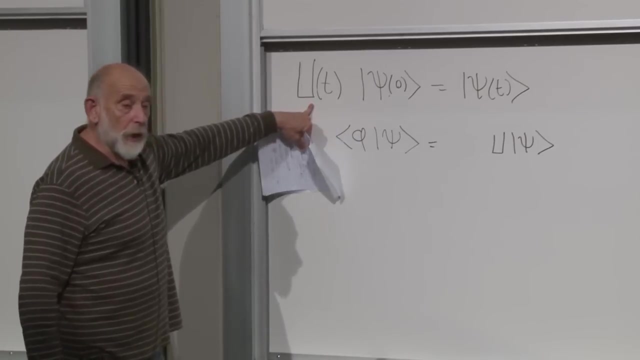 If they're not orthogonal, it is whatever, it is okay- Then the postulate is that if we transform psi and we transform phi- now, phi is a bra vector and it transforms with the Hermitian Comjugate of u. 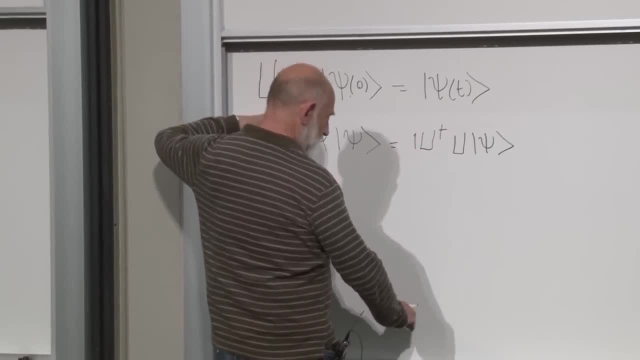 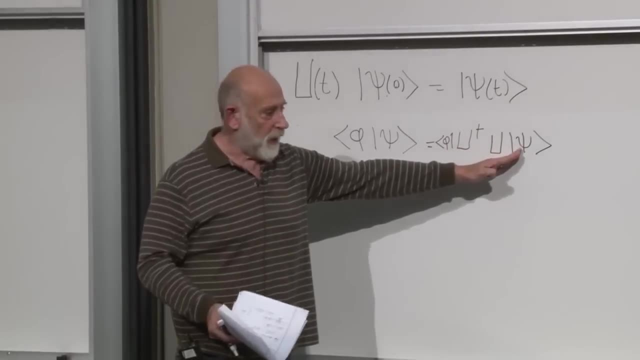 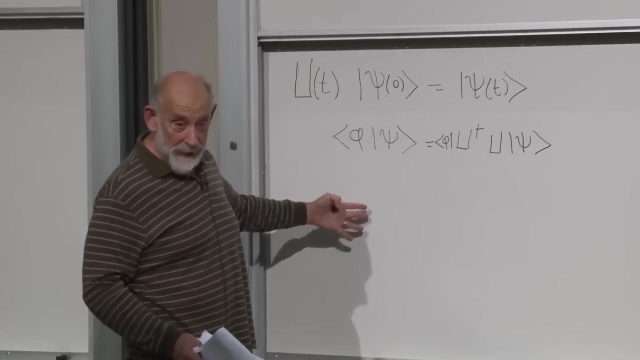 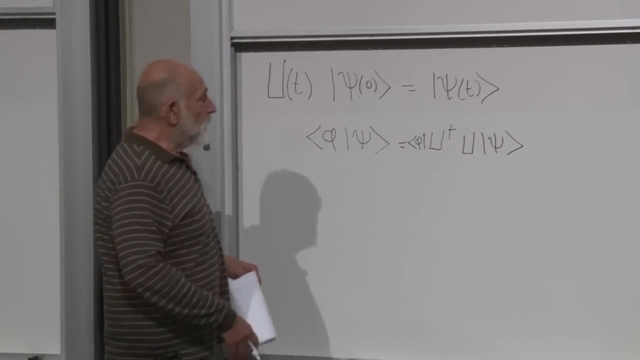 That would be u dagger so phi. What this equation says is that the transform of psi, when you take its inner product with the, is the same as the inner product of Psi with Phi. in the beginning It says that the inner products between vectors don't change with time. okay, 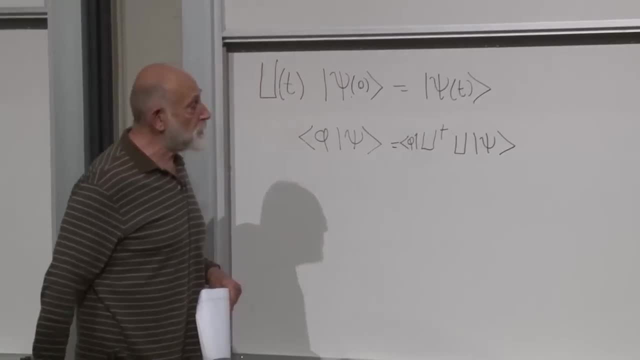 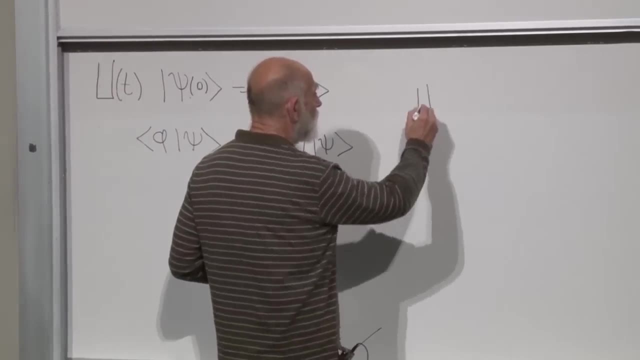 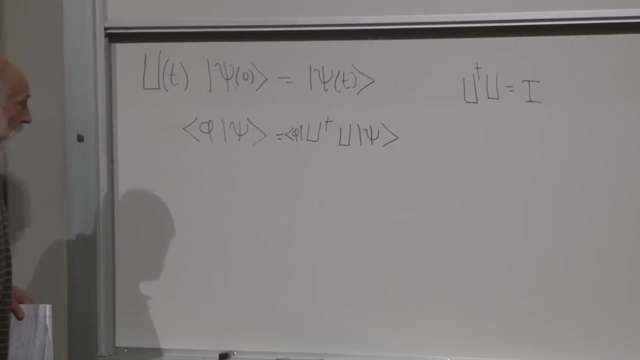 That can only be true for arbitrary pair of Psi and Phi. if U dagger times U is the unit operator And that's called a unitary operator, U dagger times U is the unit operator or the identity operator or just one. That's the notion of a unitary operator and the time evolution. 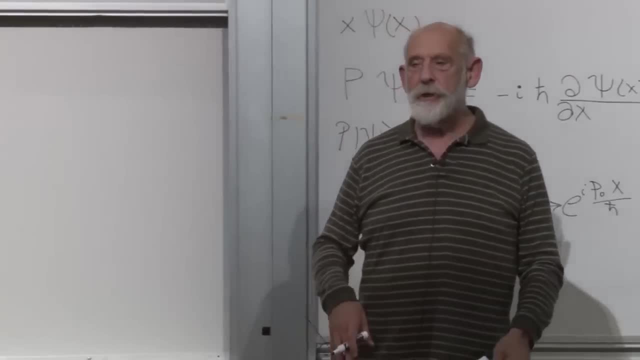 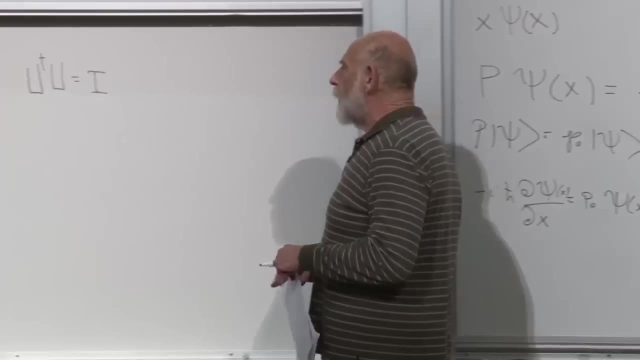 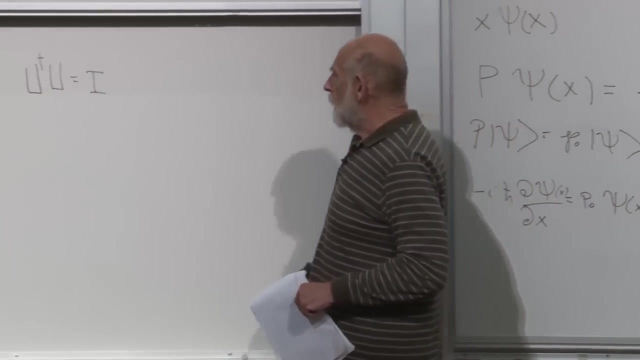 In fact, all transformations, all interesting transformations that you do on the space of states- and we're going to talk about others besides time evolution, all interesting transformations. ways of transforming vectors into other vectors are unitary. U, dagger, U is equal to one. 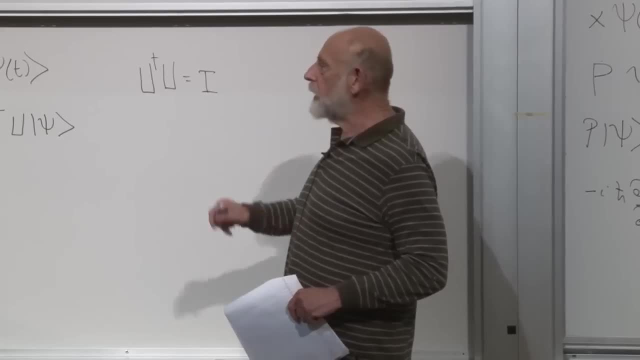 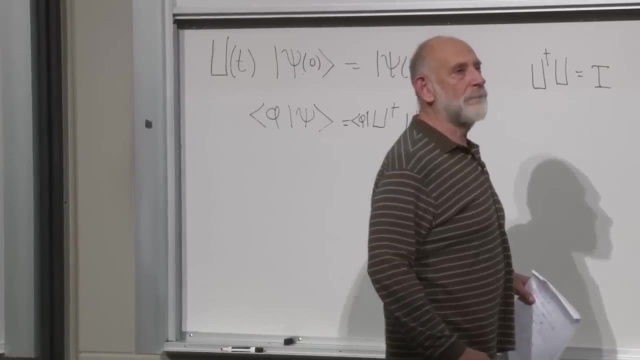 That's different than saying U is equal to one. of course U is a unitary operator. All right, Let's, uh, let's, pursue it. Yeah, Question, Yeah, The way you first said it is, if Psi and Phi were orthogonal, they would remain orthogonal. 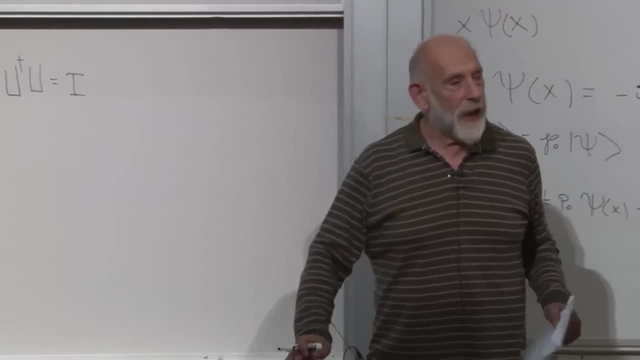 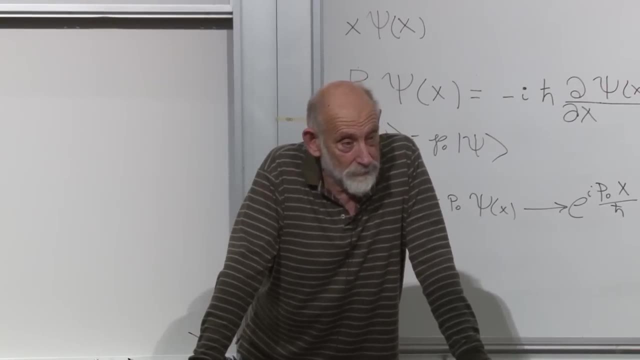 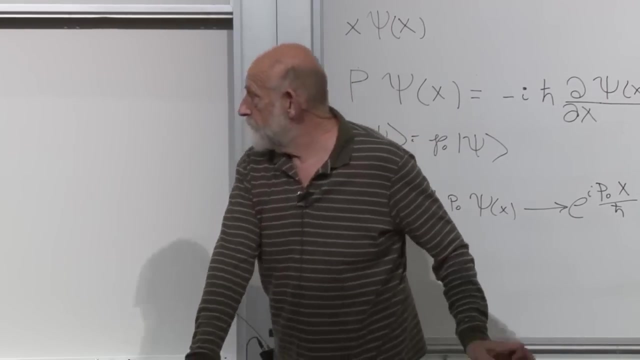 but this is a stronger statement than that This is Actually. it's not. You can prove that if U is a linear operator and it maintains orthogonality, then you can prove that it maintains all inner products. But this is the time: evolution of two state or two systems with different states. 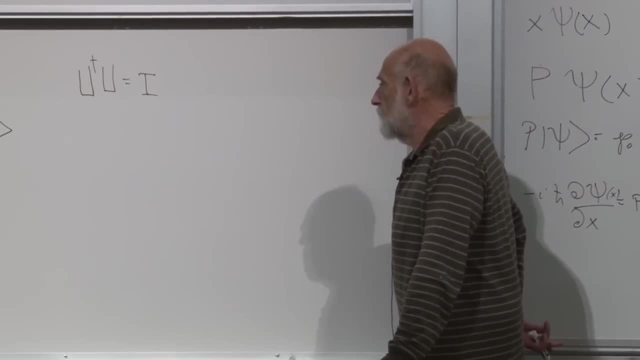 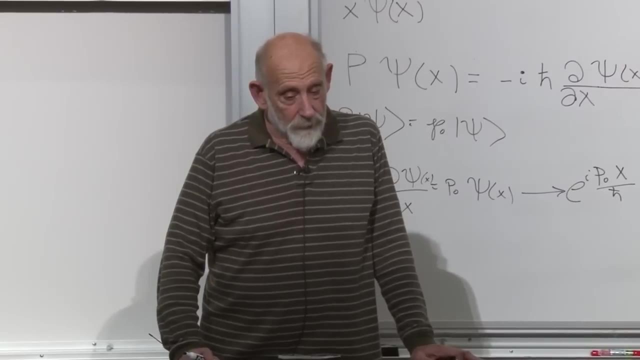 Even if they're not orthogonal, the overlap is conserved, or whatever. That's right. That's right And I said that's. that's what you're saying is correct, But I would say it follows from the If orthogonality is preserved with time. 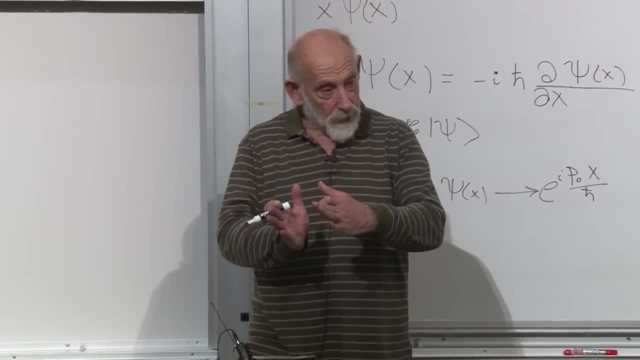 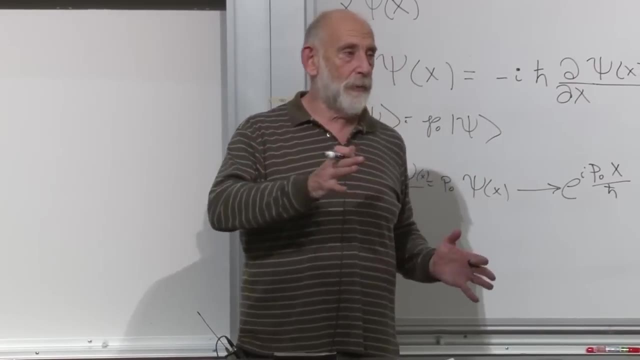 then it's possible to prove that inner products are preserved with time. That's a little exercise. First of all, think about it in just ordinary three-dimensional space. Supposing you have some operation on vectors, ordinary vectors, which preserves orthogonality. 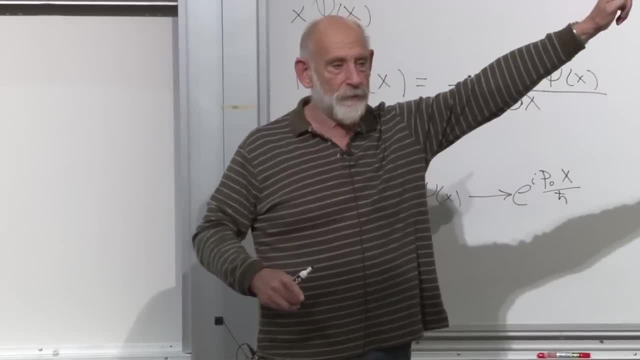 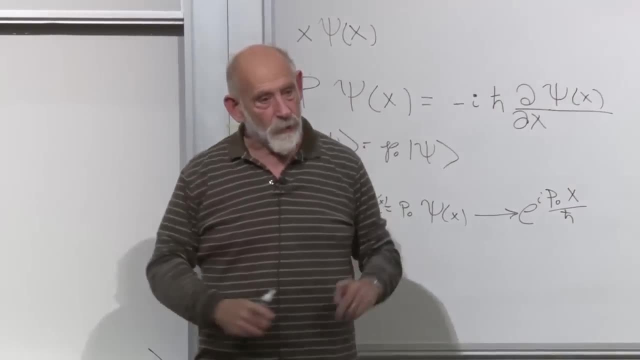 Okay, What kind of operations operators are they Okay? What kind of operations operators on pairs of vectors will preserve the fact that they're orthogonal. Rotations, Rotations, right Rotations- also have the property that they preserve the inner products or the dot products. 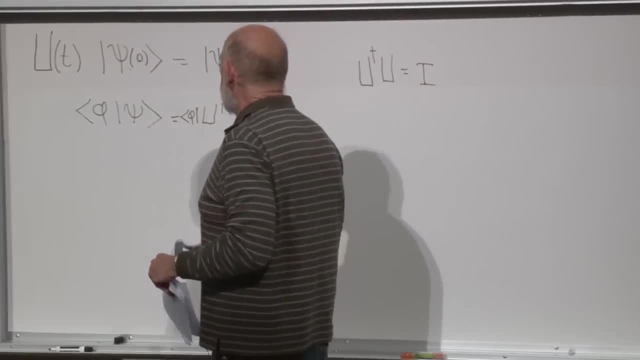 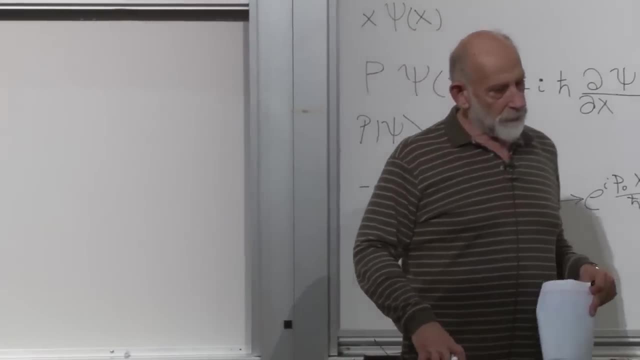 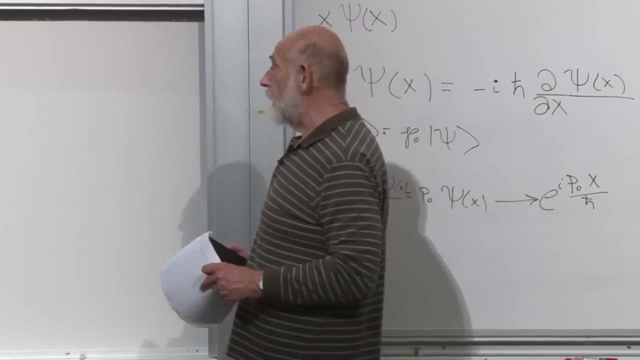 It's the same mathematics. It's the same mathematics. So this is the definition of a unitary operator. There are many unitary operators, So there are many possible. There are multiple things that could represent the evolution of a system, but they're all unitary. 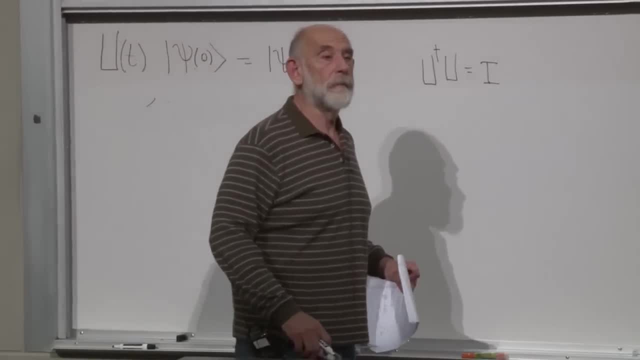 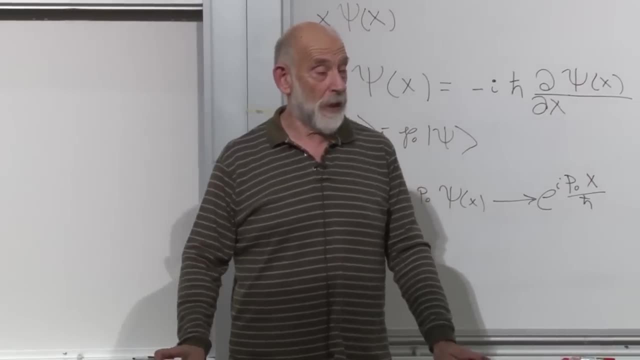 Okay, let's Excuse me. What would be an example of non-unitary transformation? Oh, Our mission. operators are usually not unitary, except that the momentum is not a unitary operator. The position is not a unitary operator. 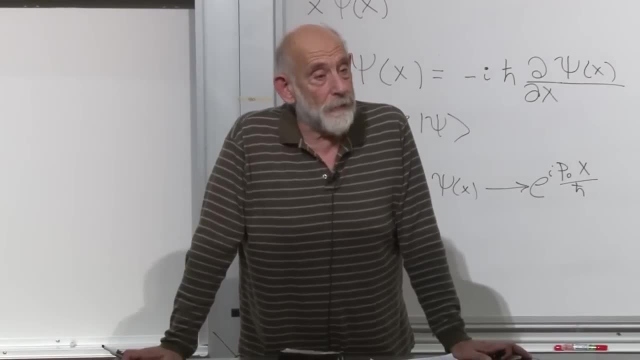 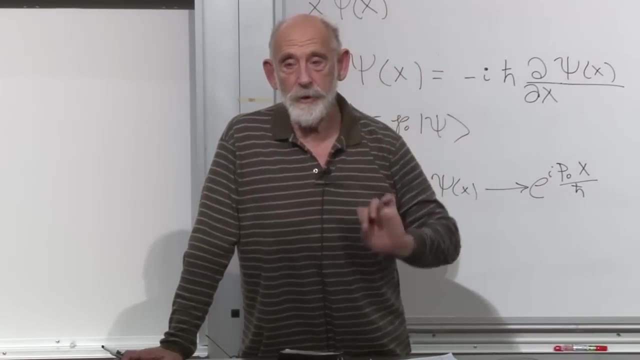 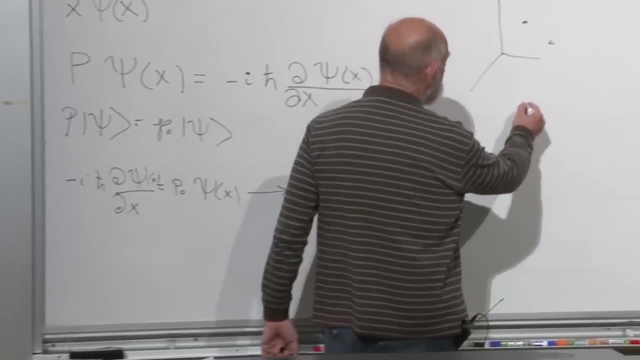 Okay. unitary operators are operators whose eigenvalues are Phases. Everybody know what a phase means. An e to the i times a real number, A point on the unit circle. A phase represents, on the complex plane, a point on the unit circle. 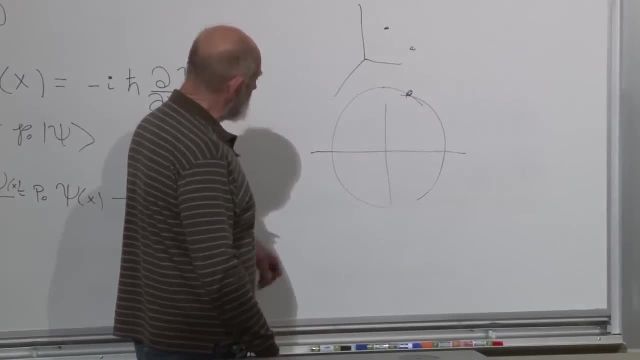 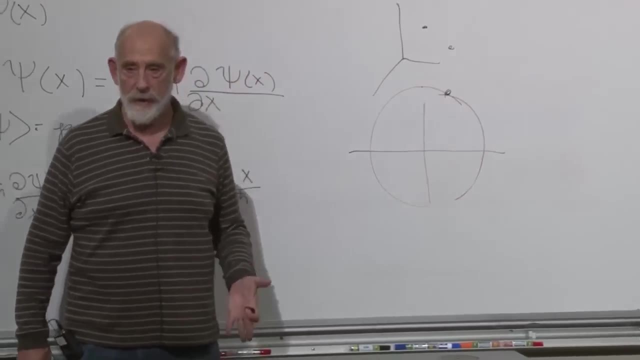 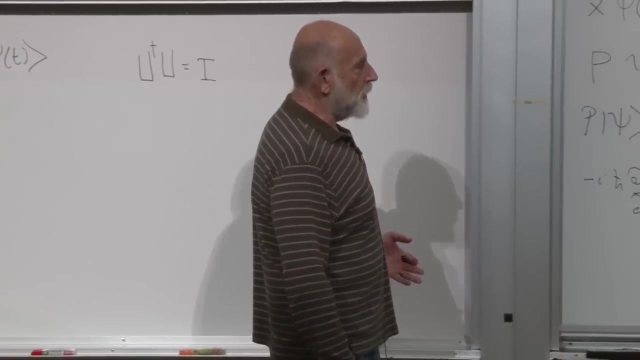 1 is a point on the unit circle. i is a point on the unit circle Minus 1 and minus i. 1 over the square root of 2 times 1 plus i is a phase. The Unitary operators are the analogs for operators of phases. 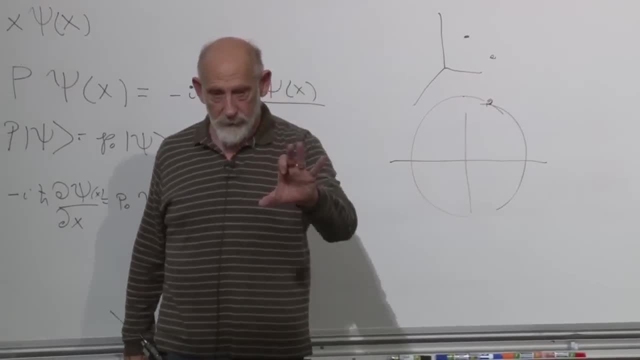 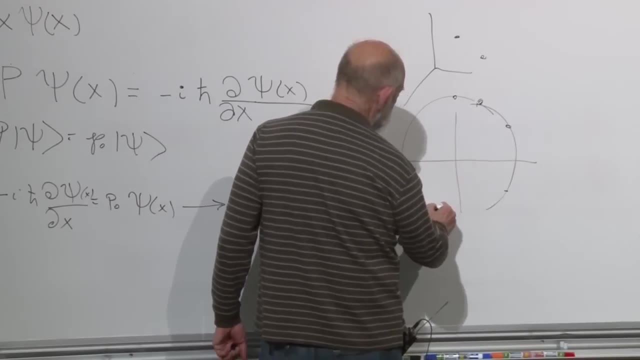 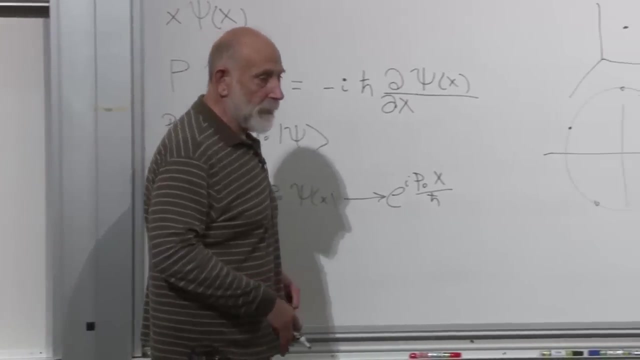 Their eigenvalues are all phases, So if I have a unitary operator and I look at its eigenvalues, they will be points sprinkled around on the unit circle. That's why they're called unitary, because in some sense their length or their 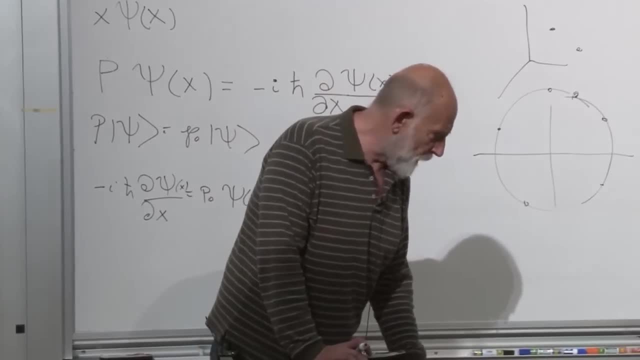 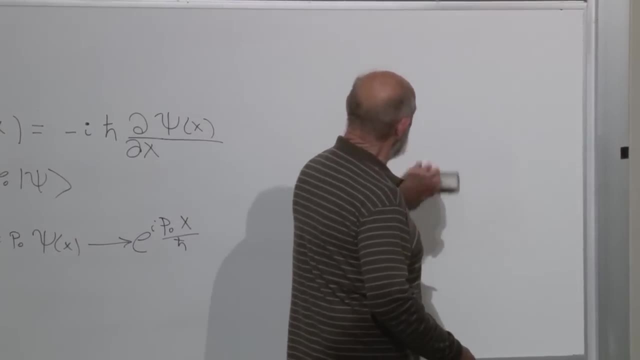 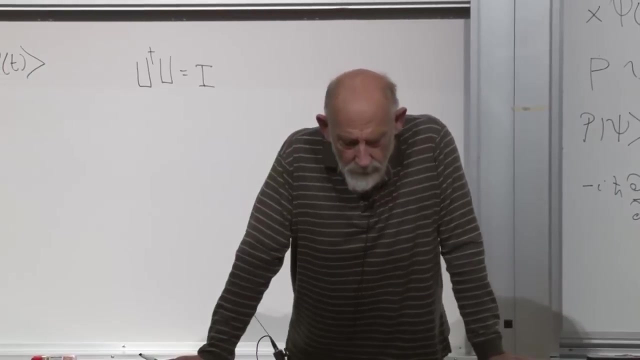 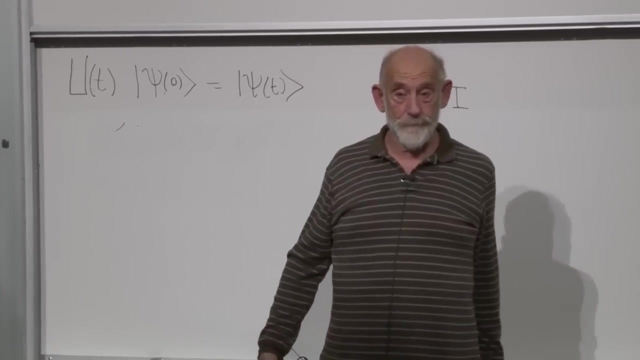 The magnitude of their eigenvalues is unit. Okay, now let's Let's see what more we can learn about u from making some reasonable assumptions. The first reasonable assumption is that if t is equal to 0, then u is just equal to 1.. 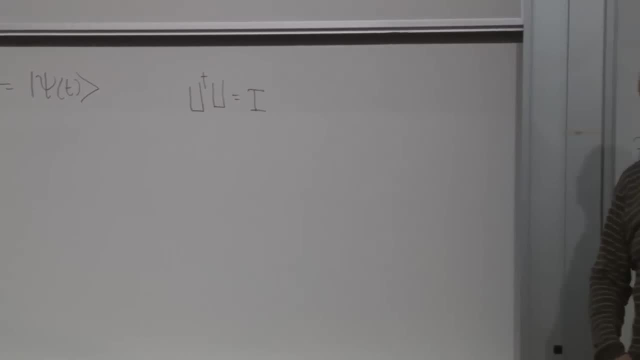 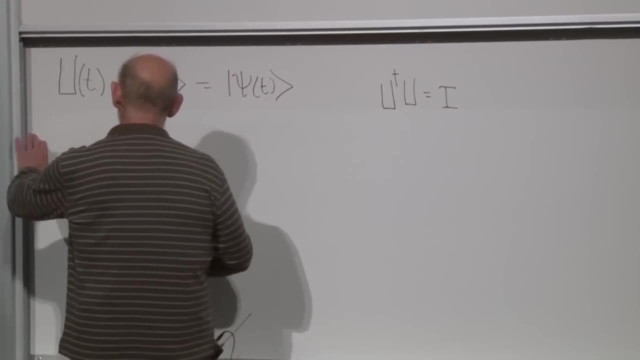 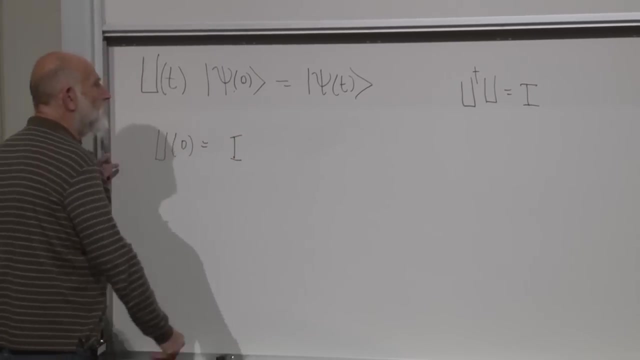 All it says is that if you don't allow any time to elapse, the vector just comes back to itself and u is equal to To the unit operator. So u of 0 is equal to i, the identity operator, the operator whose matrix representation is just 1.. 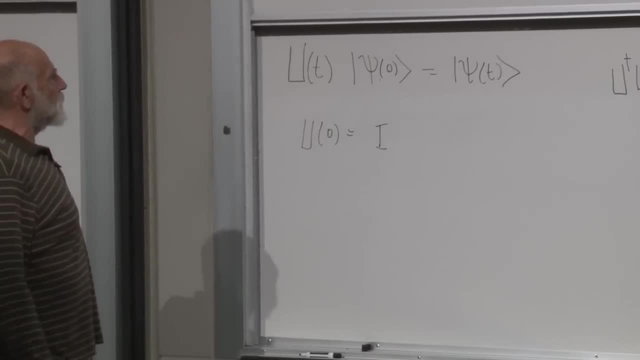 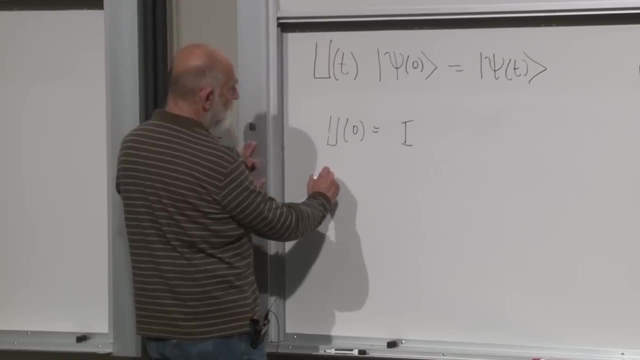 1 along the diagonals. It's just the operator which does nothing. It just takes the thing back to itself. Now is u unitary Sure. it is The Hermitian conjugate of u is the Hermitian conjugate of the identity operator. 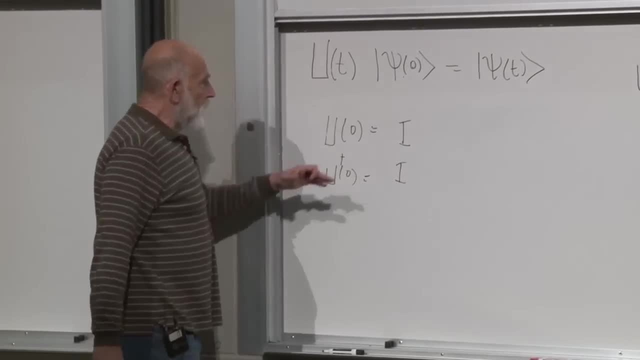 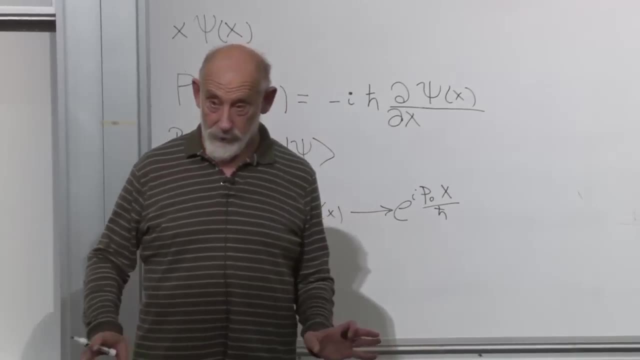 which is just the identity operator, which is the unit operator itself, And identity, times, identity is just identity. So, yes, 1 is 1 or the unit operator is unitary And it's. It's the time evolution, when no evolution happens. 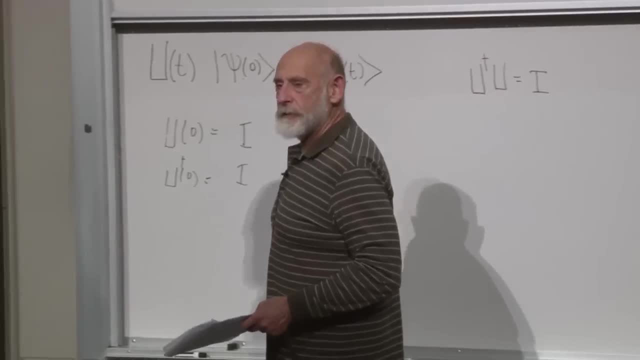 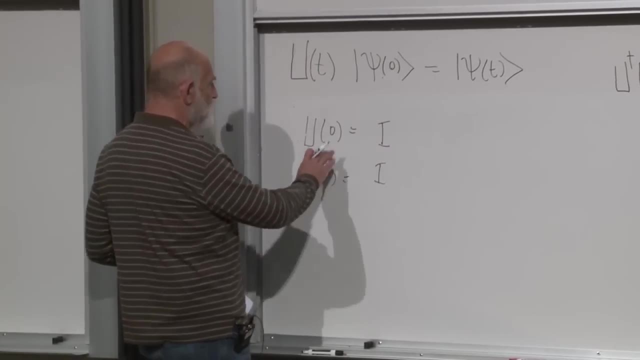 Okay, what about evolution by a very, very small amount of time? Okay, So let's, Instead of writing u of 0, let's, write u of epsilon. Take u of 0 and write u of epsilon. Take u of 0 and write u of epsilon. 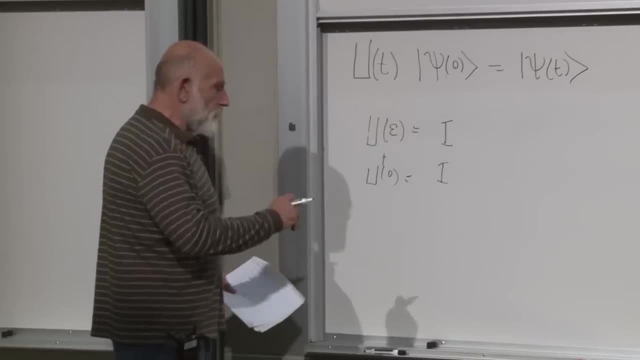 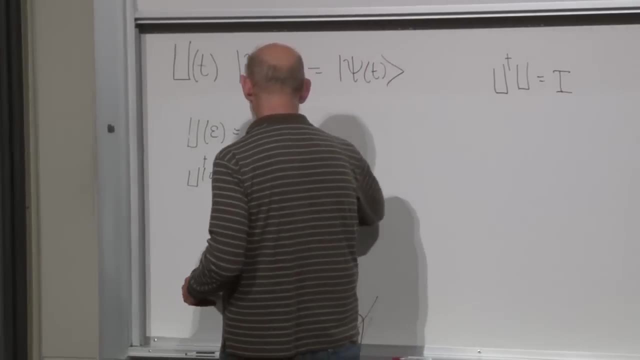 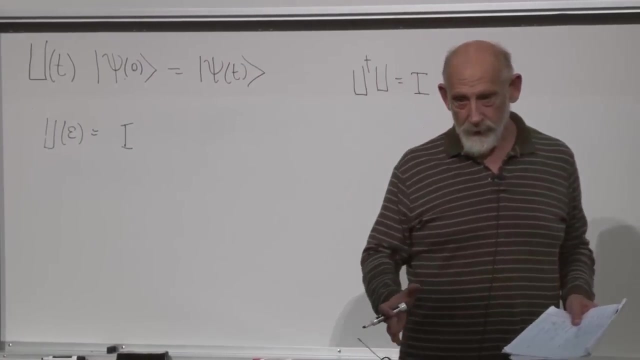 Take u of epsilon, It is not 1.. Something happens over time, evolution, But it is close to 1.. It's close to 1.. That, of course, is an assumption. That's the assumption that systems evolve continuously, That they don't make radical jumps over very, very short periods of time. 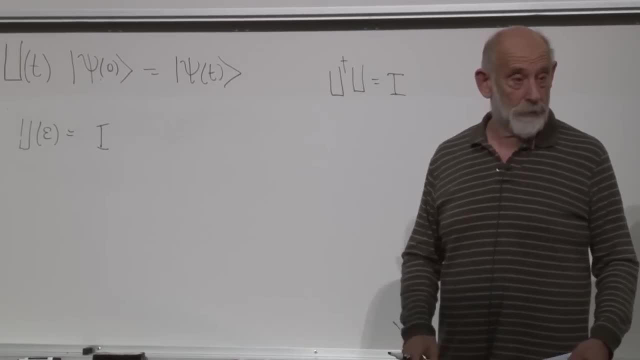 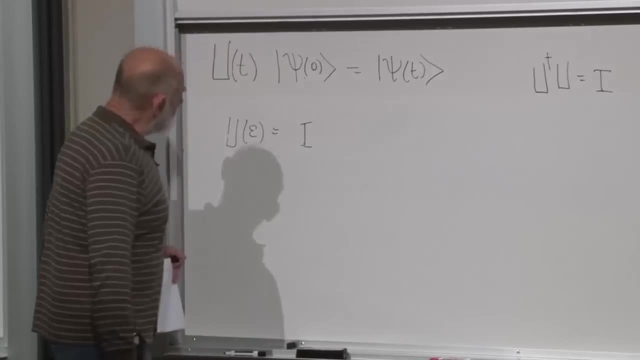 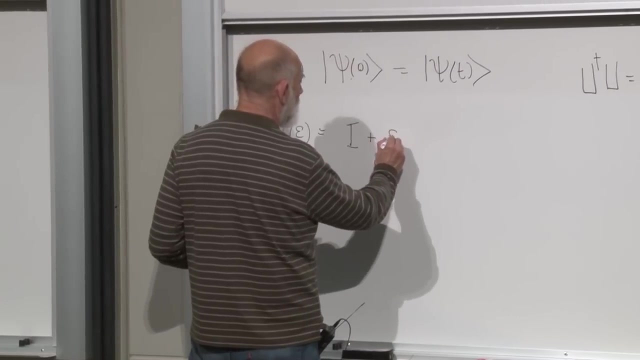 And it is an assumption. It's an assumption, ultimately, which is justified by experiment. All right, So that says that u of a small time epsilon. if we were to expand it in, small epsilon would be 1 plus something proportional to epsilon. 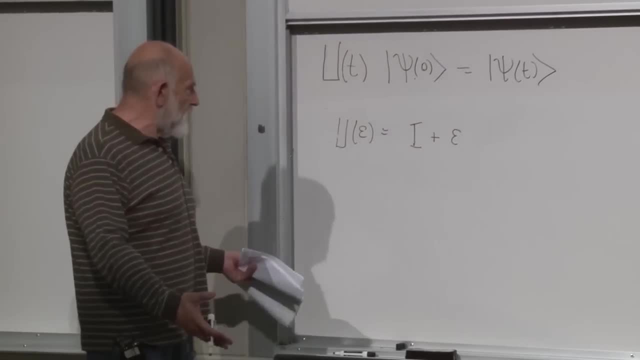 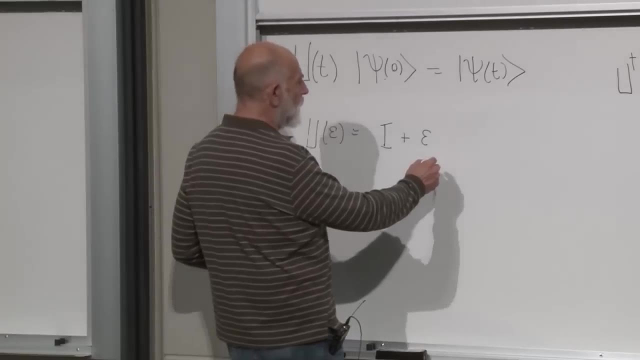 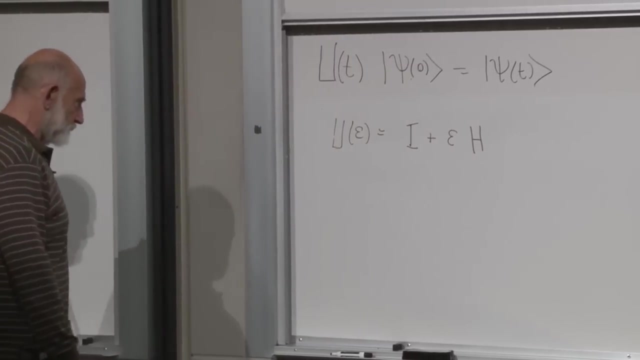 times an operator which is a finite operator. The smallness of epsilon is represented by epsilon here times something which I'll temporarily call h, but it's a wrong identification. In a minute we're going to change it. Okay, Let me not call it h. 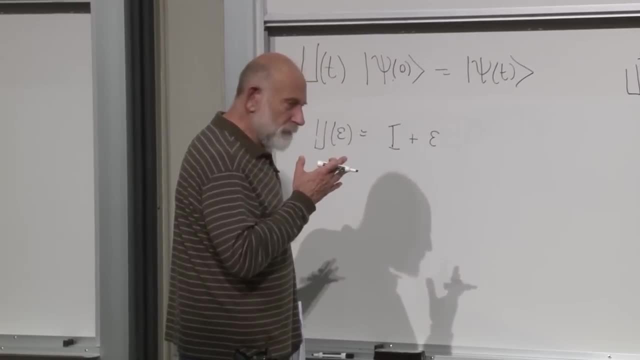 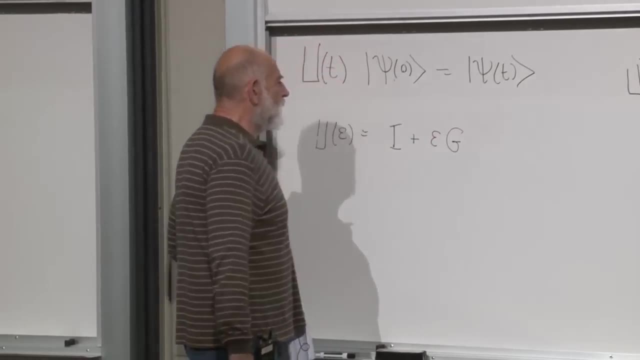 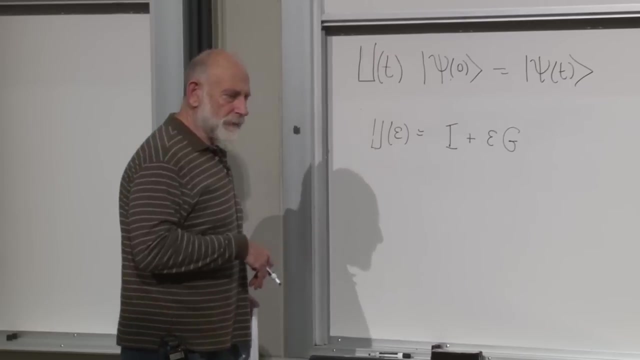 What's another letter? Give me another letter, Quick, quick, fg. No, no, no, no, no. g, g, fgh, Yeah, g, Good, All right, So u is of this form. There's nothing wrong with this. 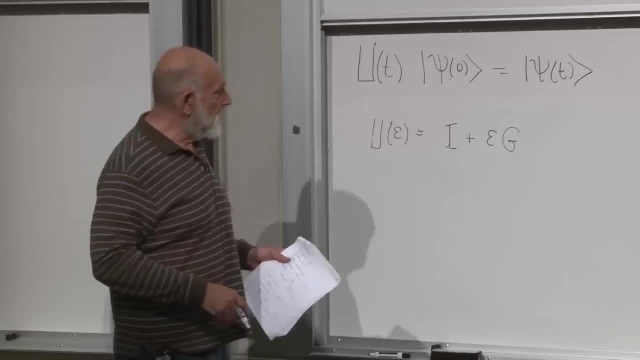 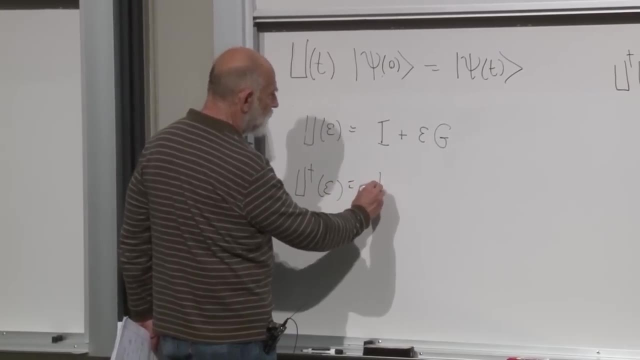 This is a correct thing. The question is, what do we know about g? So let's write down u conjugate, permission conjugate of epsilon. That's equal to 1 plus epsilon times g conjugate, the permission conjugate of g. 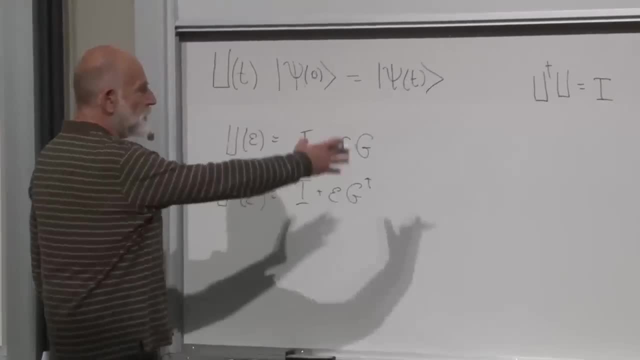 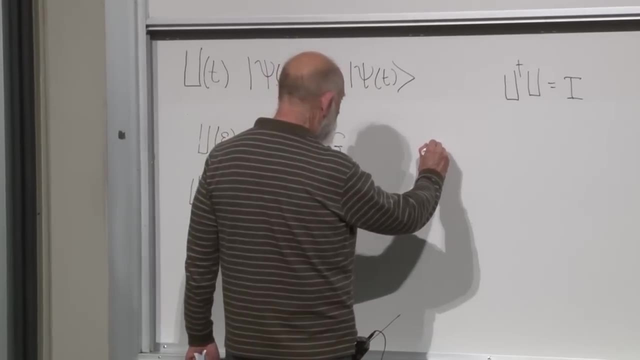 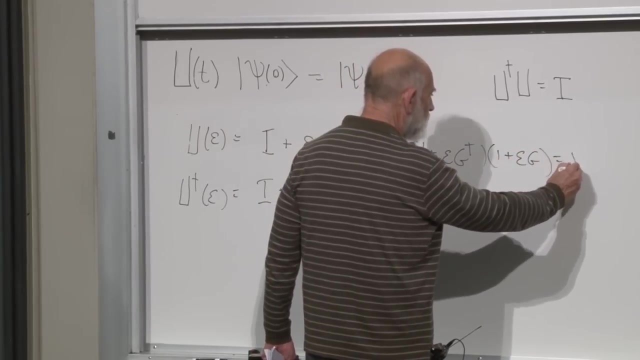 And now let's multiply these together and insist that the answer to leading order in epsilon is just 1.. Okay, So that will say that 1 plus epsilon g- dagger times 1 plus epsilon g- is equal to 1.. Looks a little queer. 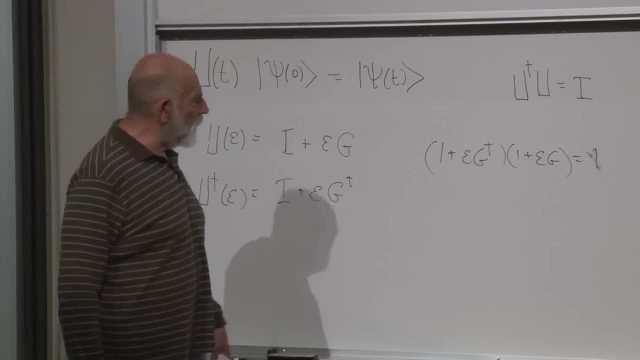 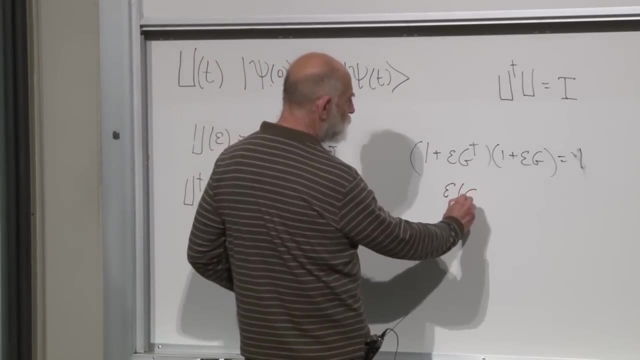 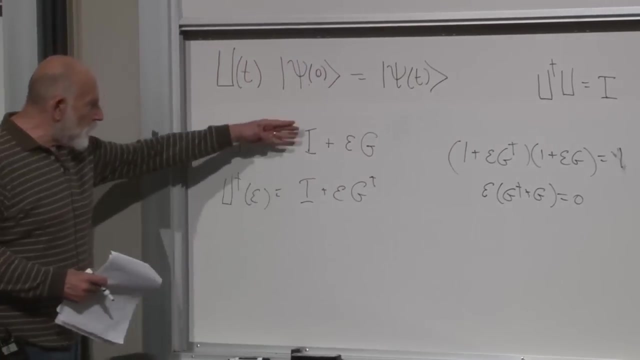 1 times 1 is 1.. So what's left over? What's left over is epsilon times g, dagger plus g, And that must be 0.. To order epsilon working. to order epsilon, the condition that u is unitary is the condition that g. 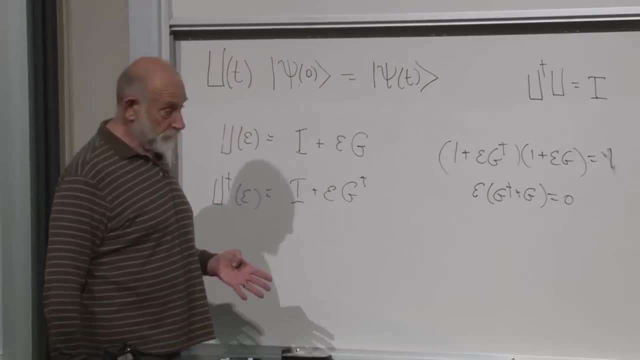 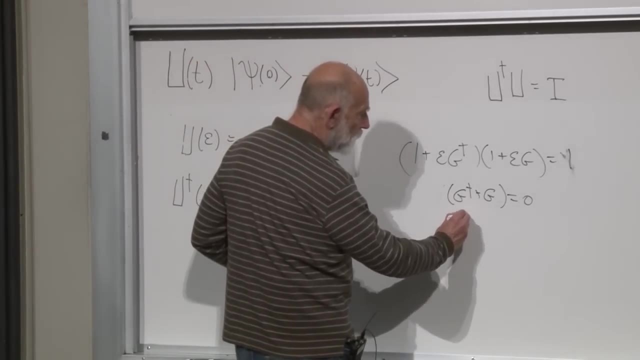 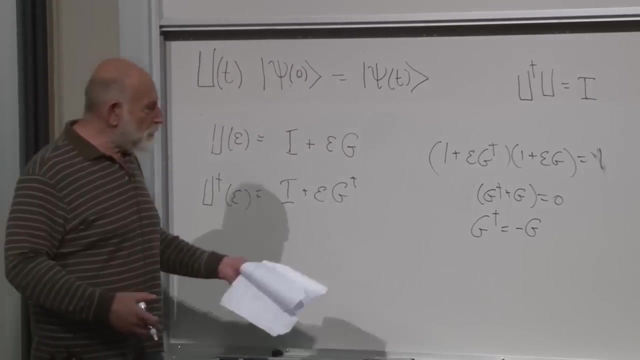 plus its own permission, conjugate is equal to 0. In other words, getting rid of the epsilon that the conjugate of g is equal to minus g itself. Operators with this peculiar property. do you know numbers that have that property? Do you know any number that has the property? 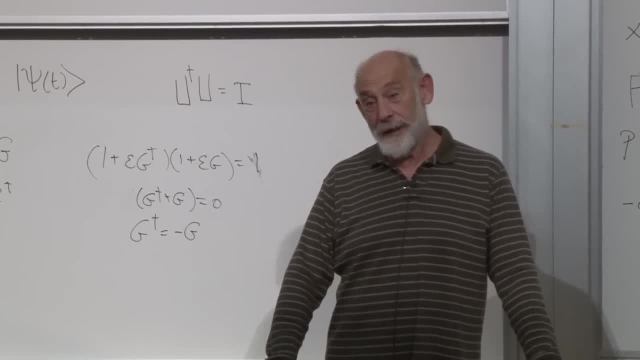 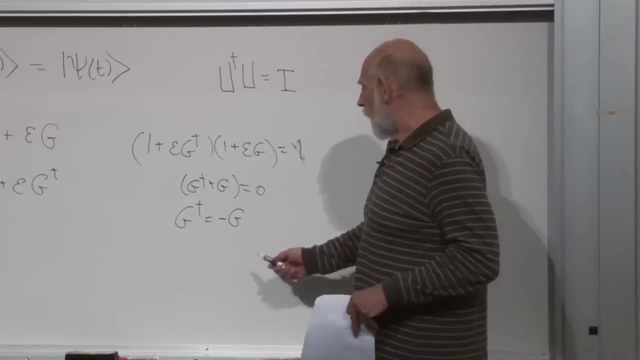 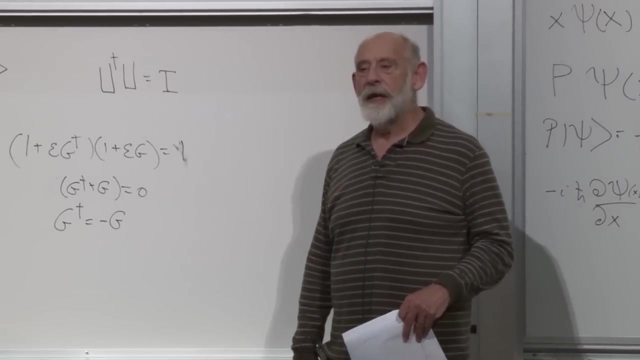 that it's minus its own complex conjugate, It is true, but there's a wider class of them, Pure imaginary things. So this is the analog of g being pure imaginary. If we multiply it by i, it becomes hermission. This is called anti-hermission. 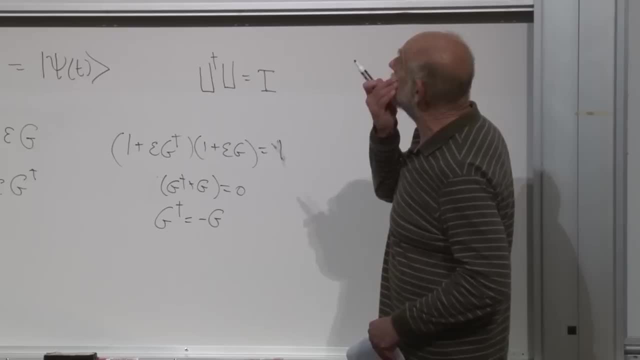 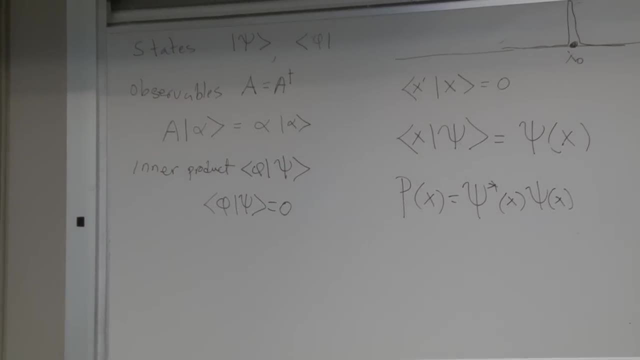 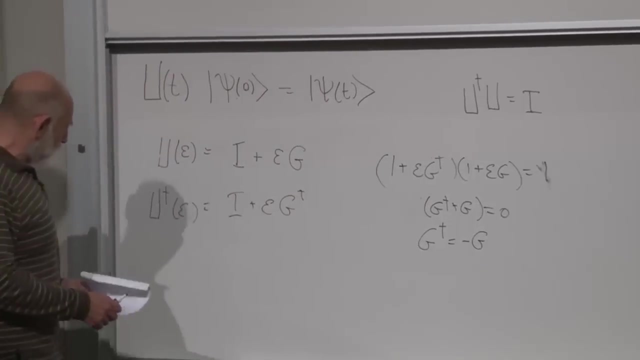 Hermission is when g dagger equals g. Did we write that someplace? Yeah, a equals a dagger is an observable. g dagger equals minus g. We can fix that very simply. Just define g dagger to be now. do I want plus or minus? 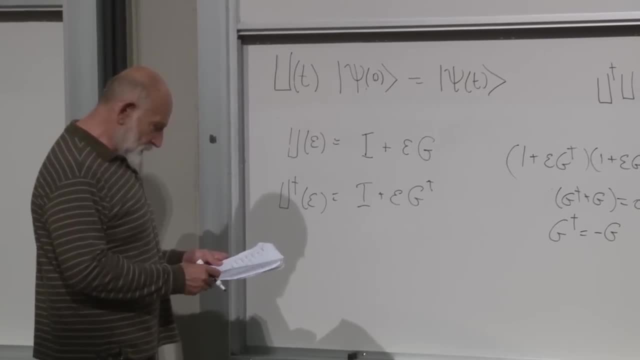 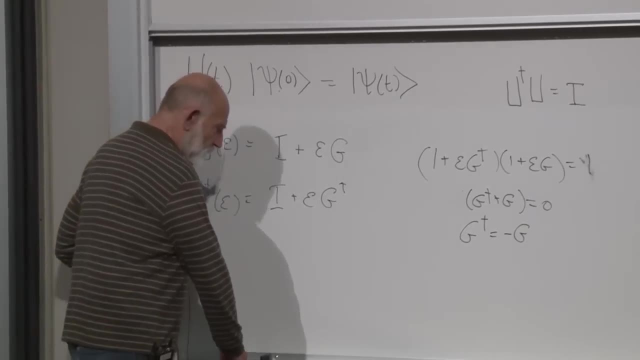 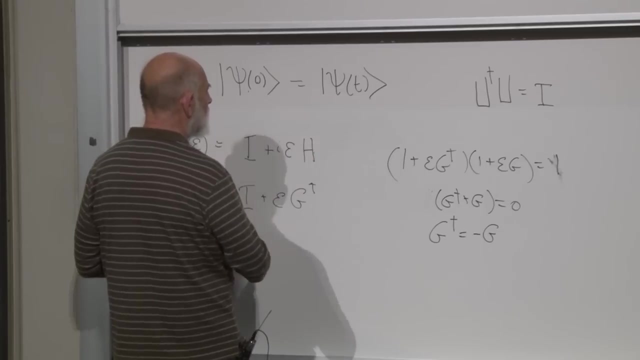 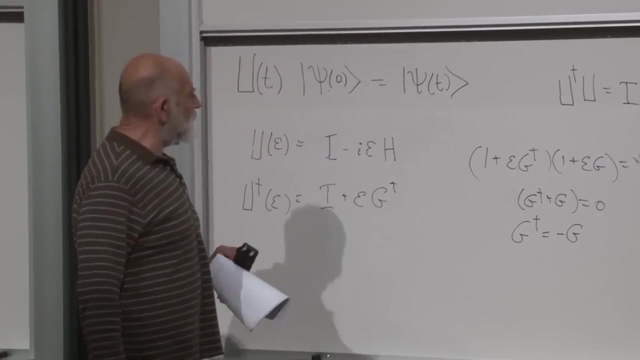 I always forget. It always takes me a minute or two to. I want to write 1 plus i, epsilon h, But I think the right answer is minus. That's a. whether you put a plus sign or a minus sign, here is a convention. 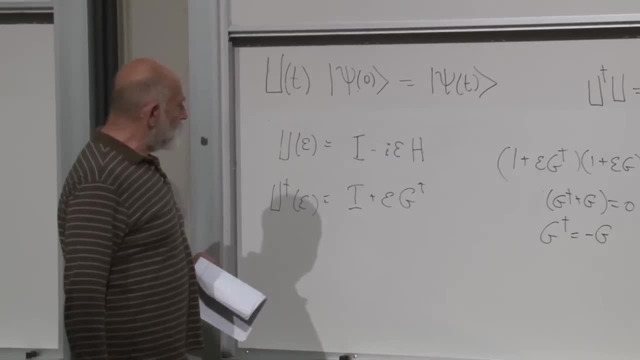 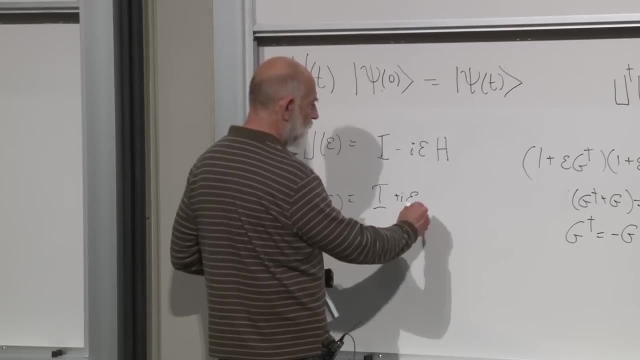 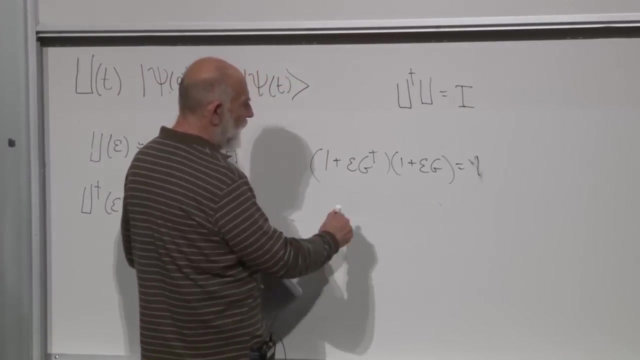 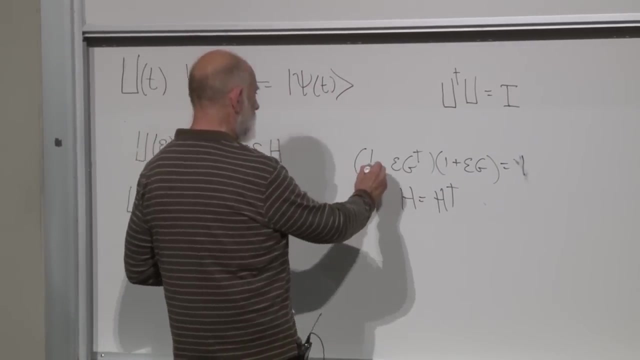 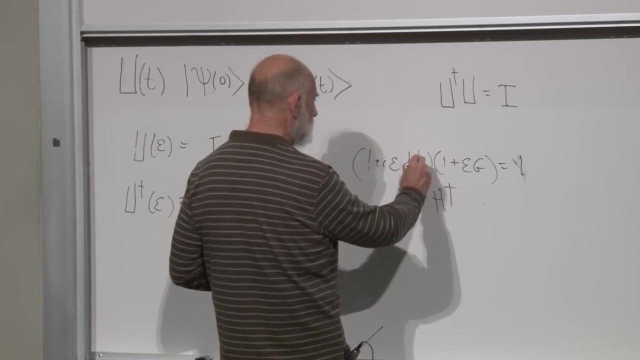 complete convention. It defines h. This one becomes 1 plus i epsilon h h dagger, And the condition just becomes that h equals h dagger. In other words, if I put a minus i epsilon h, no plus i epsilon h dagger. 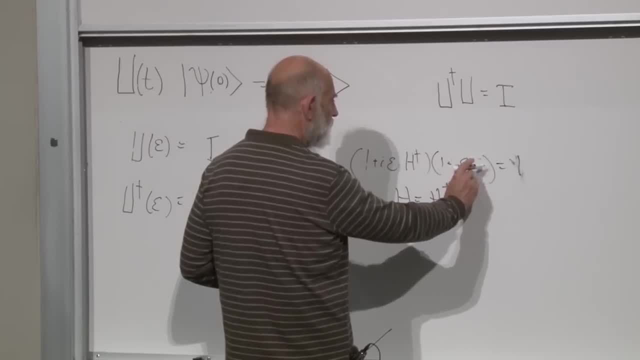 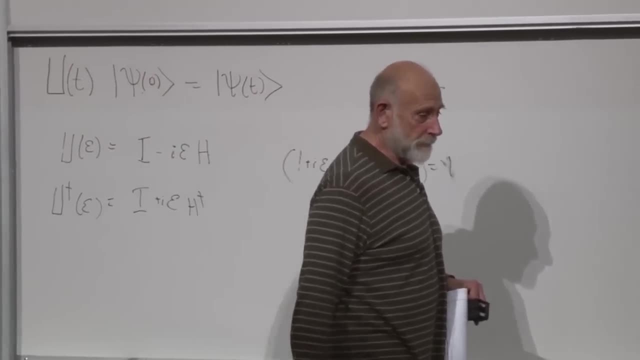 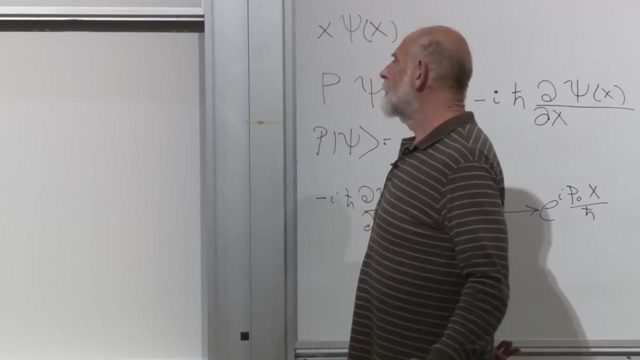 minus i epsilon h, then the condition that u is unitary is just the condition that h is hermission, In other words, that h is an observable. Yeah, What assumption are we making that allows us to ignore the epsilon squared term? We're just working to order epsilon. 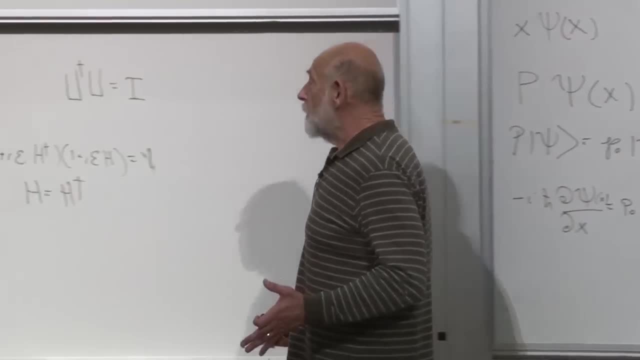 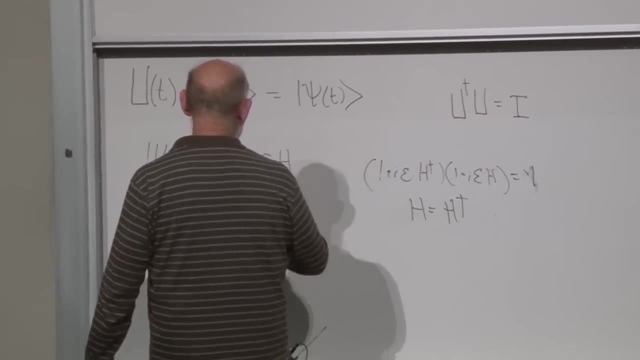 We could work to order epsilon squared, but then we would have to be consistent about it and put an epsilon squared term in here. The epsilon squared term that we would want to put in here would be minus epsilon squared over 2 times h squared. 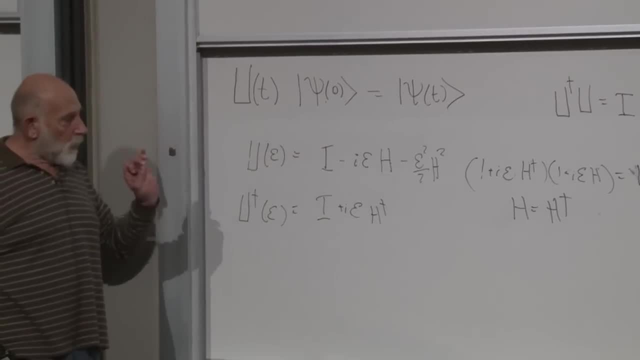 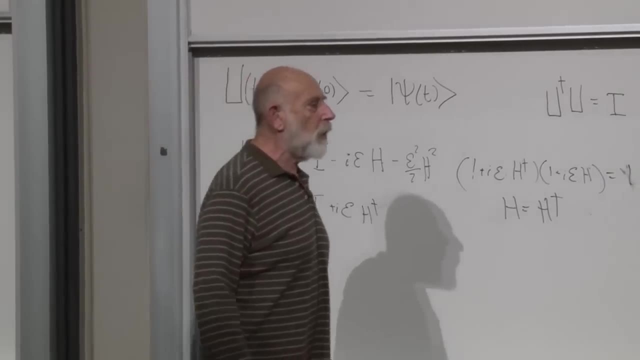 And. but we consistently work to one power in epsilon and assume that epsilon is small enough that we can ignore epsilon squared. We can do that consistently, We've done it over and over and over. But then, you're perfectly right, We do have to come back. 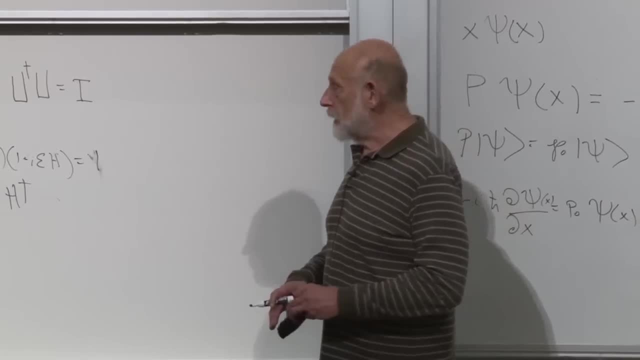 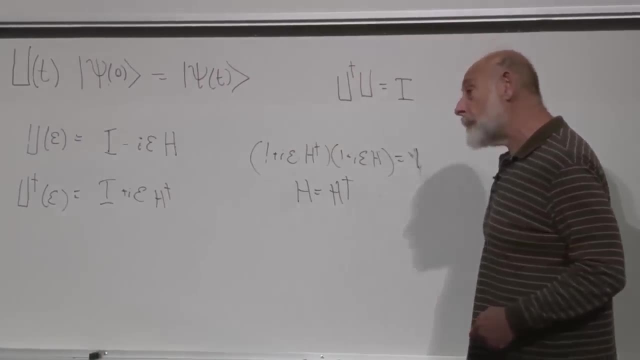 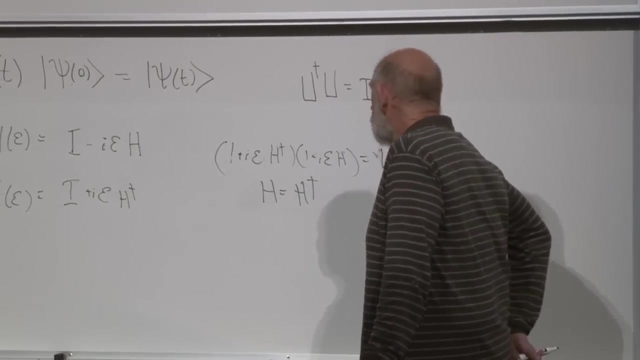 and check that the formulas make sense to higher order, and they do. I'll discuss that a little bit. But working systematically to order epsilon and dropping anything of higher order in epsilon, I just wondered if, what we, if we were following the details of it. 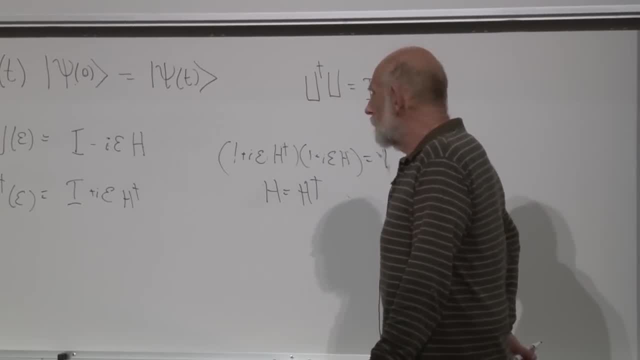 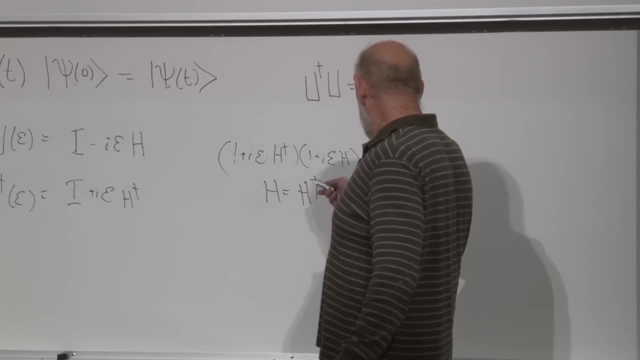 we'd have to say that h is approximately hermission, or something like that: Yes, No, well, okay, With this definition, you would say h is approximately hermission, But allowing notice that epsilon factors out of both sides of this equation. 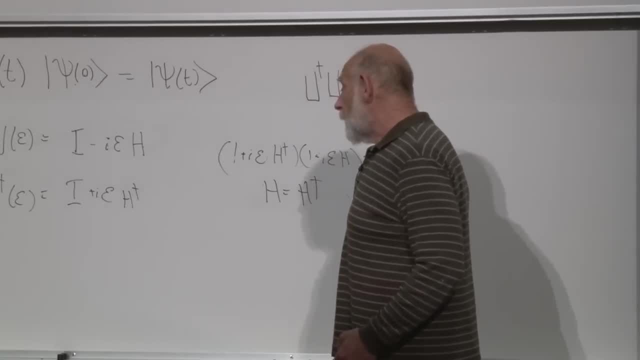 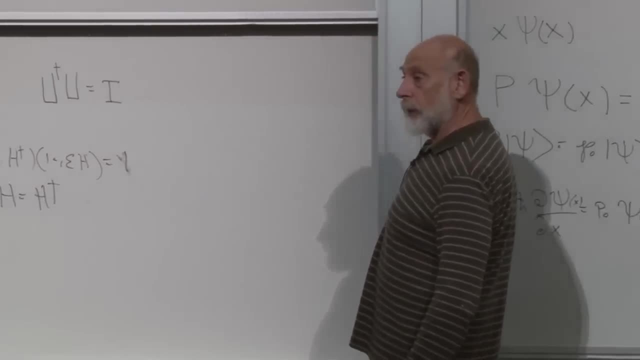 So once it's factored out, it just says that h. no, I think the thing which is approximate is this relationship here. Yeah, And I'll come back and tell you what to do. if it, I'll tell you the right formula. 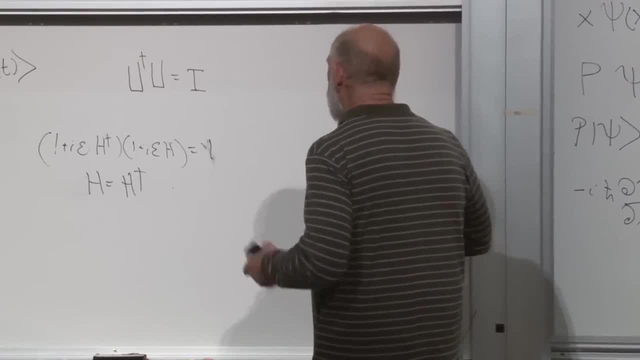 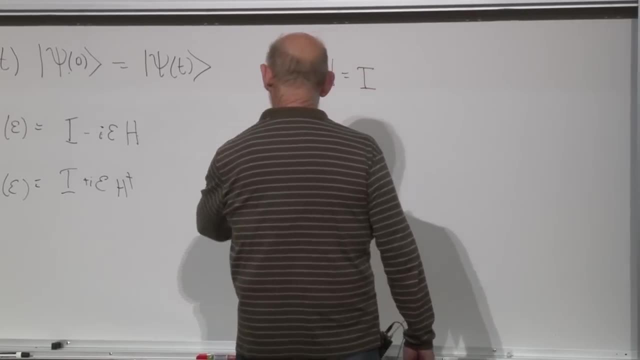 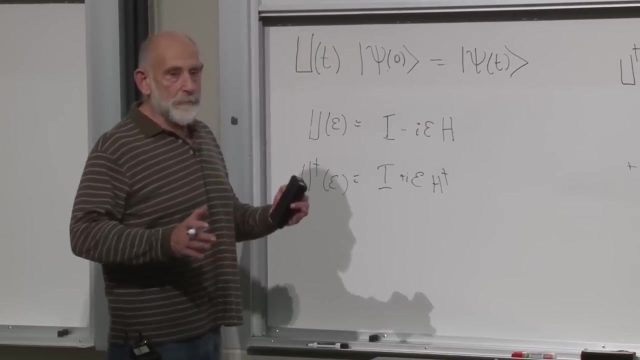 in a little while, at some point. Okay, so what do we learn? We learn that the that the unitary time evolution, which contains a u of t, also is specified in terms of a certain observable that I've called h. h stands for Hamiltonian. 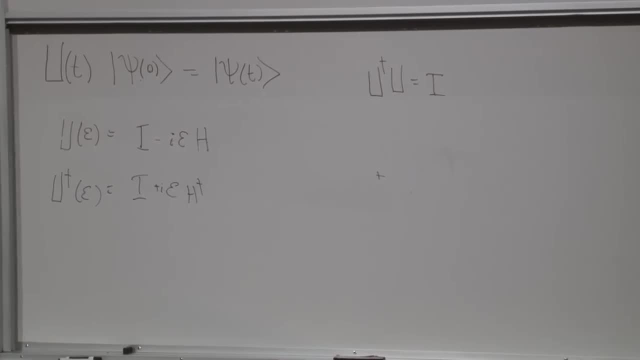 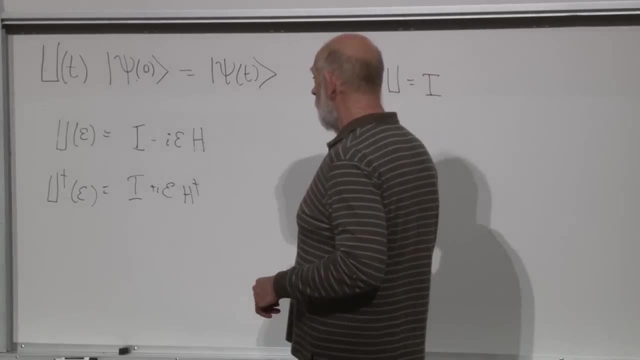 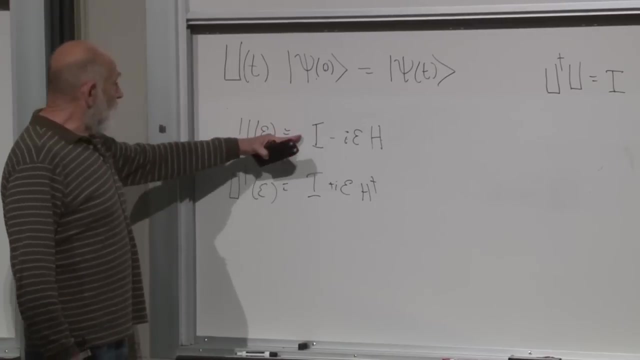 It also stands for hermission, but it stands for Hamiltonian. It is the Hamiltonian of quantum mechanics, And so we come to the conclusion that there exists an h- we will call it the Hamiltonian- and it is related to the time evolution. 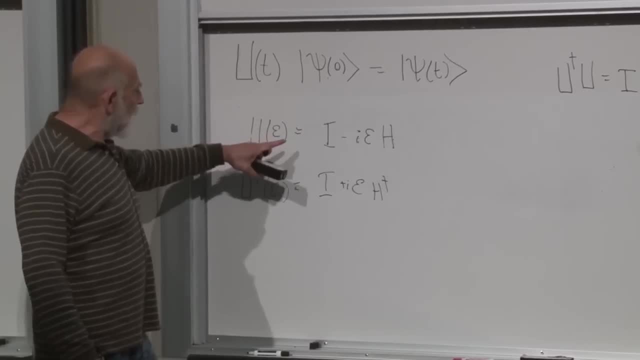 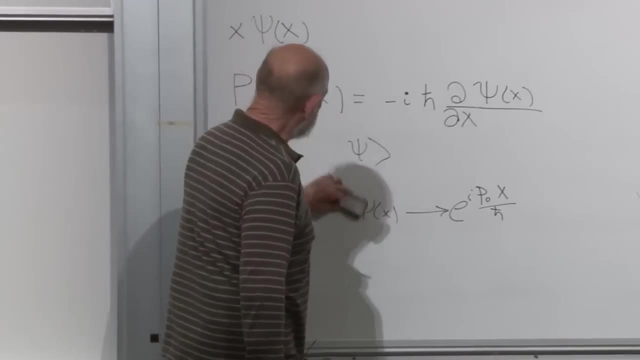 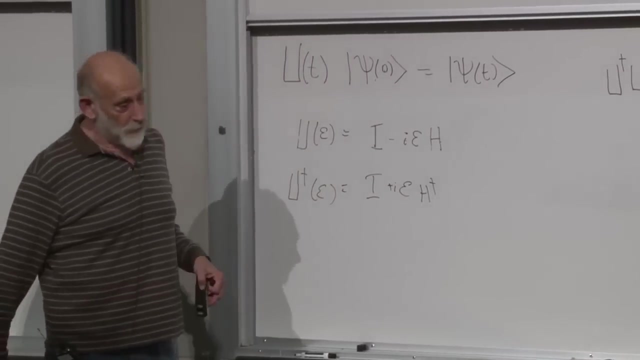 for small time intervals by one minus i, epsilon h. What is the general equation if epsilon is not small? Incidentally, if epsilon is not small, we might want to call it t, We might give up calling it epsilon. Epsilon is usually reserved. 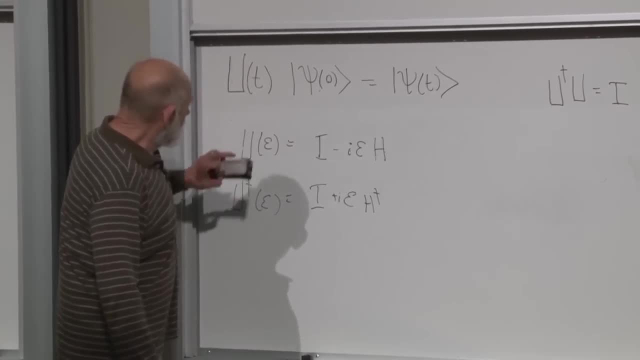 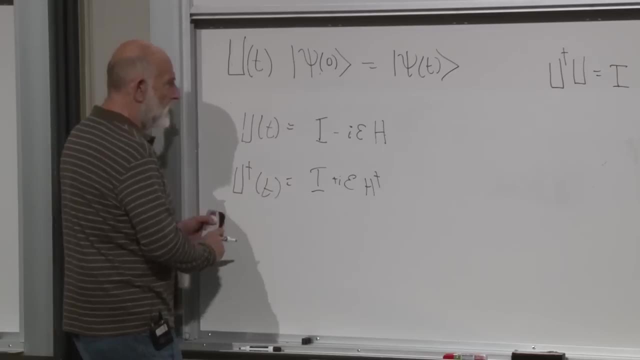 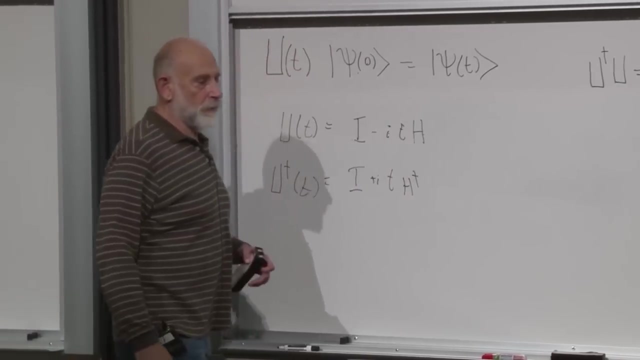 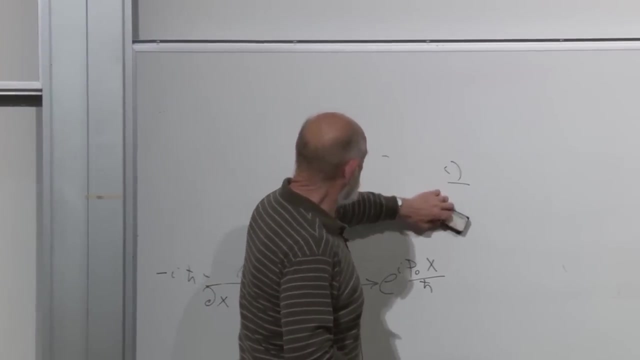 for a very small quantity. We might try writing u of t, but this wouldn't be right for large times. It wouldn't be large for large times. Let's see if we can improve it a little bit. Well, you know, I think I won't spend time at it. 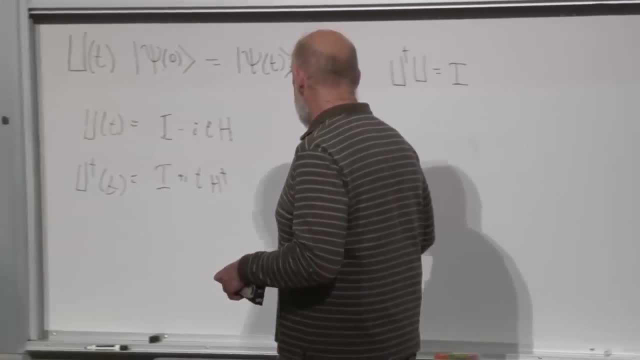 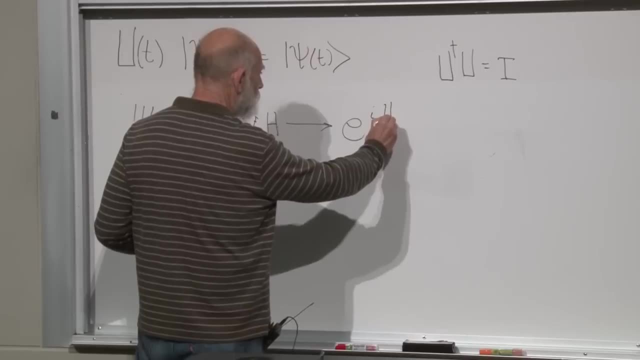 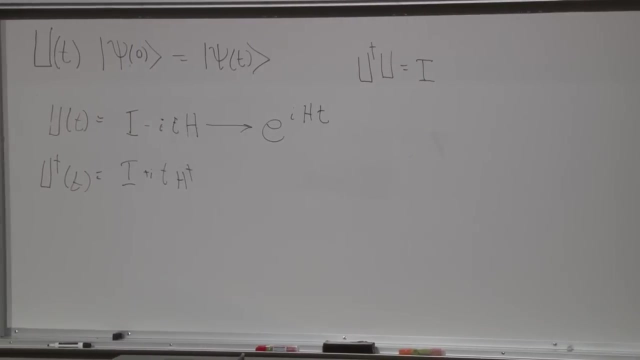 I will just tell you the answer. The answer is that this is really should be written as e to the i, h, t. Now why do I let me? let me just say a word or two about exponentials. If you have an exponential, 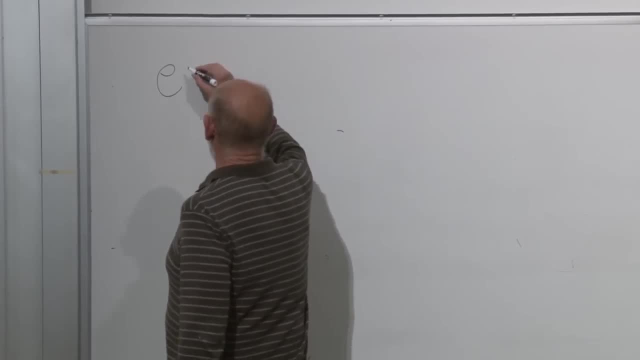 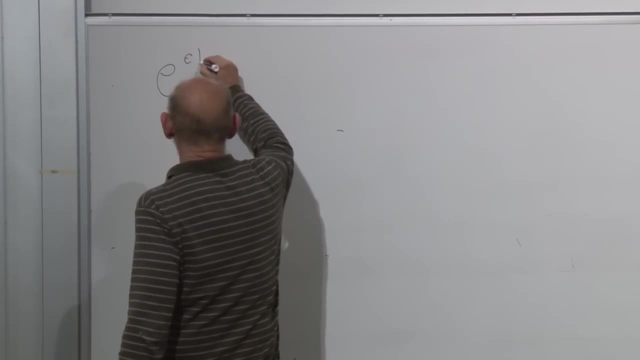 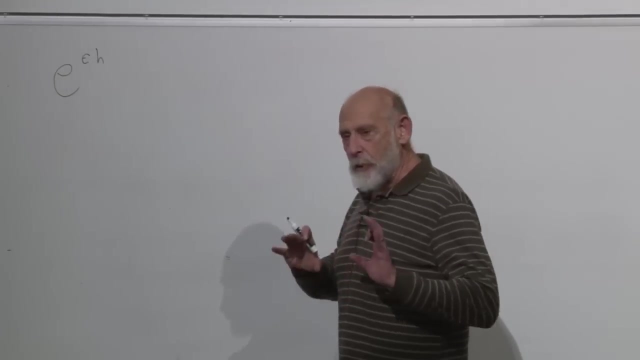 e to some small number and let's just call the small number epsilon, where epsilon is small times an ordinary number. and let me call the ordinary number little h. Epsilon times h is a small number For very small epsilon e to the epsilon h is one plus epsilon h. 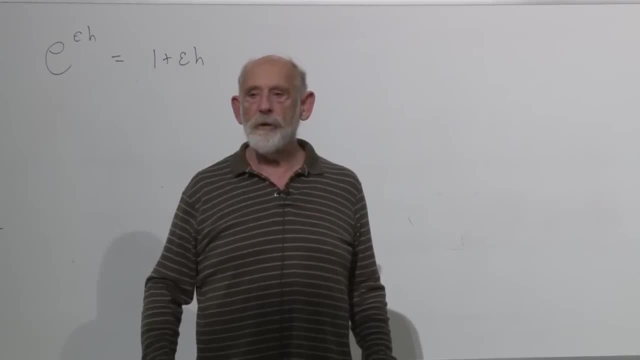 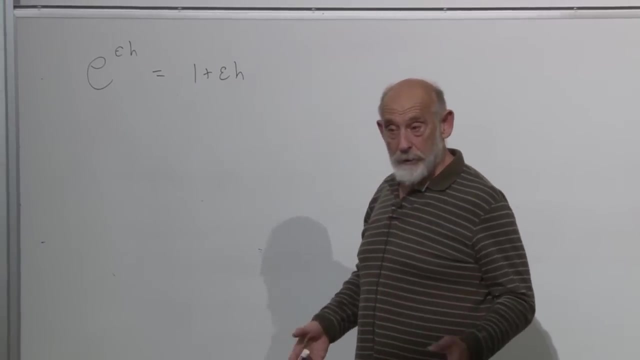 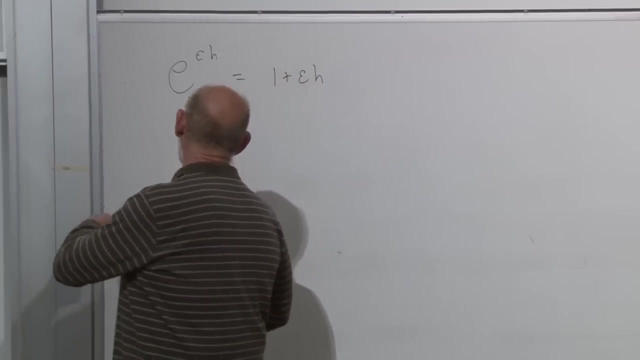 Does everybody know that? That's the formal Taylor series expansion of keeping only the first term, assuming the second term and higher terms are negligible. Okay, Now, supposing you want to take, you want to make epsilon a little bigger Instead of just epsilon? 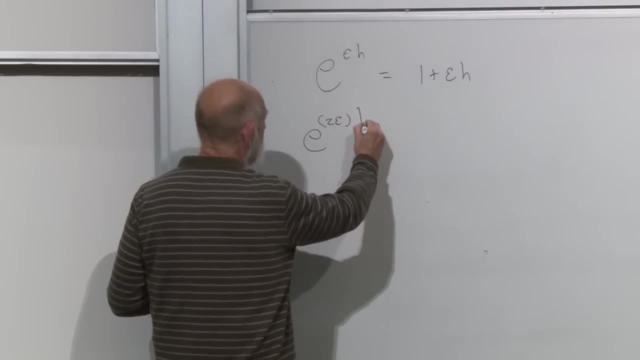 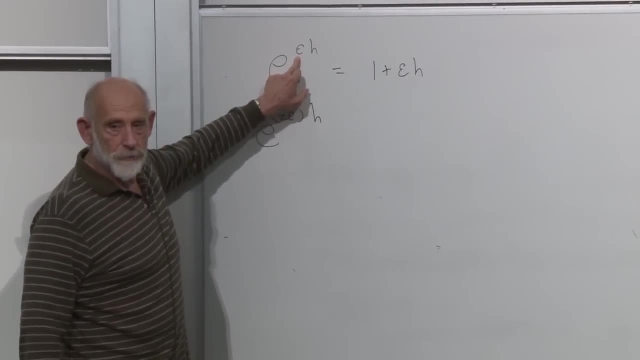 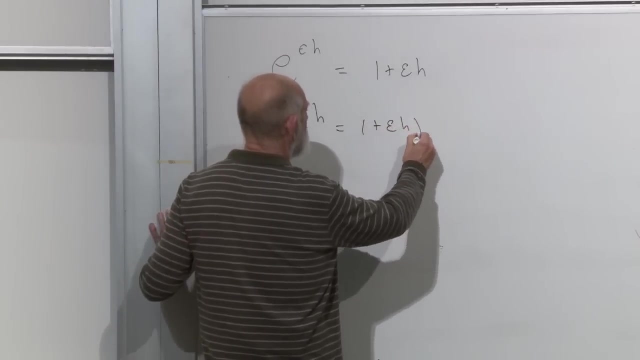 I want to take e to the two epsilon times h, E to the two epsilon times h is just the square of e to the epsilon h, E to the two times. something is just a square, so it's equal to one plus epsilon h squared. 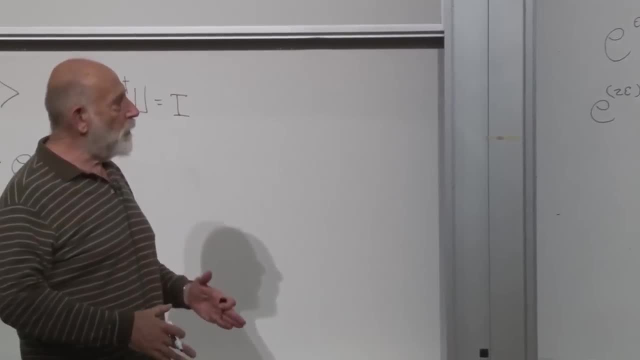 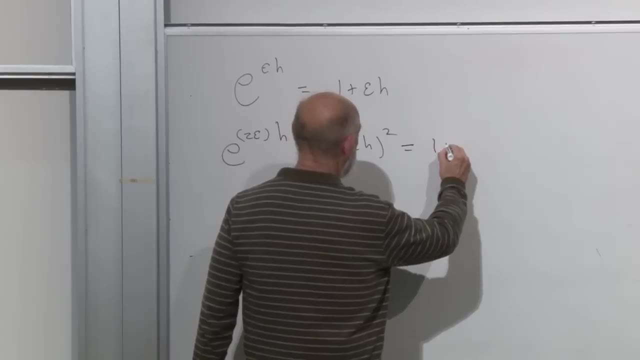 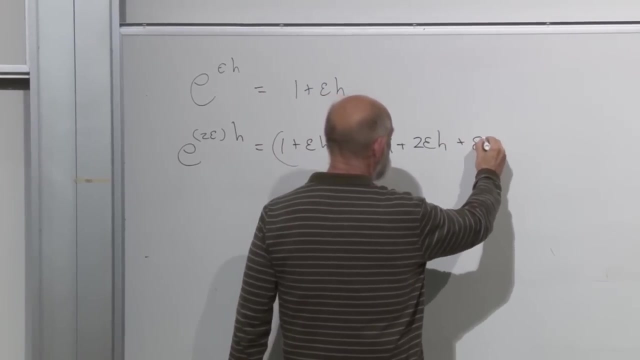 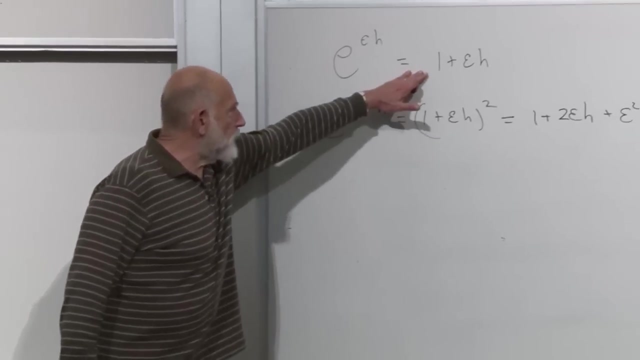 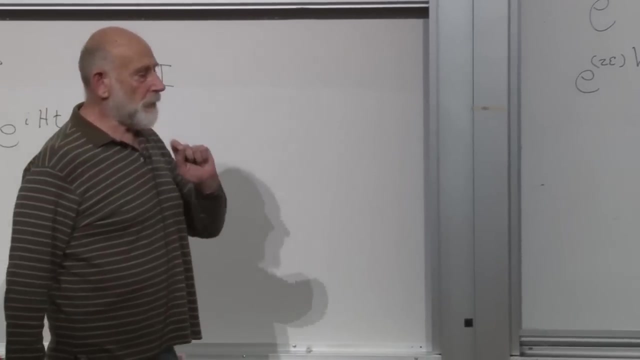 Supposing you do this over and over and over, which, incidentally, is equal to one plus two epsilon h plus epsilon squared, h squared. But this is still an approximation. This was an approximation to this. This is still an approximation to this. Here's a theorem that, if you do this, 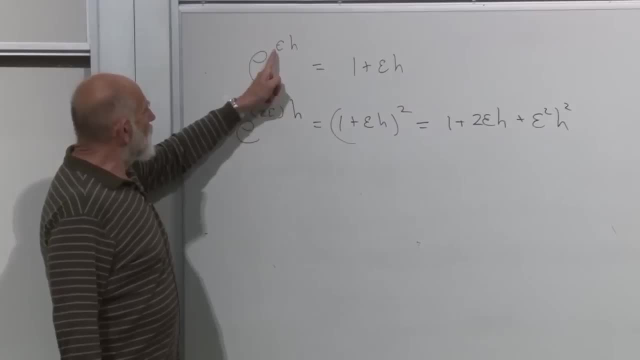 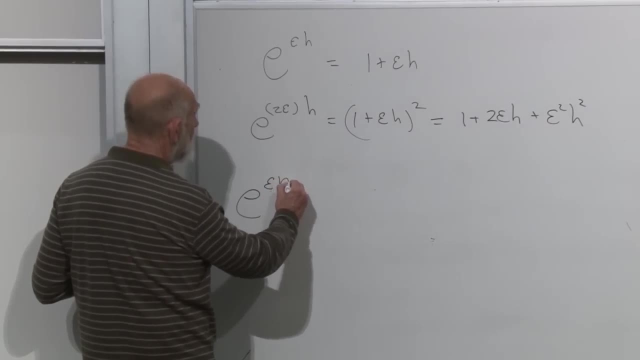 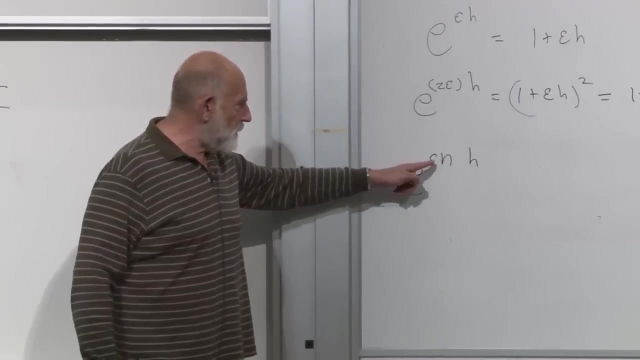 over and over enough times. let's say n times e to the epsilon times n times h, such that epsilon times n is finite. In other words, epsilon times n. epsilon is an infinitesimally small number, but I do it enough times. 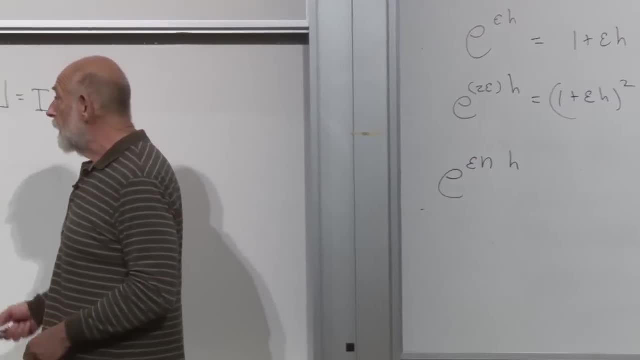 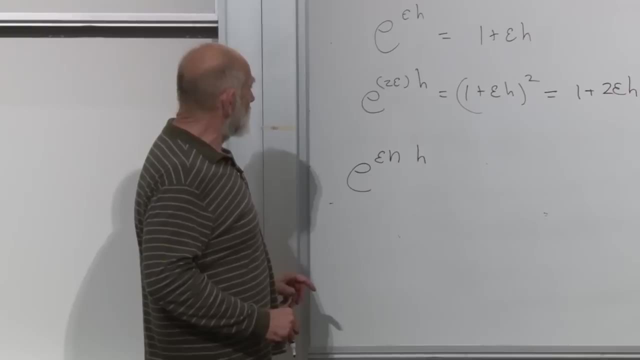 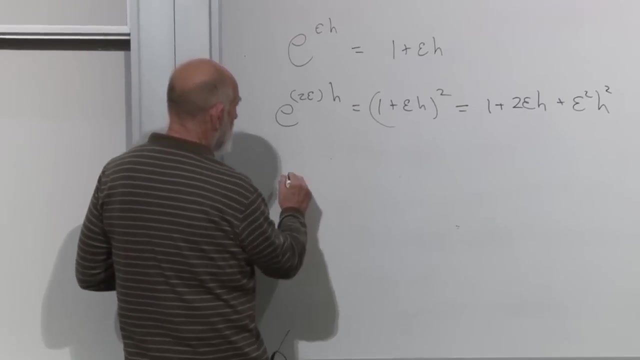 so that n times epsilon is a finite number, Namely t. I do this over and over What happens. Excuse me, let me go back. Let's do it this way: One plus epsilon h, and I do this a number of times. 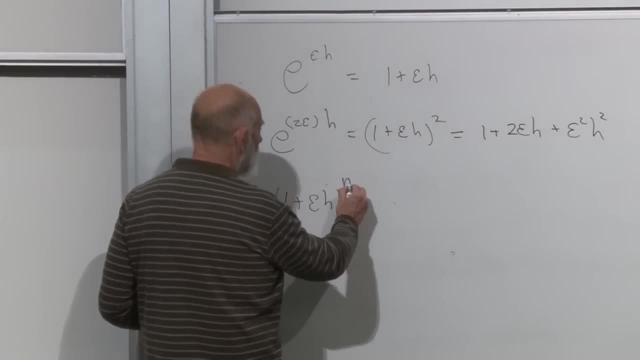 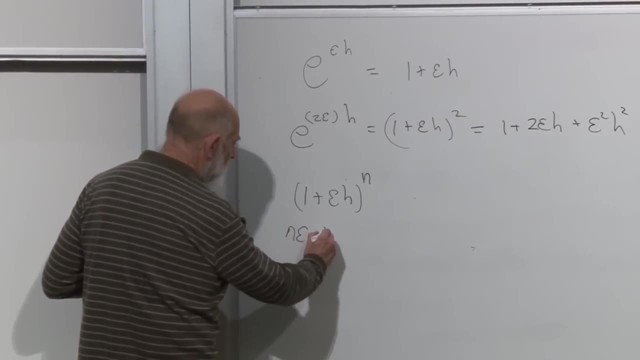 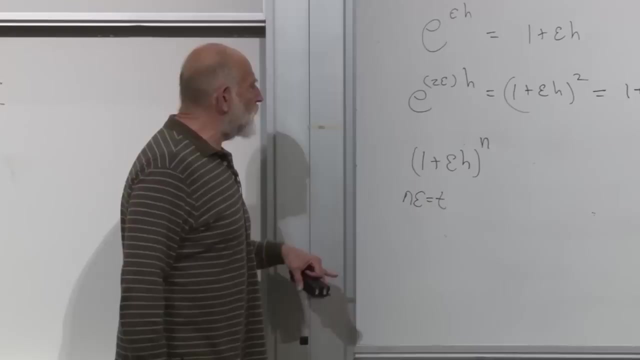 a large number of times n, such that n times epsilon equals t. What do I get? Anybody know It's a binomial expansion. Well, it's a binomial expansion, but it's also a construction of the exponential function. 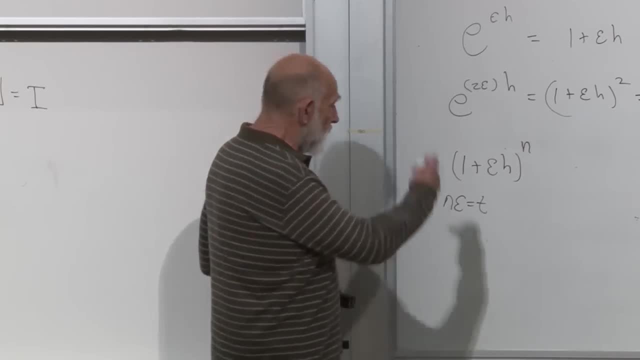 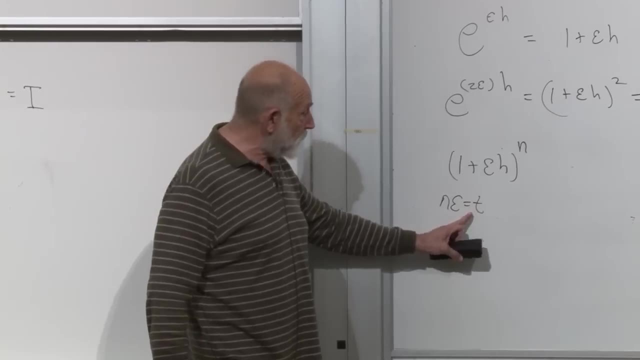 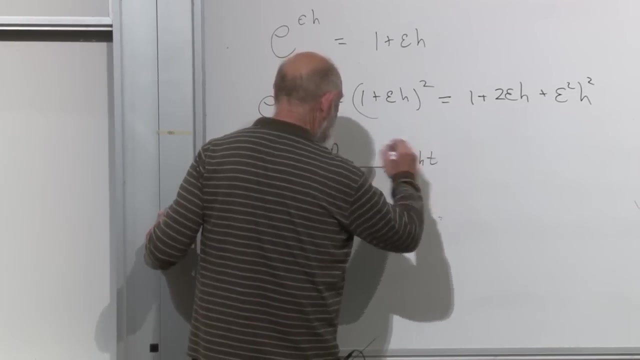 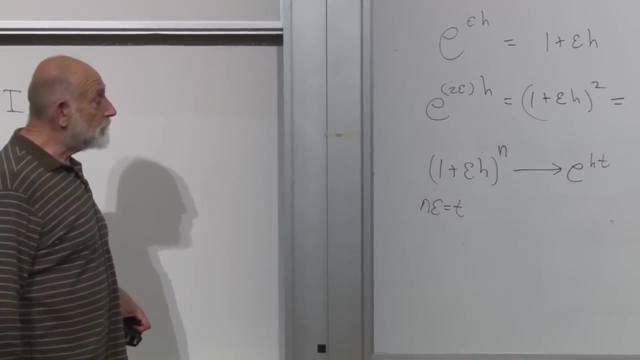 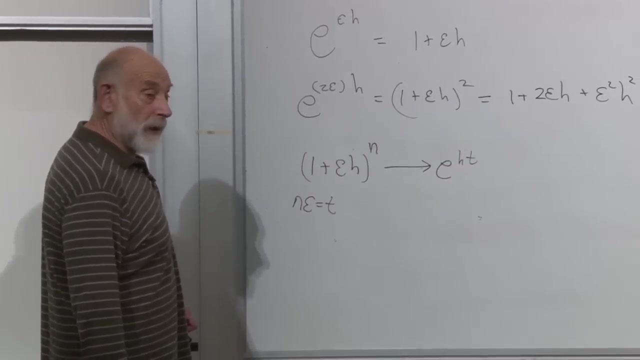 Okay, It's a rigorous theorem that as epsilon gets small and n gets large in such a way that n times epsilon is kept fixed, this just becomes e to the h squared t. Say it again: One person talk. I think it's right. 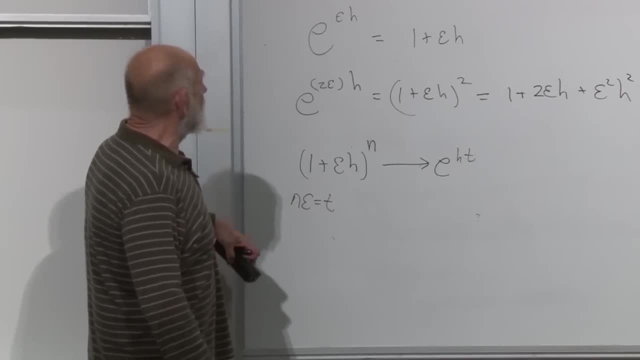 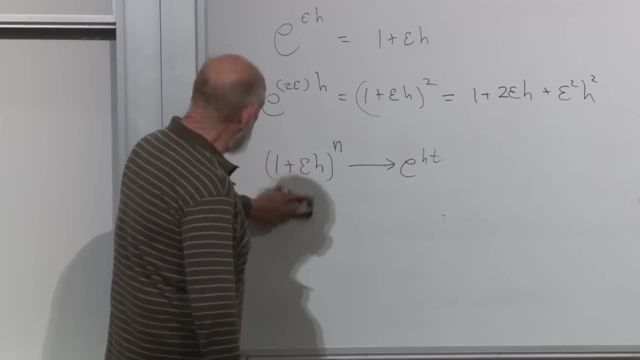 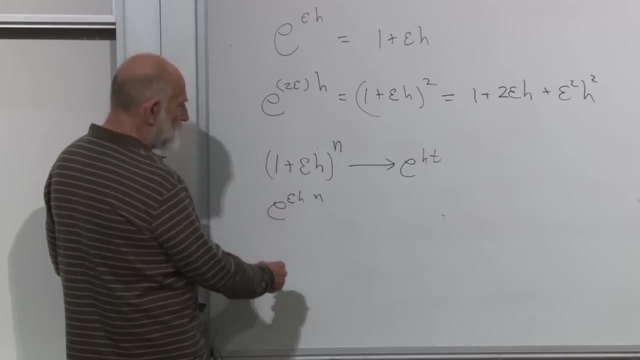 I think it's right. Right, And the way you can just understand it is by saying that for small epsilon, one plus epsilon h is the same as e to the epsilon h, and if you take it to the nth power, the epsilon just multiplies the n. 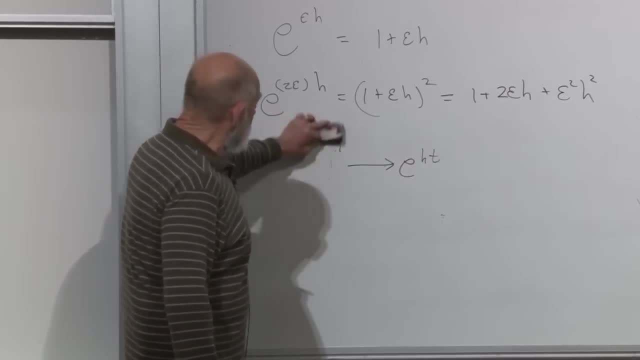 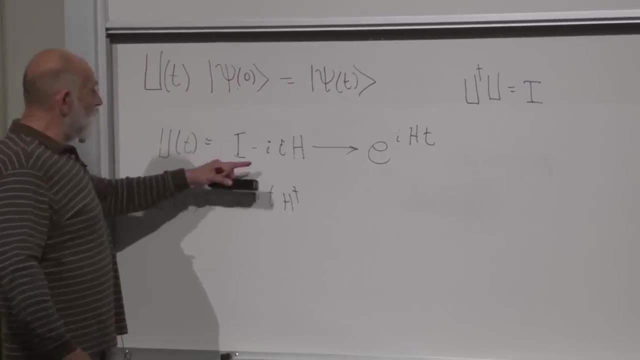 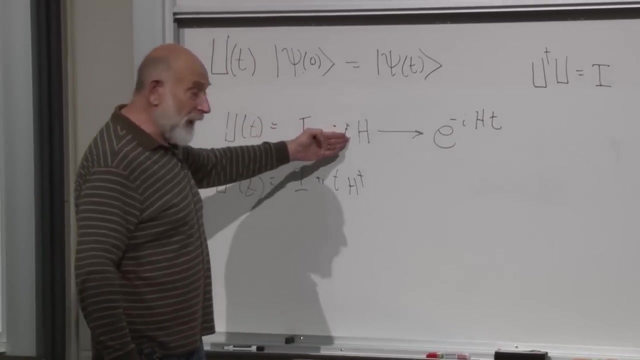 and becomes t. Okay, so I will tell you right now the generalization of this for finite times one. this should be a minus sign here. one minus i h t for finite t really becomes e to the minus i h t, and this is an important fact. 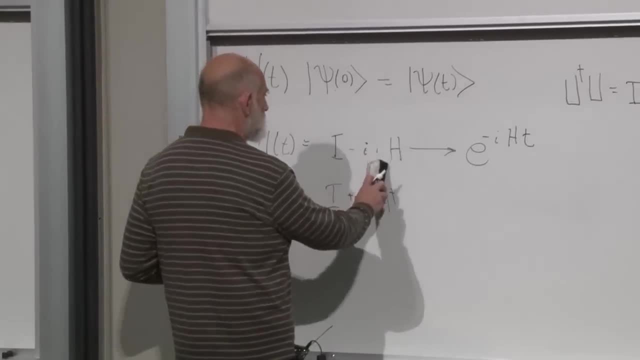 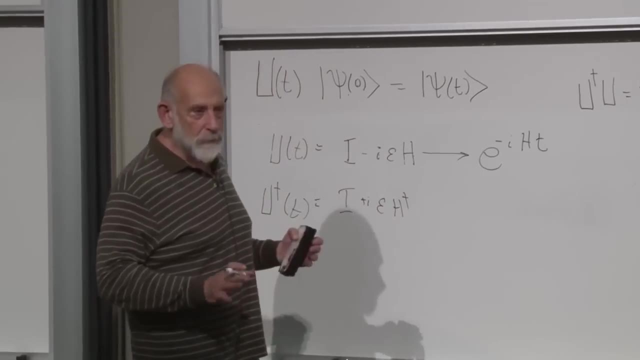 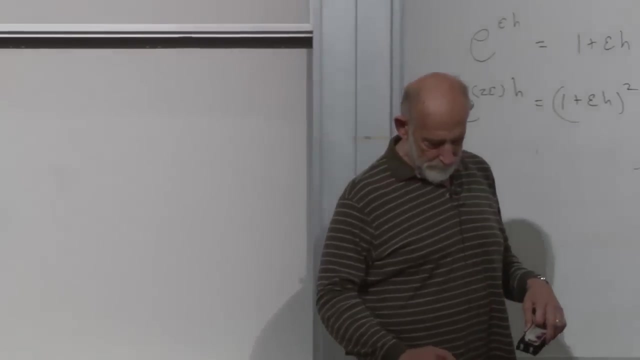 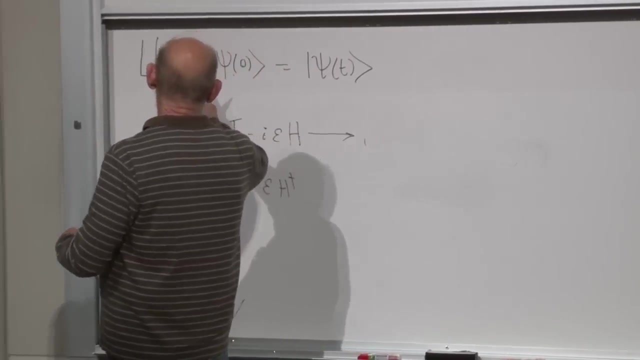 but for small intervals, small epsilon, we can just be consistent and work to order epsilon. We'll find out everything we need to know. Okay, so there's a concept now of a Hamiltonian. Let's see if we can understand this equation. 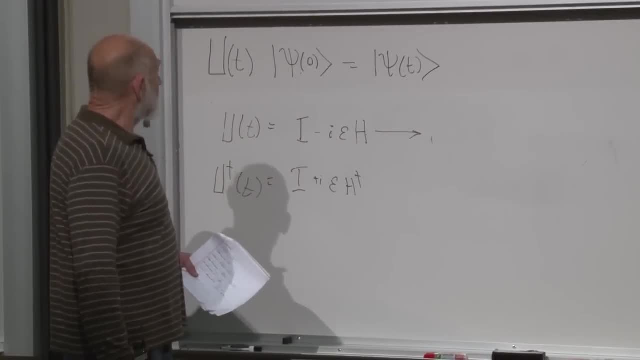 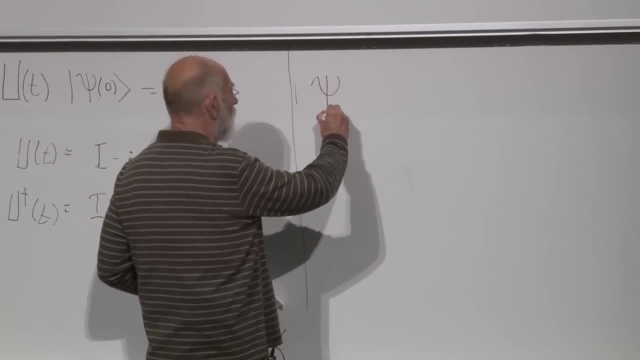 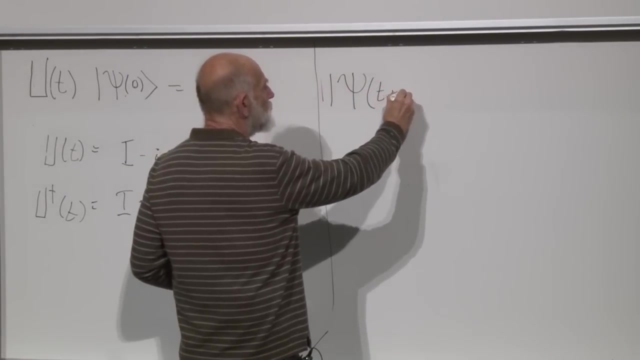 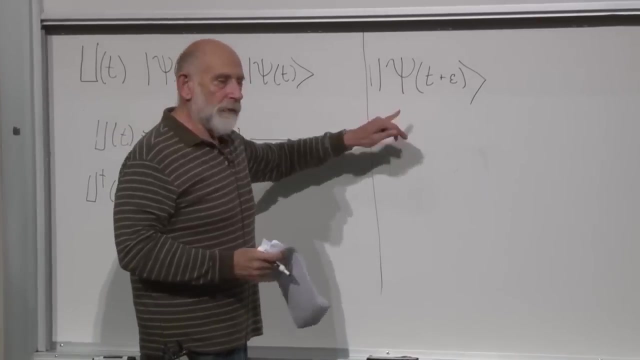 a little bit better. Let's take the wave function psi or the state vector- state vector psi at a time t plus epsilon. I'm starting at time t with a certain wave function and I'm allowing it to change over a tiny time interval. 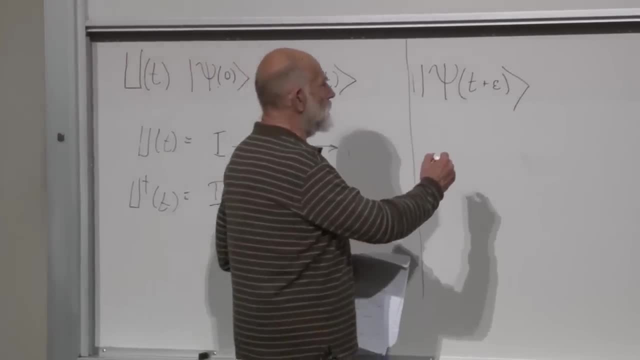 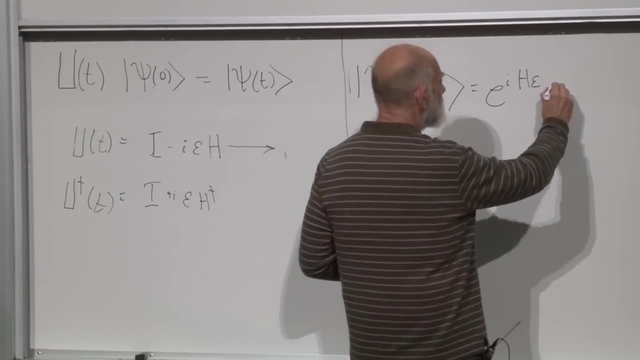 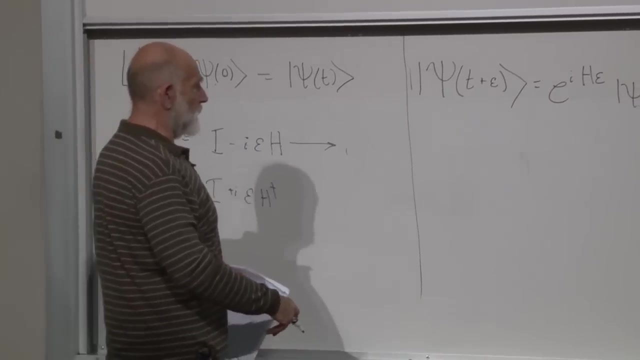 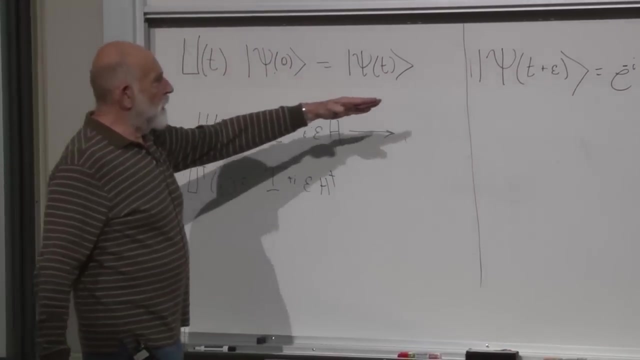 What is the answer to this? The answer to this is that it is equal to e, to the i, h epsilon times psi at time t. Let's just see what I did: Minus or plus, sorry, minus minus here, Starting at time t. 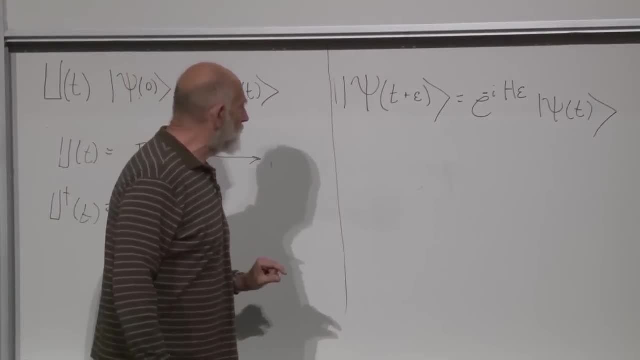 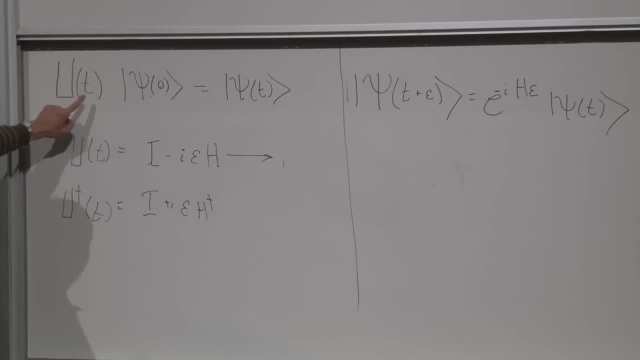 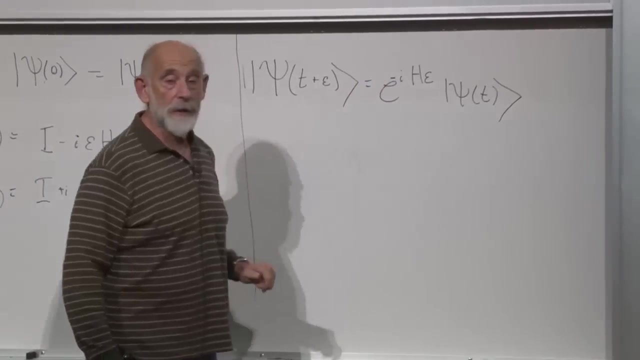 let's update by a small little time epsilon. The rule is we multiply by u of t, Sorry, u of epsilon. We're updating by an amount of time epsilon, and that's equivalent to multiplying by e to the minus i h epsilon times, psi of t. 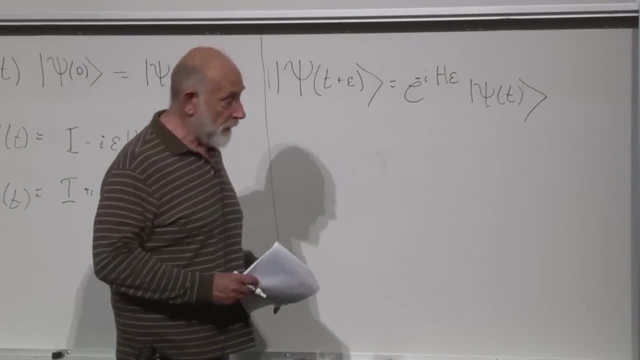 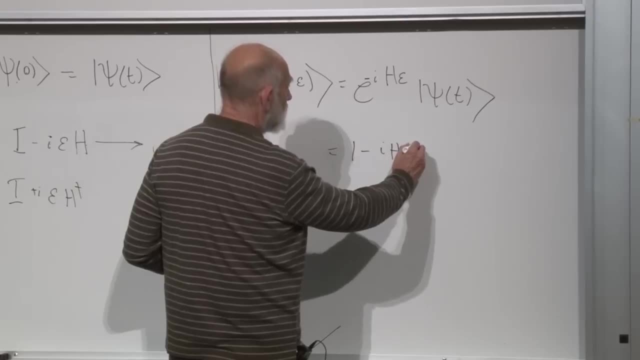 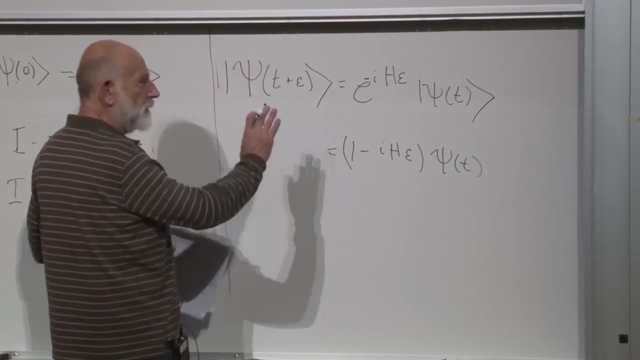 So this is the rule for going from a time to a neighboring time. But now let's write that out as one minus i, h, epsilon times, psi of t, And let's write this side. I'm not going to forget the okay. 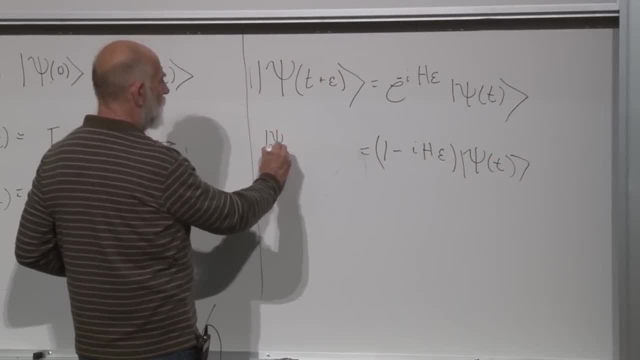 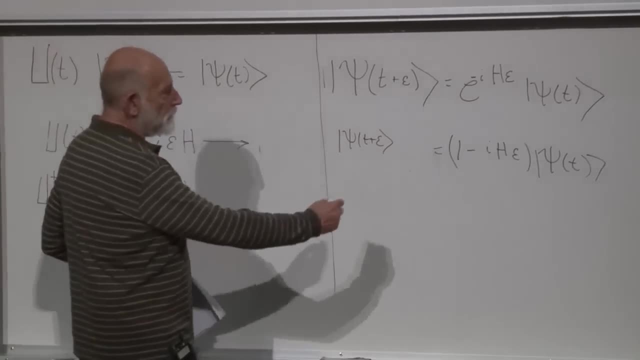 yeah, okay, yeah, let's put them in. And this one here is psi of t plus epsilon. Now let's multiply out One times: psi of t is psi of t, but let's take that over to the left-hand side. 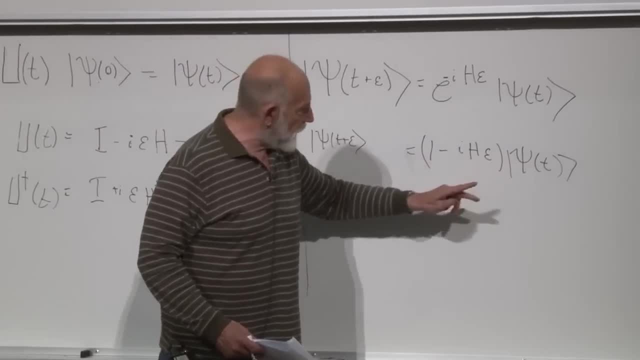 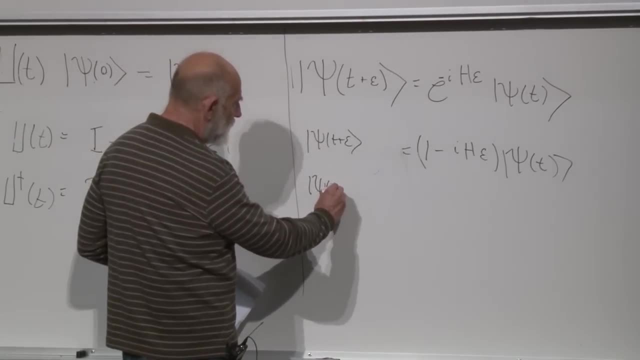 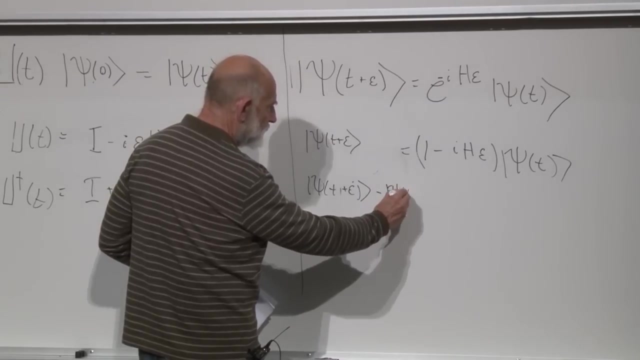 That'll give us psi of t plus epsilon minus psi of t, Just the term coming from one. The term coming from one will give us the difference between psi of t plus epsilon minus psi of t. You see where we're going. We're building a differential equation. 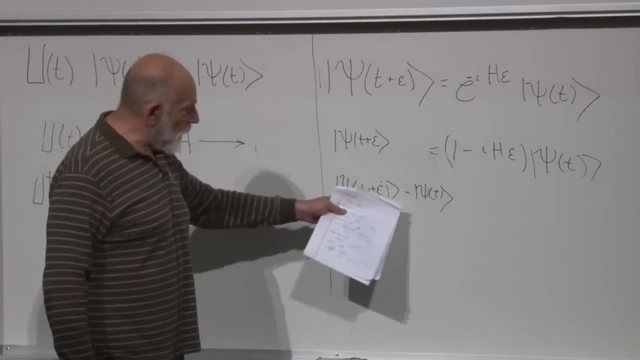 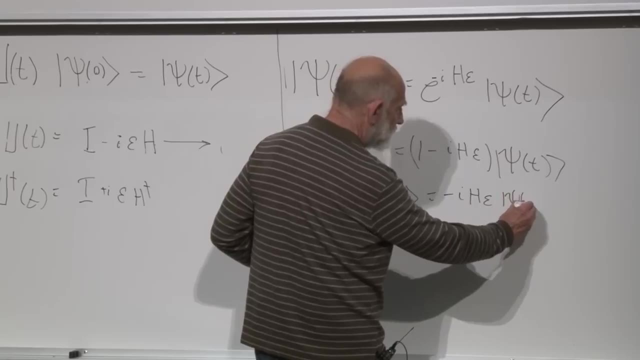 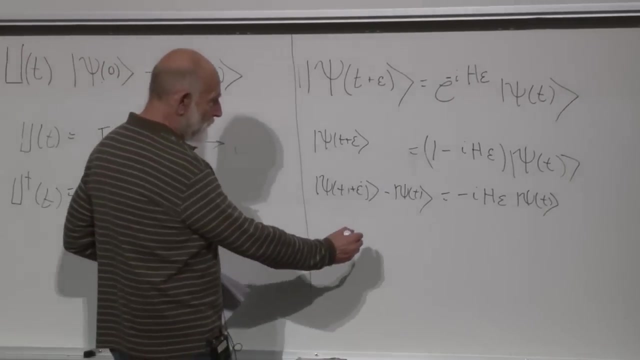 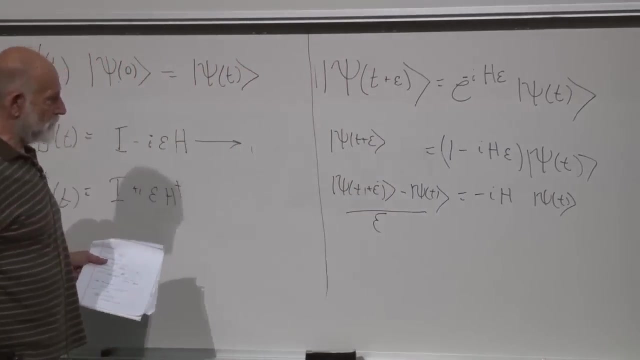 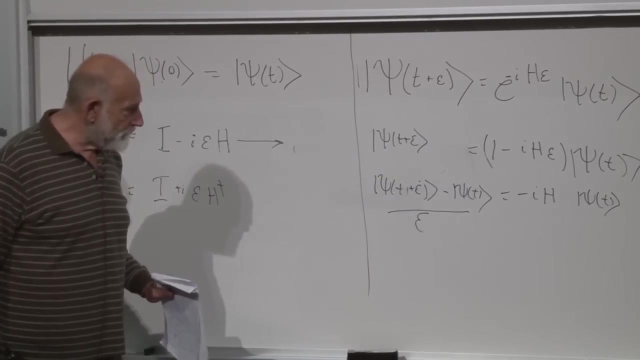 for psi. Psi of t plus epsilon, minus psi of t is just equal to minus i h. epsilon, psi of t And finally divide by epsilon. Okay, what's the left-hand side? The left-hand side is the time derivative of the state vector psi. 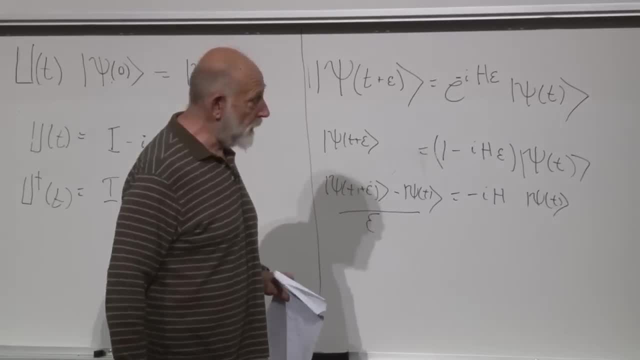 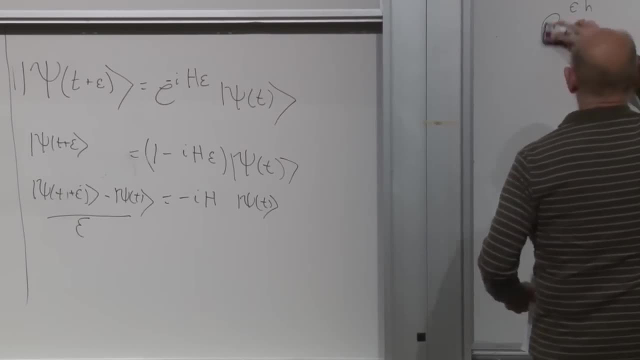 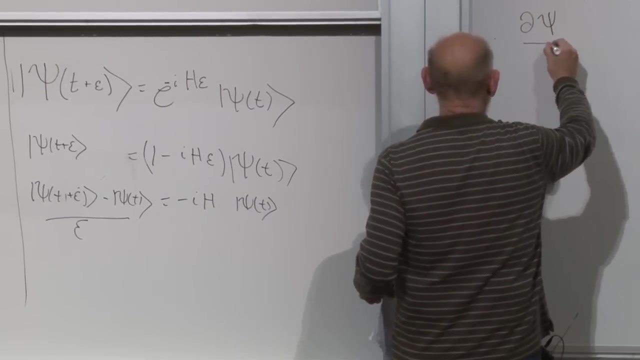 And the right-hand side is just minus i h psi of t. Okay, so that leads us finally to the Schrodinger equation. The Schrodinger equation says that d psi by d t. this could be a wave function, or it could be the state vector. 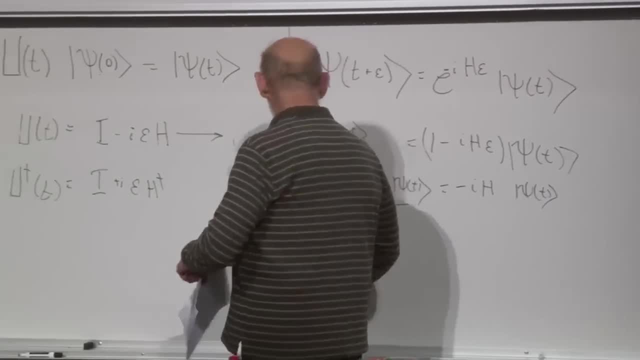 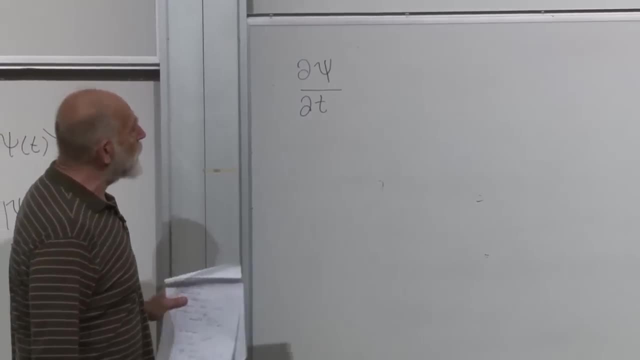 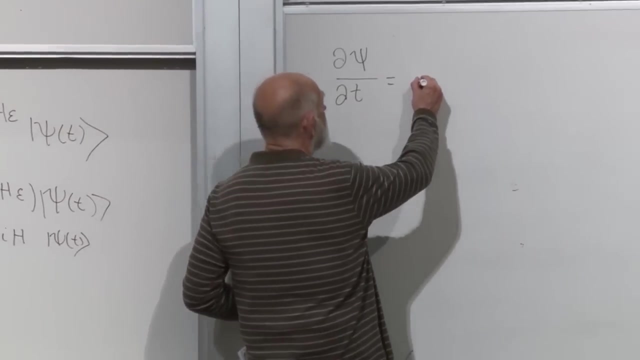 I will leave the notation a little bit abused. I won't bother writing the ket vector here. It stands for both the equation for the state vector or the equation for the wave function itself. d psi by d t is equal to minus i h psi. 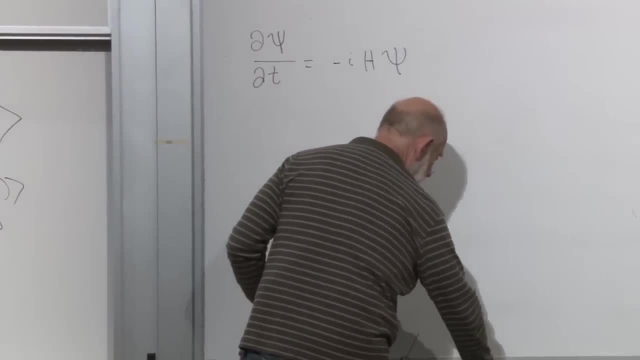 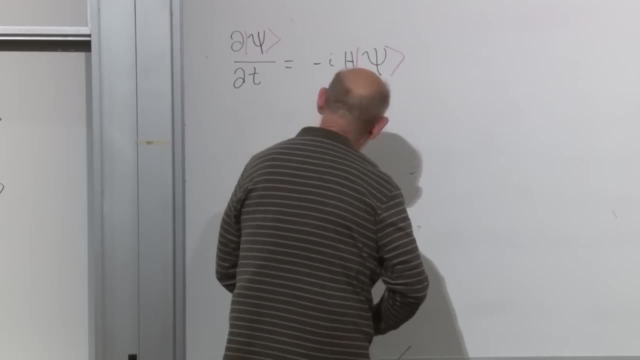 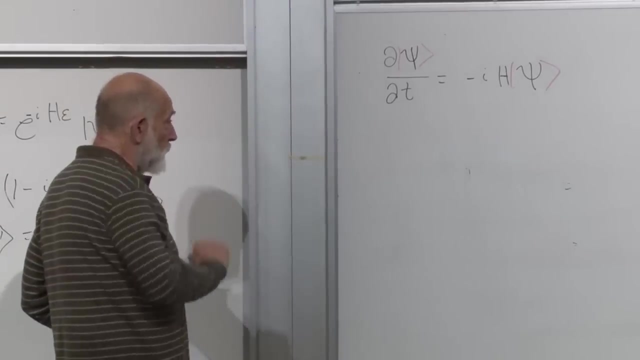 If you want to put vectors in, if you want to turn it into an equation for a state vector, you put ket notations there. Otherwise it's just the equation for a wave function. This is the Schrodinger equation. This is the time derivative. 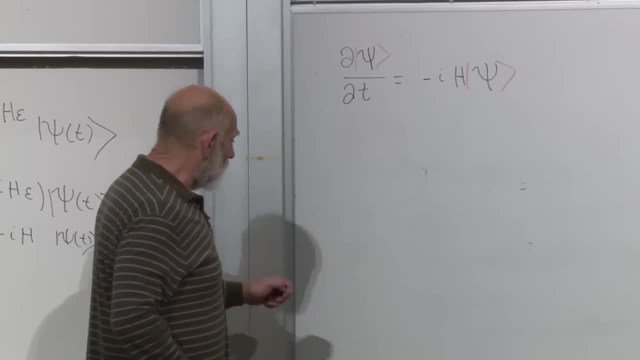 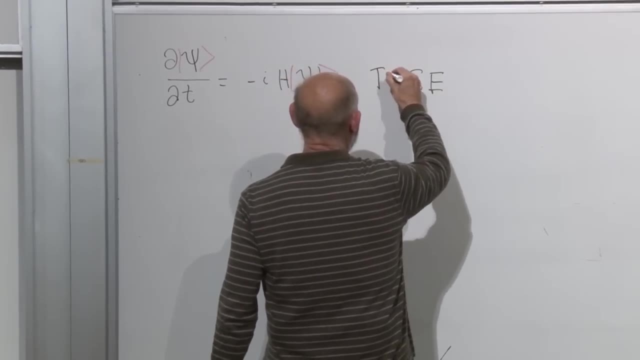 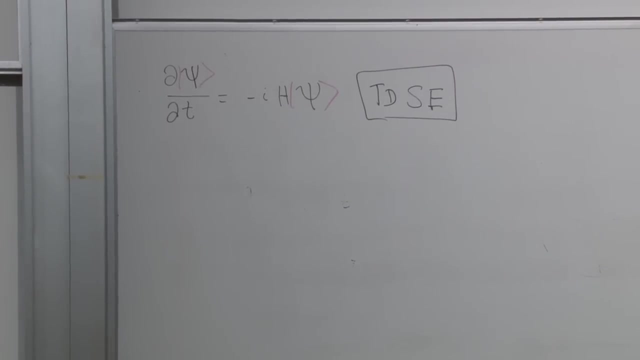 dependent Schrodinger equation. Okay, this is Schrodinger equation: time dependent, the TdSe, time dependent Schrodinger equation, And what it tells you is how the state vector changes as a function of time. if you are so lucky to know. 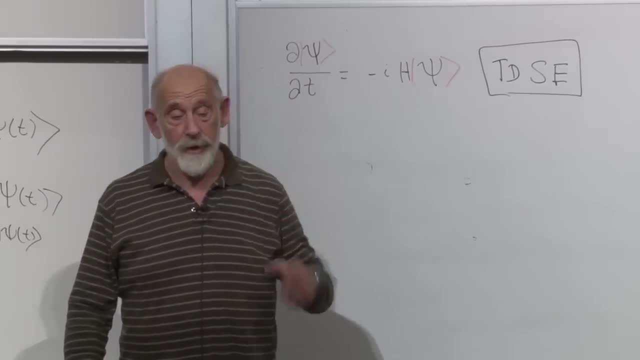 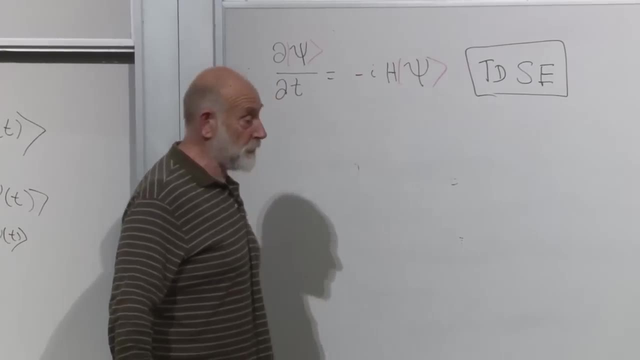 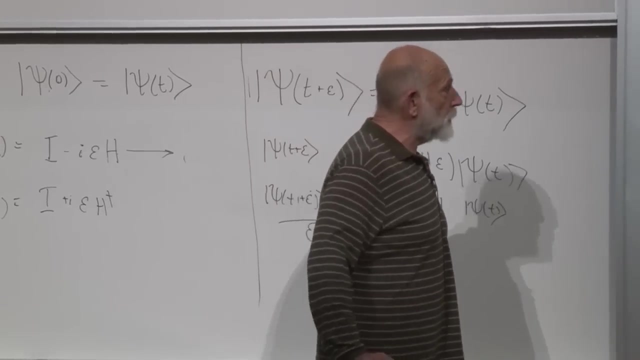 what the Hamiltonian is. Hamiltonian is a Hermitian operator and you can make all kinds of quantum mechanical systems just to play with using different h's. We did this last quarter. Okay, what about the time? independent Schrodinger equation. 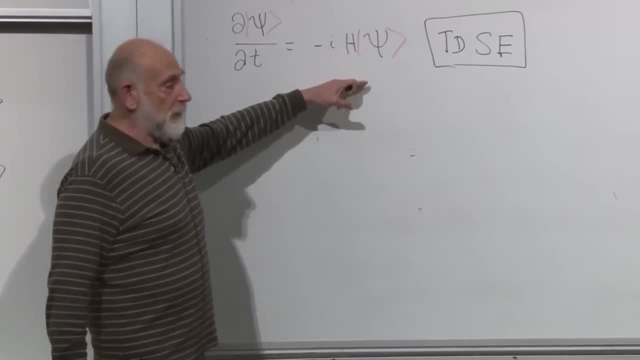 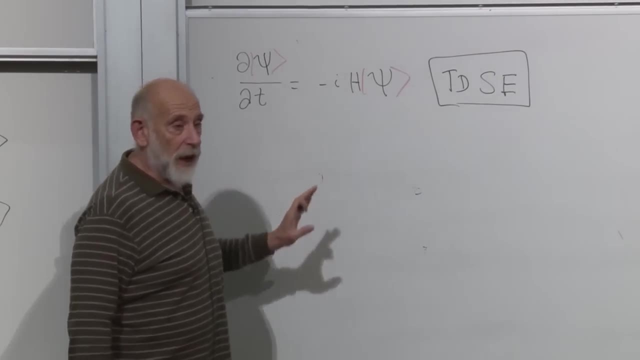 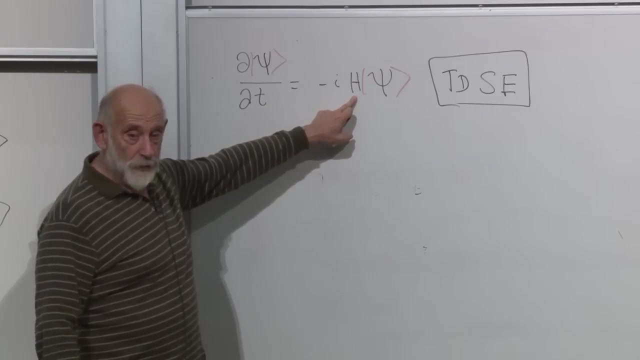 The time. independent Schrodinger equation is just the statement that h is a Hermitian operator. It has eigenvalues, It has eigenvectors. Its eigenvalues are the observable values that you would get if you measured h, And what are they called? 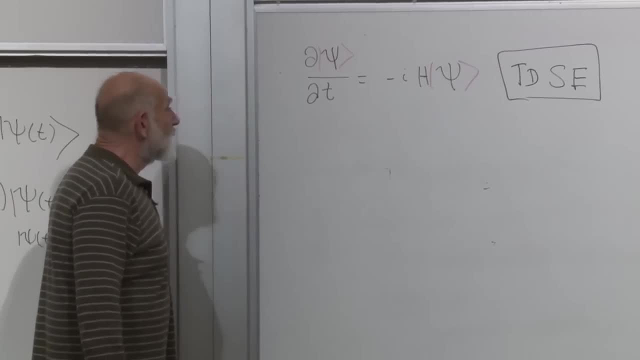 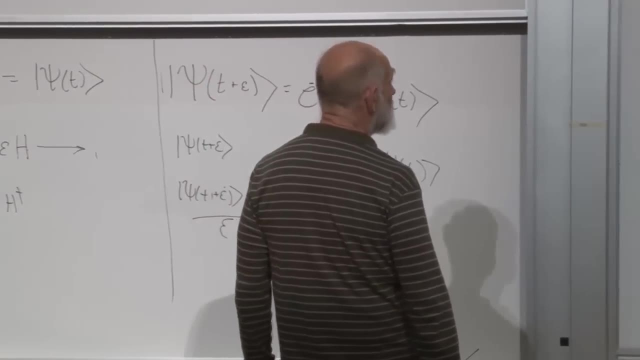 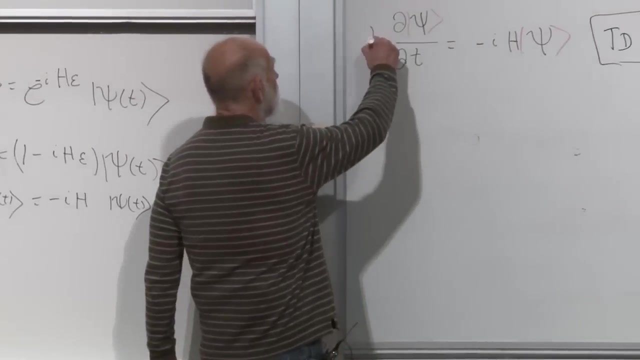 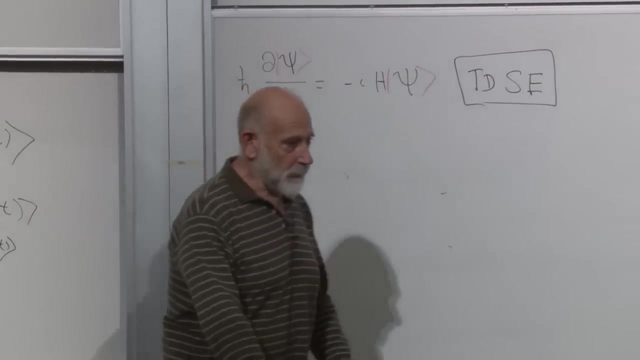 What's the name? Energy levels. Incidentally, I promised you that I would keep around Planck's constant and I've already dropped it. It goes over here. It goes over there. I don't promise by any means that I will be consistent. 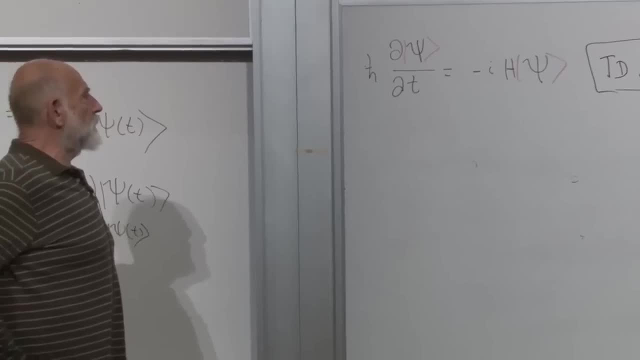 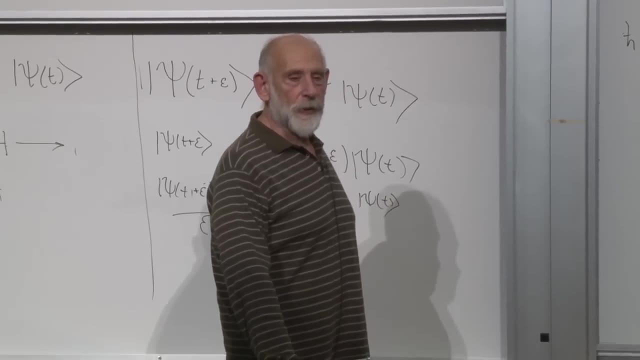 about Planck's constant. Yes, I will be completely consistent by choosing Planck's constant to always be equal to one. Sometimes I'll put it in, sometimes I won't put it in, but I will never confuse it with I or the square root of two. 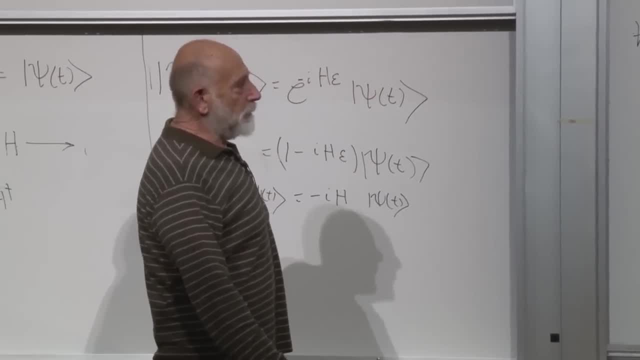 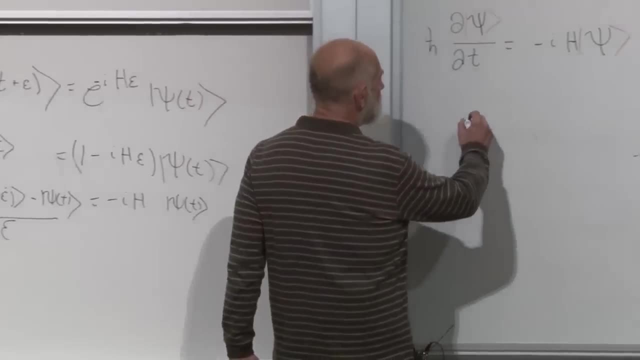 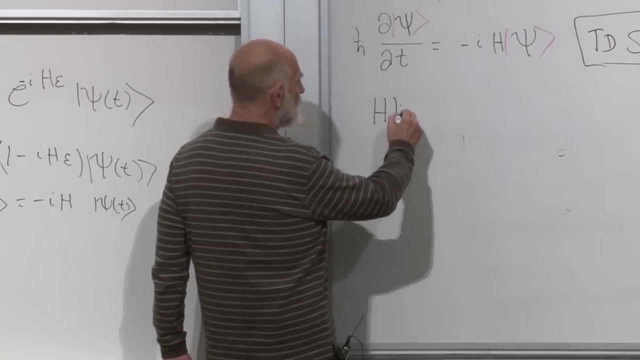 Okay, so that's the time dependent, The time independent Schrodinger equation. that's just the eigenvalue equation for the eigenvalues of h, And all it says is that h on an eigenvector of the energy, a state with definite energy. 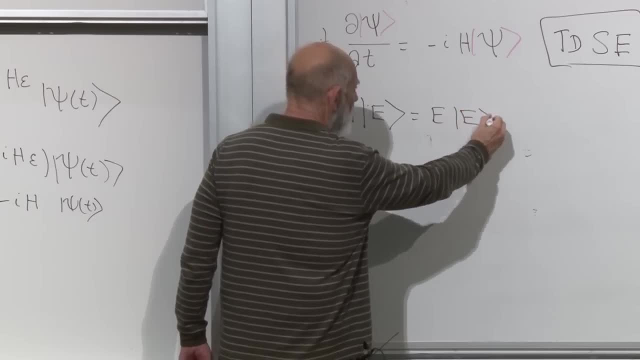 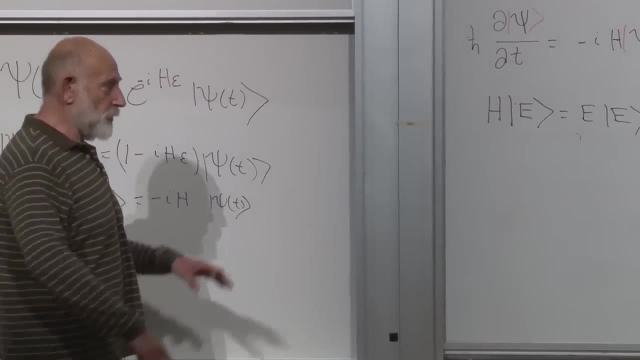 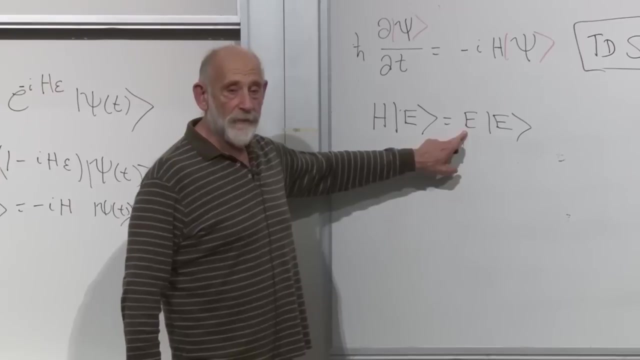 is equal to E times the energy, E being the eigenvalue of h, E being the eigenvalue of h. So this equation here is the equation which tells you how to find the states and the values of energy that go with them, that correspond to states. 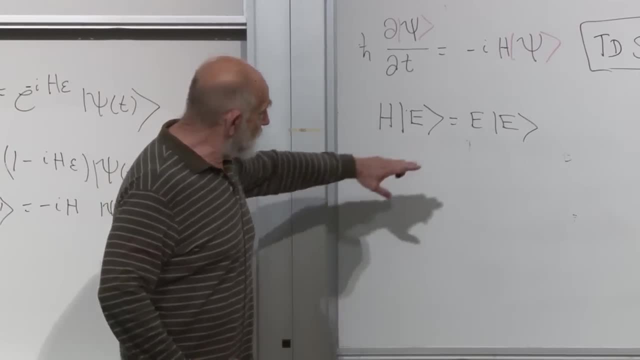 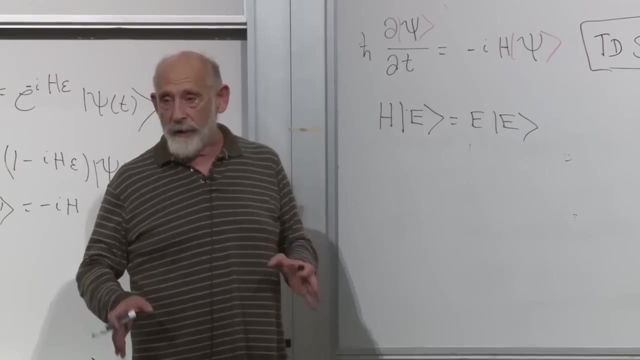 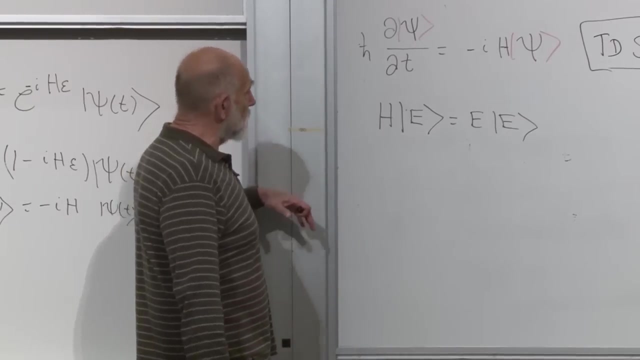 of definite energy. You solve this equation and it gives you a whole bunch of possible eigenvalues and eigenvectors. Those are the eigenvectors and eigenvalues of the energy operator. Okay, and again we went through this, we did some examples. 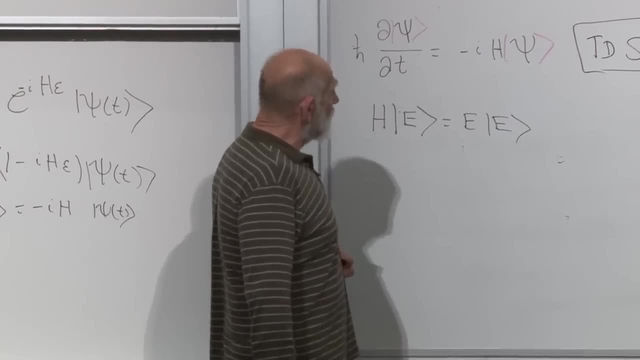 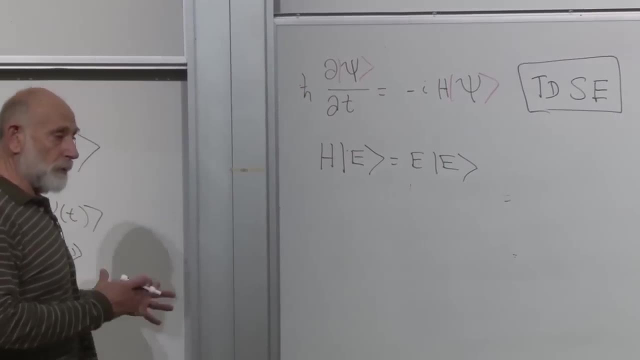 last two quarters ago. On the other hand, this equation tells you how the state vector changes with time And, as you can see, it's the same h in both equations. so the question of the energy level of a system are intimately bound up. 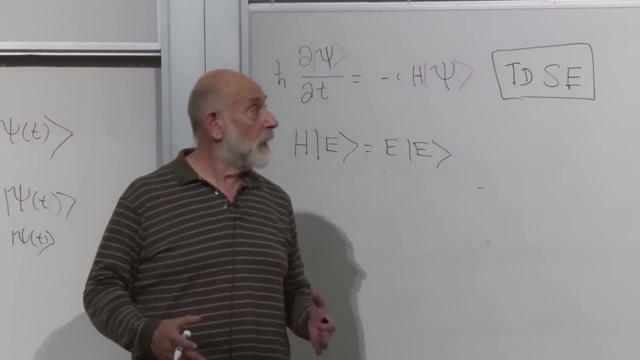 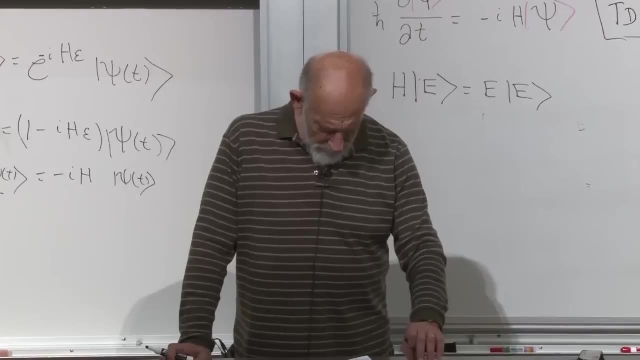 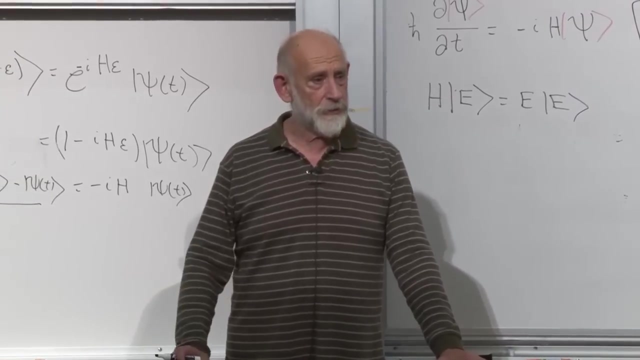 with the way that the system changes with time. Okay, so good, And that's that's quantum mechanics in a. I said before it was quantum mechanics in a nutshell. Well, it's a slightly bigger nut, but that's it. 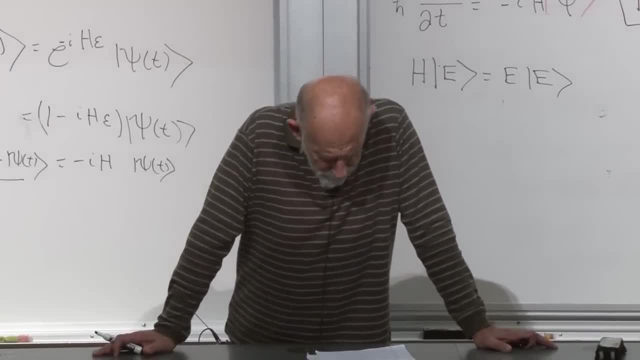 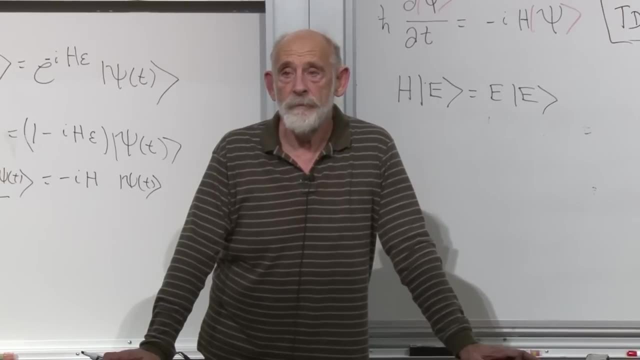 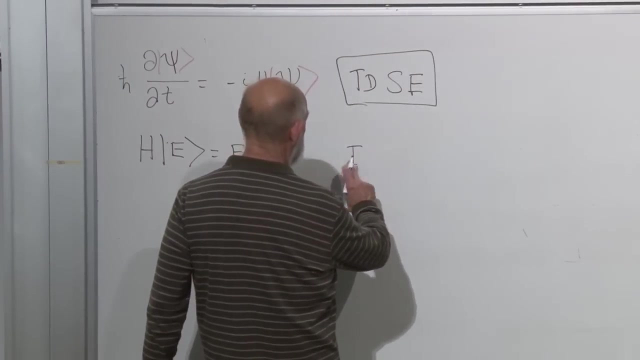 That's what you need to know. That's a summary of a quarter's worth of quantum mechanics That we did Any questions? Okay, can you if, if in the time-dependent equation time it's a time-independent Schrodinger equation? 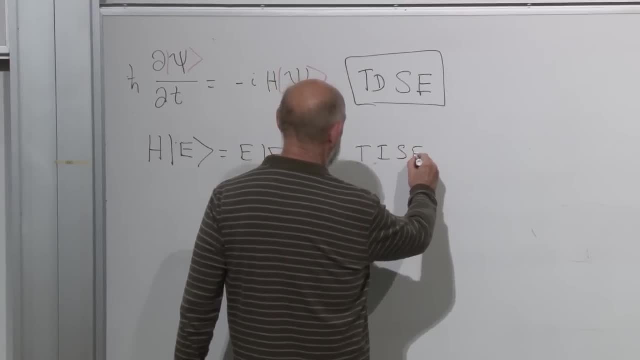 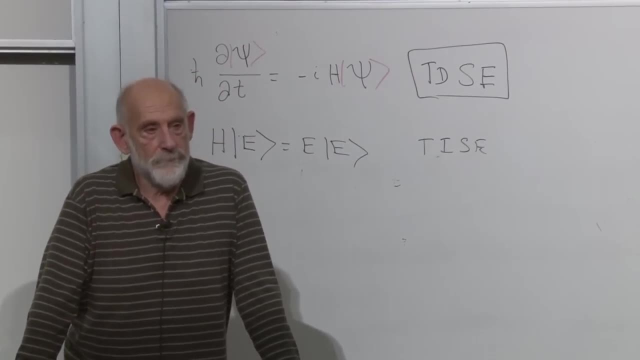 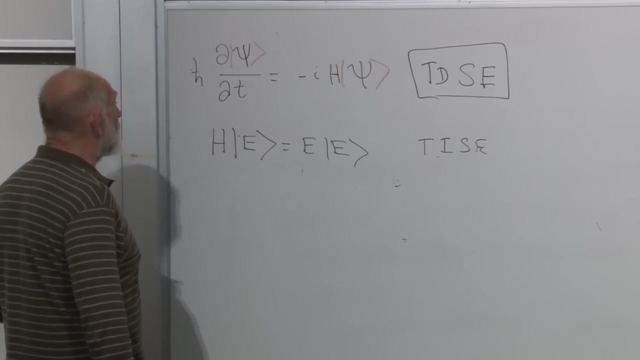 If in the time-dependent Schrodinger equation you replace psi with e, Psi with e, Yeah, can you, can you do then then you can drop the ket things. Oh, yeah, yeah, yeah, yeah, yeah, yeah. 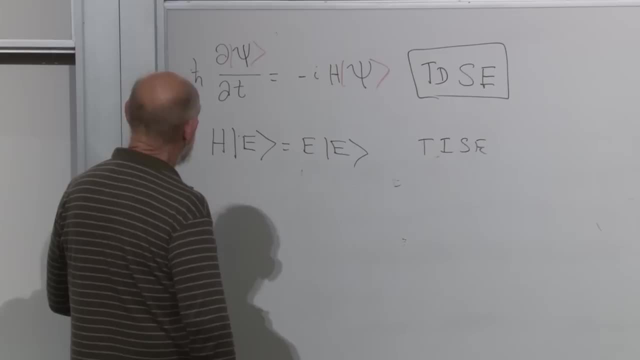 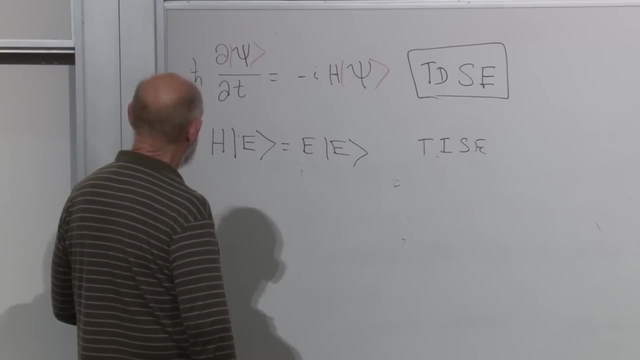 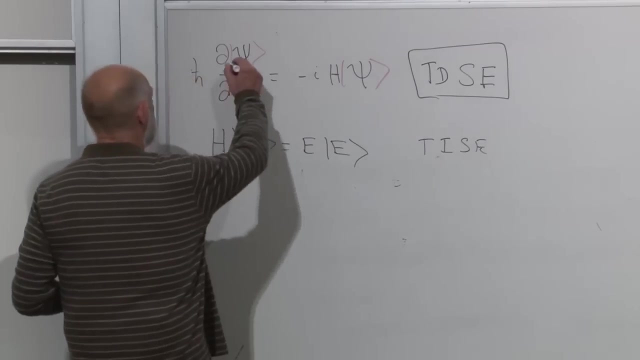 if you're not going to do the ket things right, Then it becomes just an equa-, a differential equation, because h times e will be just e times e. No, well, we, no, we don't want to drop the. 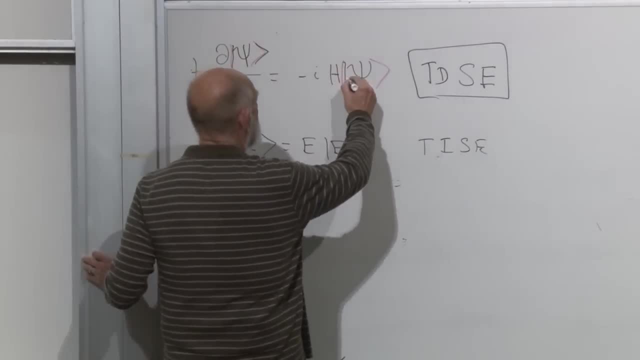 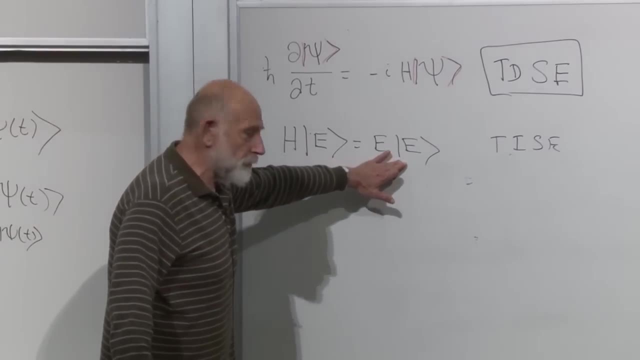 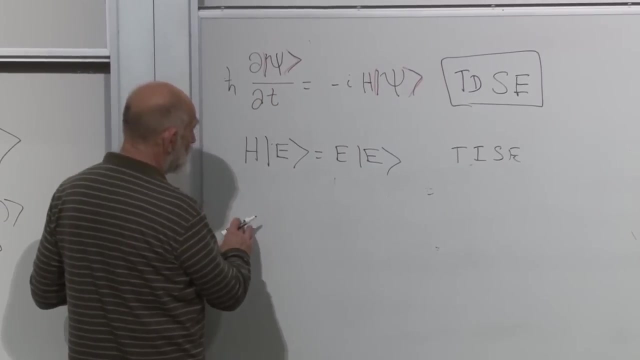 the ket symbol. Leave the leave the ket symbol there, All right. leave the ket symbol there for the moment. all right. What we can do is we can ask how a eigenvector changes with time. that we can do, So we can plug in here and we can ask how the eigenvector changes with time. 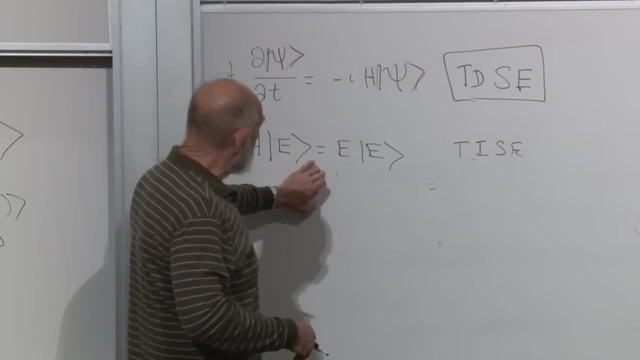 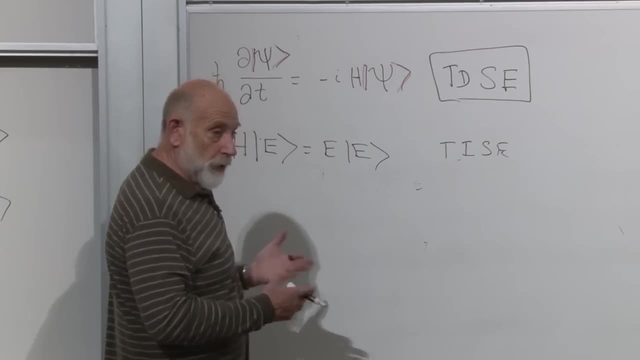 And the answer is that the eigenvector will change with time by just multiplying it by i times the energy level. That's what tells us how eigenvectors change with time. Anybody remember the answer? how an eigenvector changes with time? 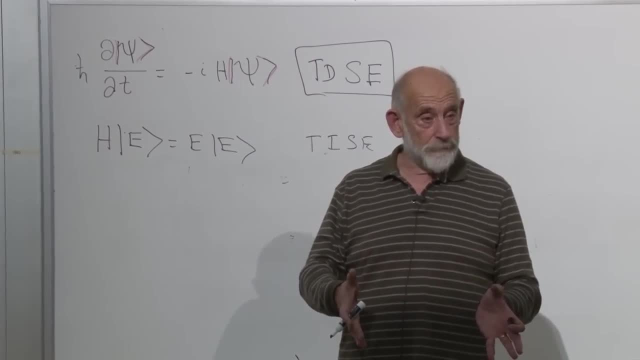 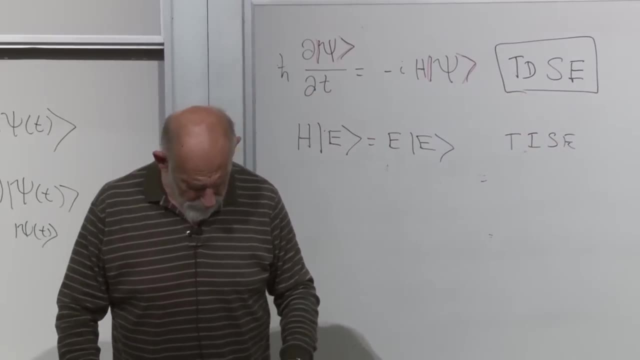 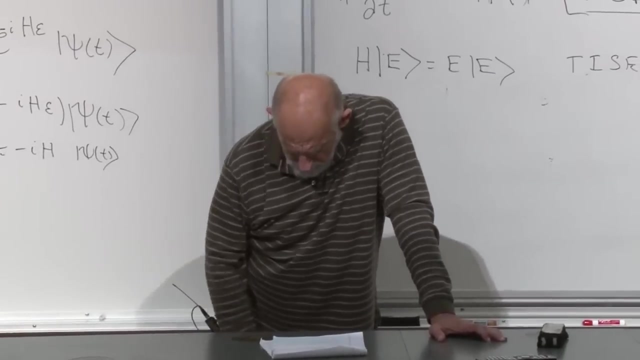 It just gets multiplied by e to the i times the energy times time. Okay, so that that we can go through that. we don't need It's in the notes, go back to it and and check it out. All right now the time evolution is one example of transformations. 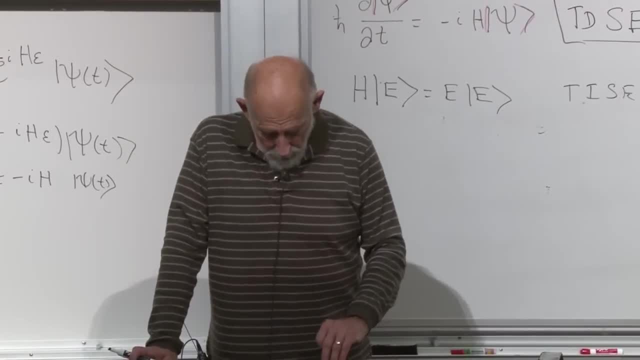 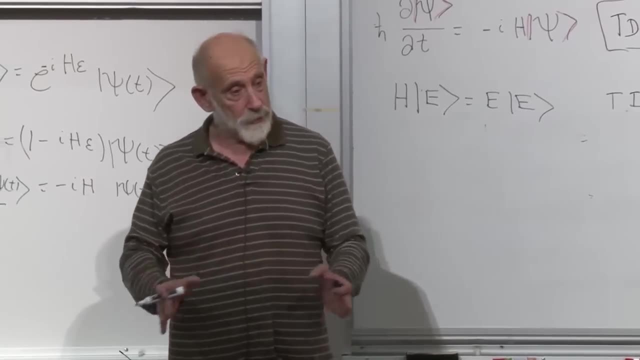 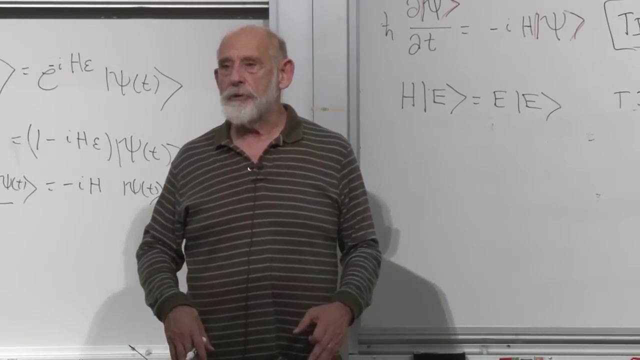 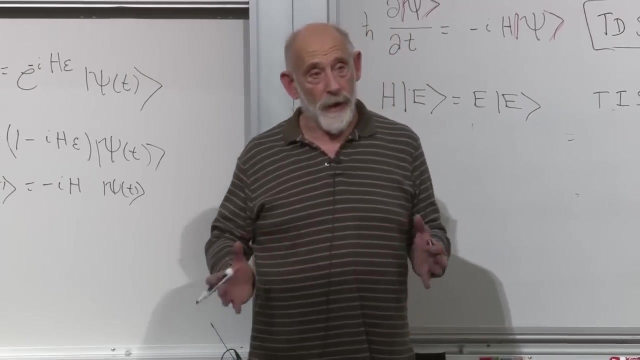 that you can do on a system which preserve certain facts about the system In particular, which preserve the inner products between vectors, In other words, which preserve the logical relationships between vectors, Preserve the notion of orthogonality, Preserve the notion of vectors being the same vectors. 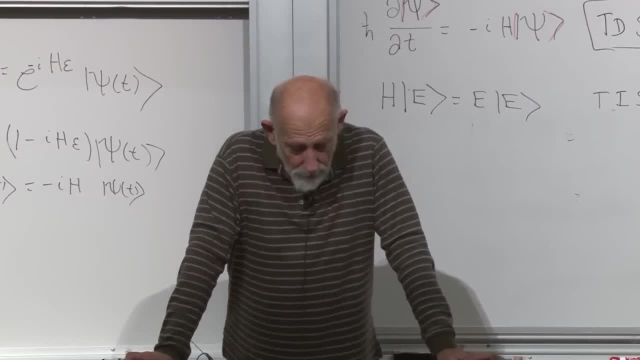 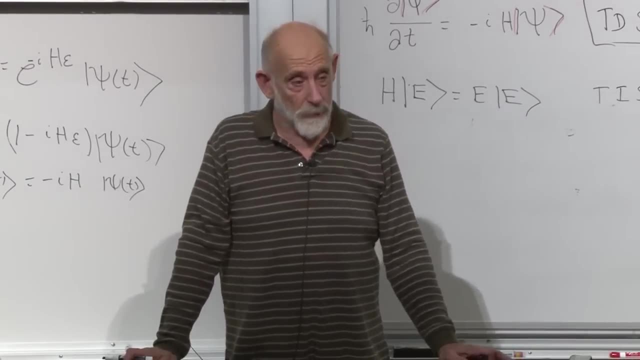 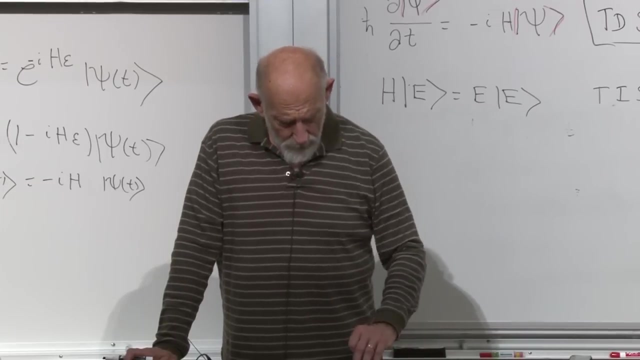 And and that kind of that. There are many other kinds of transformations that you may want to do on a system In particular. among them are symmetry transformations. We will need to talk about symmetry transformations Now. I will tell you where we're going. 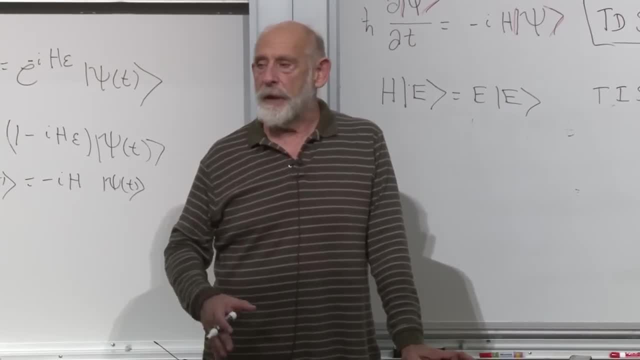 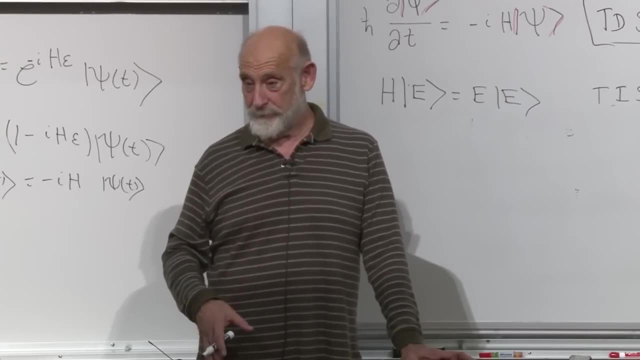 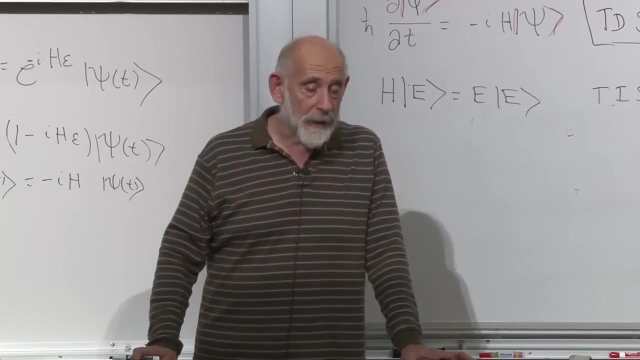 One of the most important symmetries of nature that occur over and over and over again in all sorts of contexts, but in particular in the theory of atoms, is rotational symmetry. A atom, in particular a hydrogen atom- A hydrogen atom is an electron moving in a central force field. 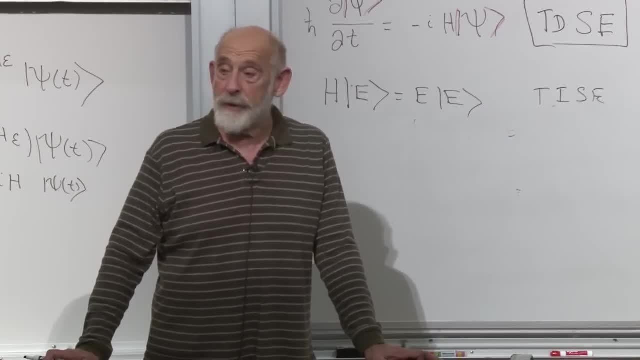 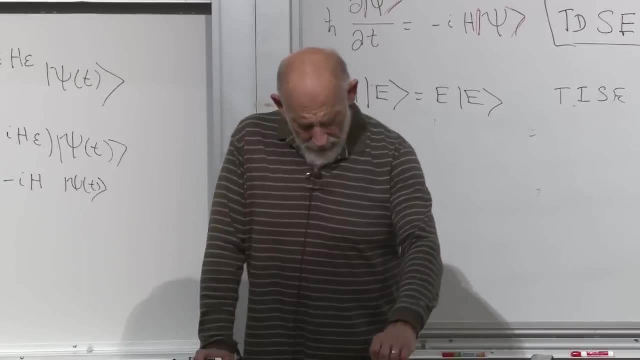 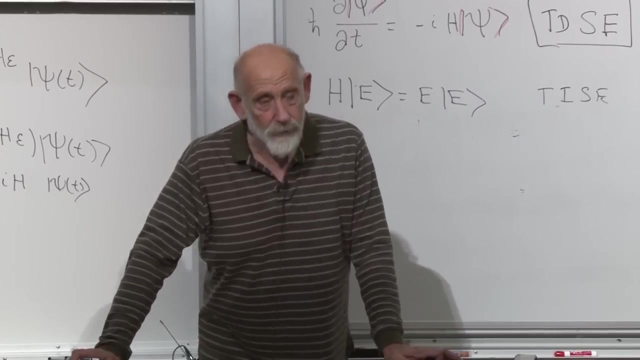 The equations of a hydrogen atom are rotationally symmetric, And that's because the potential energy, the Coulomb potential, is rotationally symmetric. it's a central force, And so hydrogen atoms, and basically all systems in nature really, but hydrogen atoms in particular- enjoy rotational symmetry. 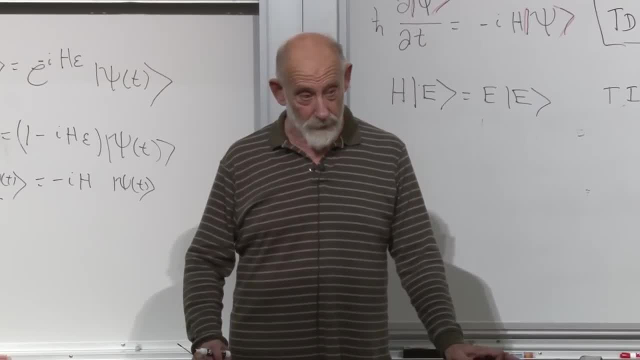 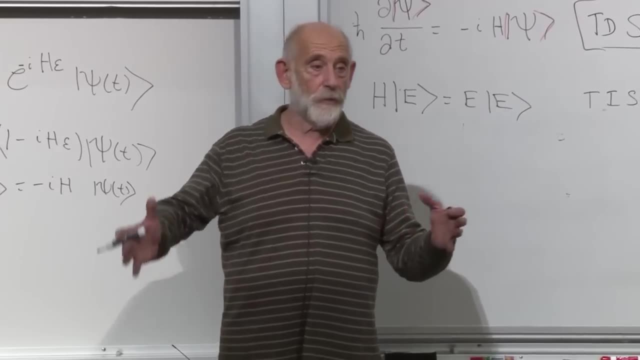 If you rotate. all it means is that if you rotate your coordinates, the description of the hydrogen atom doesn't change, Or another way to say it is: if you rotate the hydrogen atom, it's still a hydrogen atom. It may or not, may not be the same state, but 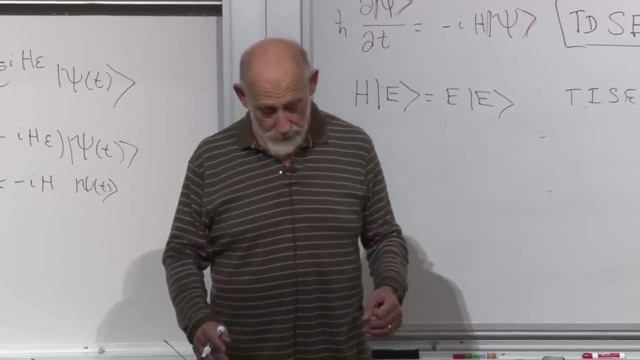 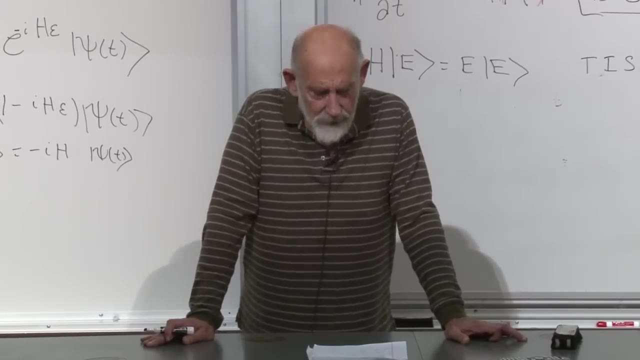 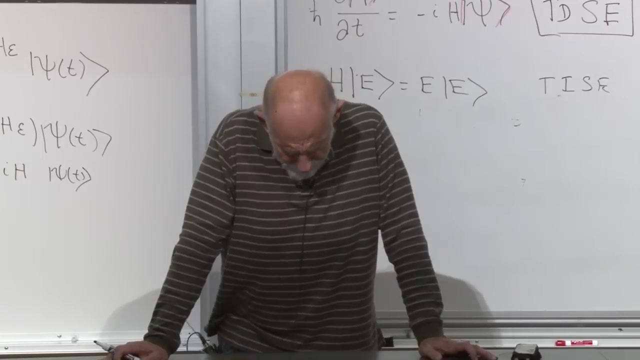 it's still a hydrogen atom described by the same set of equations. So The notion of a symmetry Is central in quantum mechanics. It was also in classical mechanics, but it comes up and really hits you over the head in quantum mechanics. And we need to explore some more. So it's a little bit of an extraction, oforters, to answer your whole question: No accomplishment, It's themselves. By the way, we've seen ear to ear a lot of used to talk about support chemical reactions. 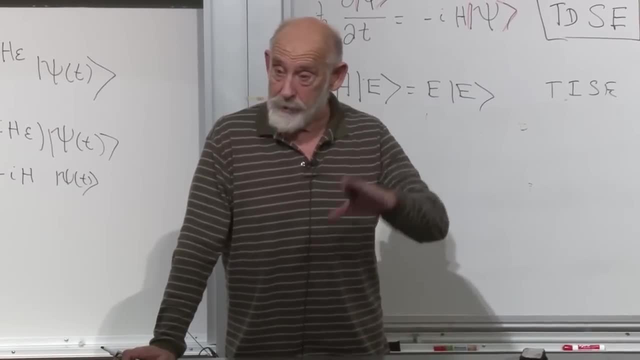 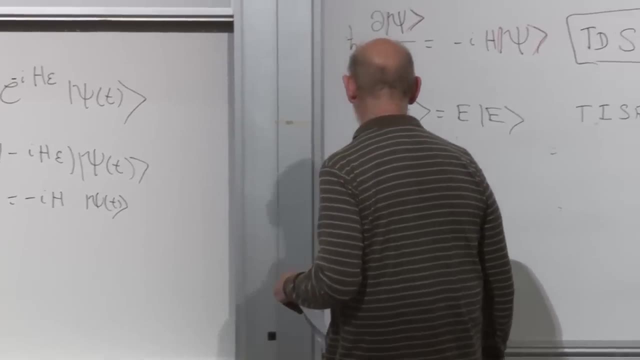 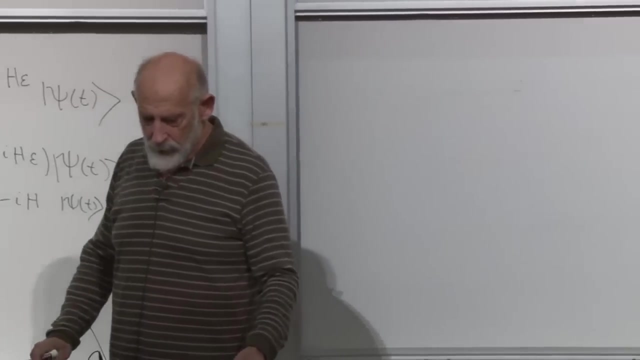 Or largely for the purposes of understanding rotational symmetry. we need to understand the concept of a symmetry, So I'm going to spend 15 minutes explaining exactly what a symmetry is. Keep in mind if you want to keep one in mind. there are two that you can keep in mind for. 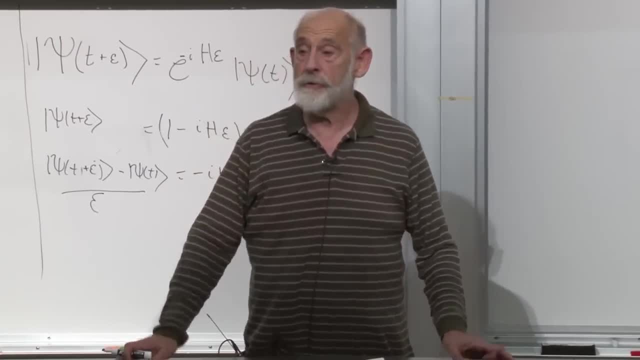 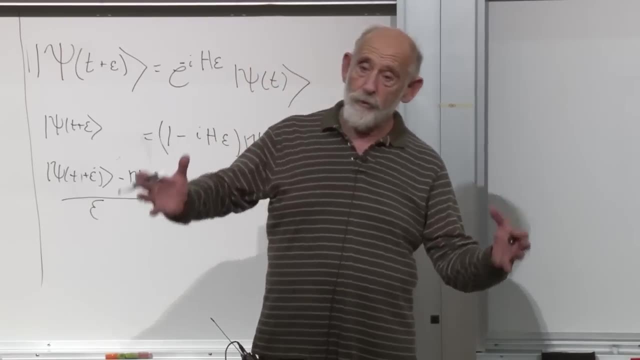 just to have something in your head. One of them is rotation symmetry, where it just says that if you take a system which satisfies a certain set of equations and you rotate it physically, rotate it physically, rotate it about an axis, you may or may not change it. 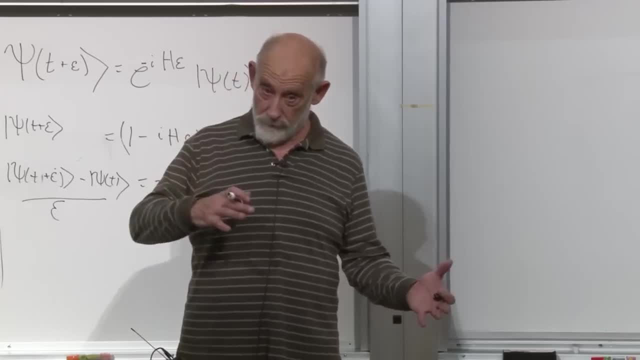 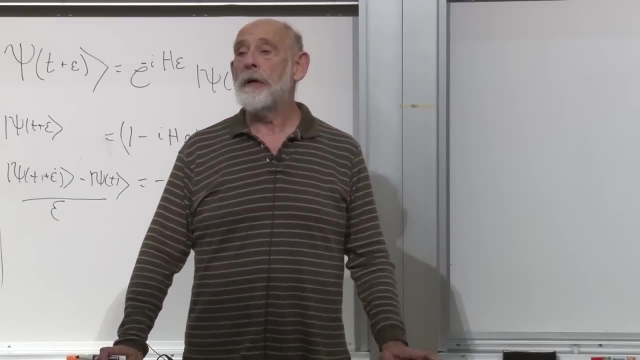 I can tell you this: If you rotate me, you'll change me, Right, Yeah, you will. If the Earth weren't here and I was in outer space and free space, then the Leonard equation, whatever the equation governing me is, 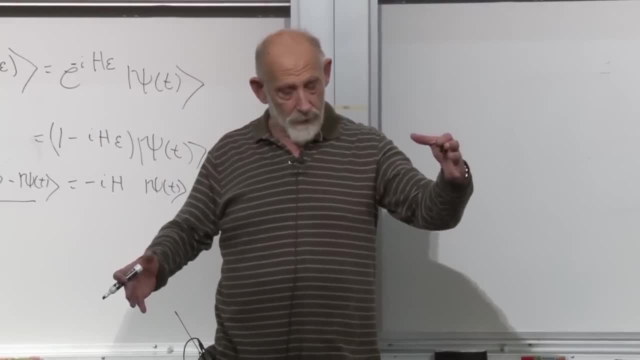 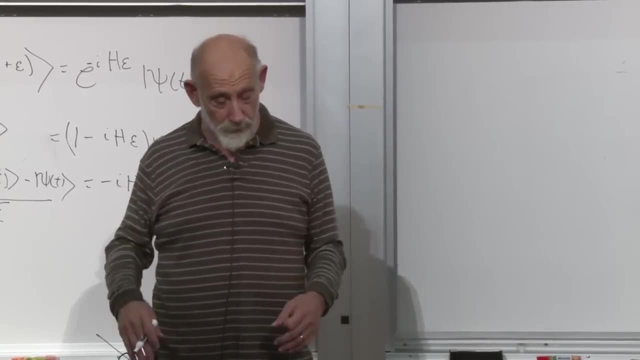 Would be the same for the rotated or the unrotated. Another way of saying it is: I couldn't tell whether I was rotated or not If you rotate me and then just go away. I can't tell that I was rotated because the equations that govern my metabolism, my internal structure and so forth are exactly the same. 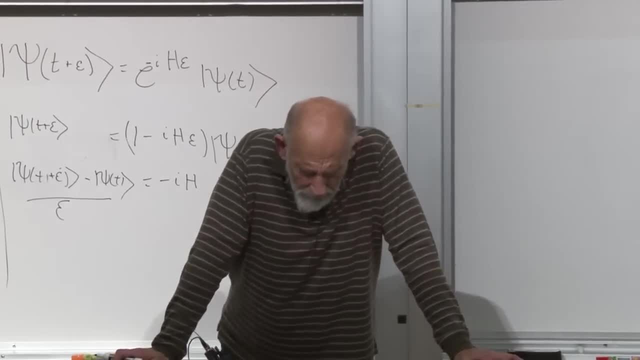 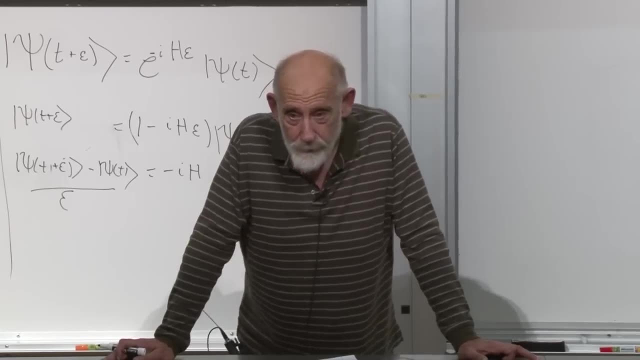 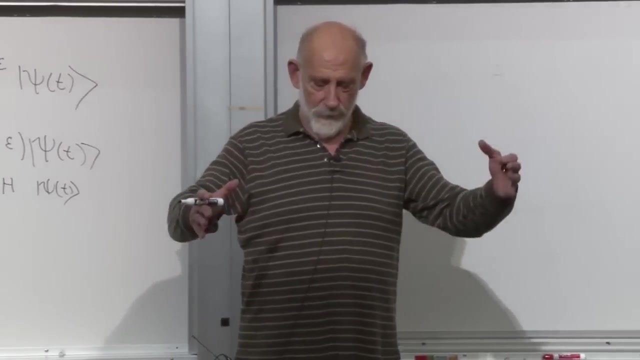 as had I not been rotated. Okay, so rotation symmetry is one example. Another example is translation symmetry. If you take me in outer space And you set me down and you say, how do I feel? I feel fine. You take the same state, but you translate me over by a meter and you ask me how I feel. 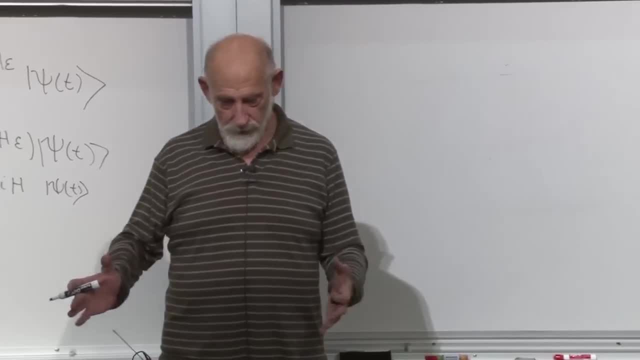 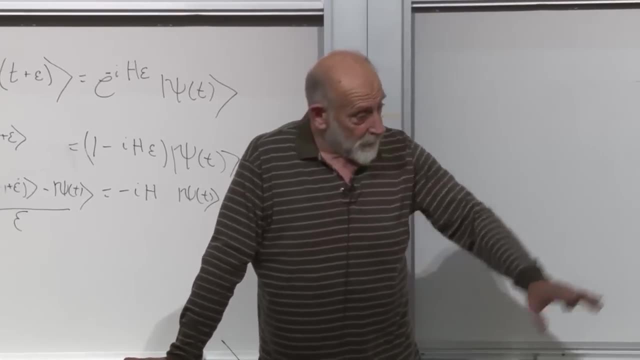 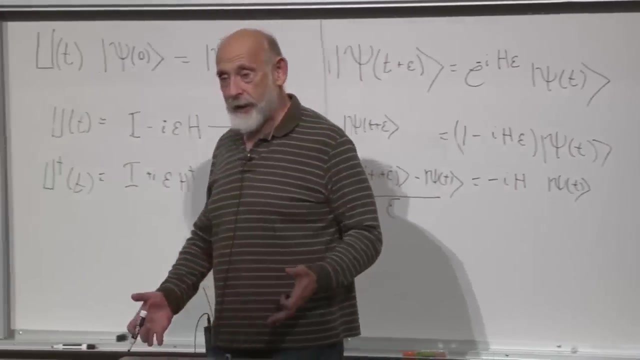 I say exactly the same as I felt before. It's a symmetry. On the other hand, there are situations where translations may not be a symmetry. If there was a furnace over there, a fire, hot fire, and you put me over here and you. 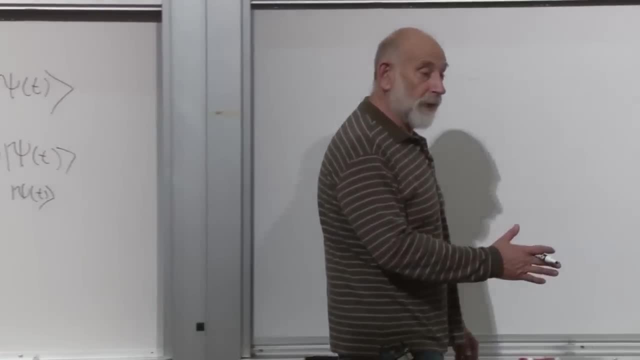 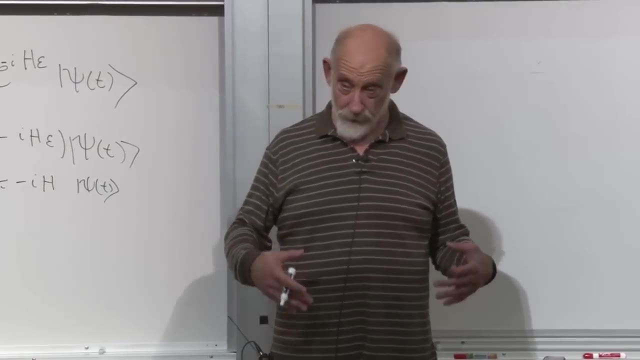 said: how do you feel? I feel fine. Now translate me over to here. How do you feel? Well, I don't feel so fine. So the presence of an object may break translation symmetry. On the other hand, if you think about it a minute, wait a minute. 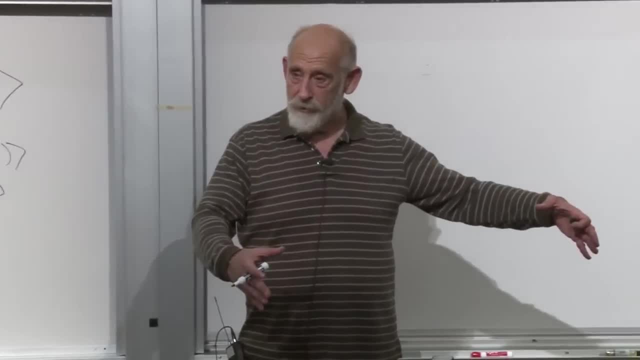 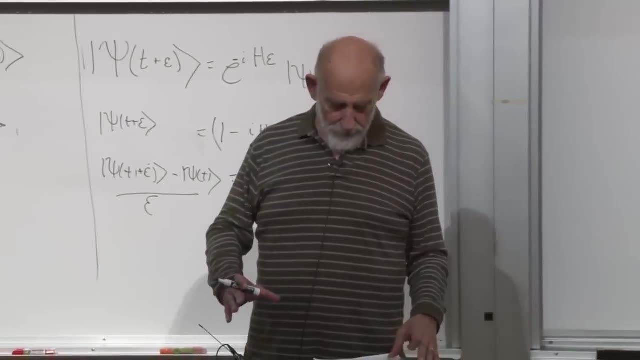 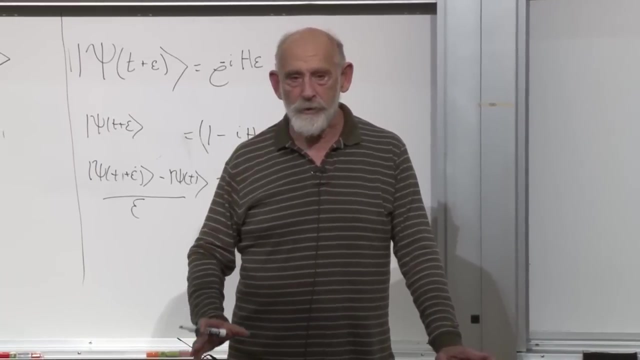 What if I really translate everything me and the furnace? Then we restore the translation symmetry. So symmetries are operations or there are operations that you can do on states of systems. Okay, And if the operation doesn't change the equations, doesn't change the properties, 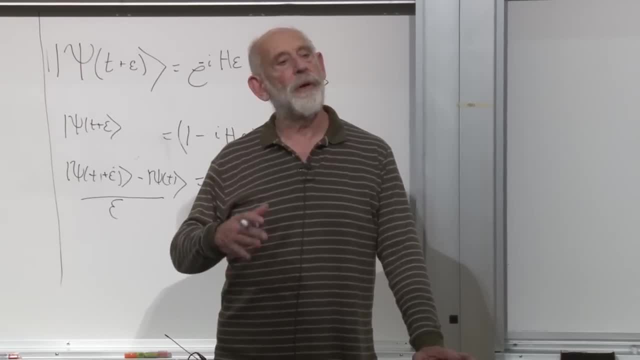 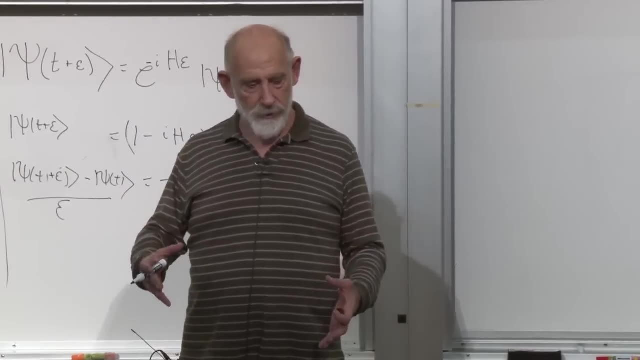 of the system doesn't change the way you describe the system, then that transformation is called a symmetry For a free particle, for any ordinary system, if it's out in outer space, far from anything else, and you translate it, that's a symmetry. 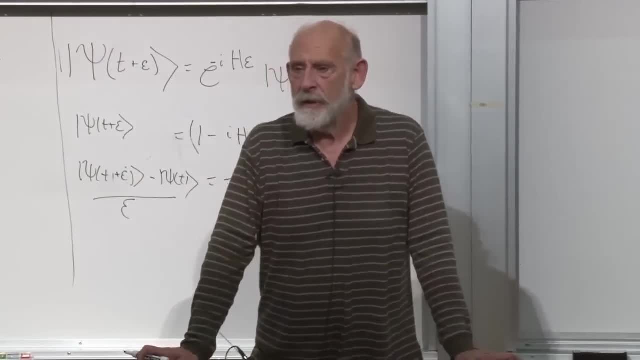 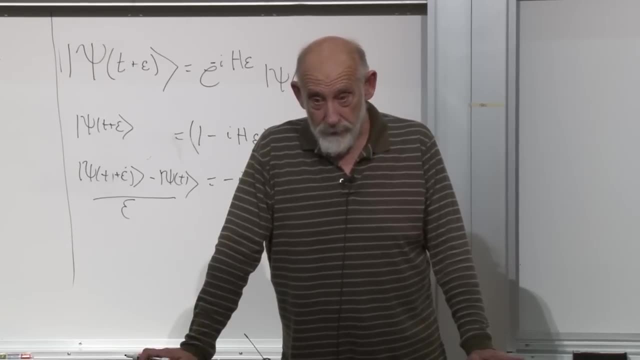 You rotate it? that's a symmetry. What if you squeeze it? Change its dimensions by squeezing it? That's a symmetry. That's a symmetry. That's a symmetry. That's generally not a symmetry. You know, if you take a crystal of rock, salt or something and you squeeze down on it and 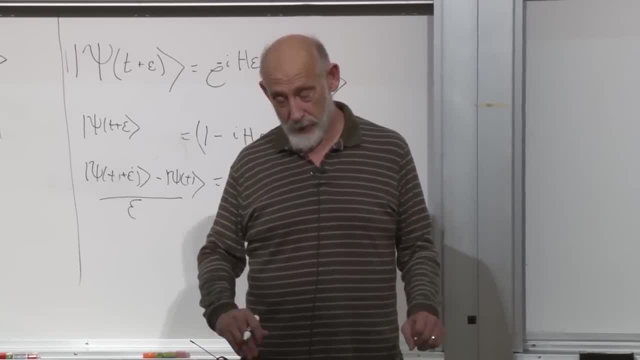 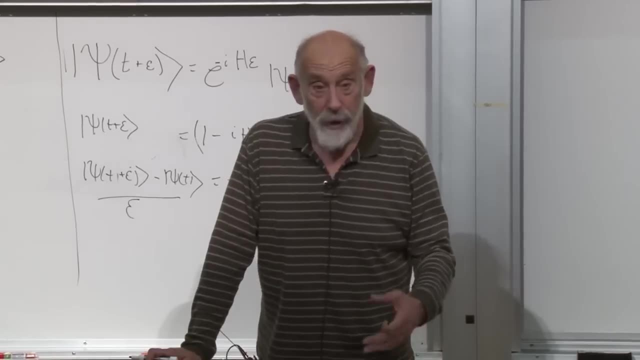 compress it by a factor of two, it doesn't behave the same way. So there are all kinds of things which are not symmetries. Nevertheless, they still may be operations that you can define, but they may not be symmetries. 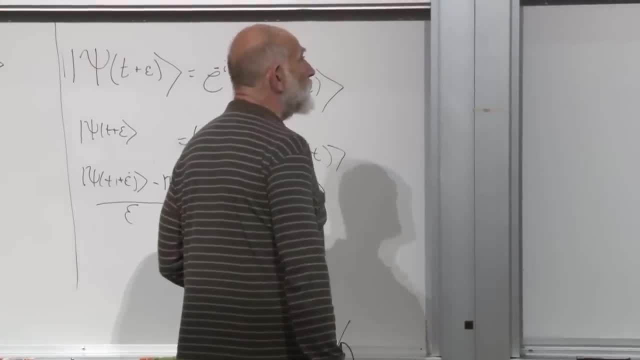 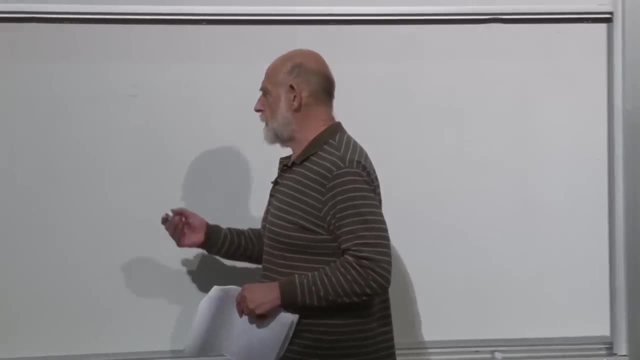 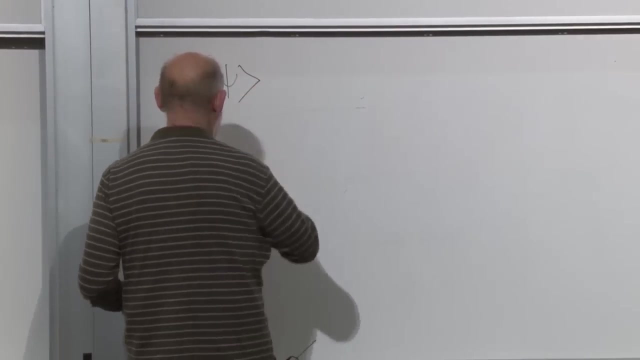 Okay, Let's talk about the condition. Let's first of all try to explain, Let's try to quantify that idea. We have states, Let's the generic or typical state of the system that we're interested in is called psi. We're going to do an operation on it. 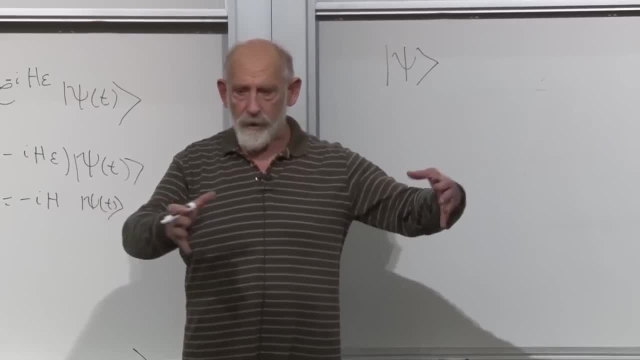 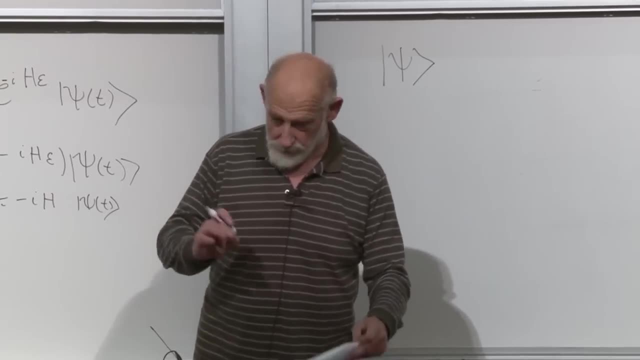 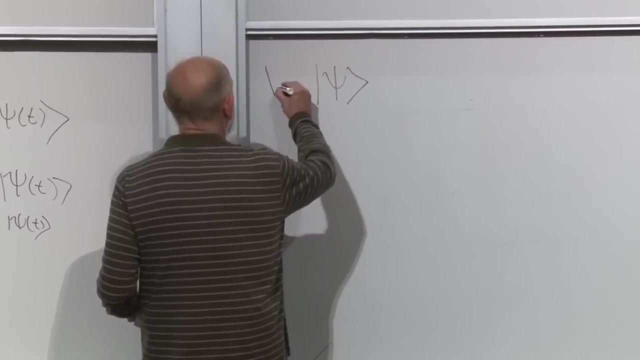 That operation might correspond to rotating the system, it might correspond to translating the system, or it might correspond to something uglier than that, like squeezing it or stretching it, but doing something to it. Okay, Let's represent that by an operator v. 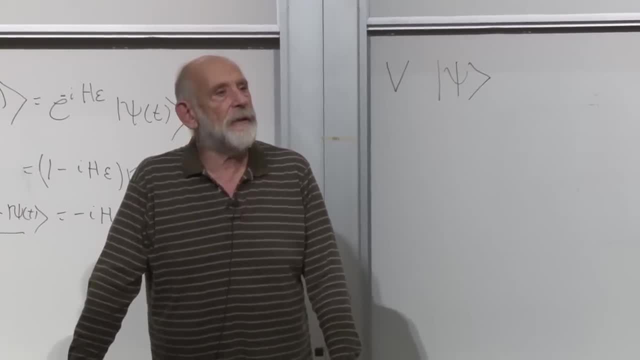 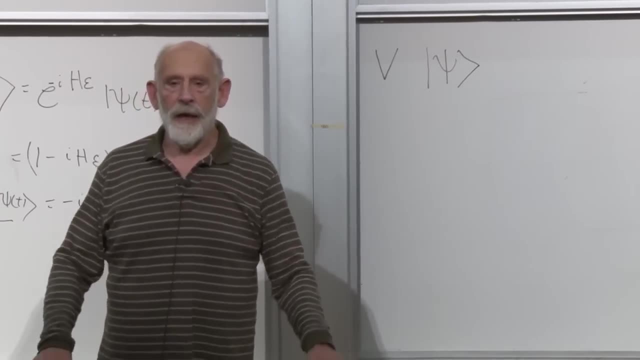 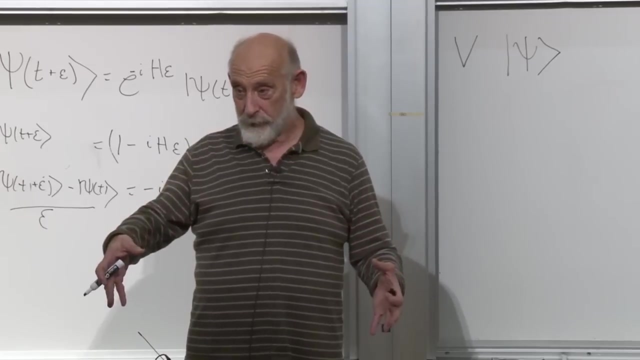 I use v because I've already used u, but I intend it to be a unitary operator. Why a unitary operator? Well, if I really have a symmetry and I have two states which are different than each other, I apply the symmetry operation. I expect them to stay different. 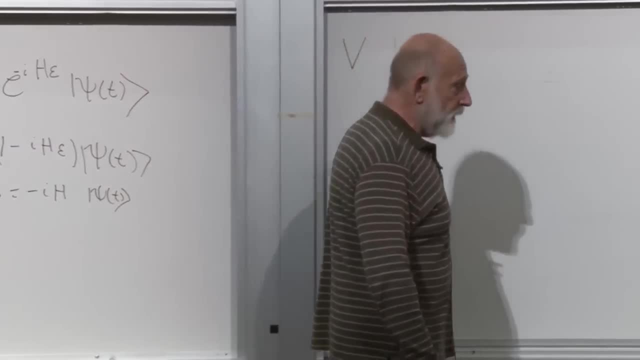 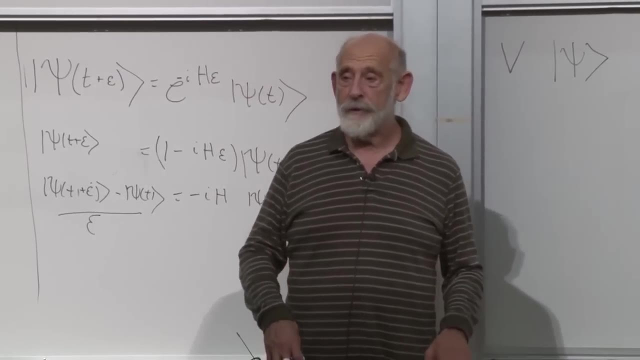 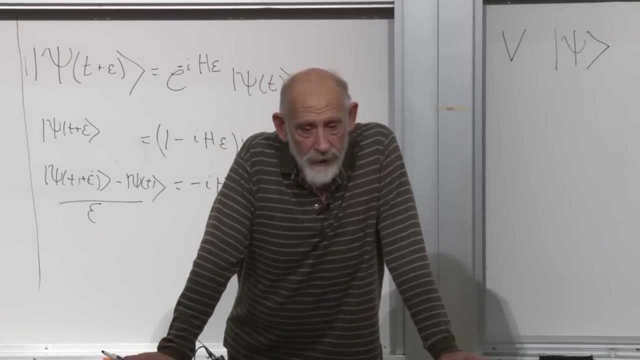 If there are two states of of me- happy me and sad me. they're different from each other, they're observably different. there's a there's an observable that you can measure the happiness operator, and they're different. 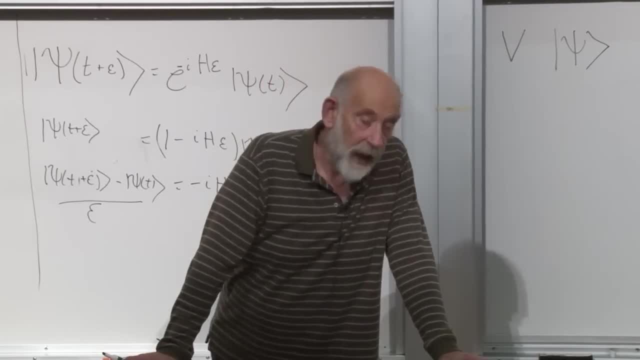 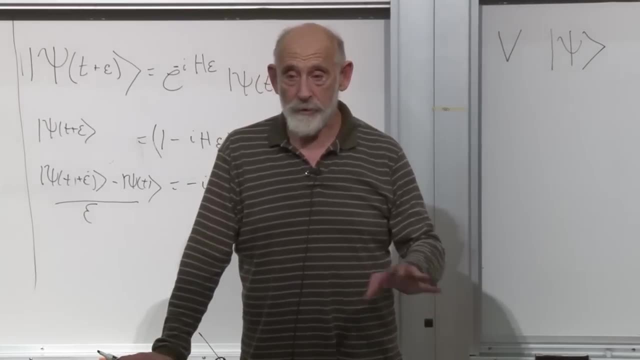 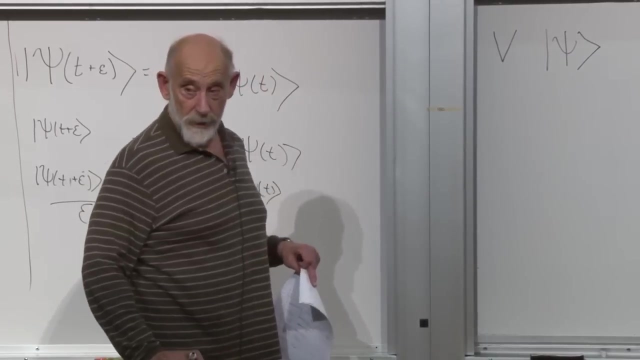 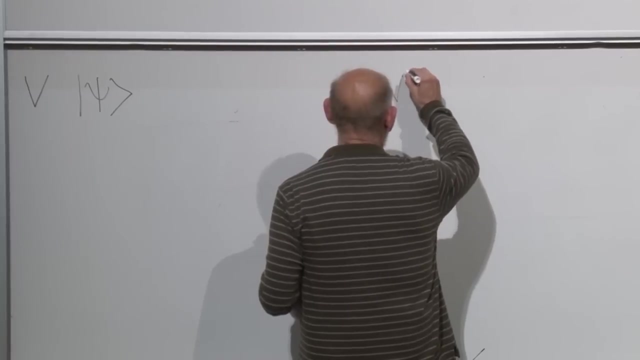 If you then rotate the state out in outer space, the distinction should remain. So that means that orthogonal states should remain orthogonal when you do a symmetry operation, and that says that the operator v should be unitary, So v is unitary and it represents v equals v, dagger, v equals 1.. 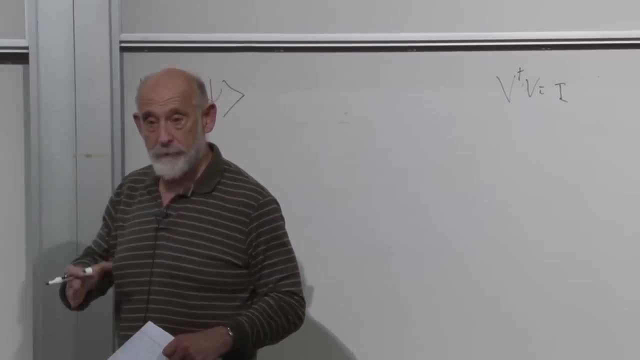 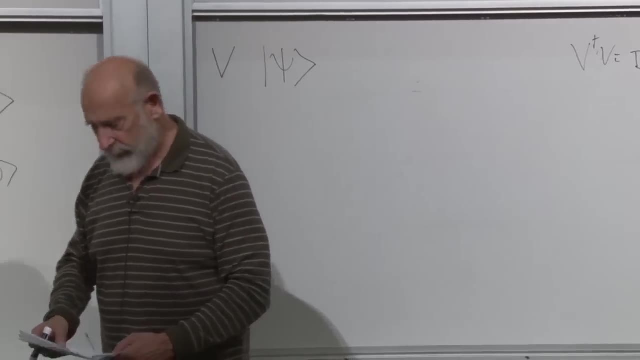 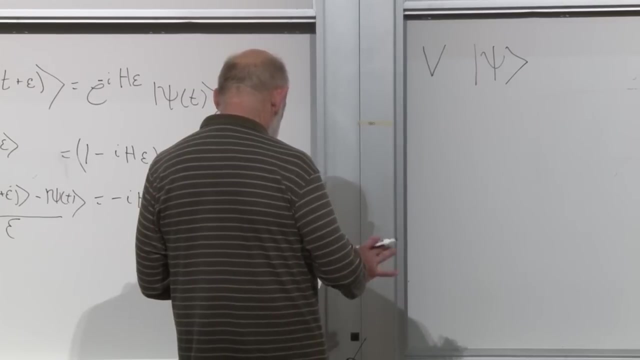 I don't use u because I'm saving u for the special case of time translation of evolution. Okay, Now let's suppose. Yeah, This is a little bit tricky, So we'll: There's u's and there's v's and it's. 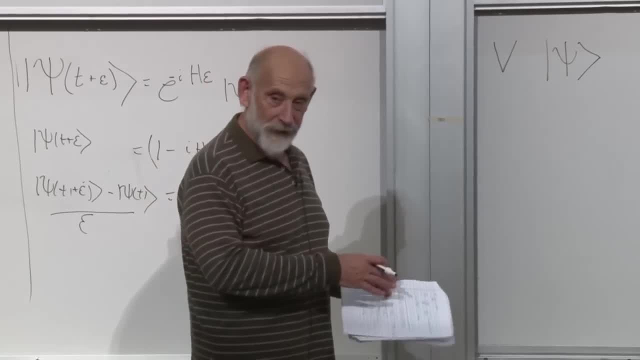 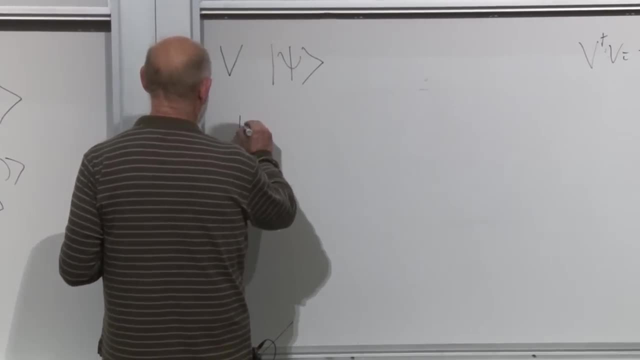 it's quite tricky. It takes me half an hour each time I try to do this to get it right, but it's also very, very simple. Okay, Let's suppose that a wave function or a state vector. I'll use them interchangeably. let's. 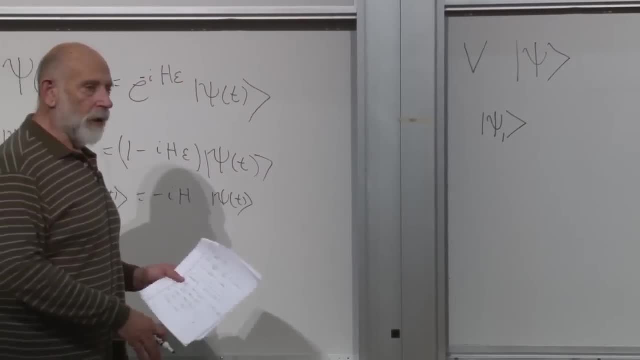 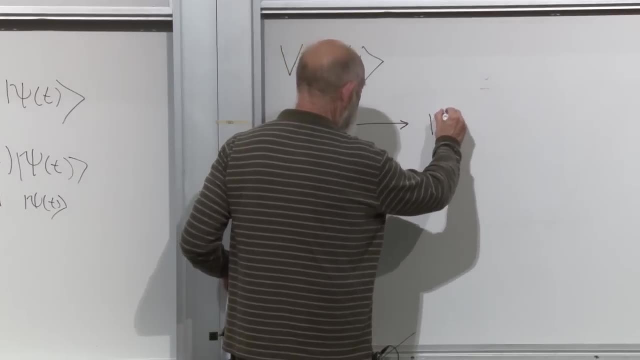 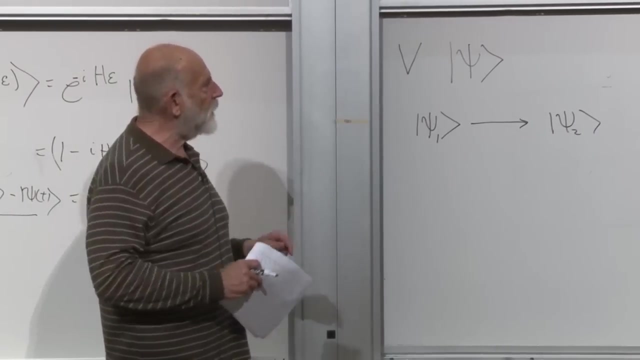 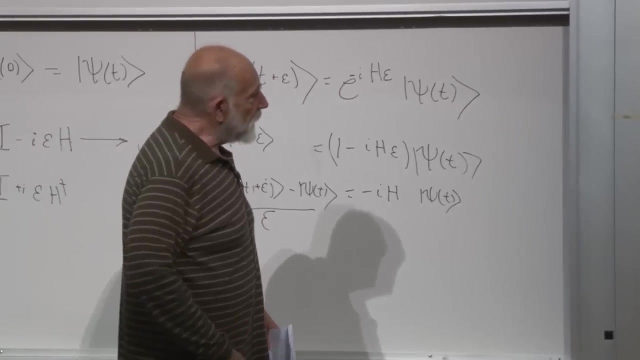 call it psi 1.. Under time evolution. Okay, So psi 1 becomes psi 2.. If I take psi 1 and I allow it to evolve with time, let's represent that by putting a little u here. U represents time evolution. 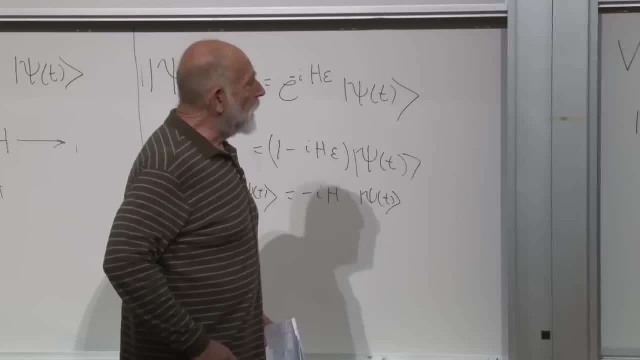 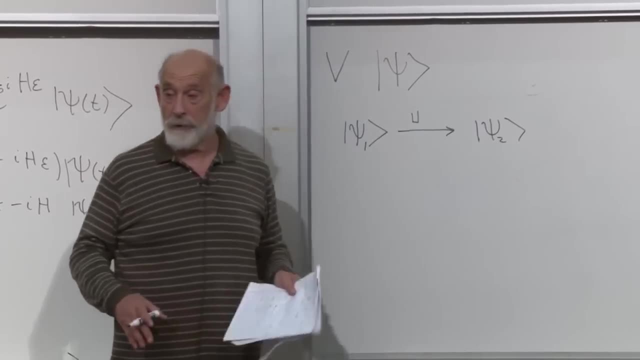 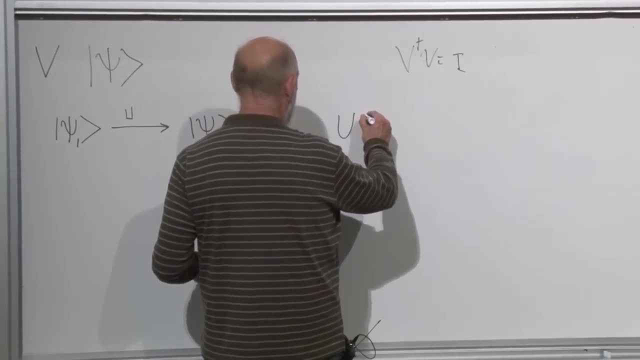 V does not. V is something else, And if I take psi 1 and allow it to evolve for a certain amount of time, it will become psi 2.. Okay, So that's under u. Another way to say that over here is that u on psi 1 is equal to psi 2.. 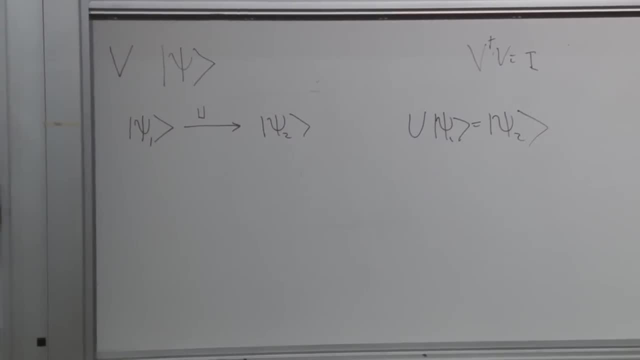 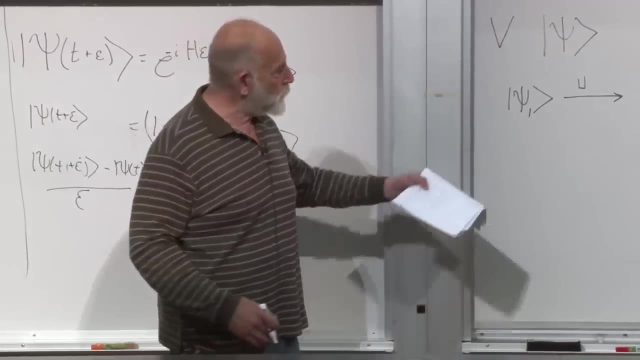 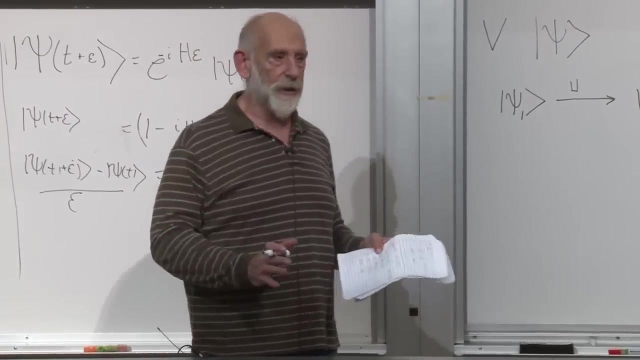 That's all: Evolve psi 1 for a little bit of time and you get psi 2.. Okay, Now let's imagine the transformed version of this. Transformed, it could be by rotation, it could be by translation, by some symmetry operation. 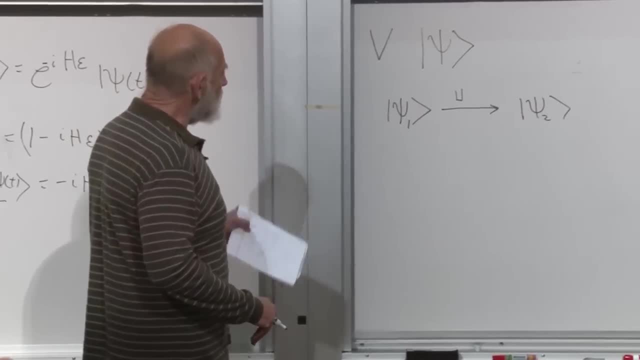 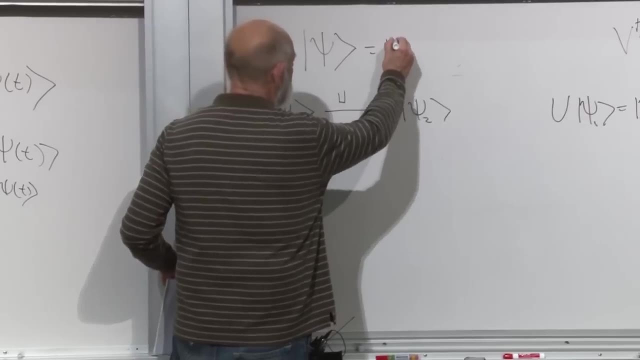 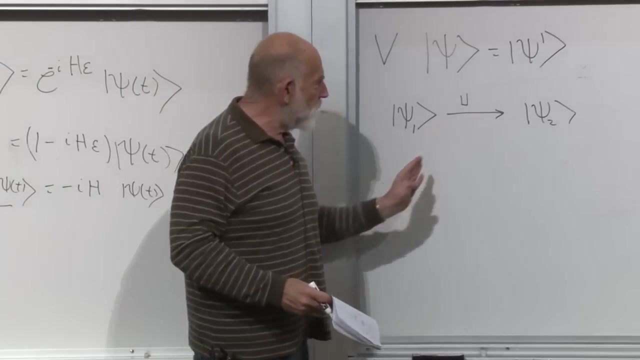 What does this equation say for the transformed things? Well, let's call this, let's call this psi prime. Now, there are too many. let's keep in mind exactly what's going on here. 1 and 2 represent some initial state and some final state. 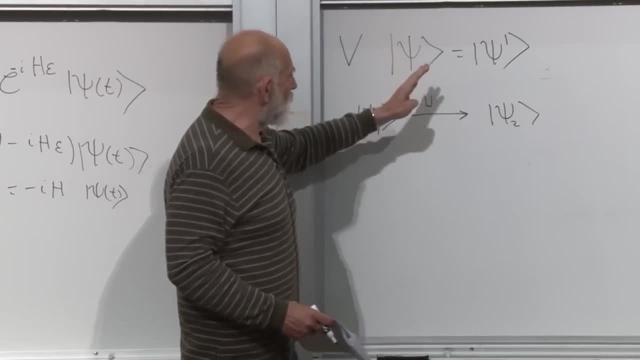 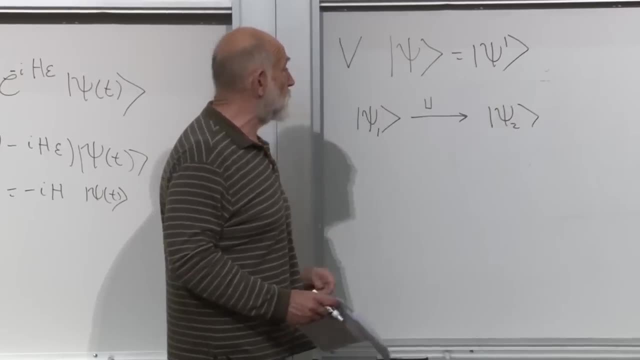 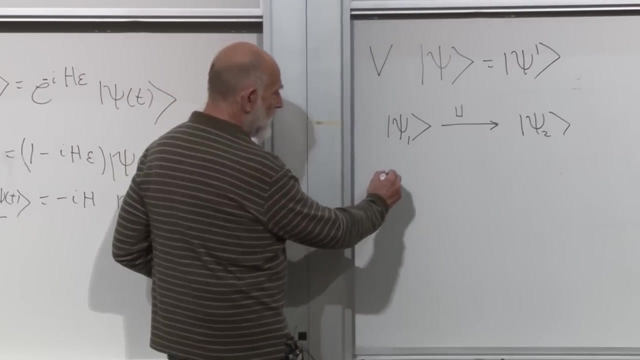 Evolution from one to another. Prime and unprimed represent the action of the symmetry operation, which could be rotation, Could be rotation or it could be translation. Okay, Here's what I maintain. If there really is a symmetry, then psi 1 prime. 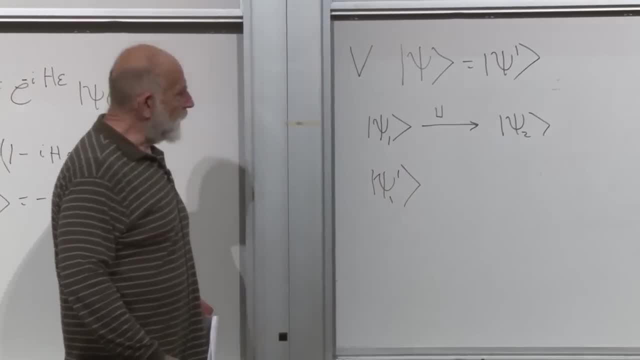 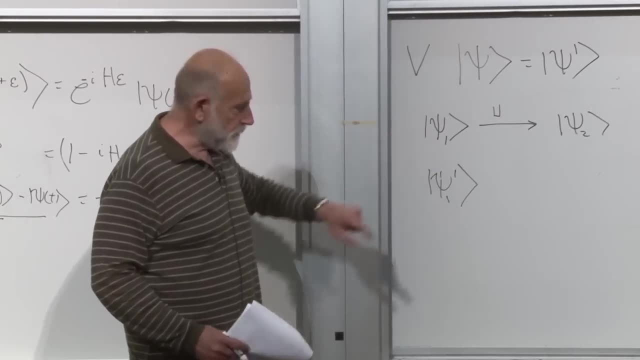 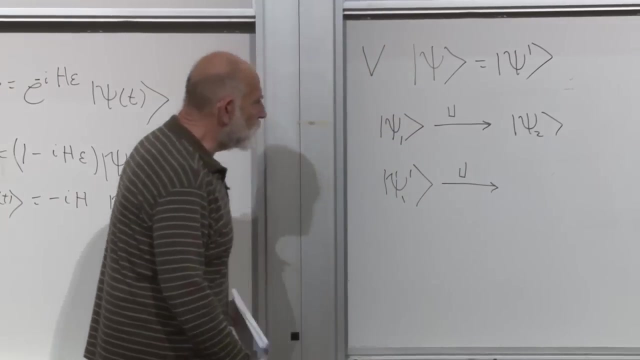 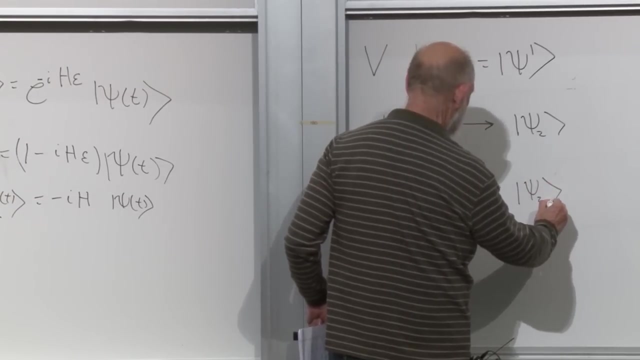 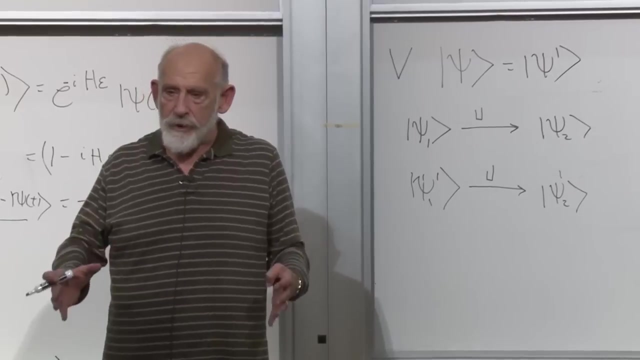 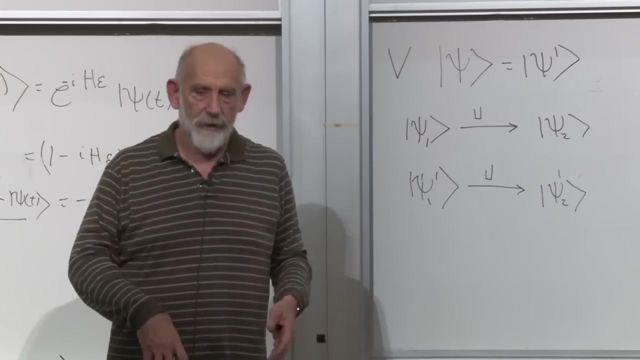 If we were talking about rotations, then psi 1 prime is just the rotated state of psi 1.. Psi 1 prime will evolve to: 2. The rotated version of psi 2.. Let's see what that says. Okay, If I evolve myself over a period of time and I'm in some state and I get some other state, I go from happy to not so happy. 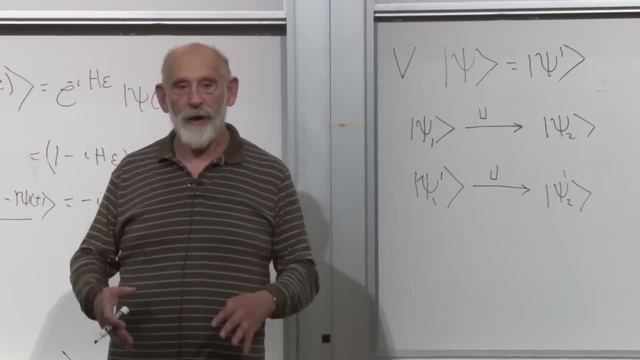 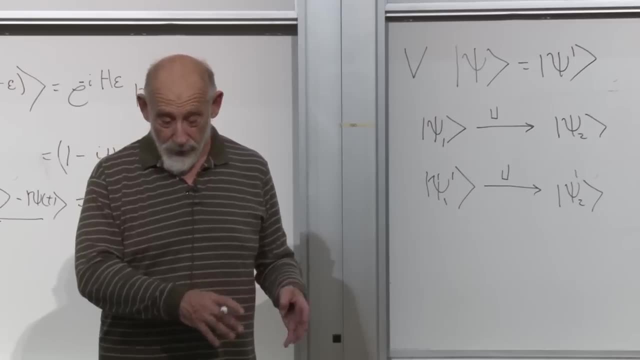 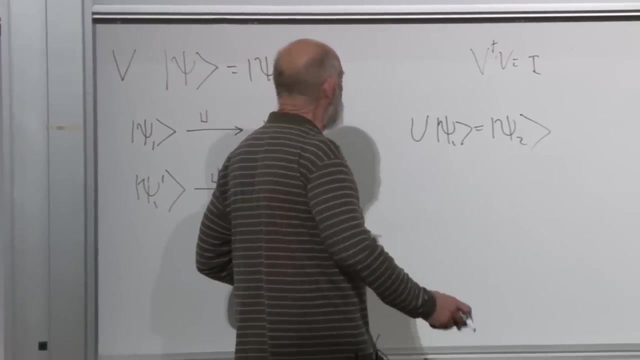 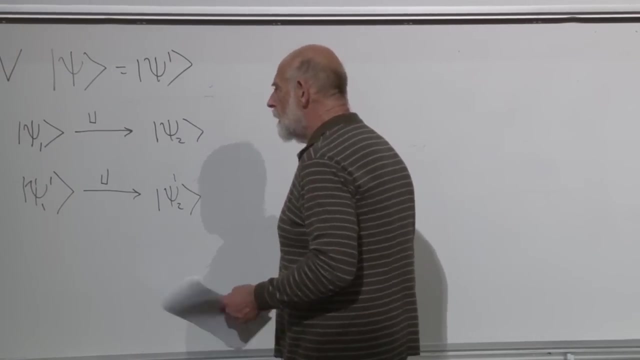 Then when I rotate myself, I should also find, under the same evolution, that I go from the rotated happy state to the rotated not so happy state. That's what it really means to have a symmetry: That the evolution of the transformed state behaves the same way as the original state. 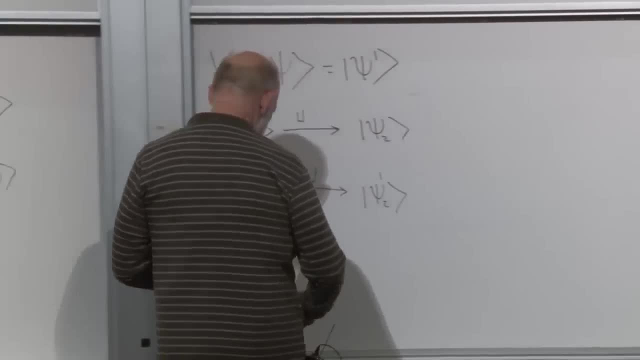 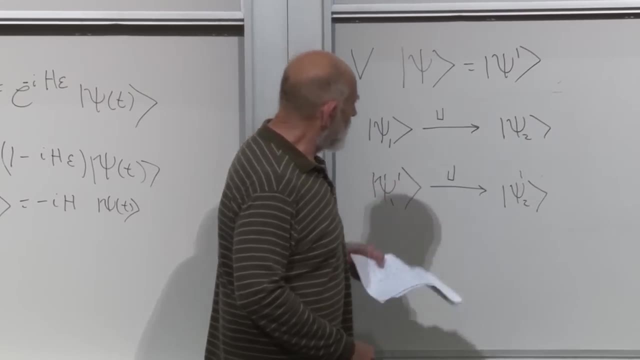 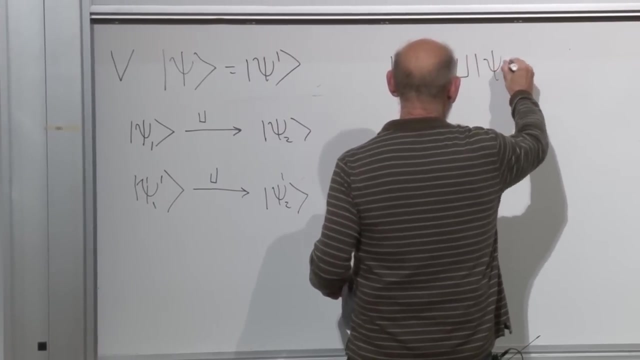 It's a little bit tricky. Okay, Let's see if we can make an equation out of this now. Yeah, Yeah, Okay. So the first row here is just the equation that psi 2 is u psi 1.. That's what this says. 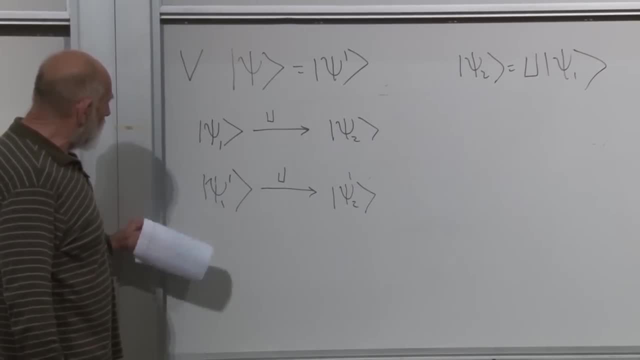 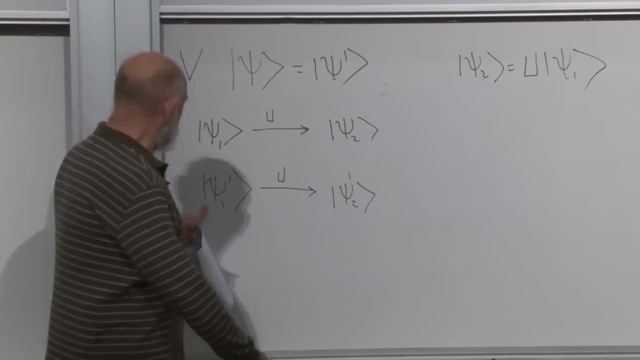 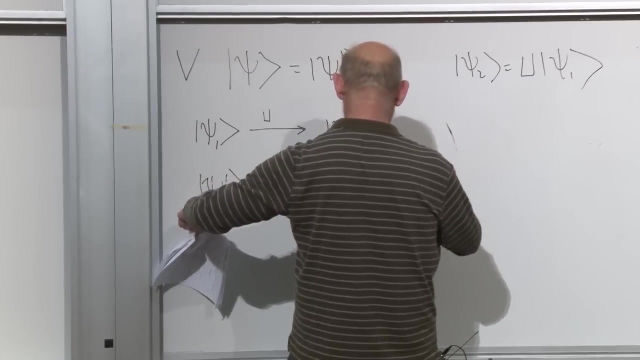 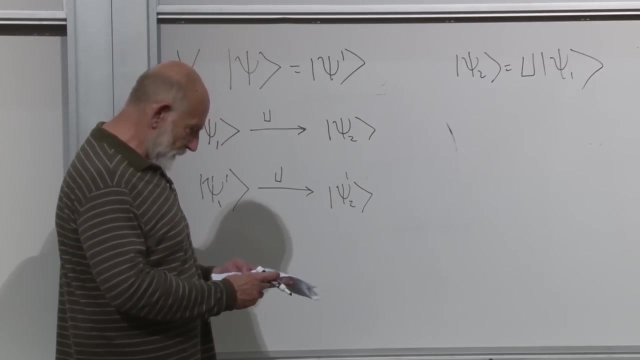 The second equation. let's go to the second equation. To go from unprimed to prime, you multiply by v. So the second equation here says that v. It says that. I'm sorry, This always confuses me, Ah. 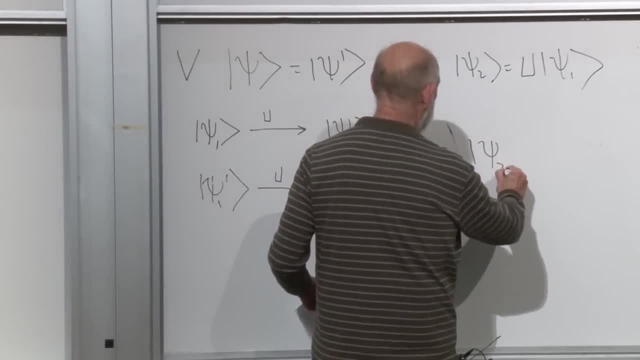 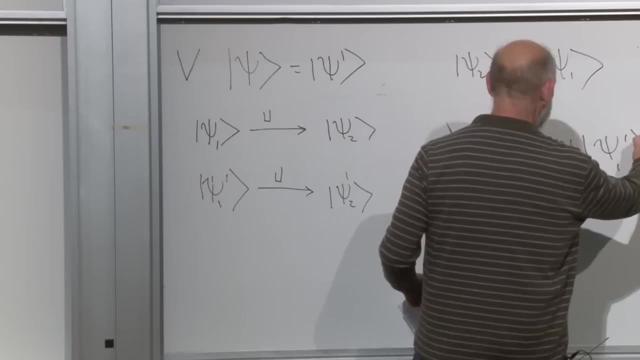 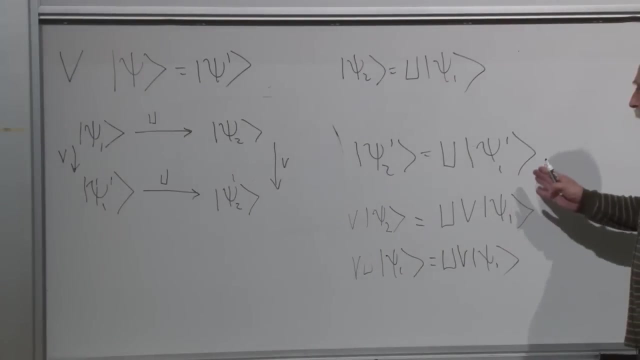 It says that psi 2 prime is equal to u times psi 1 prime. To go from 1 to 2 is time evolution. To go from unprimed to prime is v, is the symmetry operation. All right. So psi 1 prime is v times psi 1.. 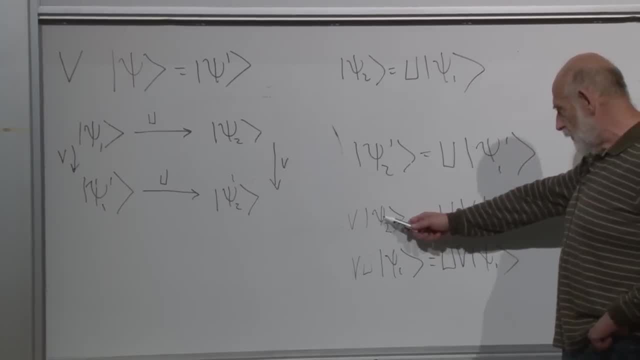 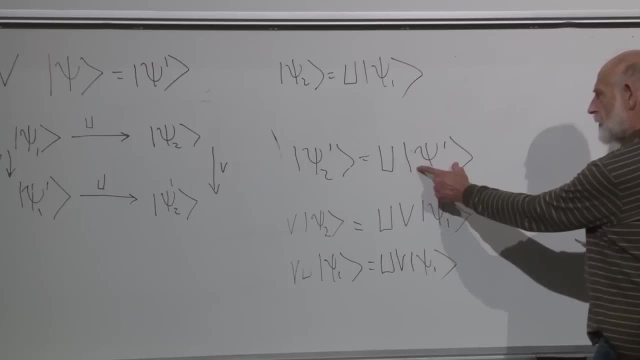 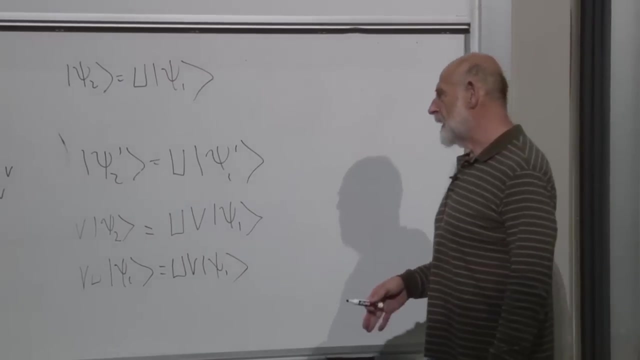 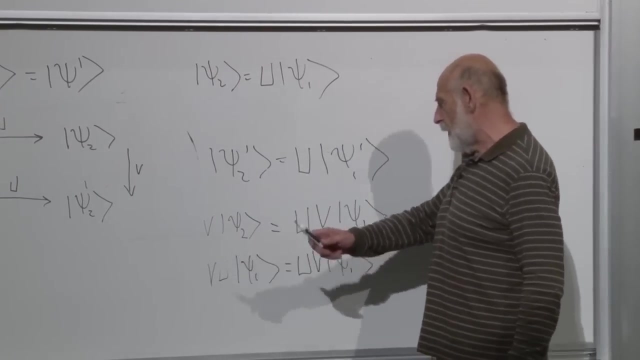 All right, So we have uv times. psi 2 is u times psi 1.. Times psi 1 prime and psi 1 prime is v times psi 1.. Okay, That's the right-hand side. The left-hand side is v on psi 2, but psi 2 is u times psi 1.. 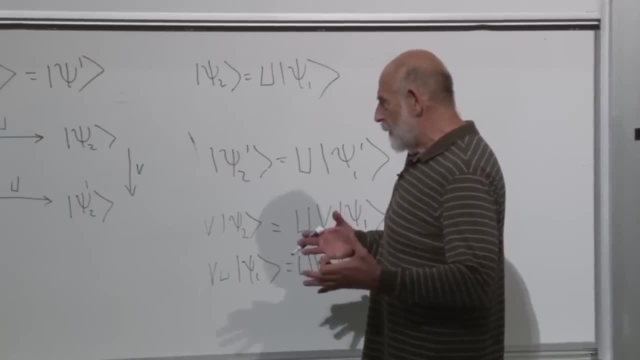 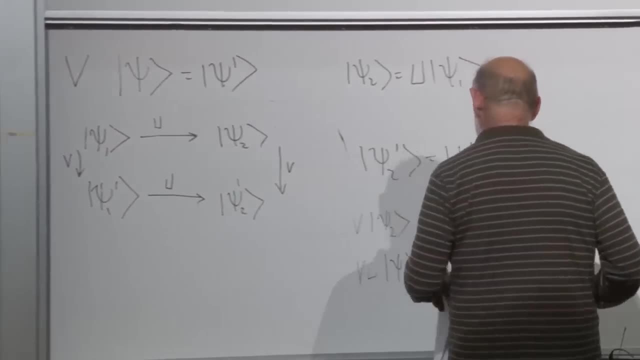 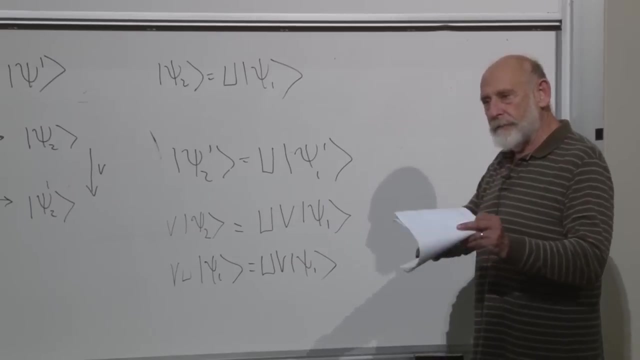 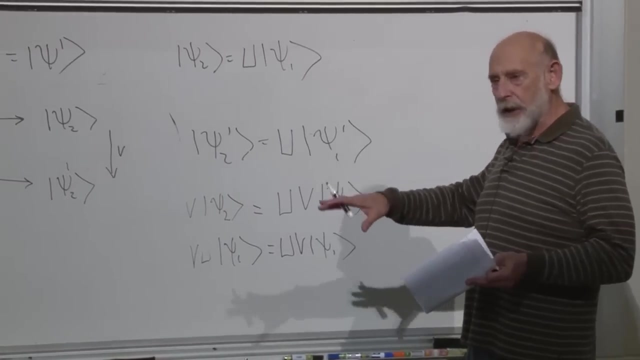 So, after perpetual confusion that has It stumps me every time. I try to do this on the blackboard. What it says is that if a thing is a symmetry, in other words, if it preserves the way evolution takes place, if it's a transformation which preserves the time, relationships between vectors. 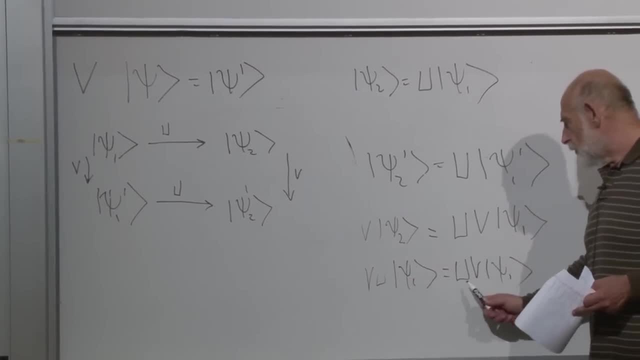 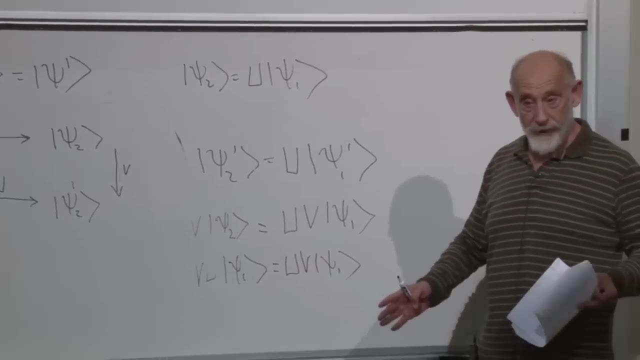 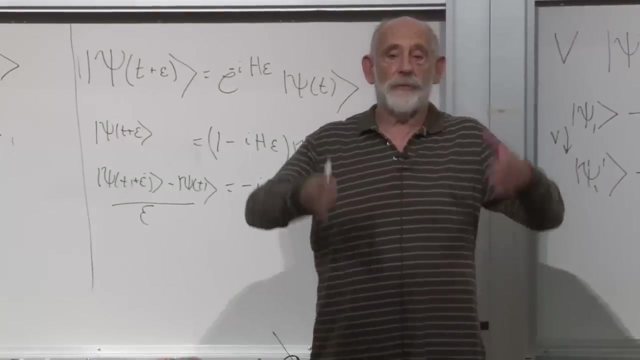 then it says that v times u must be equal to u times v. This, of course, must be true for every state if it's to be a true symmetry of nature. A true symmetry of nature. rotation symmetry, for example, is not something which only applies if I'm standing vertically upright. 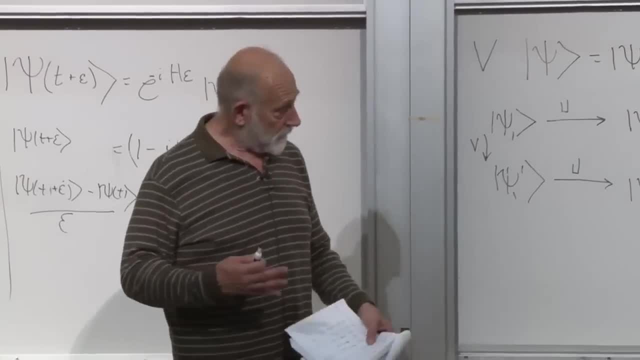 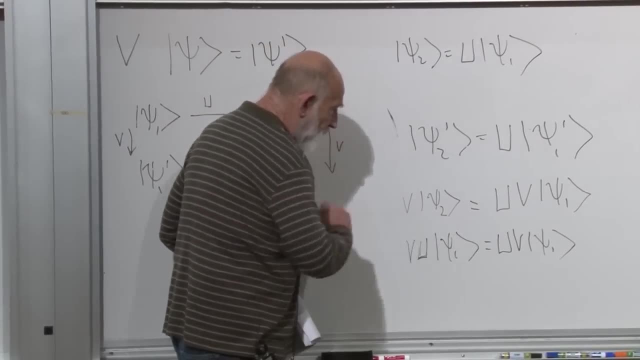 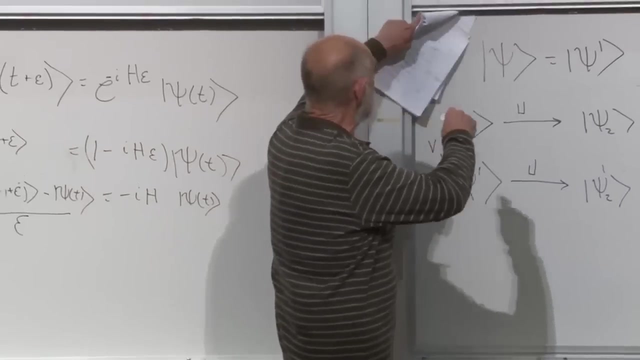 It should apply to any particular state of the system. And so if v times u on any psi 1 is equal to u times v on any psi 1, what it says is that symmetries of nature are such, they're operations, they're v's. 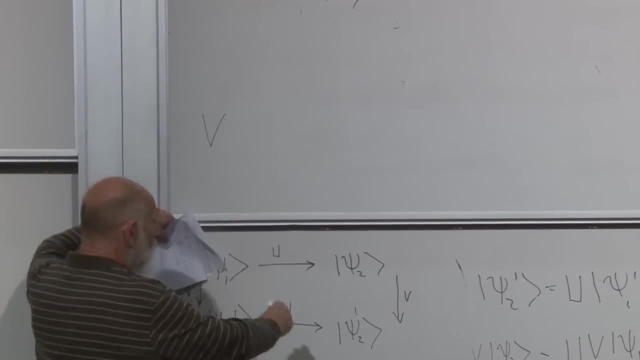 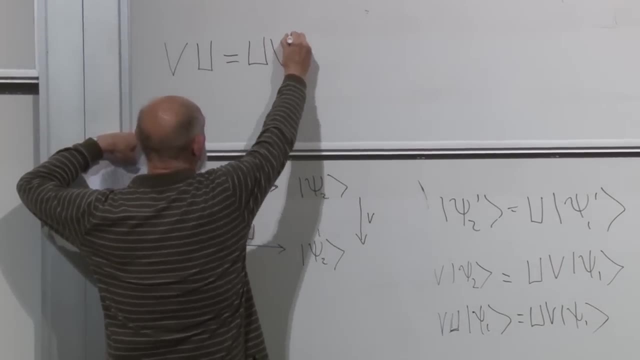 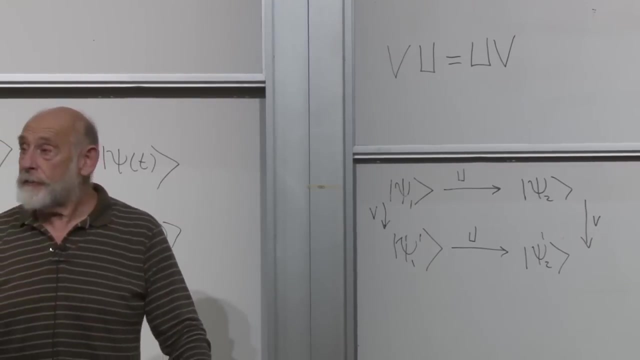 unitary operators which commute with the time evolution operator For all, For all, For all, Yes, in fact, for all time. We'll see. it's enough for it to be true for one time and it will be true for all time. 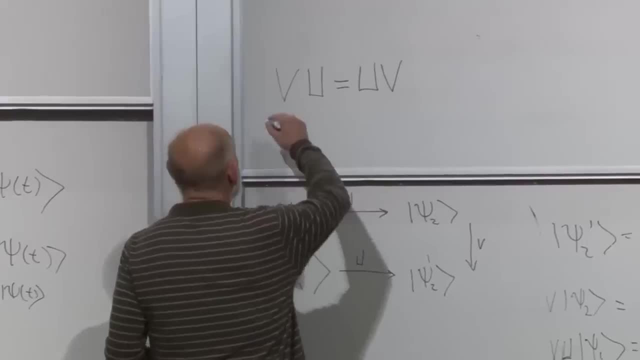 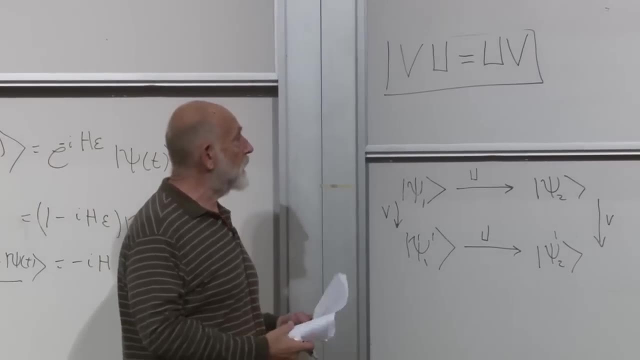 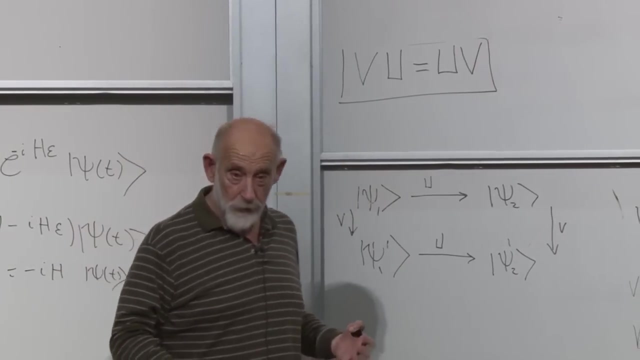 But yes, that's correct. Okay, So unitary operations, things you can do to the state vectors which preserve orthogonality, which commute with the time evolution operator, are symmetries that preserve the evolution, the evolutionary relationships. 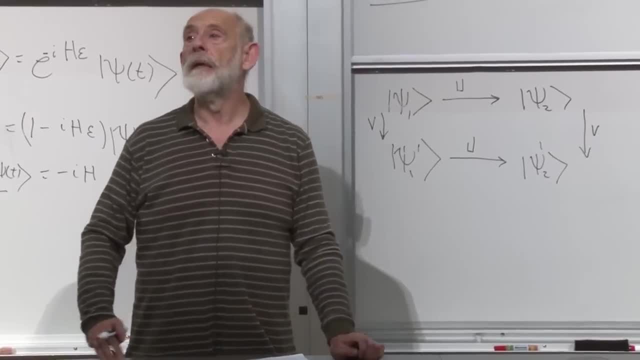 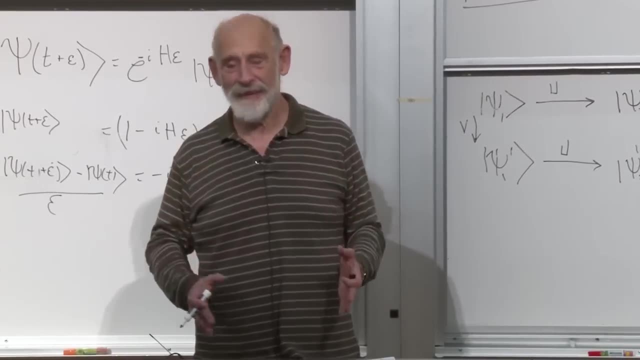 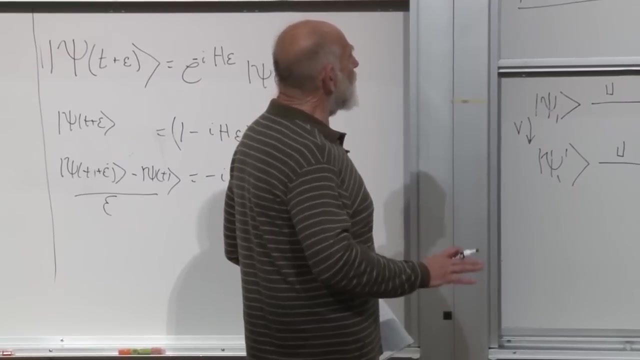 So physically, you're saying: you can rotate and then wait, or you can wait and then rotate, Exactly. The words are very simple and they make perfect sense And yes, that's exactly what it says. Okay, So how do we identify symmetries? 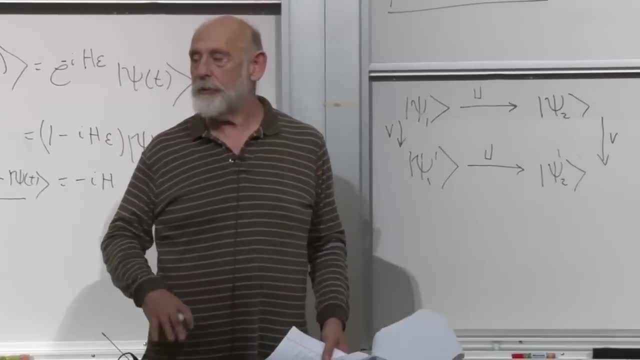 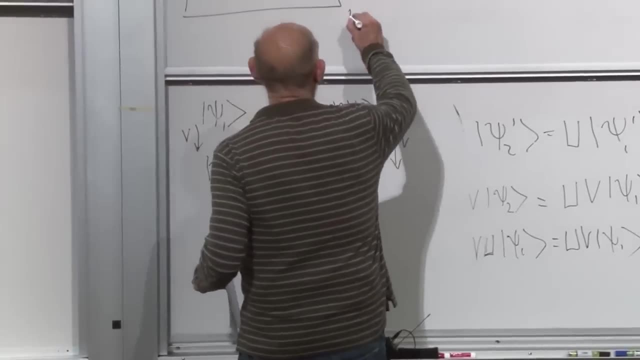 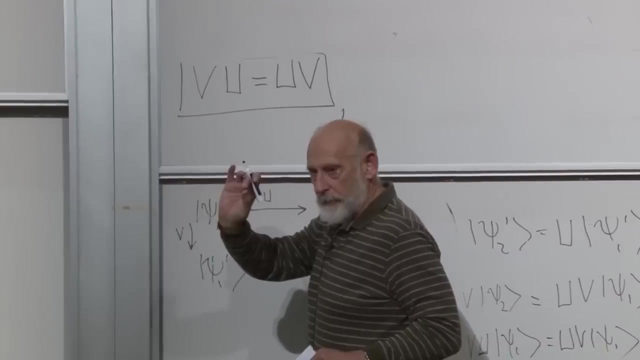 We look for operations which commute with the time evolution operator. Now, remember that the time evolution operator is itself. Let's take the limit of a small time evolution just to analyze it a little bit. This says Well, first of all, 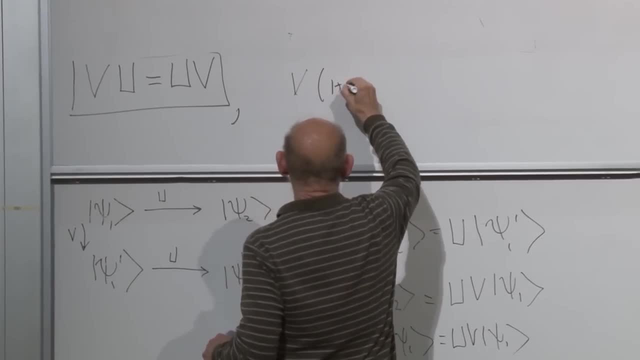 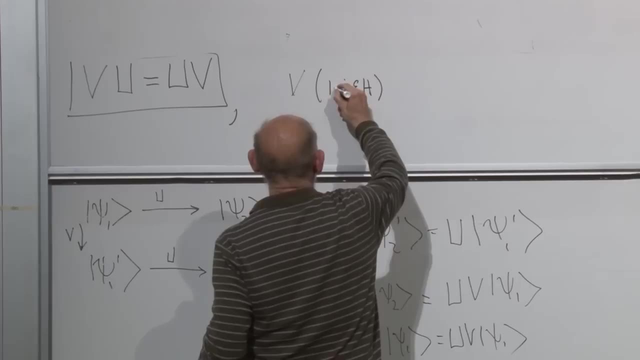 Yeah, okay, It says that v times 1 plus i epsilon 8,, 1 plus i epsilon h, 1 minus i epsilon h, 1 minus i epsilon h is equal to 1 minus i epsilon h. this is the first order again. 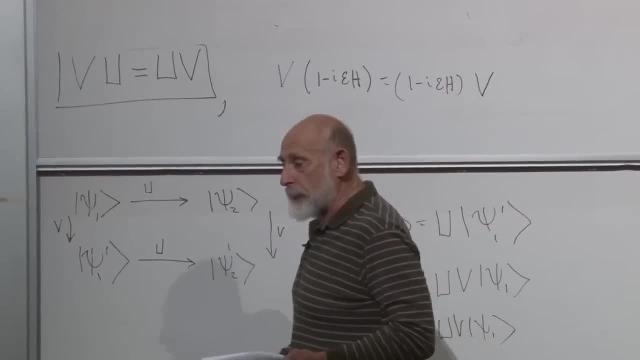 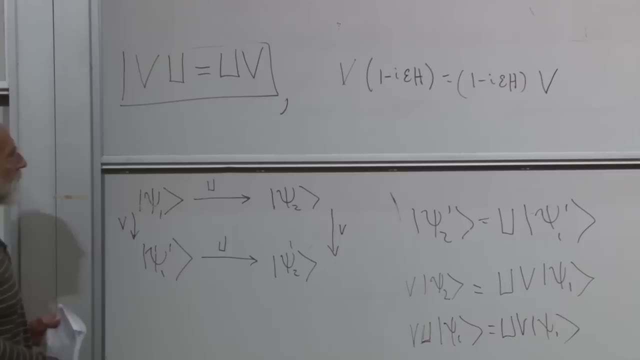 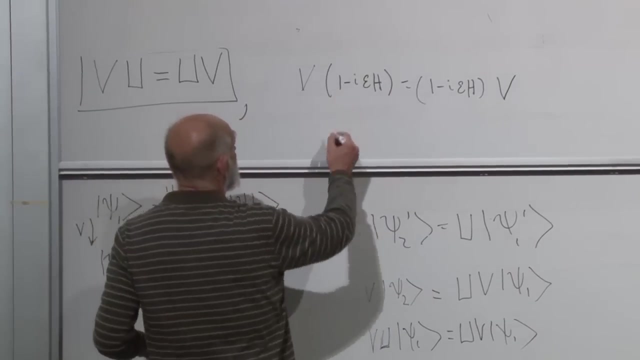 times v. I'm just expanding it out. The first order is good enough. It gives us everything we really want to know. First of all, v times 1 is equal to 1 times v, so those cancel, And what it says is that minus i, epsilon v, h. 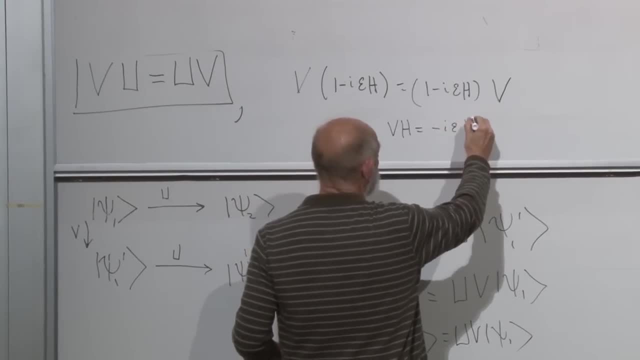 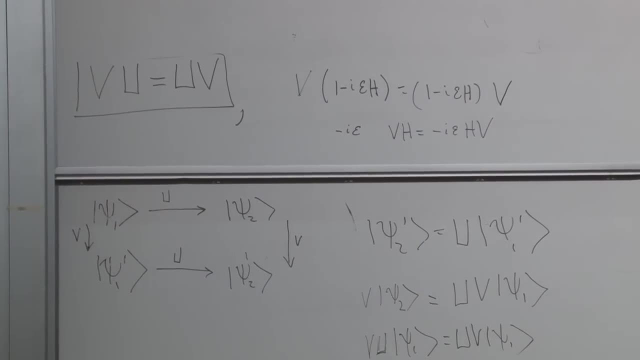 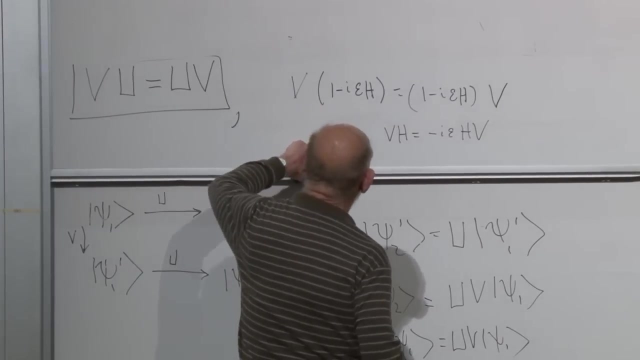 equals minus i epsilon, h v. Well, canceling out the minus i epsilon, it says that v commutes with the Hamiltonian. Okay, Let's cancel out these things. the minus i epsilons. a symmetry is a unitary operation. 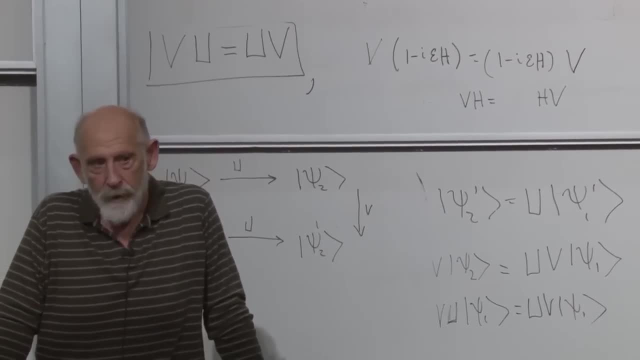 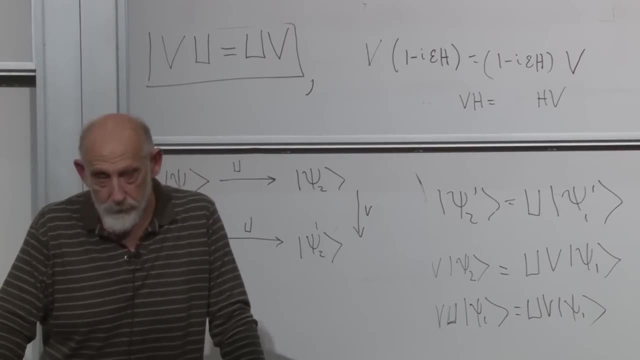 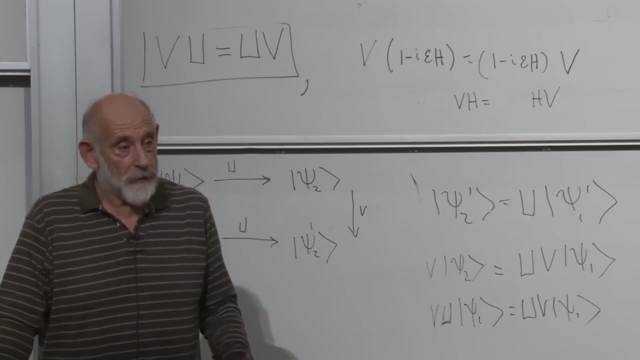 which commutes with the Hamiltonian. Any unitary operation which commutes with the Hamiltonian is a symmetry and any symmetry is a unitary operation which commutes with the Hamiltonian. That's very abstract. That's extremely abstract, and in order to appreciate it, 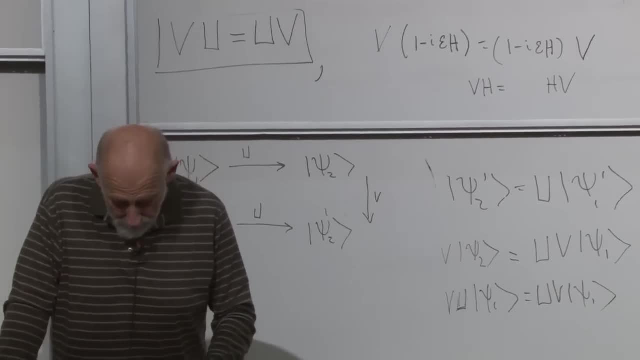 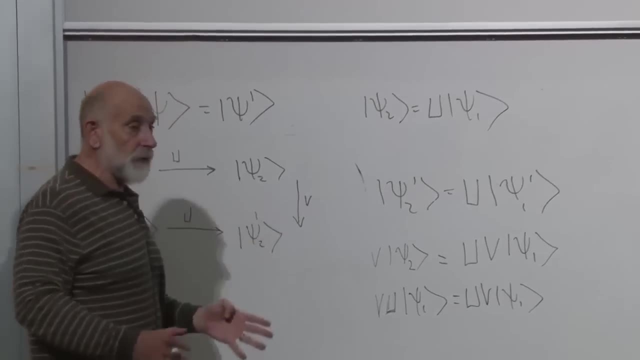 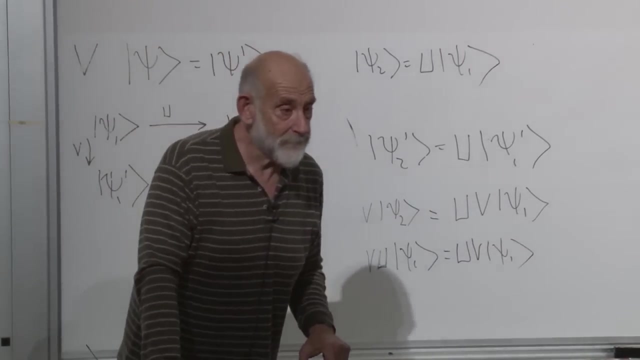 we have to do a couple of examples. We'll do some examples in a moment, but let's just focus on that- that unitary operations on the space of states which commute with the Hamiltonian are symmetries. What limited v to being unitary? 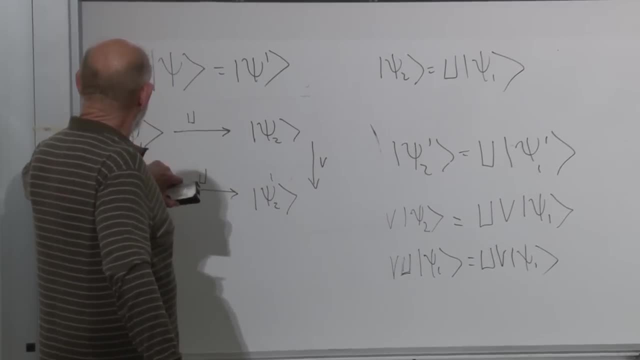 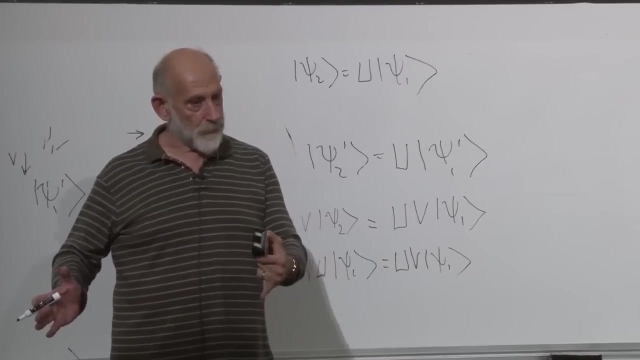 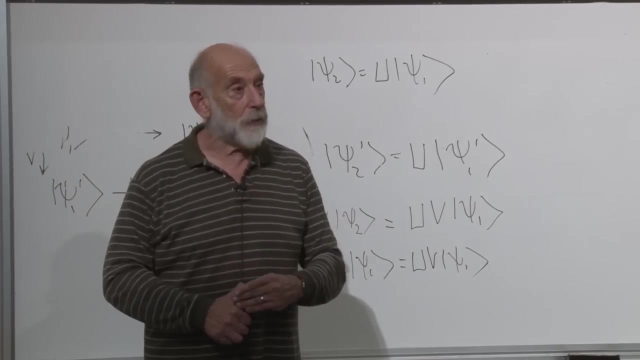 What limit? Sorry, What required? that v is unitary. Oh yeah, A symmetry. whatever a symmetry is, it preserves logical relationships between the vectors. So it's an assumption. It's an assumption that the symmetries of nature take orthogonal states to orthogonal states. 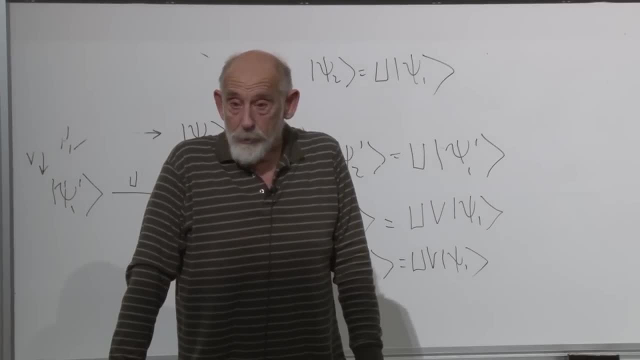 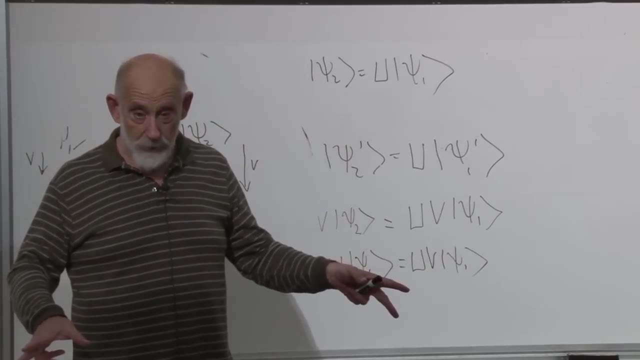 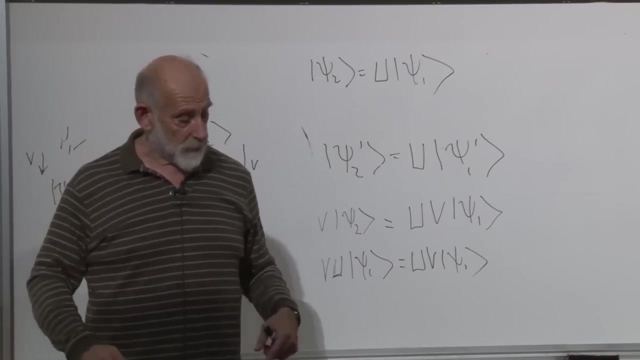 Okay, That seems plausible. A symmetry should not take two states which are distinctly different from each other and act on them to give states which are not distinctly different from each other. You wouldn't call that a symmetry, You could say mutually exclusive. Yeah. 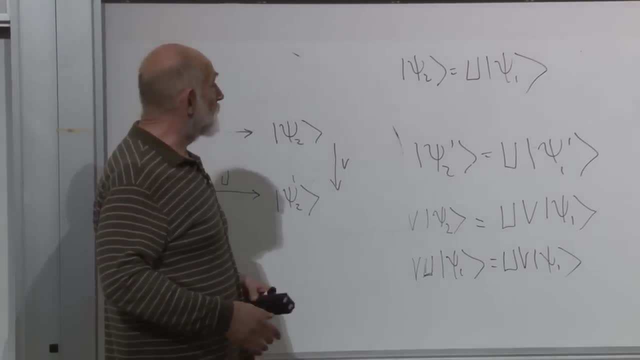 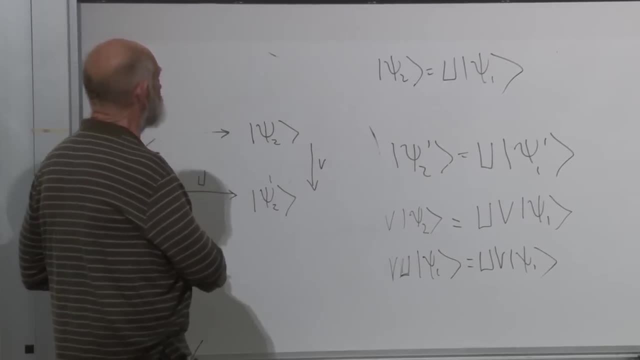 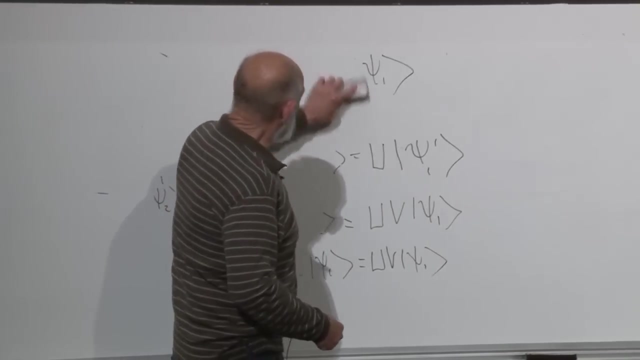 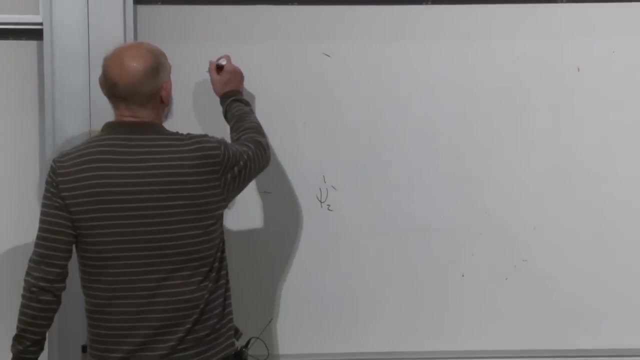 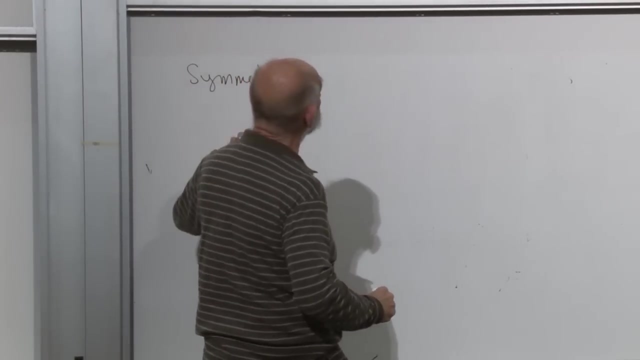 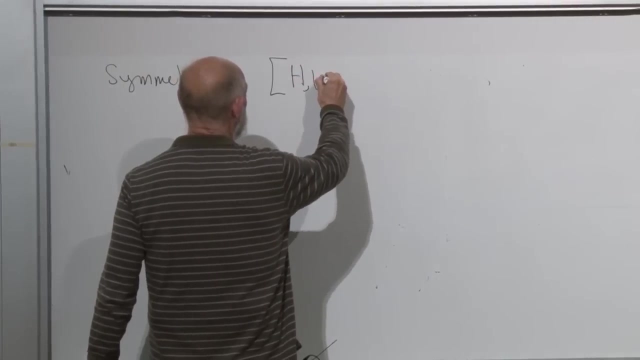 Mutually exclusive. things should stay mutually exclusive, Right? Okay, So we now have an abstract mathematical definition of any symmetry operator of any symmetry. This will become much clearer when we do some examples. Symmetry Commutator of h with v is equal to zero. 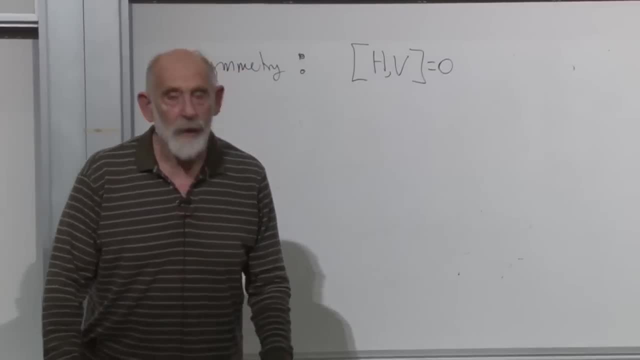 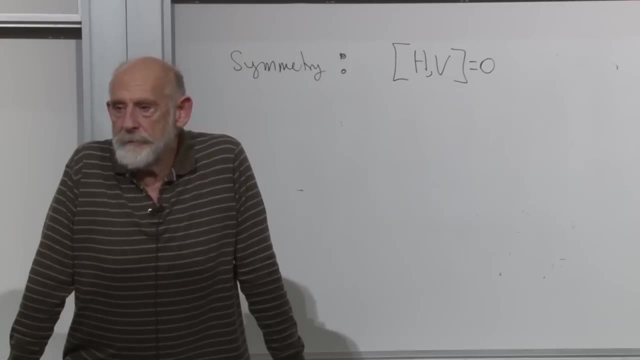 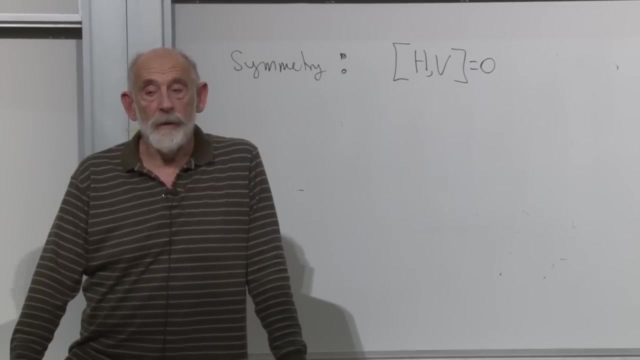 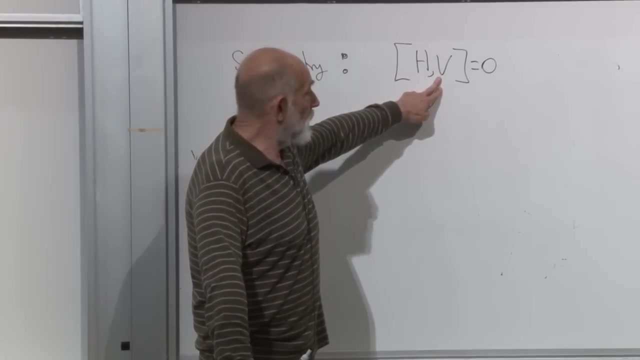 That's what it says. Do you remember from two quarters ago what the commutator of a thing with a Hamiltonian is? The time derivative of it? Yeah, So what this says is that whatever the operator v is, it's conserved. 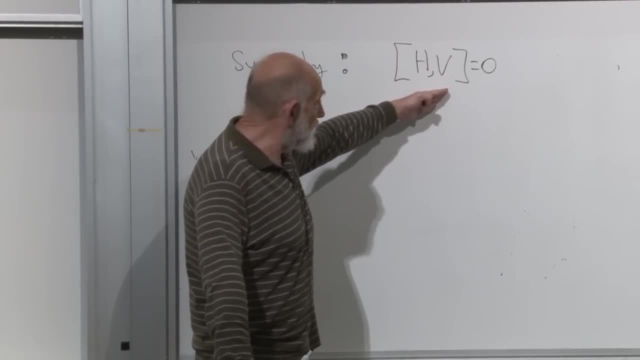 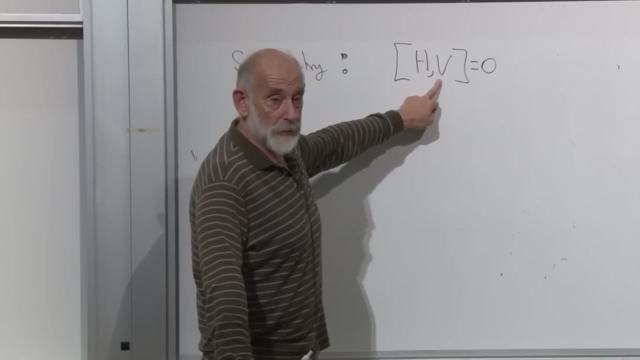 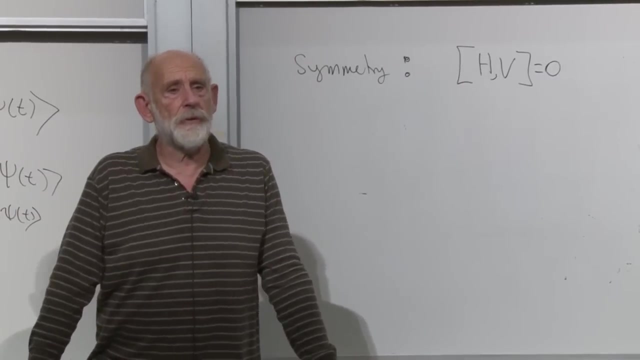 Conservation of a certain quantity- in this case v, meaning that it commutes with a Hamiltonian- is the same as saying there's a symmetry. You've seen this before in classical mechanics. What's the connection between symmetries and conservation laws, called in classical mechanics? 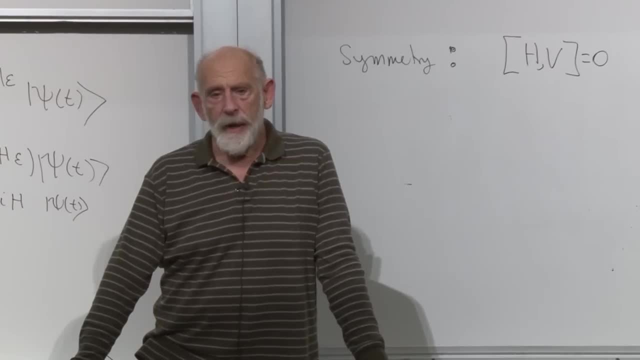 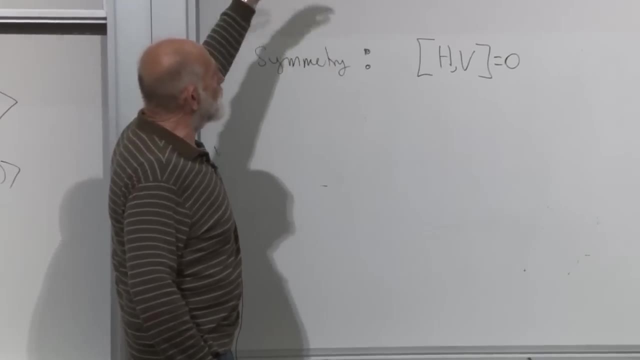 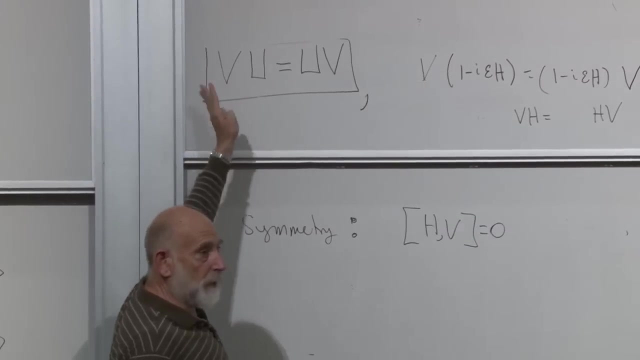 It's called Noether's theorem, Right. It's much simpler in quantum mechanics. It's much simpler in quantum mechanics. We don't need any fancy Lagrangian or anything else. All we need to know is that time evolution commutes with the symmetry operation itself. 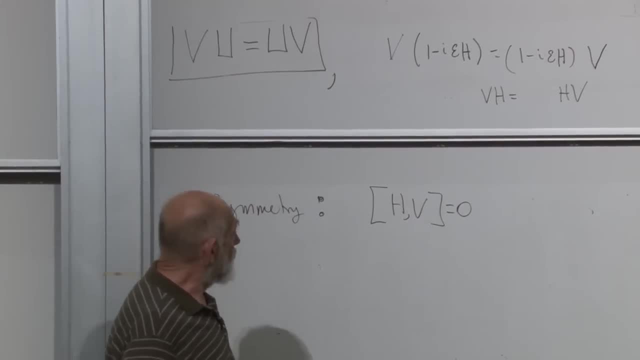 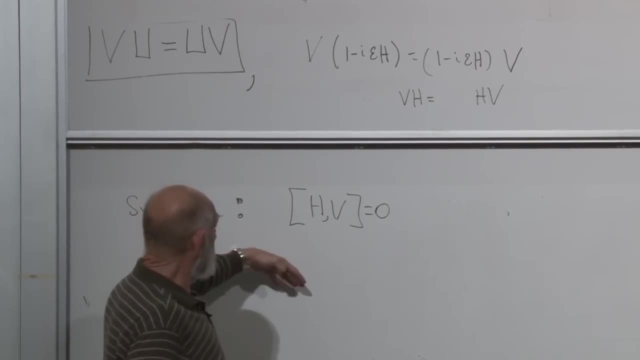 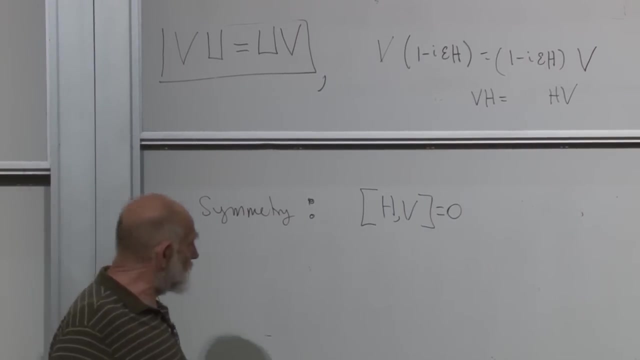 And that can be read in two different ways. It can say that doing the symmetry operation, Well, it says what it says. It can be read two different ways, but they both say the same thing. Okay, so that's Now. let's go one step further. 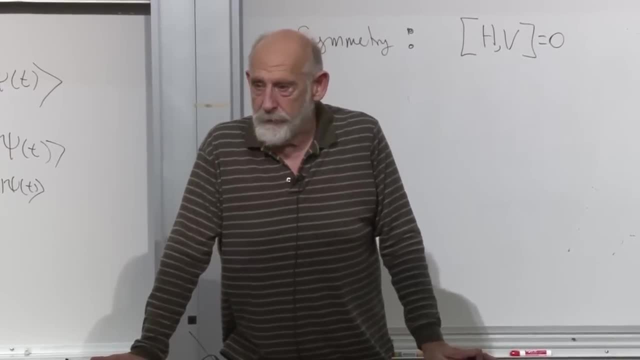 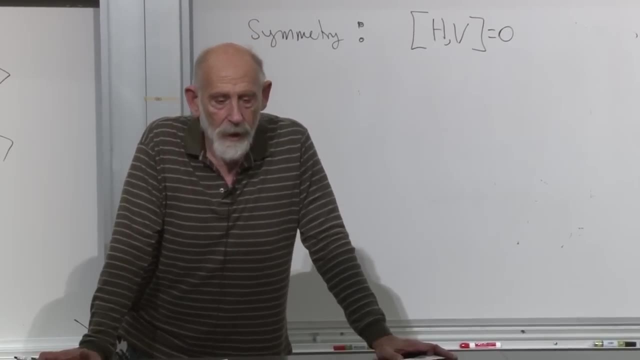 There are different kinds of symmetries. Let me give you some examples of two different kinds of symmetries. There are discrete symmetries and there are continuous symmetries. Let me give you an example of a discrete symmetry: Um. 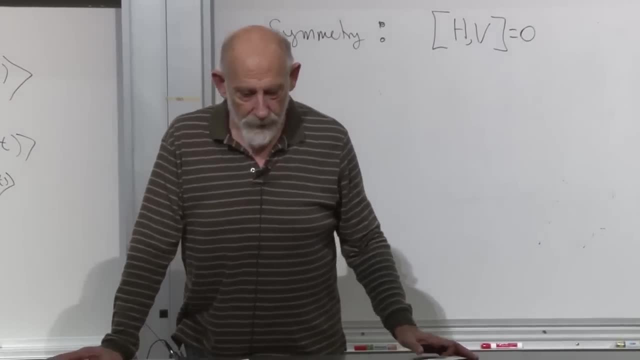 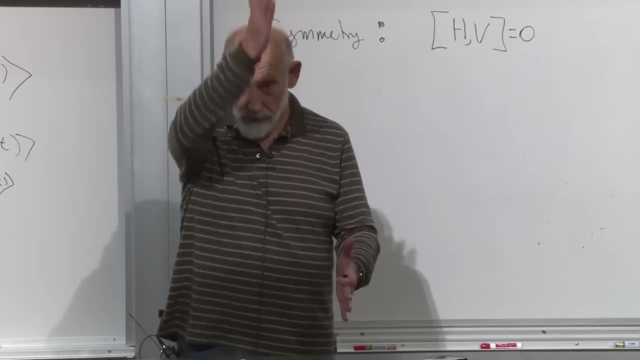 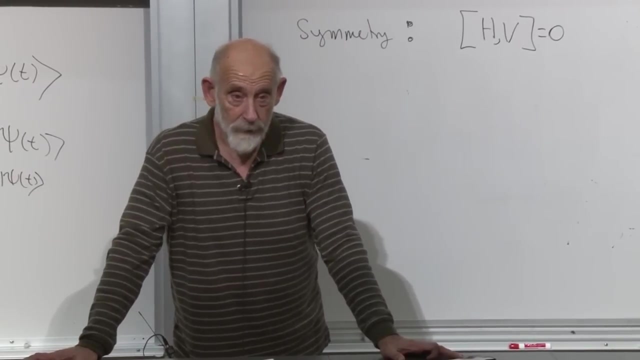 Think about reflection in a mirror. Reflection in a mirror takes a right hand to a left hand. Okay, That's the mirror image of a left hand as a right hand. That's a discrete operation. It takes left to right but there's nothing sort of in between. 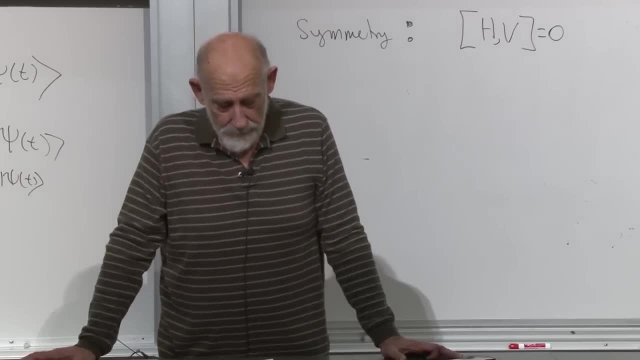 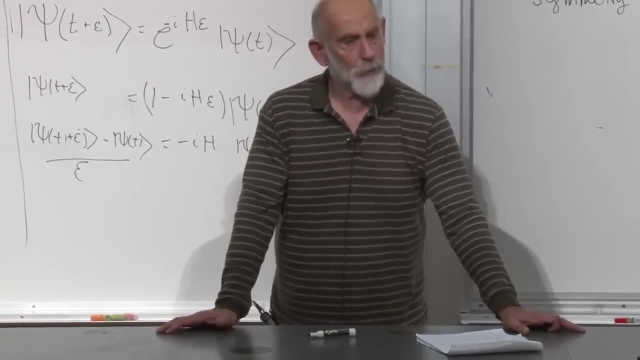 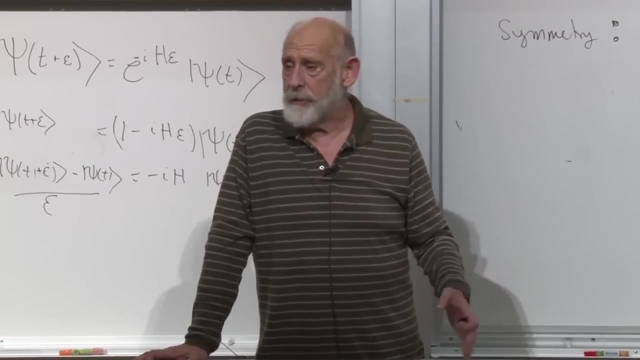 It's just a discrete operation left to right. Let me give you another example of a discrete operation. Um, Let's suppose we have a pair of electrons or a pair of particles, A pair of particles, and they happen to be the same kind of particle. 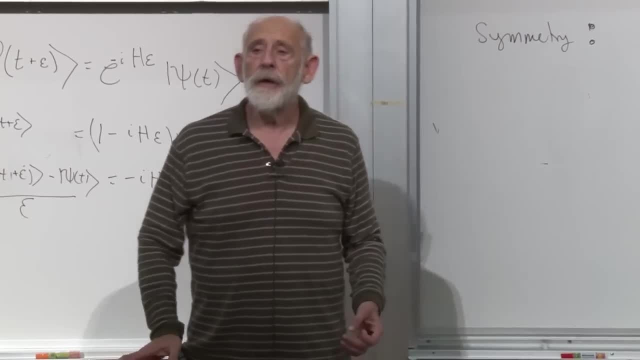 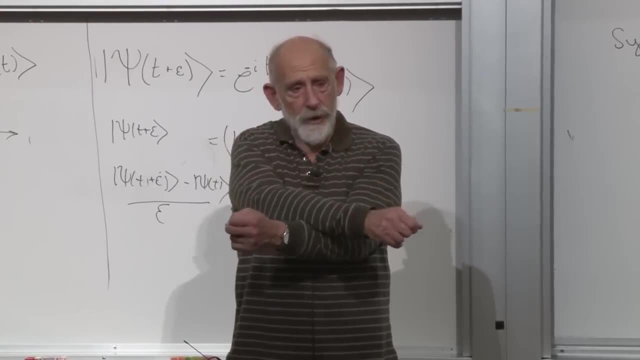 A pair of electrons or a pair of protons, Then if I take the two particles and I interchange them, whatever the state is, I interchange one particle with the other particle. That's a symmetry. Why? Because the particles are of exactly the same kind. 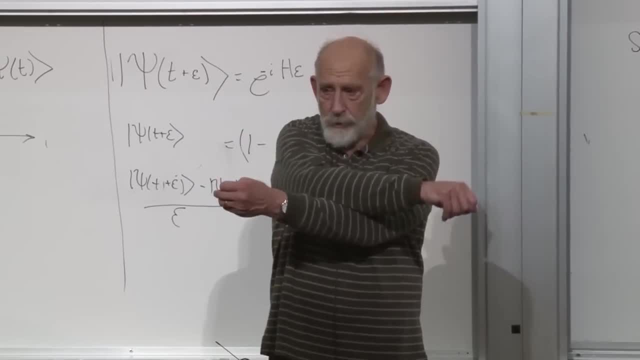 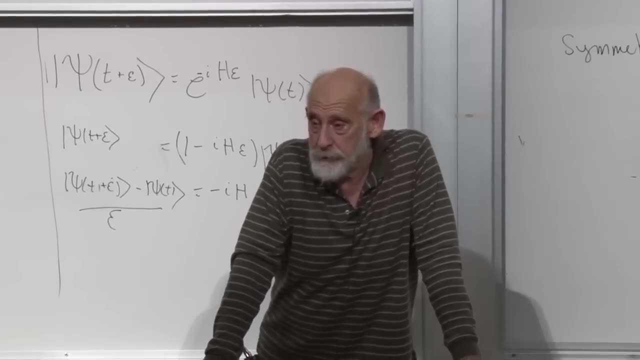 A proton over here and a proton over here is the same as a proton over here and a proton over here. That's just interchange of them. Those are discrete operations. Discrete operations means that there's sort of nothing in between, Or let's say heads and tails. 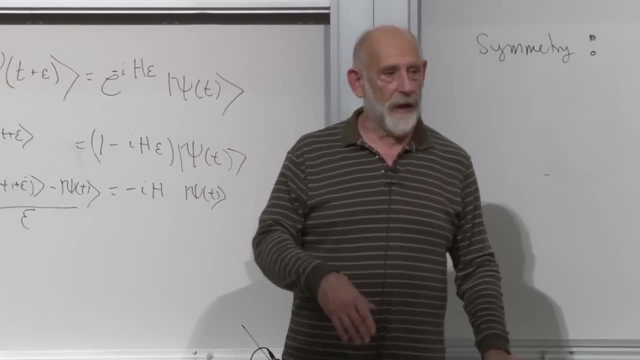 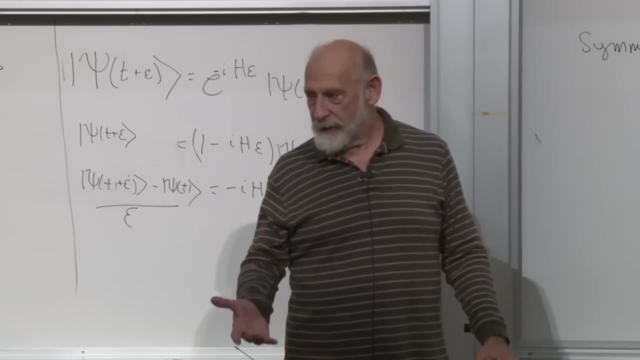 Just say heads and tails, A head and a tail. If the coin happens to have no markings on it, whether it's heads or tails, and you turn it over, then the physics of the coin and the flipped coin are exactly the same. 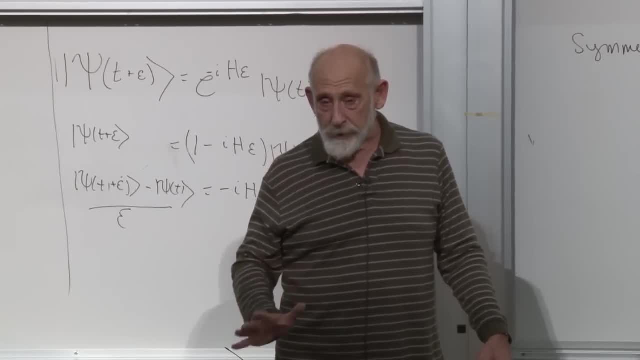 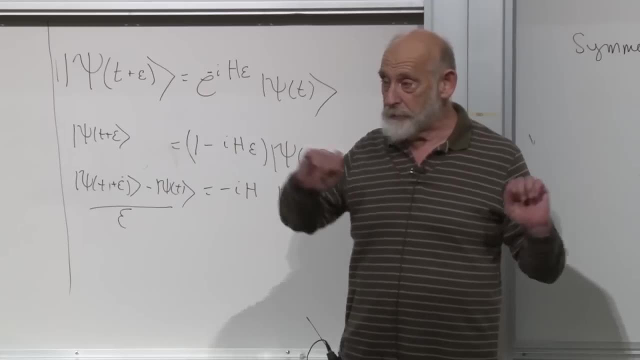 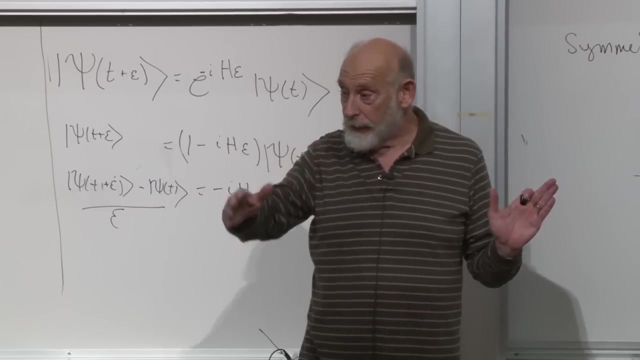 Those are discrete operations. By discrete I mean in distinction to continuous operations, And continuous operations are like rotation in space. Rotation in space, you can do a very small rotation. Small means one by a very small angle. In fact you can go further. 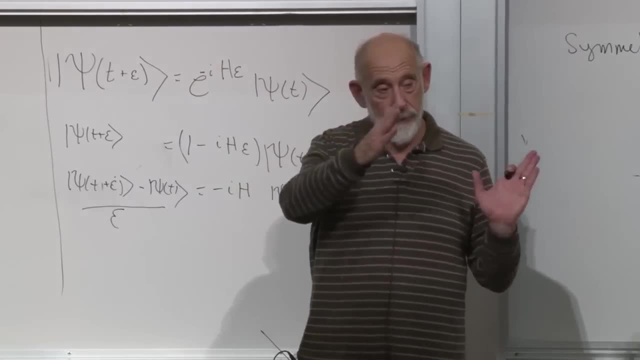 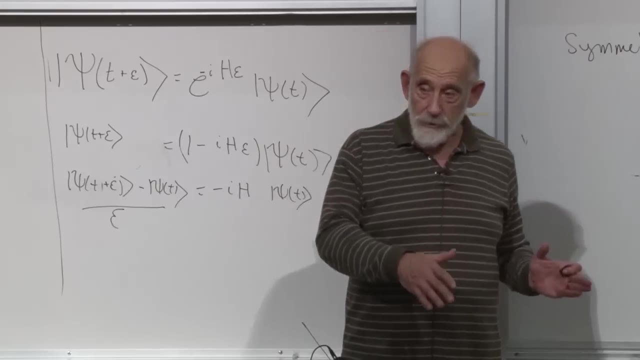 You can say that every rotation about an axis can be built up by tiny rotations about that same axis. That means that the rotations have a continuity to them That the flip of a coin does not have. Flip of a coin is either its heads or its tails. 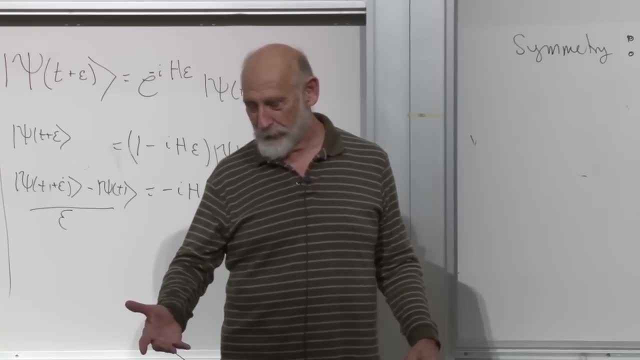 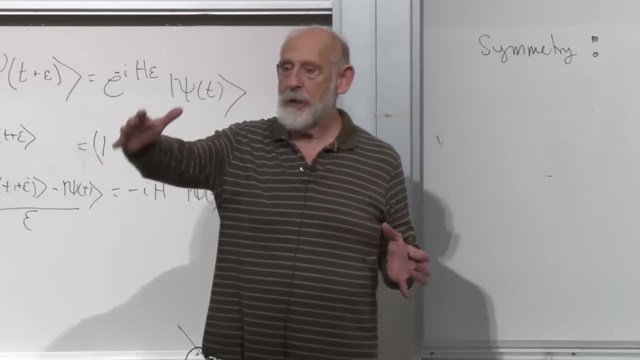 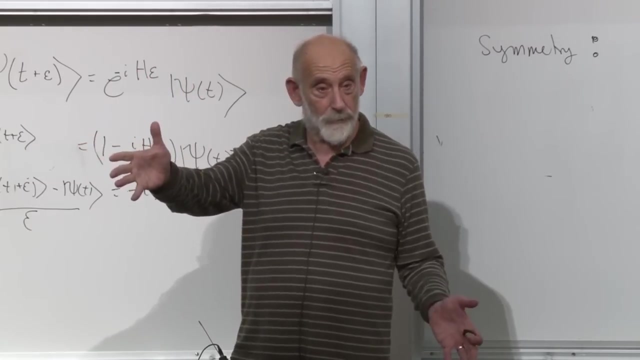 and there's nothing in between- for classical coins, For systems in three-dimensional space- or two-dimensional space for that matter- you can rotate them. You can rotate them by 90 degrees. That's a transformation, But you can build up that 90-degree rotation. 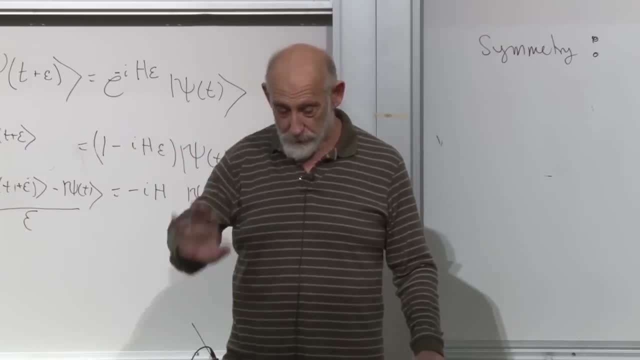 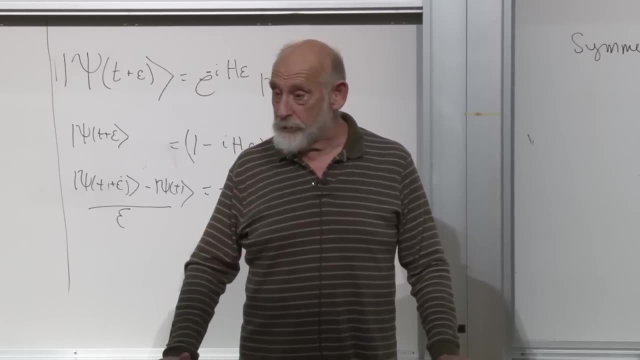 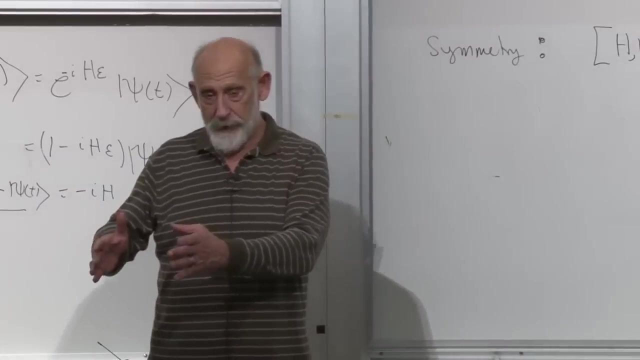 by lots of little, infinitesimal transformations. Those are called continuous symmetries. What about translation symmetry? Is translation symmetry continuous or discrete? Well, it's continuous. You can take any translation of a system and think of it as being compounded out of lots of small translations. 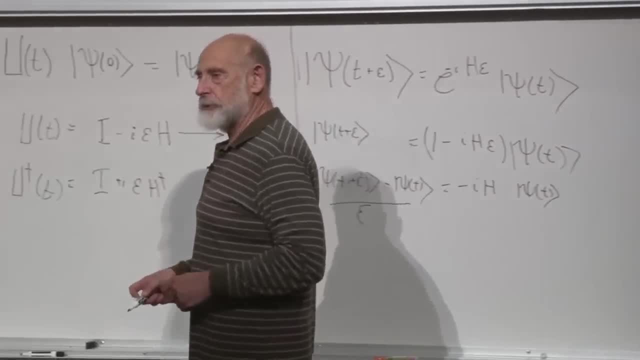 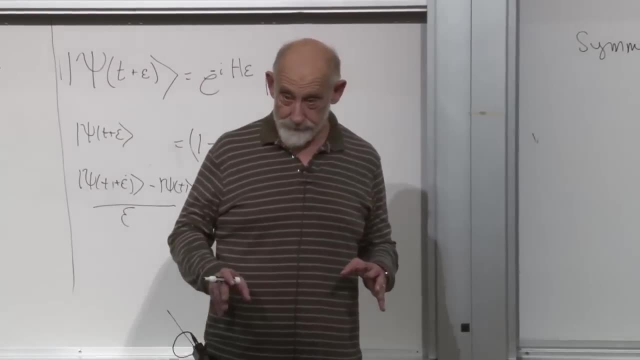 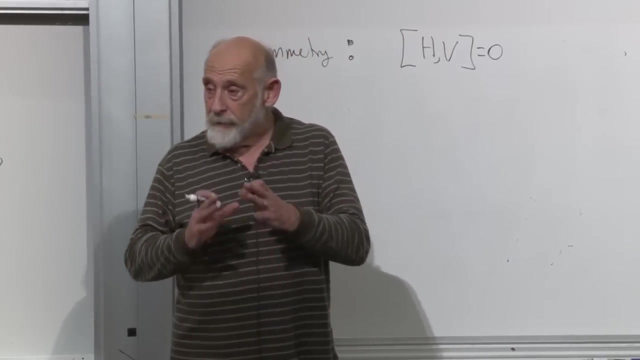 The continuous symmetries are the ones in particular. the rotation symmetries and translation symmetries are the ones I want to focus on. Okay, What do we know about continuous symmetries? We know we can build them out of lots of little elementary. 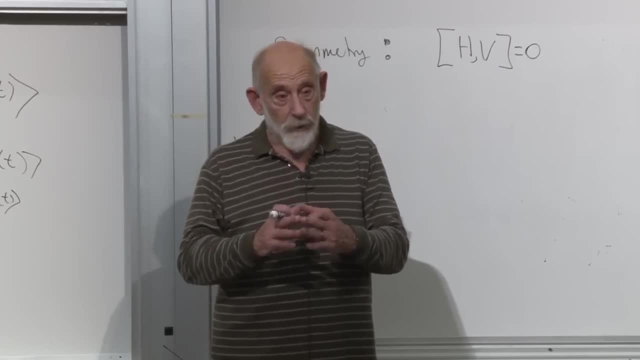 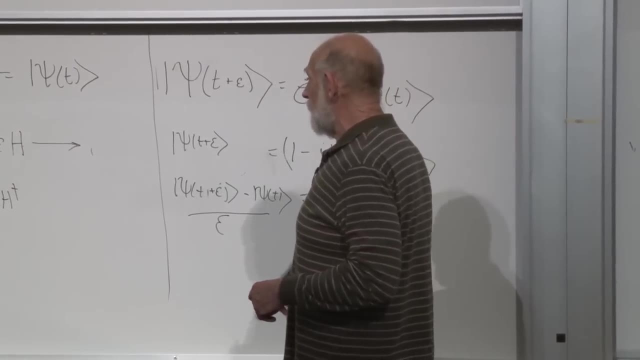 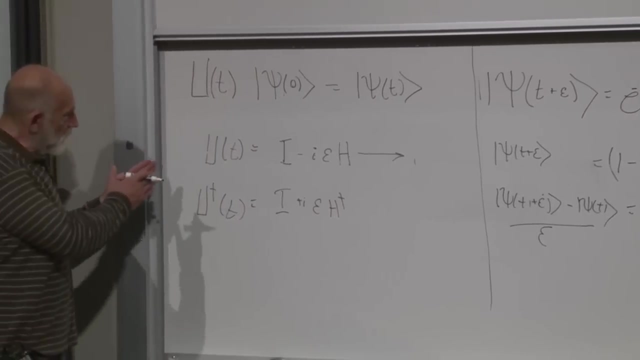 small transformations. So let's focus on the small transformations. We're going through basically the same manipulations that we went through over here. Time translation is a continuous thing. You can build up a time translation by 10 seconds by thinking of it as lots of little. 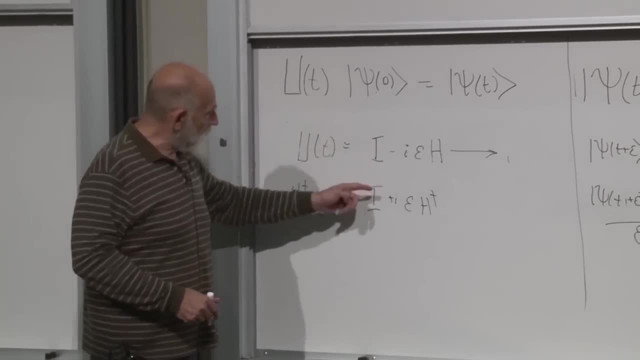 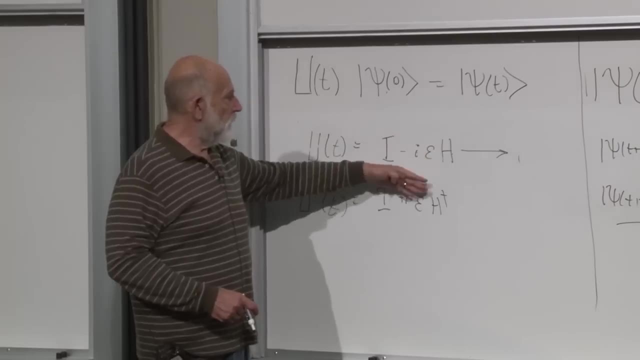 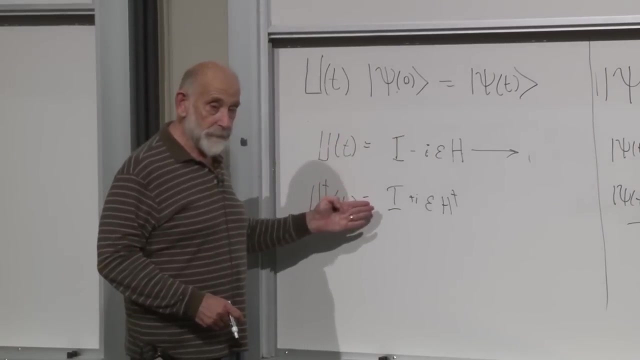 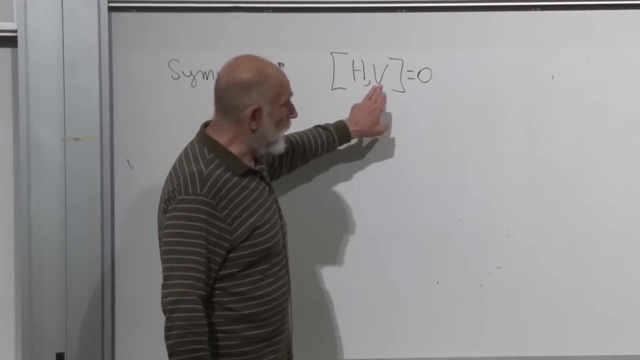 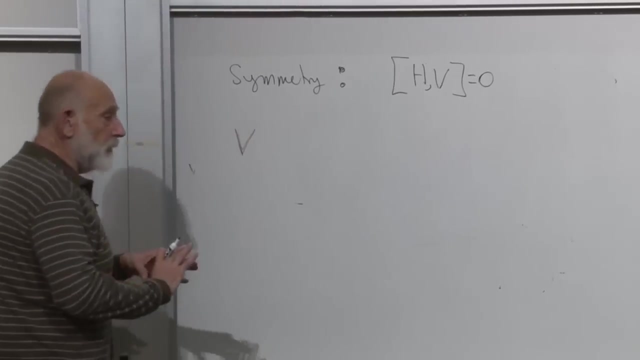 time. translations by microseconds. Okay, And that led us to the conclusion that u's are related to her mission operators through this relationship here. Exactly the same is true of every continuous symmetry. Exactly the same thing is true: Every continuous symmetry can be thought of as being built up. 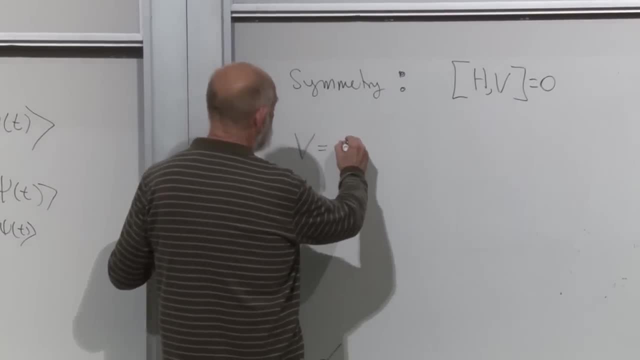 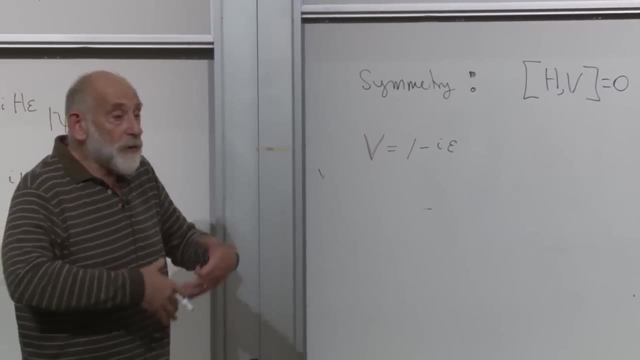 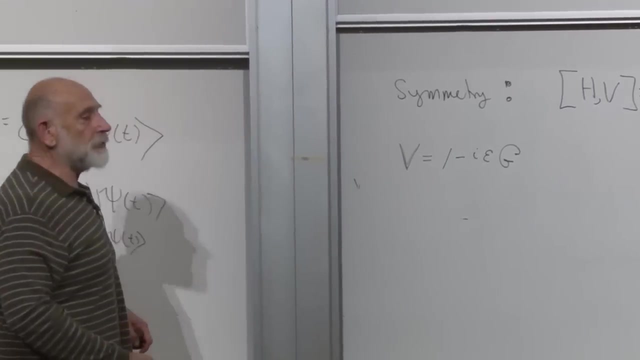 by little, infinitesimal ones, which have the form one minus I. epsilon not times a Hamiltonian, but something some her mission operator. Let's call it G. G stands for generator. G stands for generator, And what we're thinking about now? 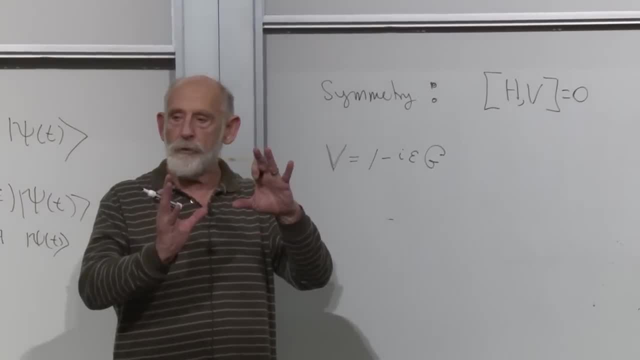 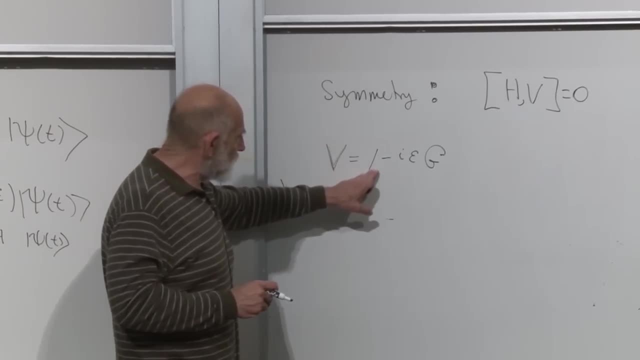 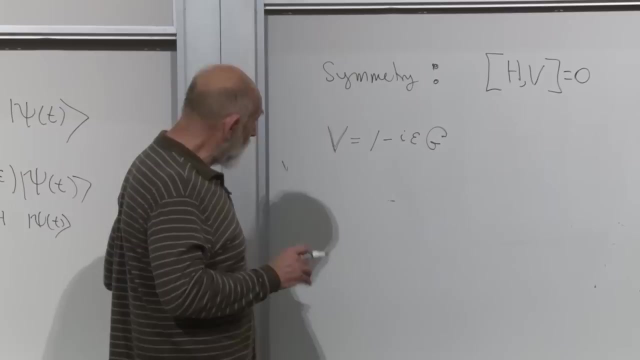 is a symmetry transformation, but one of them which is very close to being the identity. Such a transformation can always be represented as something close to the unit operator, and close to the unit operator means just shifted by a small amount By the same argument. 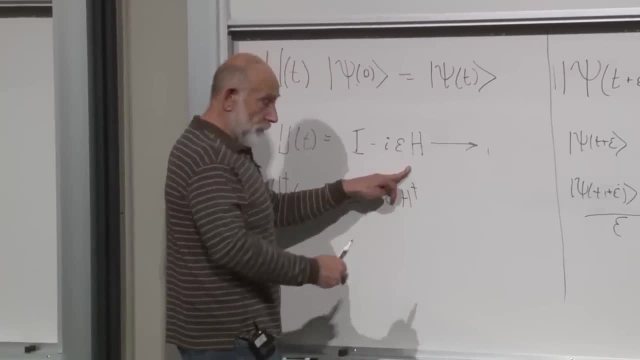 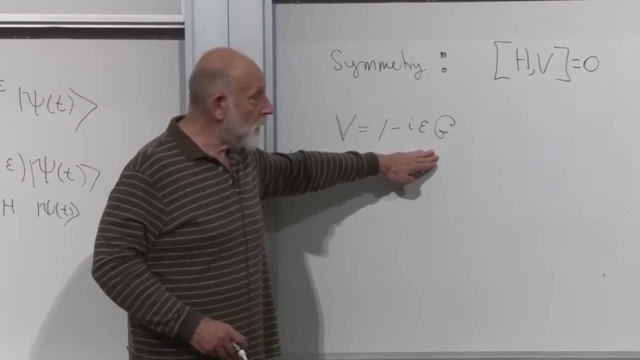 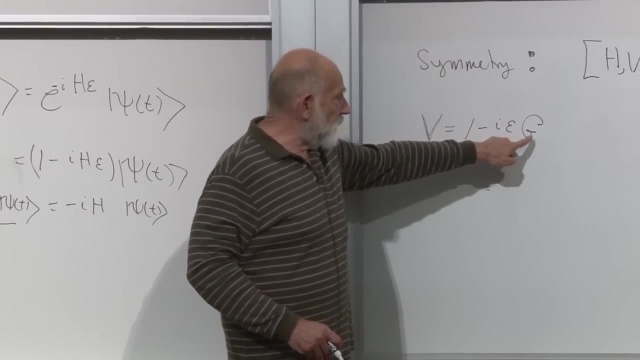 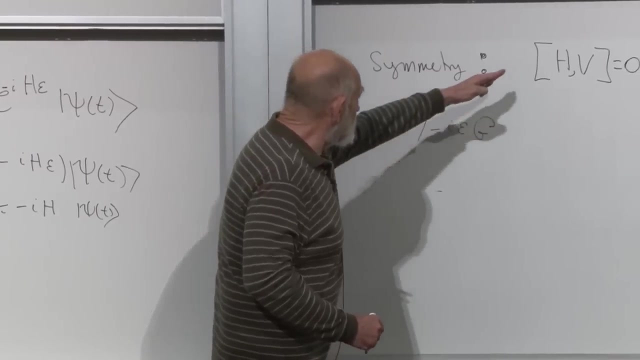 that told us that H is her mission, G is also her mission. Symmetry operations, which are continuous, can be represented in terms of infinitesimal transformations which are generated by a generator, G. And if we plug this into here and we then write, 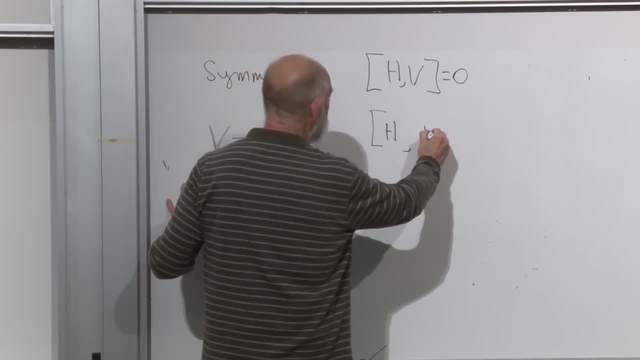 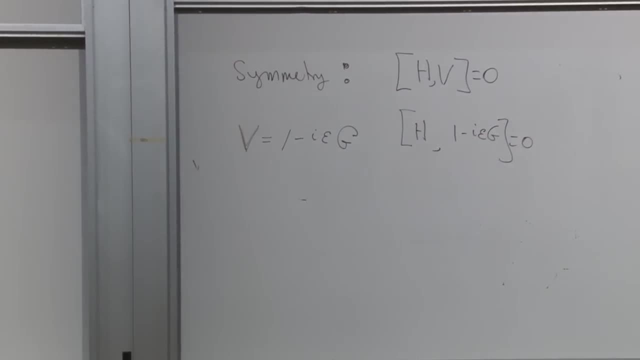 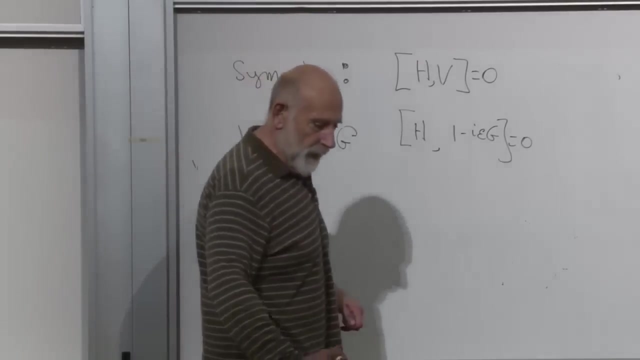 the commutator of H with one minus I, epsilon G is equal to zero. what does that say? What's the commutator of H with one? Commutator of anything with one is zero. Everything commutes with the operator zero. 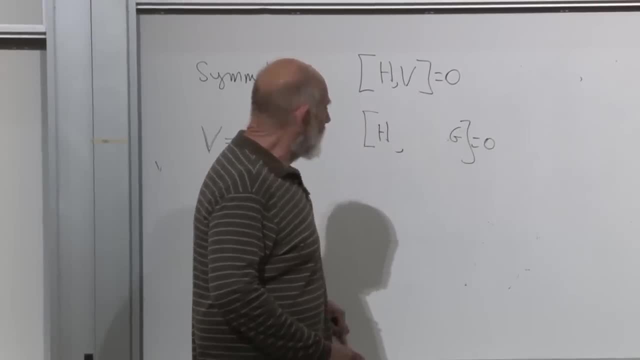 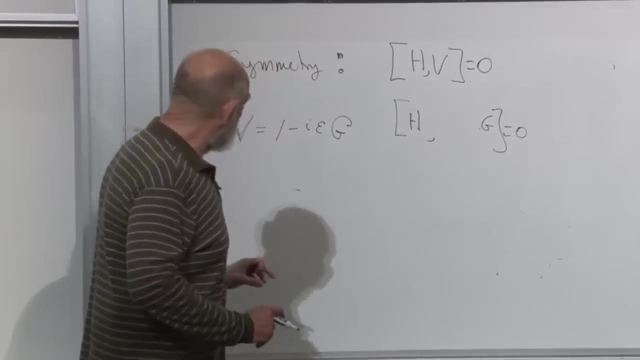 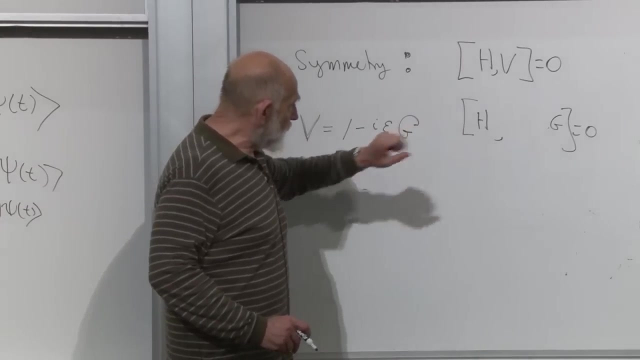 The I epsilon that factors out, and what it tells us is that symmetry operations are generated by. this is what it means to be generated by. generated by means can be built up by lots of little ones. They're generated by things which commute with the Hamiltonian. 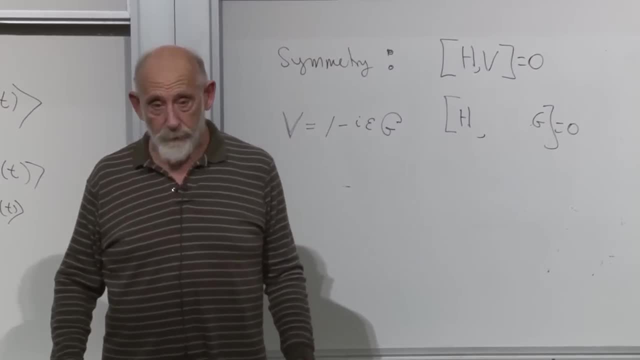 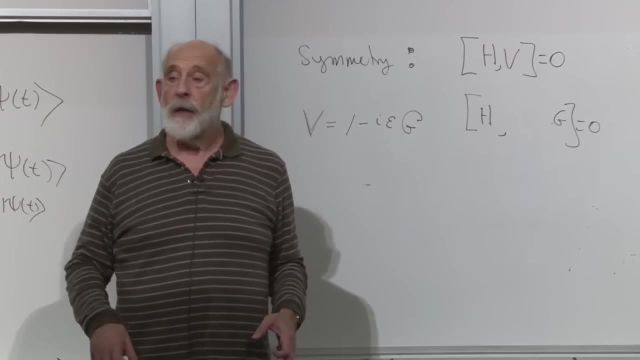 So if you want to find all of the symmetries of a problem, you'll start looking around for all the things which commute with the Hamiltonian. There's another feature of things which commute with the Hamiltonian. Do you remember from last quarter? 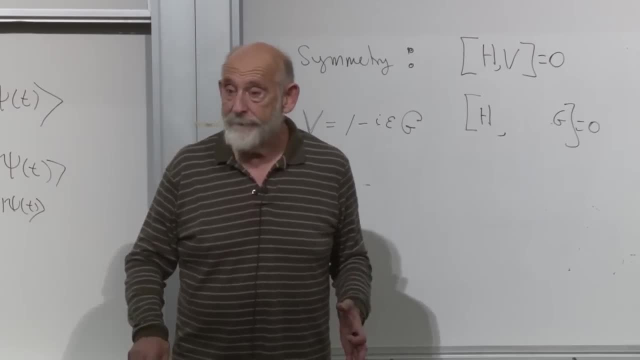 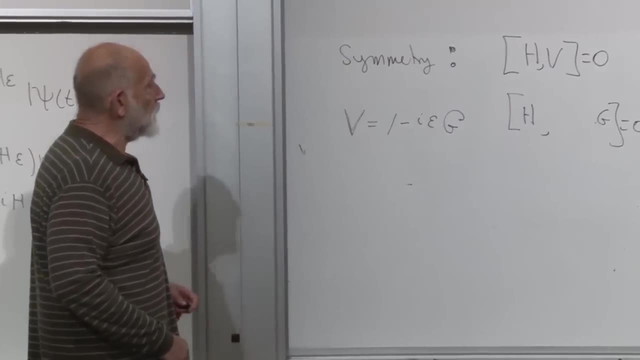 It's true both in the yeah, what was that? They're conserved. So conservation and symmetry are closely connected. If you want to find all of the symmetries of a problem, it's equivalent to finding all the things which are conserved. 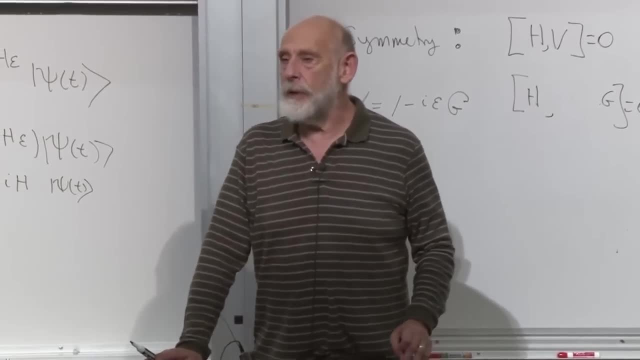 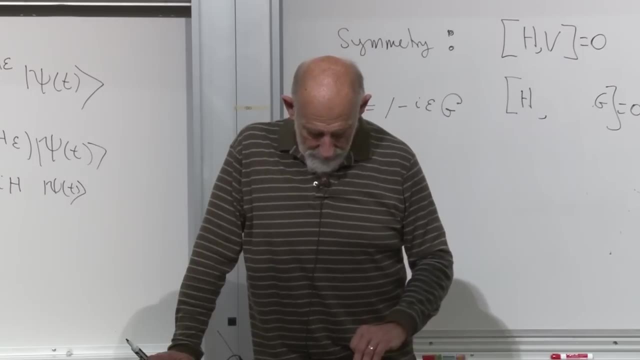 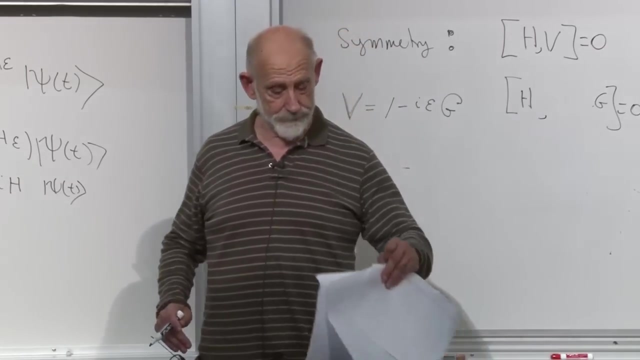 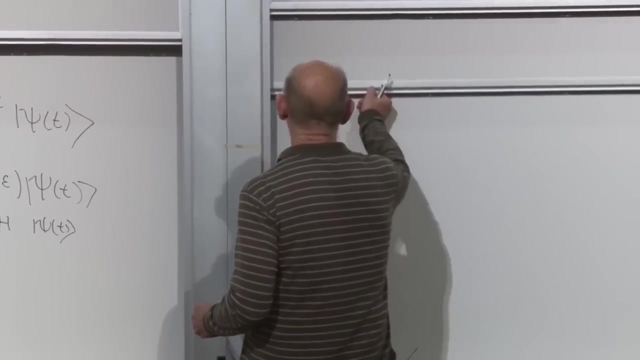 All right now. this was very abstract and so we need to do an example or two to get the idea. Let's do an example and let's begin with translation. Translation of a particle from one place to another. Okay, Translation of a wave function. 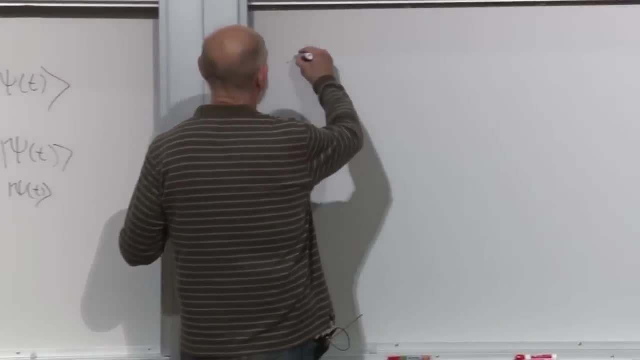 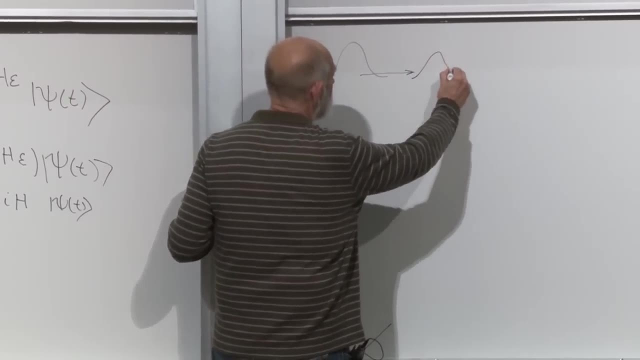 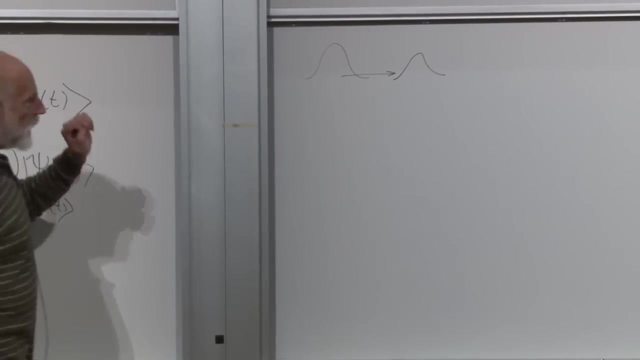 We want to take a wave function. Here's a wave function And we're going to move it a little bit, We're going to translate it to a new wave function And we want to find out what operation does that If we have a psi of x. 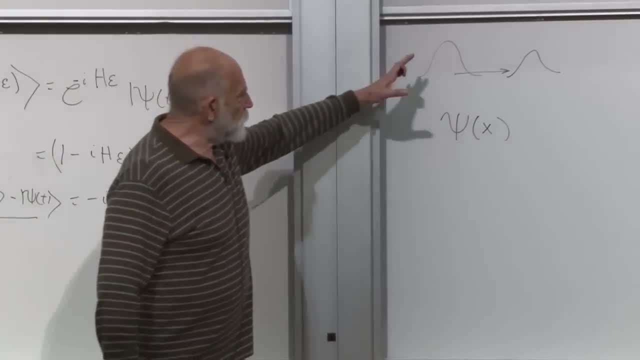 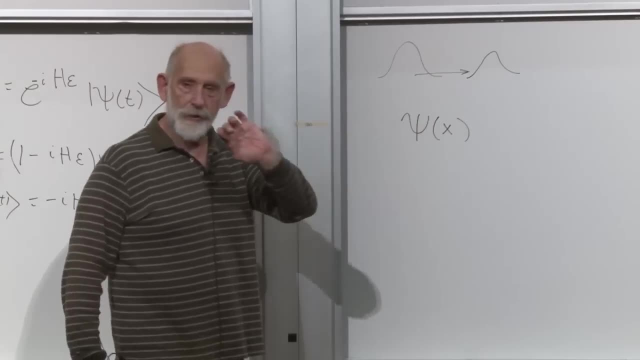 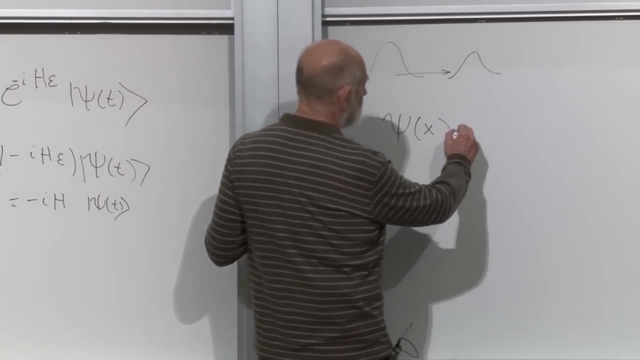 what operation do we do to translate it? We're going to translate it to a new position. We're going to take that new position to only deviate by a small amount, by amount epsilon. but we know what the answer is. The answer is: 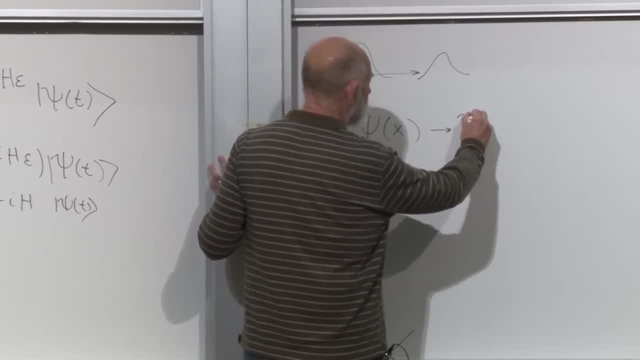 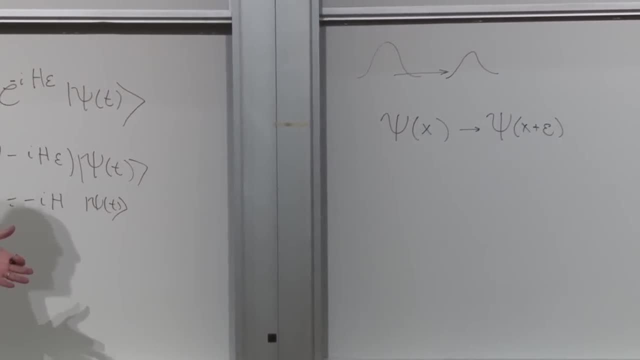 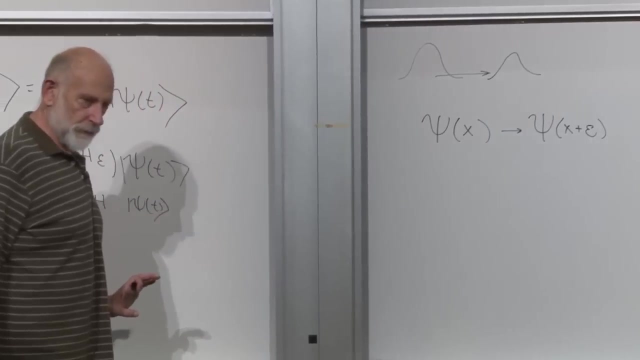 psi of x goes to psi of x plus epsilon. Epsilon now could be a large number. We're just translating by a large number, but specifically I want to think about the size of a small translation. Translation by a little bit Okay. 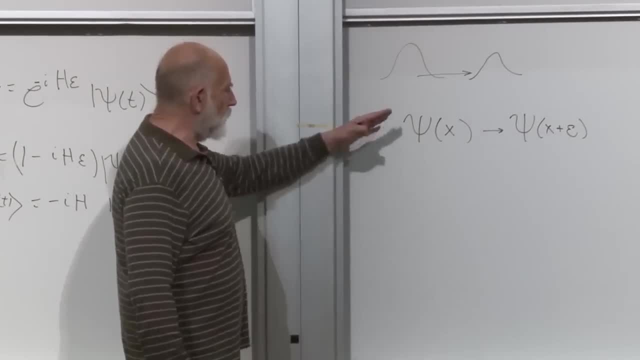 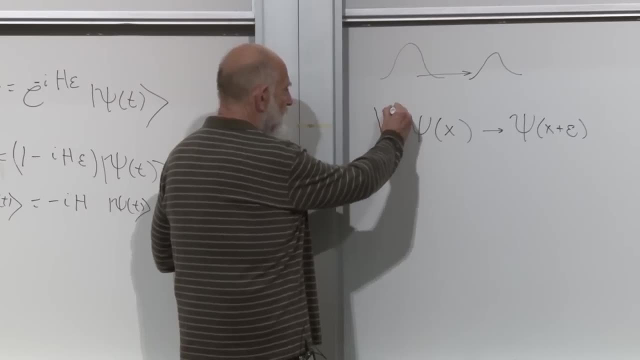 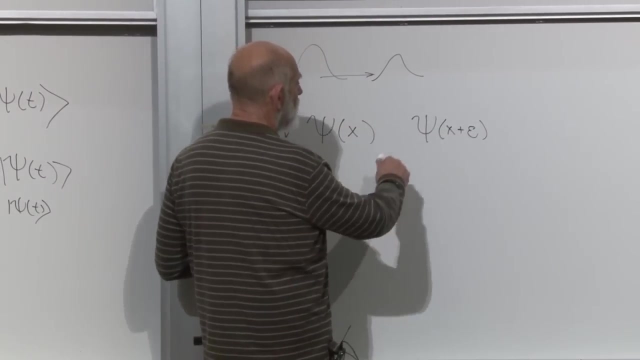 So psi of x. in other words, we can write that the translated wave function. in fact, we can write it this way: Whatever v is, whatever v is- we haven't figured out what v is yet- but whatever v is. 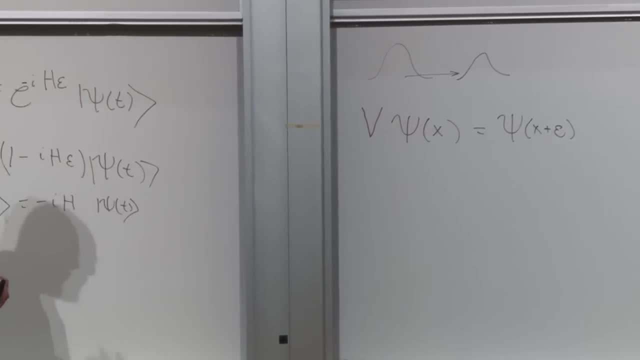 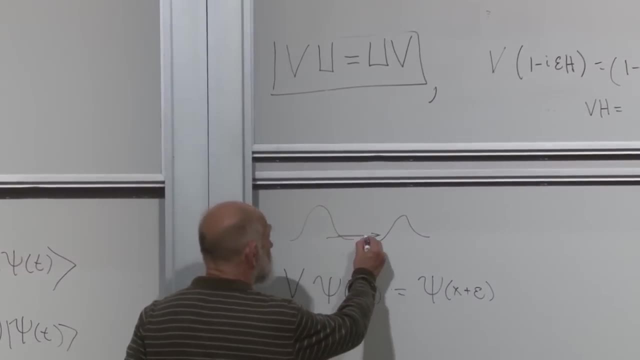 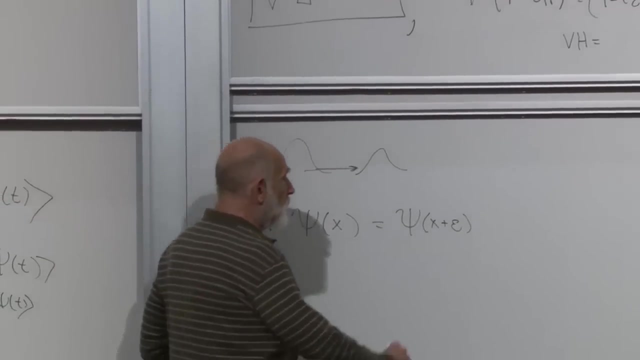 it acts on psi of x. to give us psi of x plus epsilon, That's pretty easy. That's what the v does in this case. It acts on psi of x and it translates the wave function by amount, epsilon. Okay, Now if epsilon is small, 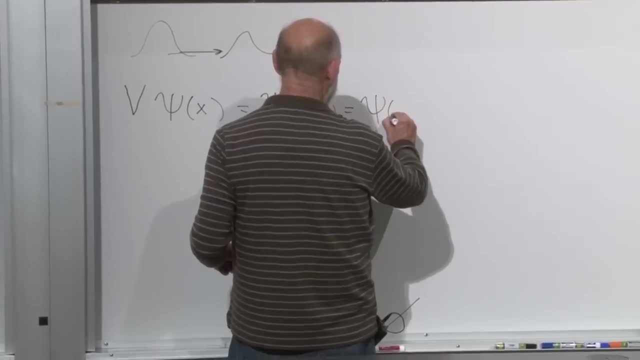 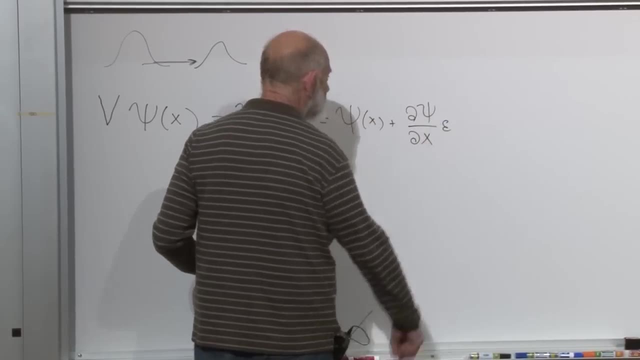 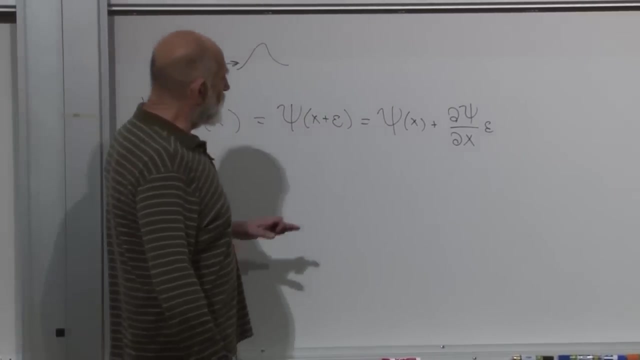 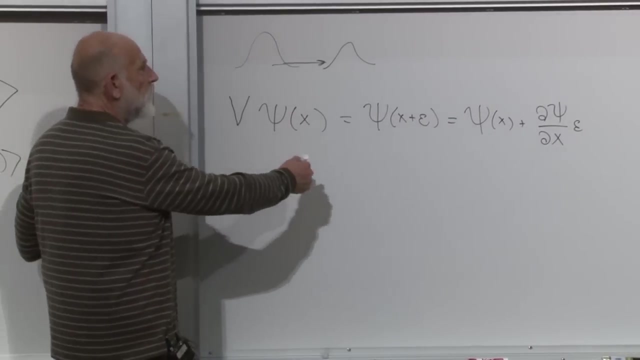 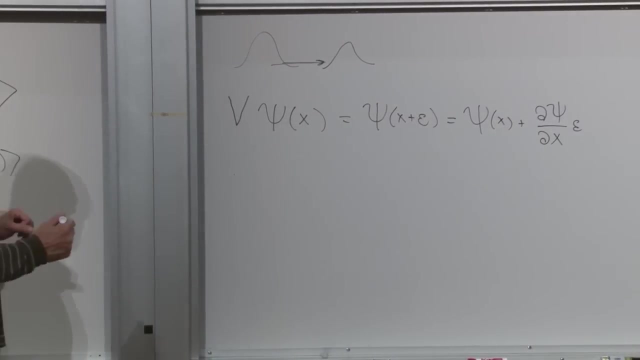 we can also write that this is equal to psi of x plus the derivative of psi with respect to x times epsilon. So what v does, what v on psi does, is it gives back the same psi plus something proportional to the derivative. That suggests: 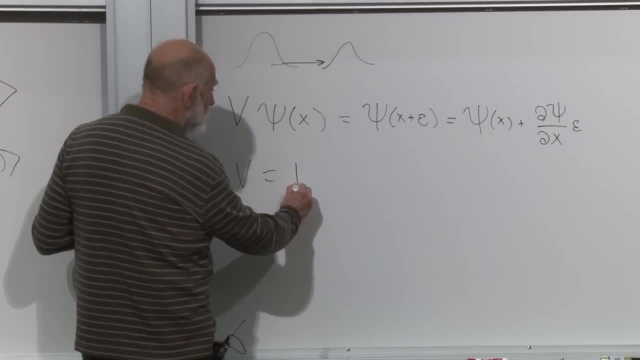 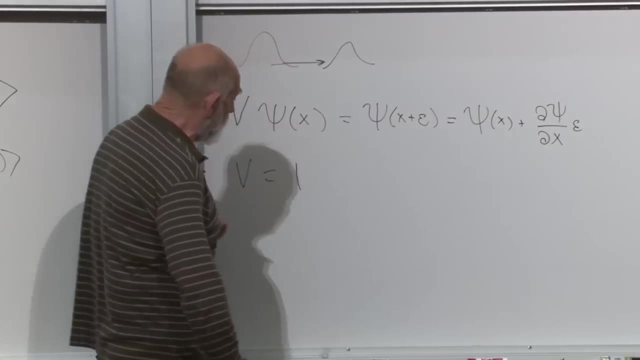 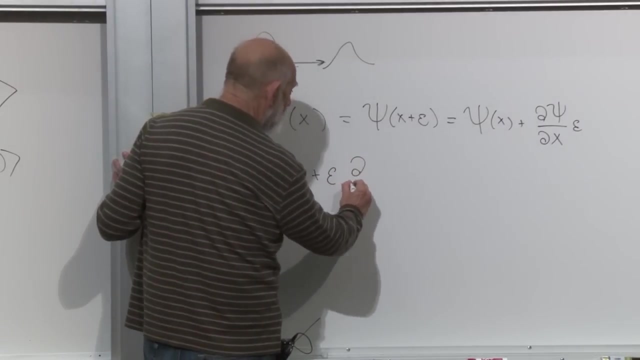 it doesn't suggest. it proves that whatever v is is, it's the unit operator. that's the first term here. it acts on psi of x and the small change is epsilon times, the derivative operation. I haven't written on x, we could write on x. 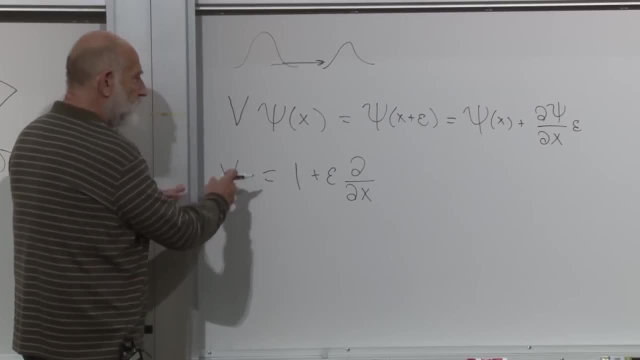 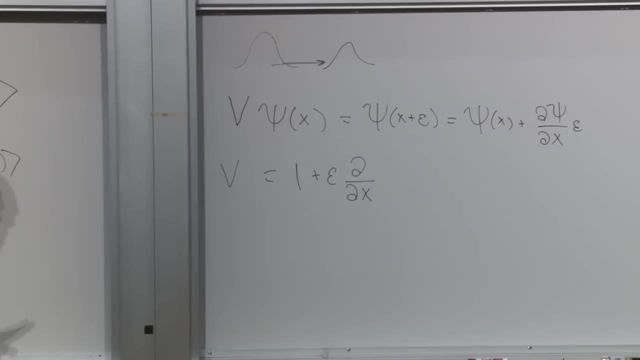 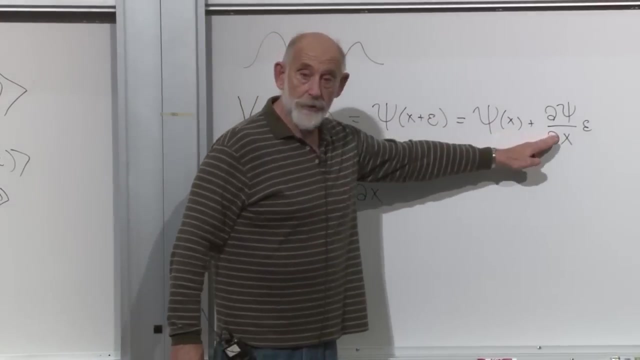 v, sorry times. psi v is an operator, it's the unit operator plus epsilon times the derivative operator. We can act on any wave function and what it will give us is the wave function infinitesimally displaced. Now, what about d psi by? 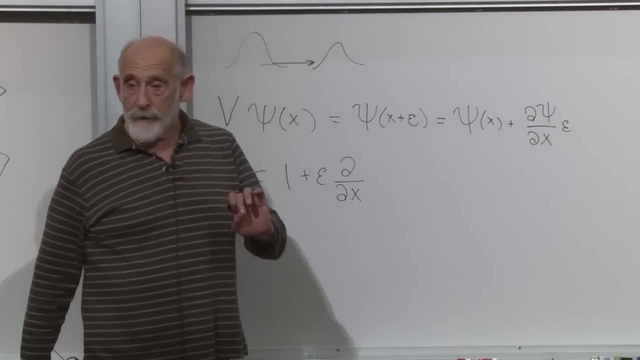 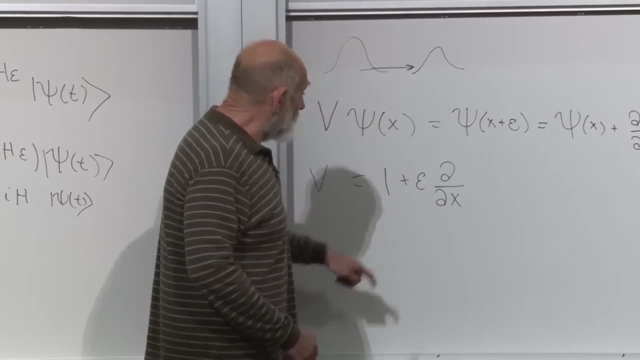 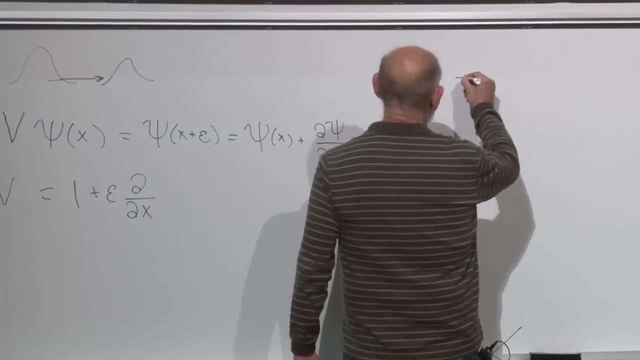 dx. what about d by dx? d by dx is an operator. it operates on wave functions. it's a linear operator. it's connected with the momentum operator. Remember the relationship. the momentum operator p equals minus i h bar d by dx. 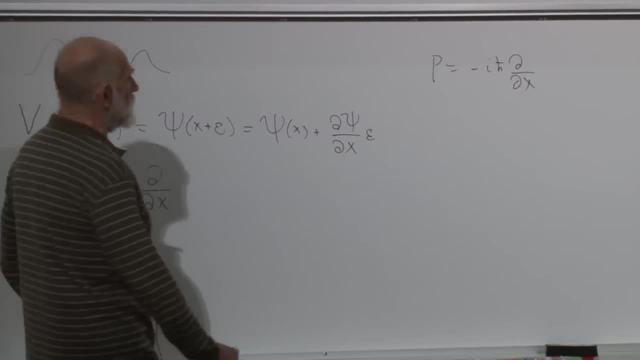 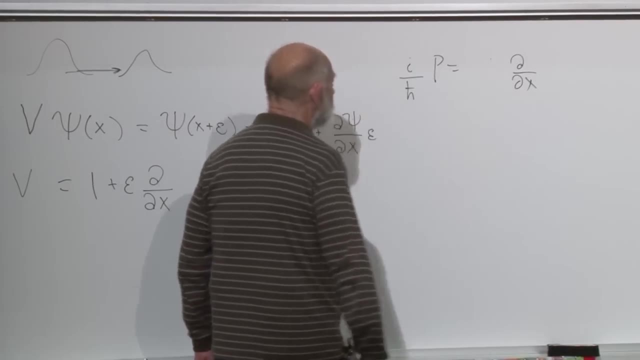 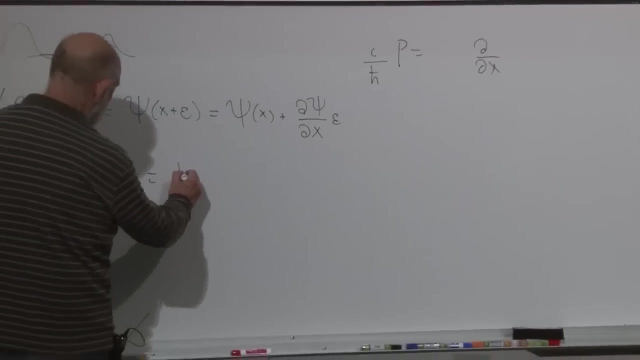 Alright. so what do we want to do? We want to write: let's multiply by i- get rid of the i here- and divide by h bar Differentiation- is i over h bar times momentum. So let's write this that way. one. 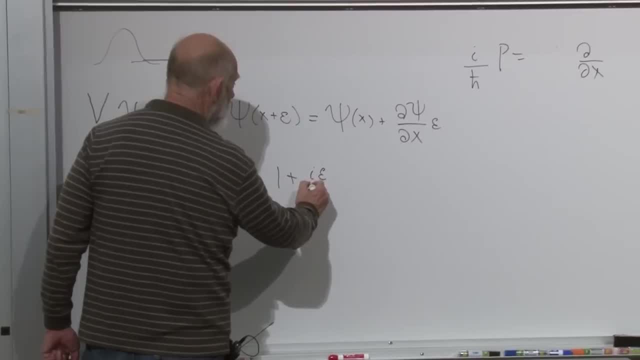 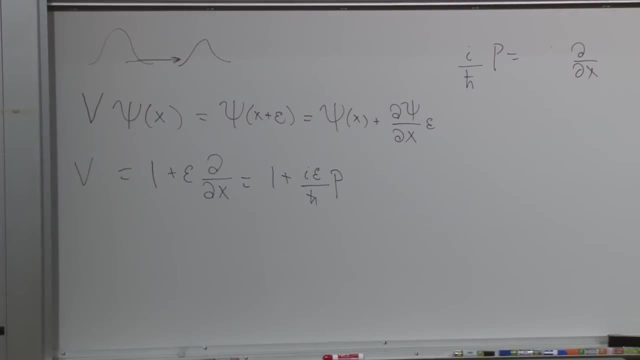 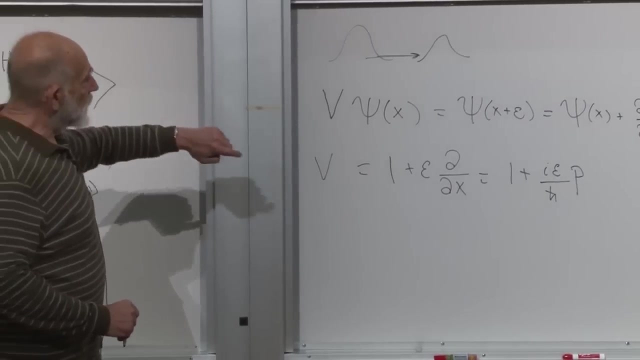 plus epsilon i. epsilon over h bar times the momentum. We now have an example of a infinitesimal symmetry operation. By infinitesimal I mean just by a little bit of a shift. And we found out what its generator is, The g. Where was it? 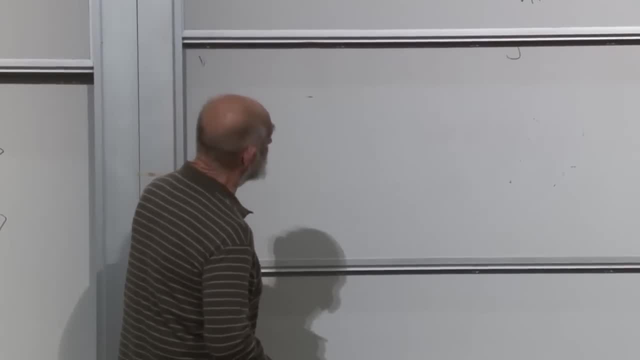 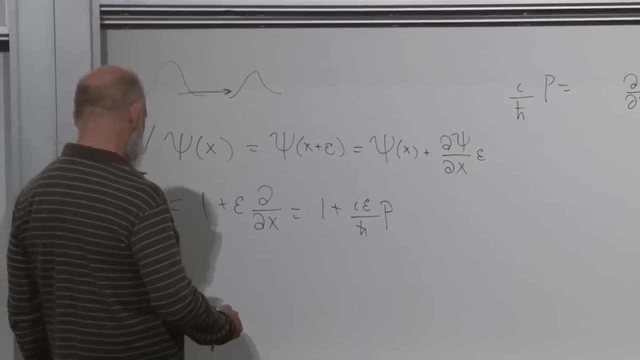 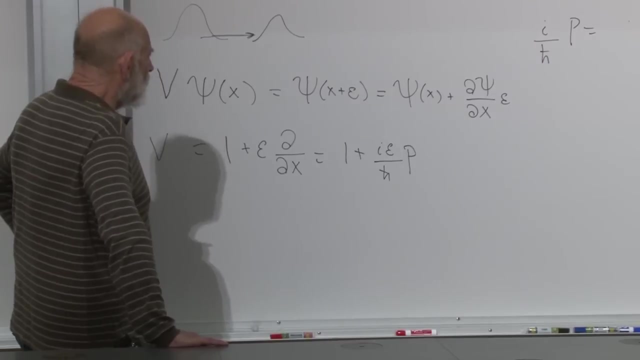 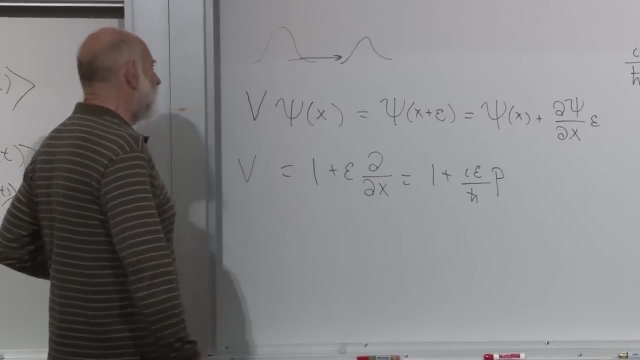 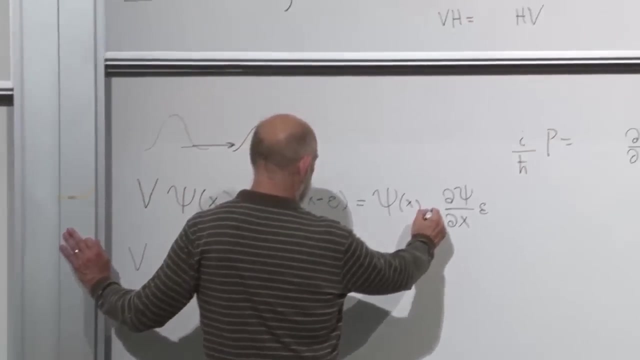 Did we have g here? Well, yeah, v is one minus i, epsilon g In this case. I would have much preferred that I defined things so that this came out to be minus here. but Yeah, this one, I think that's right. 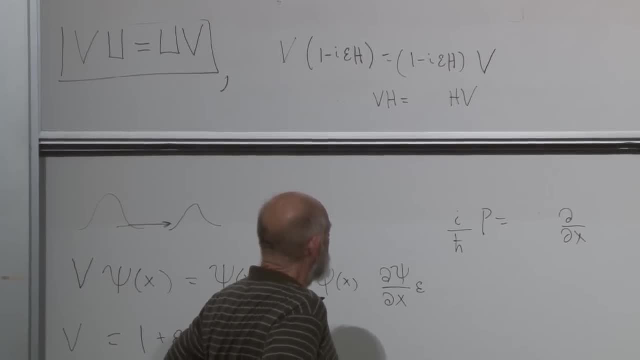 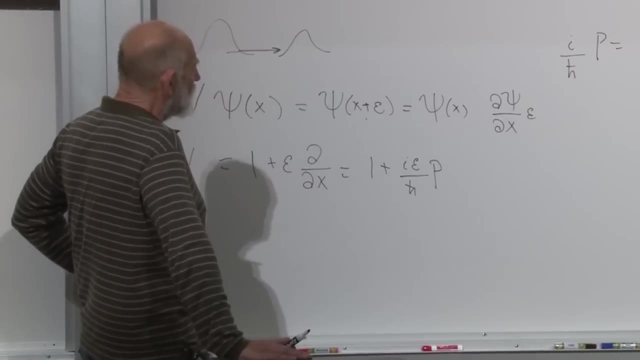 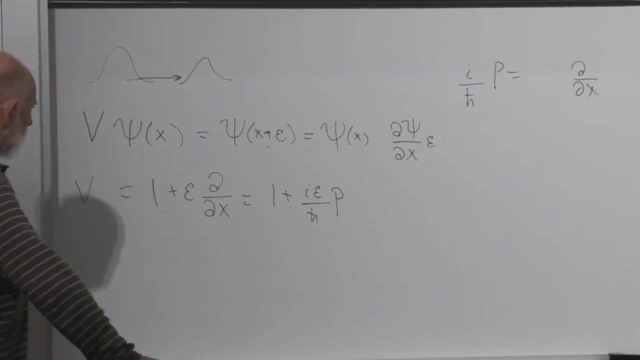 No, no, that's right. You think this is wrong? It's right, So let's see. So I substituted. I think I got this right. Wait, wait, sorry, did I? Yeah, that's right. 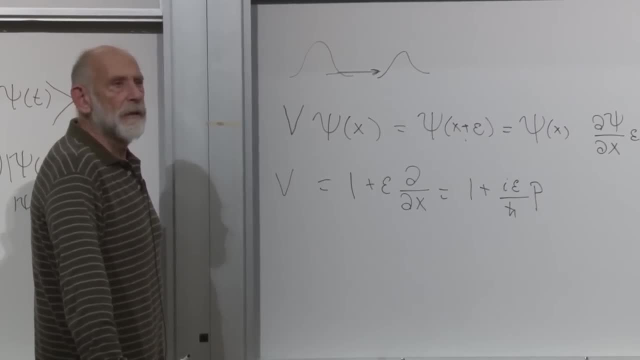 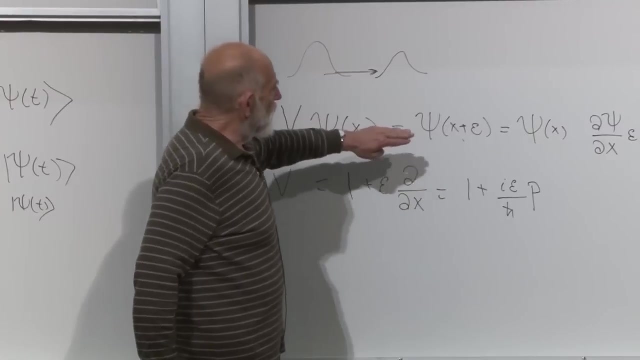 Do you disagree with this? No, I think it's right. Alright Now. um, Ah, I think if I shift the wave function to the right, if I shift the wave function to the right, that's really pretty good. I'm putting a minus sign here. 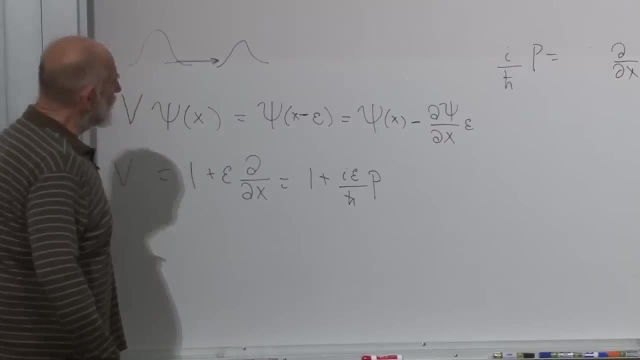 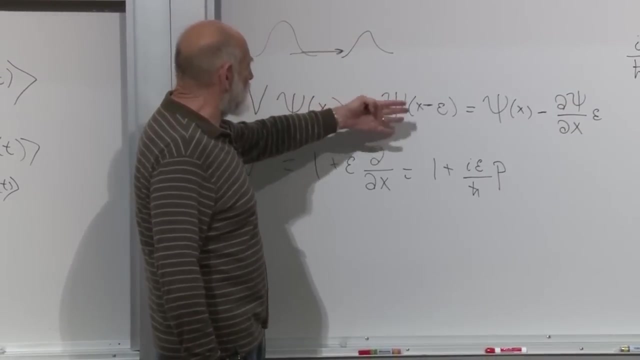 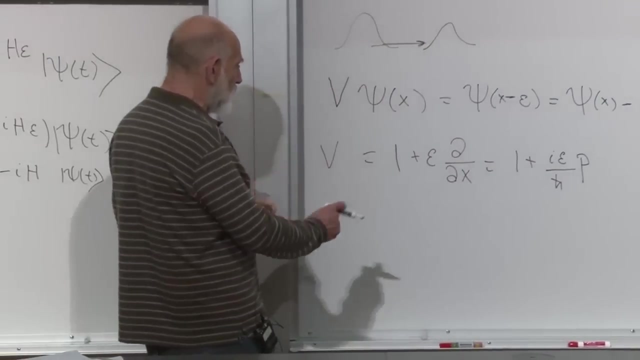 Yeah, Yeah, I made a mistake in defining a shift to the right A shift. It looks like it should be x plus epsilon, but psi of x goes to psi of x minus epsilon, So this is actually a minus sign here. 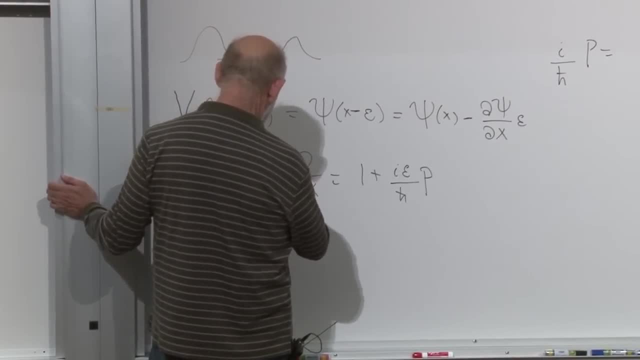 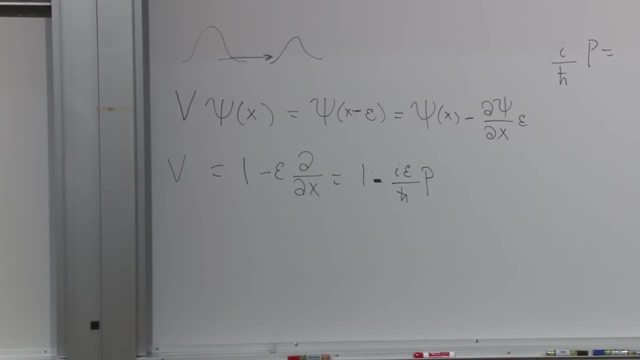 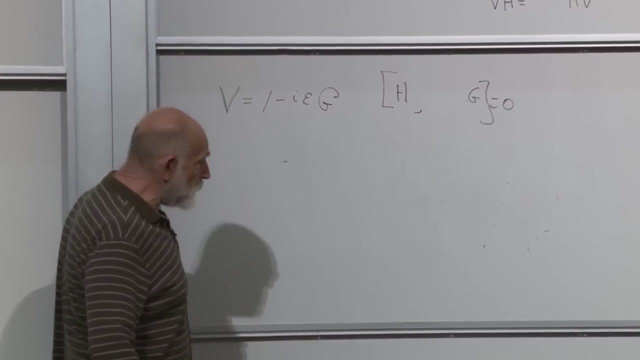 If you track that through, we will find out that there's a minus sign here. Yeah, Okay, so it identifies for us what the symmetry generated g is for translations. And what is it? It's the momentum divided by Planck's constant. 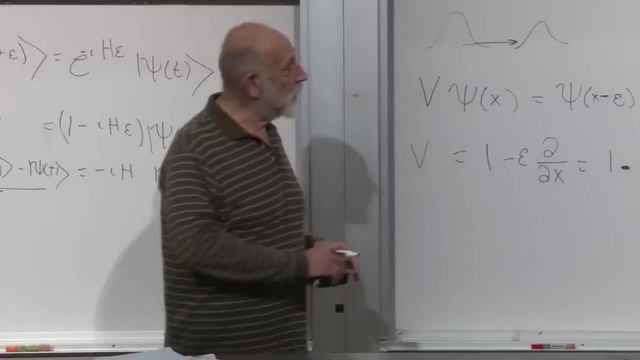 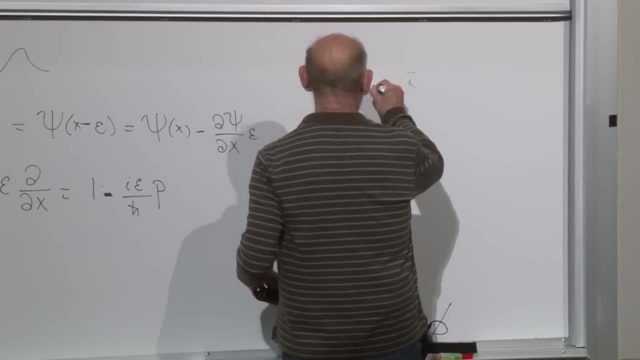 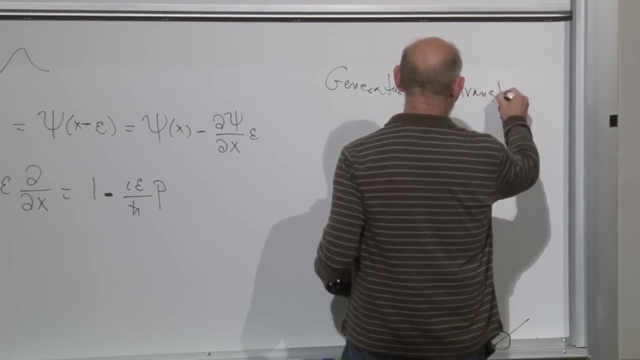 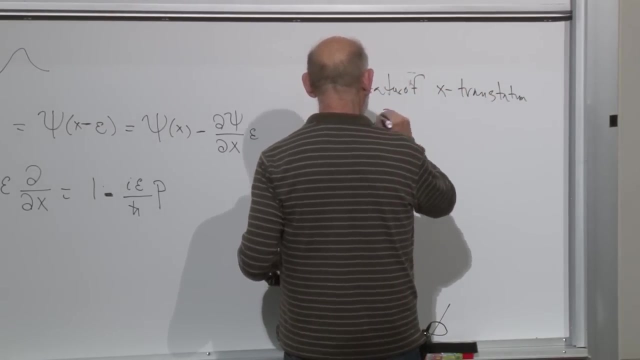 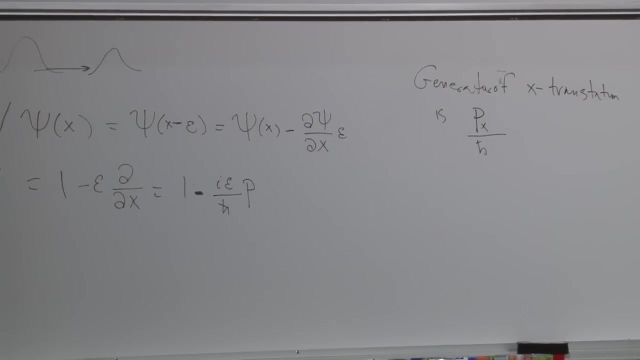 Momentum divided by Planck's constant. we can write that the generator of translations- here's the language, the generators of x translation- is p sub x, p sub x, strictly speaking, divided by Planck's constant. We can drop the Planck's. 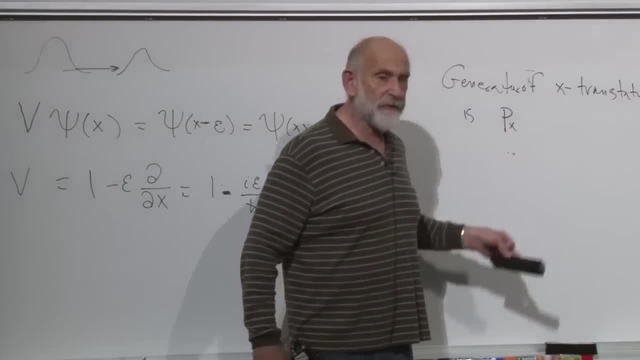 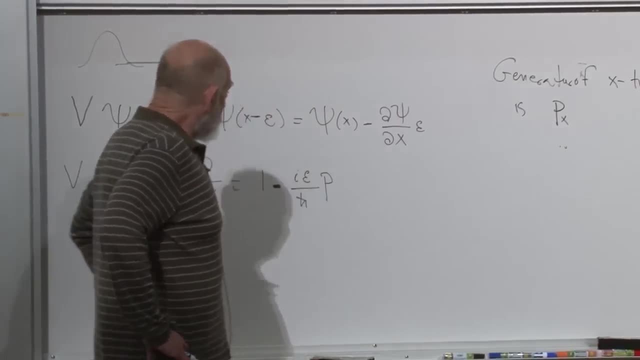 constant. I will drop the Planck's constant and, as a matter of fact, the definition, the official definition really doesn't have the Planck's constant in it, But there's an example. There's an example p of x. now. 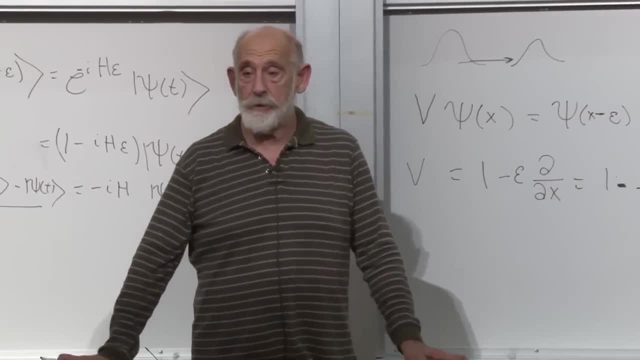 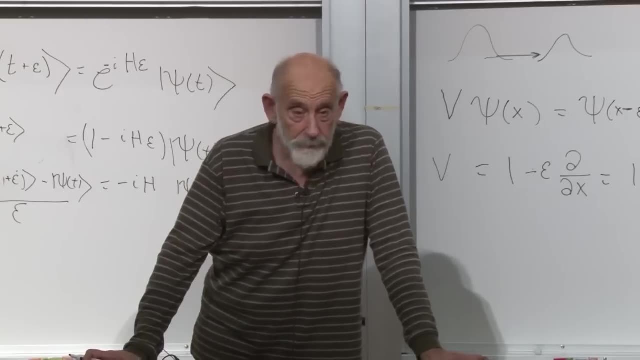 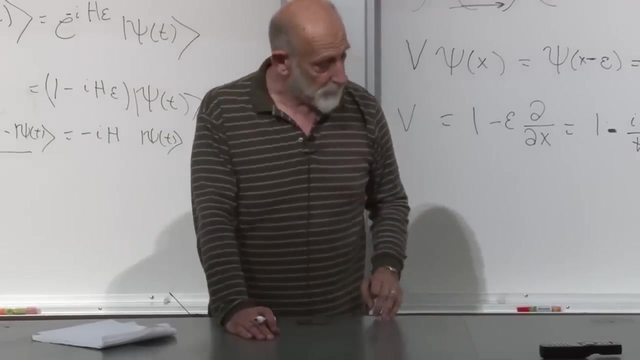 is p of x. is the momentum along the x-axis conserved? Depends on the Hamiltonian. It depends on the Hamiltonian. So let's write down a Hamiltonian. The Hamiltonian for a free particle, a particle moving in empty space with no. 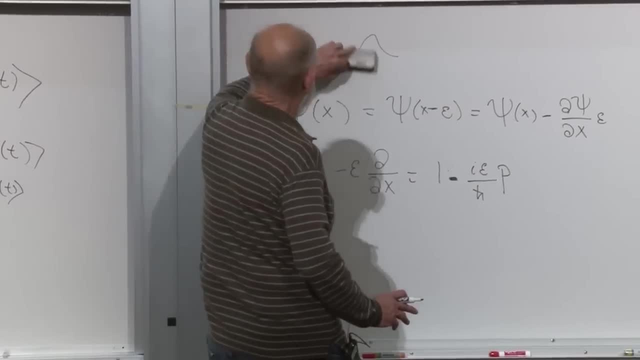 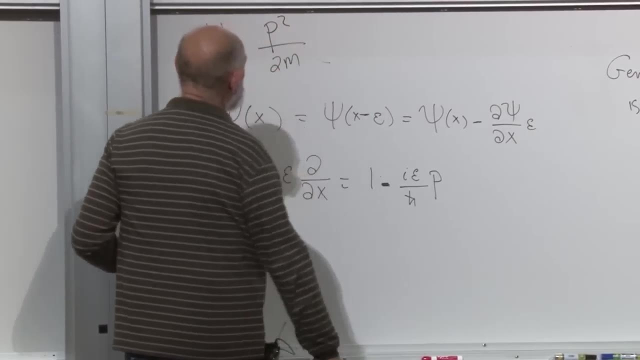 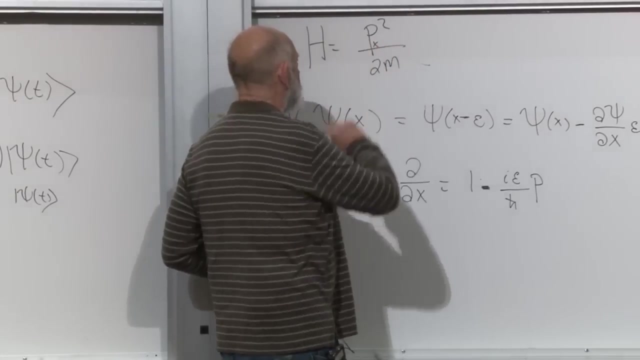 forces acting on it. h, in that case, is just p squared over 2m, The momentum squared divided by twice the mass. If this is a one-dimensional problem, then it really is just px, just the x component of momentum. 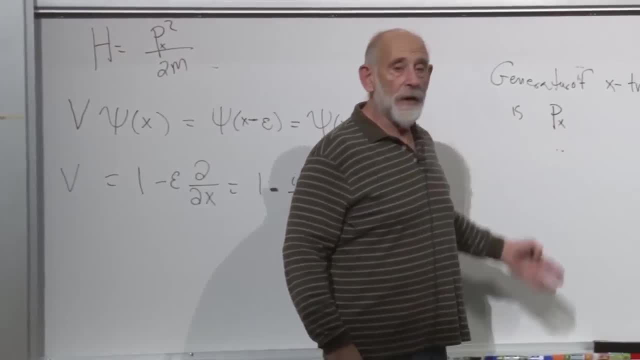 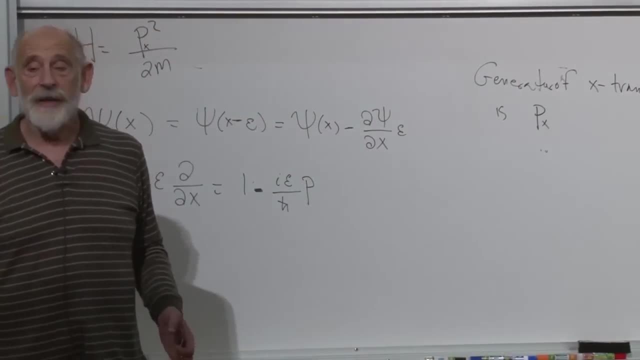 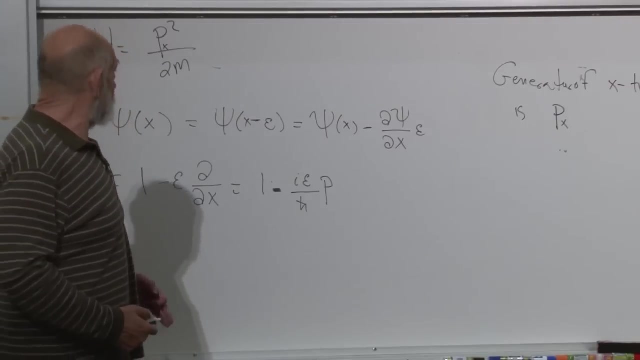 Does the x, does the Hamiltonian commute with px? Well, that becomes equivalent to the question of whether px commutes with px squared. Yes, Every operator commutes with every function of itself. p of x commutes with p of x squared. 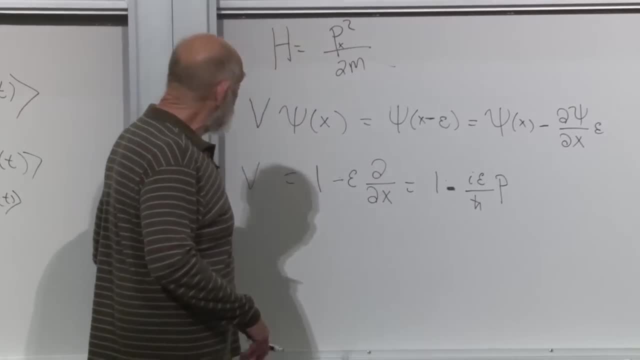 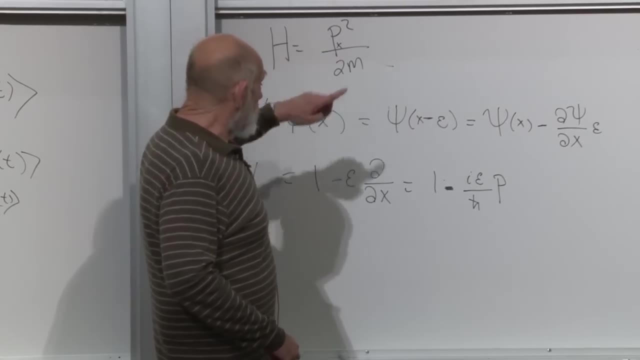 it commutes with p of x. cubed it commutes with any function of p of x. So for a free particle moving along the x-axis. we first of all find that the momentum is conserved and of course we also have a translation. 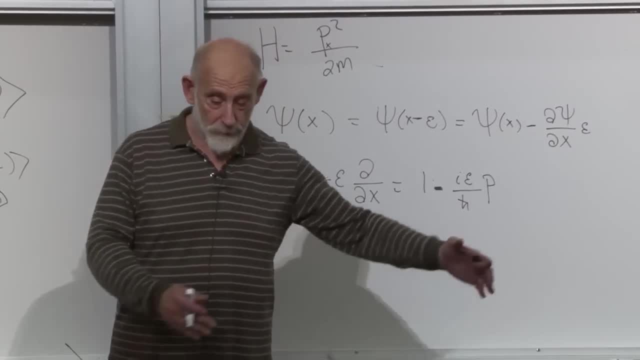 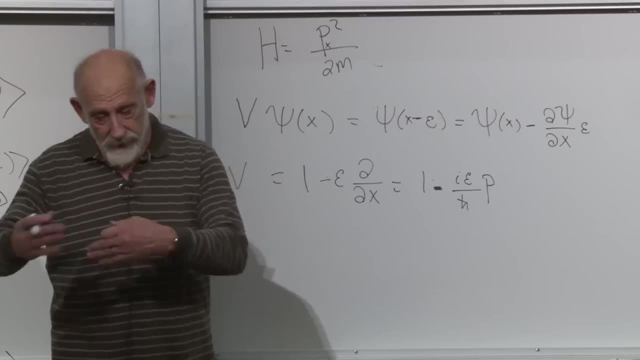 symmetry. The translation. symmetry is just the fact that the free particle will behave the same way wherever you start it. If you start it here and it gets to here, then if you change the starting point, everything will just translate. Okay, so that's. 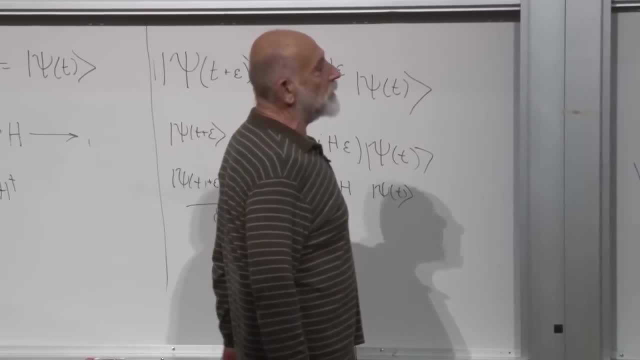 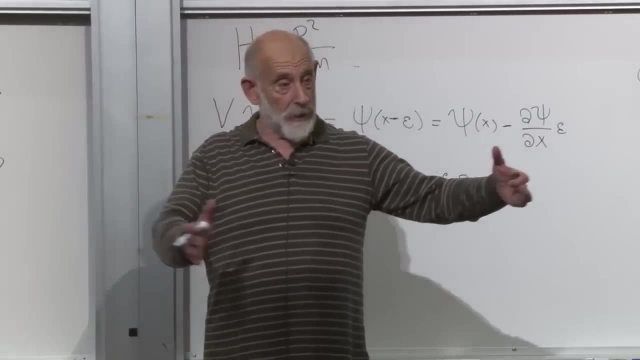 an example: p is both a conserved quantity and the generator of translations. What if there are more directions of space? If there are more directions of space, then there are several symmetries. You can translate: along the x-axis: you can translate: 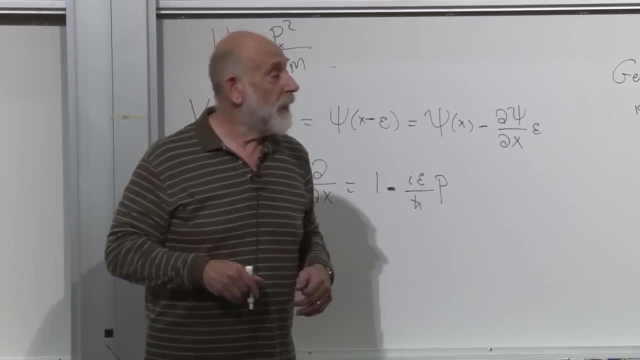 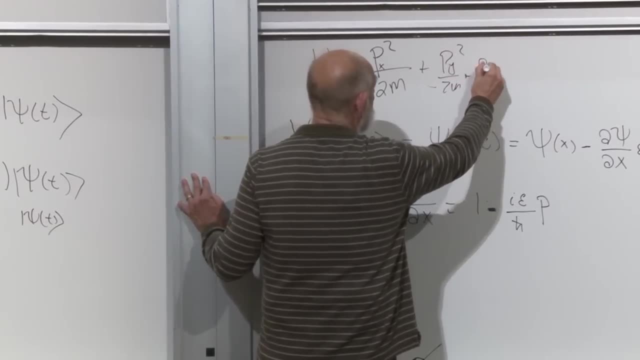 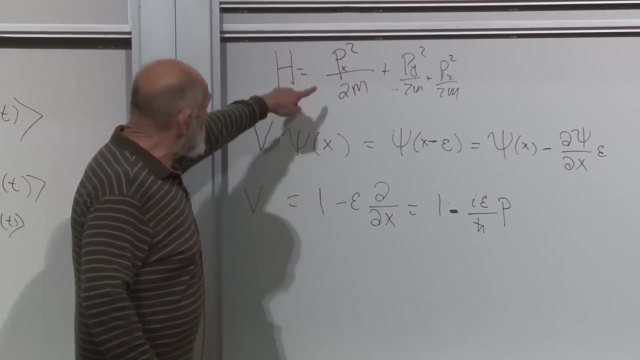 along the y-axis. you can translate along the z-axis. In that case the Hamiltonian becomes px squared plus py squared over 2m, plus pz squared over 2m, And the translation symmetry along the x-axis is still just px. 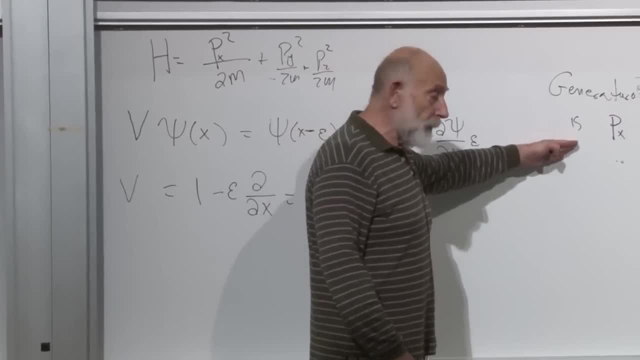 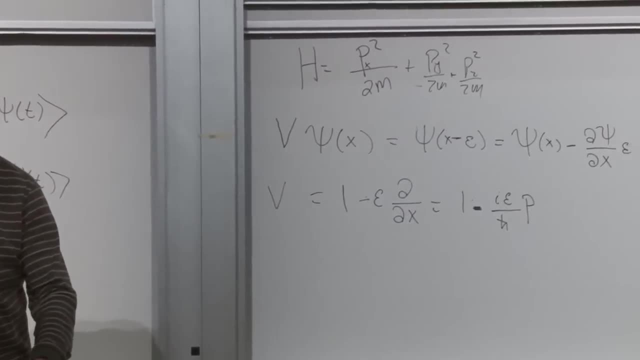 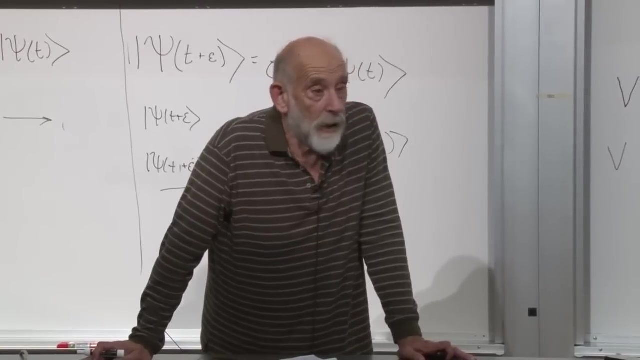 Translation along the y-axis, the generator is py, and so forth, and each of them commutes with the Hamiltonian. So this is an example of the connection between symmetries and conservation laws, which is very simple. The next time it looks like we're about out of time. 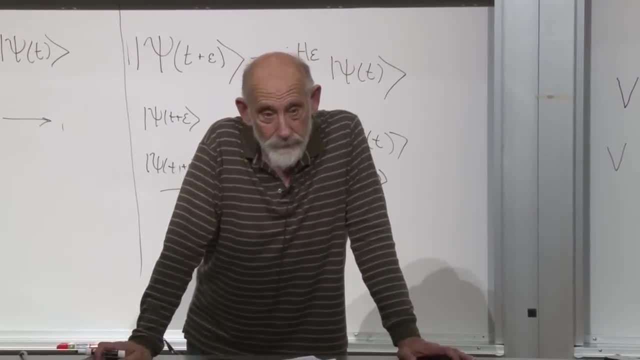 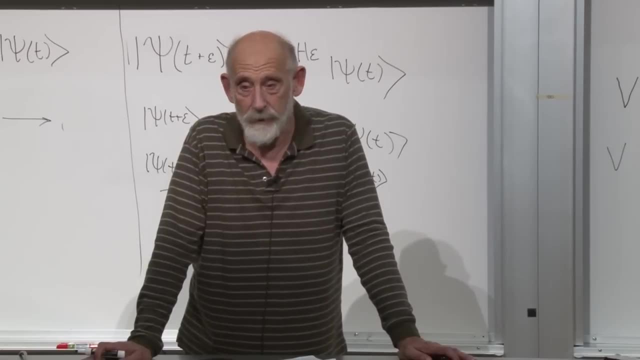 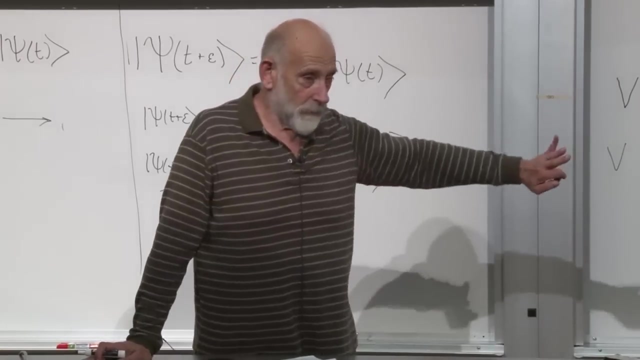 but the next time we will do rotation symmetry. Rotation symmetry is much more interesting, it's much more involved and it will bring us to the subject of group theory. There's some group theory here, but the group theory is completely trivial. 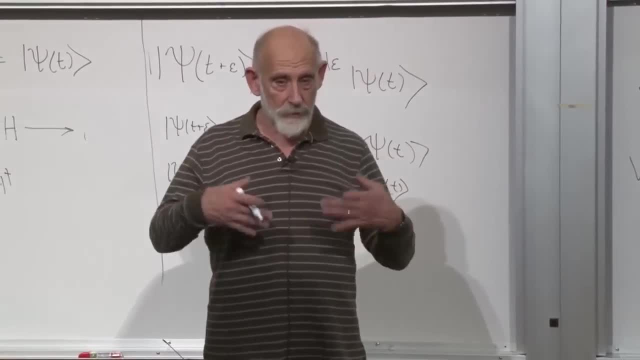 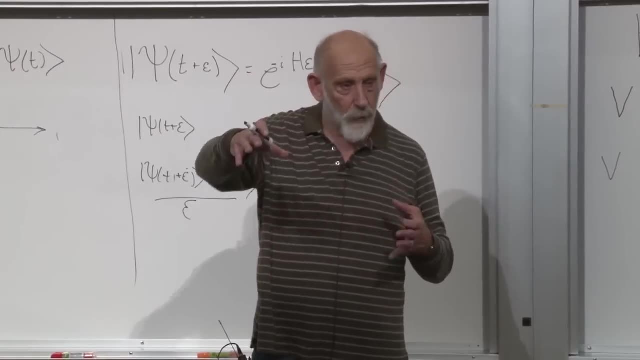 The next time we will talk about rotations in space. and what's interesting about rotations in space is they don't commute with each other. A rotation about x followed by a rotation by y is not the same as a rotation by y. rotation by x. 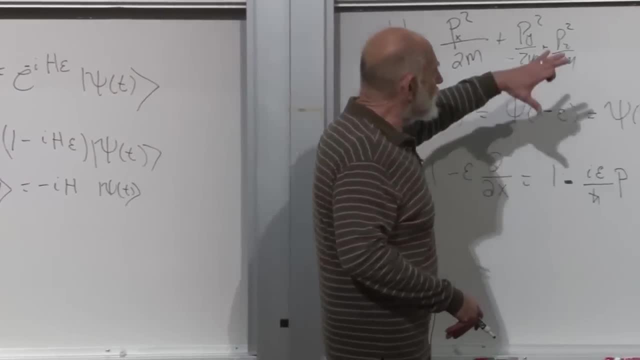 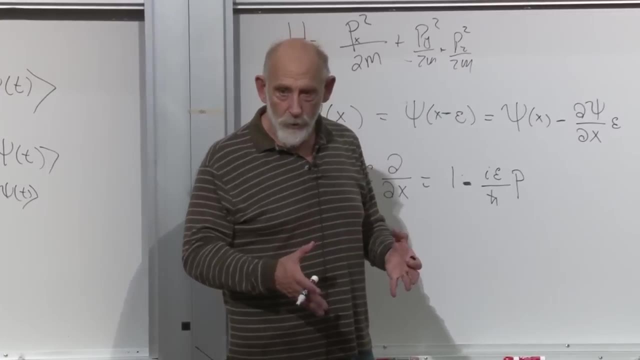 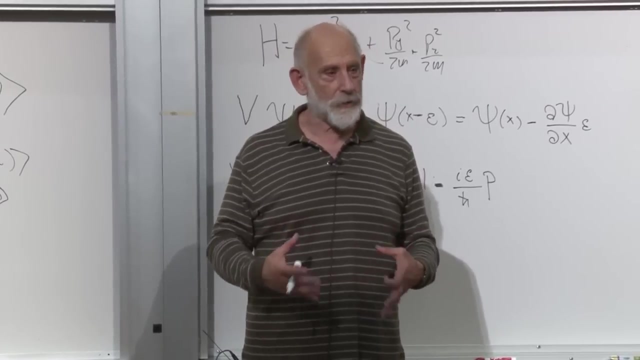 And that will give us the idea of non-commuting symmetries, Symmetries, collections of symmetries which don't commute with each other. and when we find those, they have power. They have real power to tell us about all kinds of physical properties. 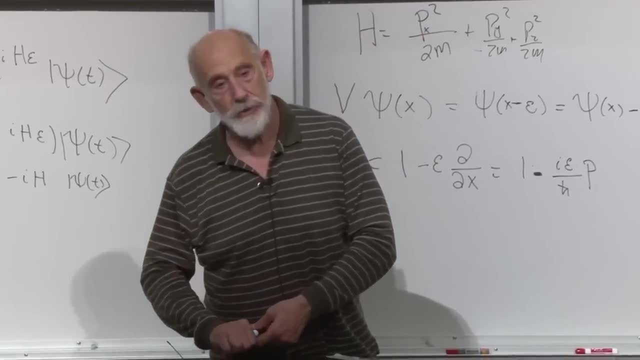 of a system. Okay, so next time, rotation symmetry. For more, please visit us at stanfordedu. 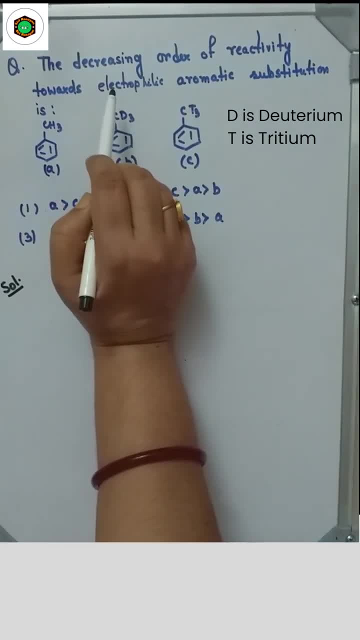 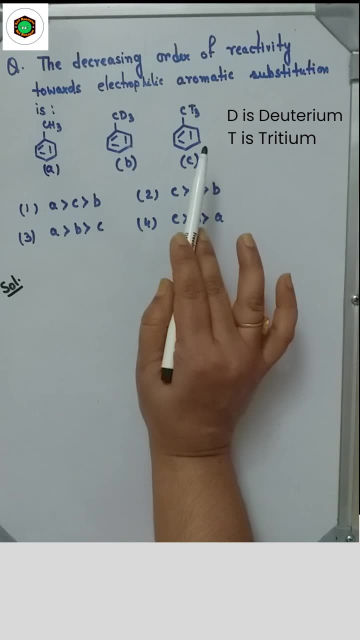 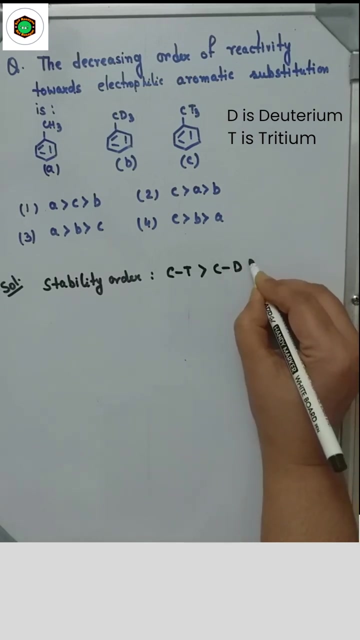 Hello students, welcome back to SIRPRASAYAN. In this lecture I will explain. the decreasing order of reactivity towards electrophilic aromatic substitution is three molecules are given. four options are there? CT bond is more stable than carbon deuterium bond. It is more stable. please subscribe. Thank you for watching.